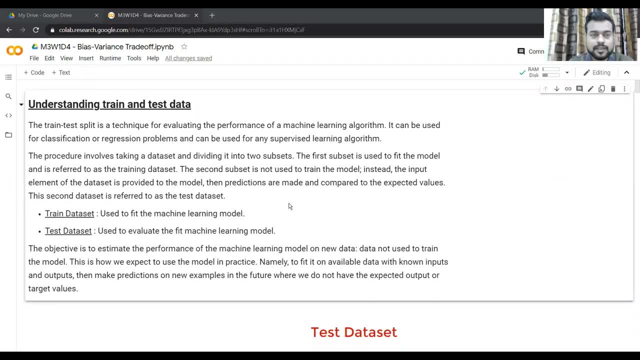 to dive into what is bias and variance. Firstly, we want to understand how training is basically done and why we want to spread our whole data set, which we have at our disposition, into train and test. So yesterday you saw the first implementation of the linear regression in. 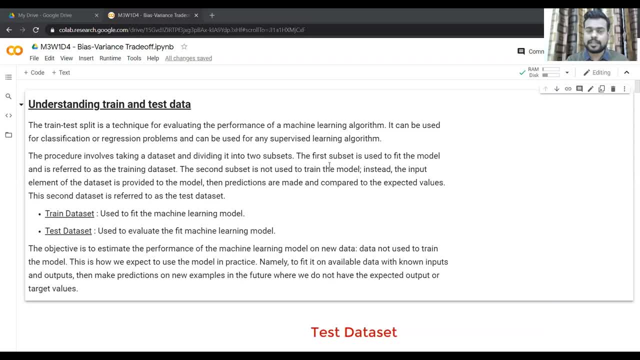 which the data set was divided into a train data set and test data set. Usually we have 80% or 75% data as trained and the remaining as test. So whenever we are training a model, we only allow the model to look at the training observations and then, once that model is trained, 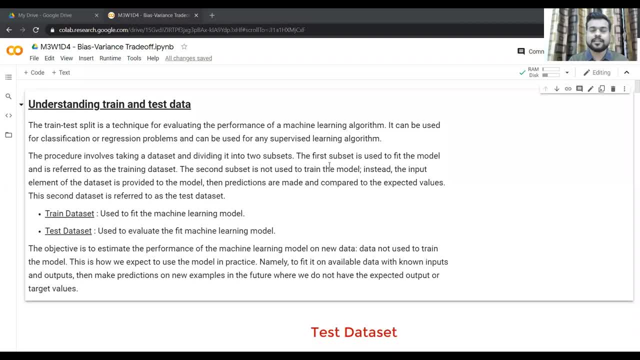 as in, the parameters of the models are learned using the training data. we use that same model to test on the our test data set. So the training data set was divided into a train data set and test data set. Usually the training data set was divided into a train, test and test data set and see how our predictions 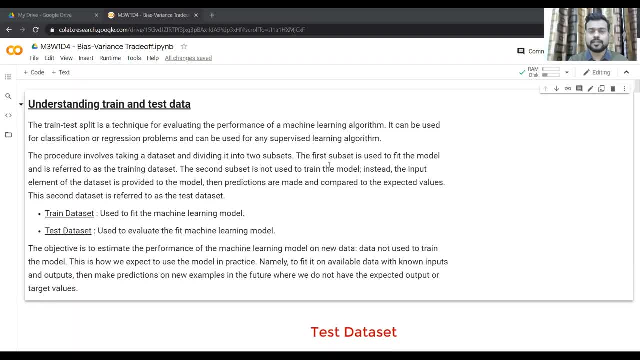 hold. Okay, so this is a very important concept. So the train test split is a technique for evaluating the performance of a machine learning algorithm, So it can be used for any classification or regression problems and, of course, can be used for any supervised learning algorithm. 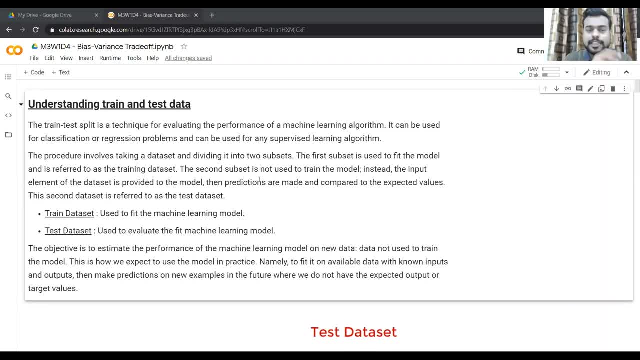 So, as you're already familiar that this procedure involves taking a data set and dividing into two subsets, that the first subset will be used to fit the model and which will be used to fit what we refer to as the training data set right, The second subset is not used. 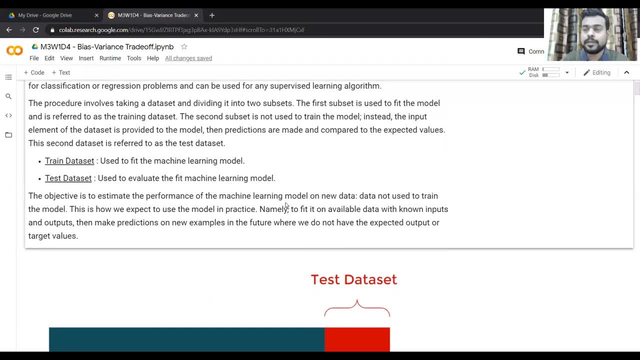 to train the model. Instead, the input element of that test data set is provided to the model and then the model comes about, comes up with the predictions, and then we match with the actual values we have in our train data set. So when I say actual values, so of course, 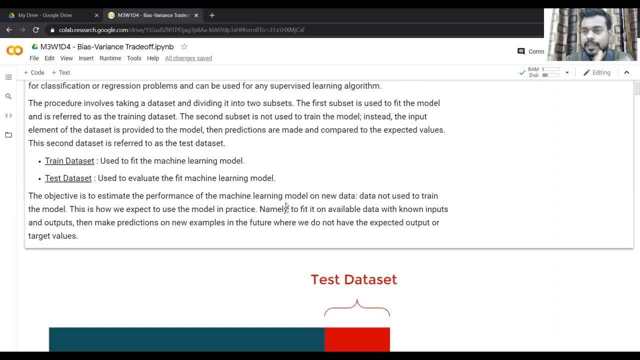 I'm referring to the dependent variable, right? So you will be essentially out of the model. Our objective is to model the dependent variable. So when we're making predictions, so we are predicting the dependent divide. that is the dependent variable, So we have one predicted. 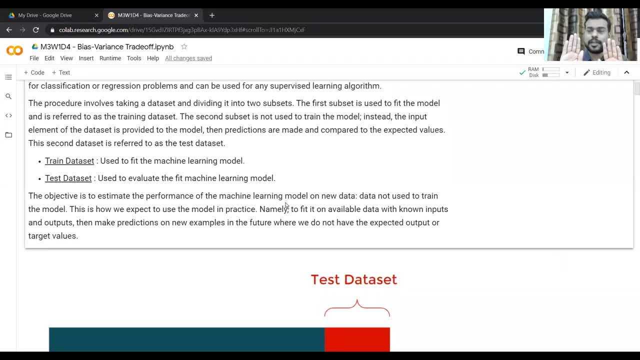 value and a list of values, and then we have corresponding actual values and then we try to see how much deviations are there from our predictive set of values, and the actual value- and that is how will be- will sort of evaluate our machine learning algorithm, right? 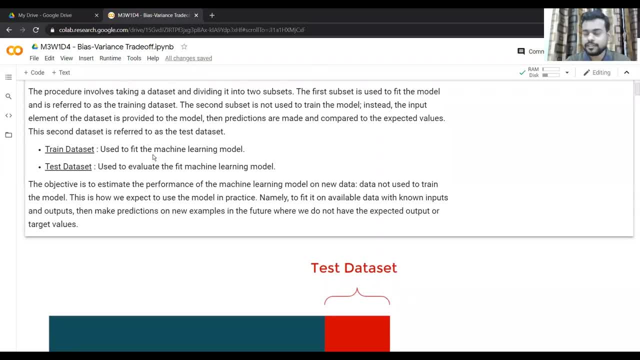 So Yeah, so the train data set is used to fit the machine learning model. So whenever I'm saying fit to fit, that means there are some parameters of the of any machine learning algorithm, right? So for linear regression you have beta naught, beta 1, beta 2.. So these 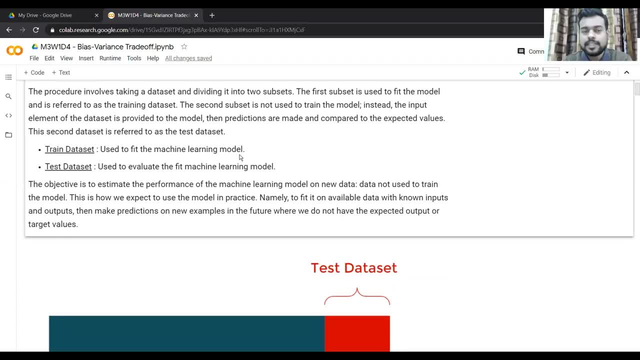 are referred to as the parameters, and using the train data set, Our objective is to learn these parameters. So for any, let's say, a particular data set you are given, so beta naught can take. so after that training has been complete, So beta naught can take value, Let's say 2.5. 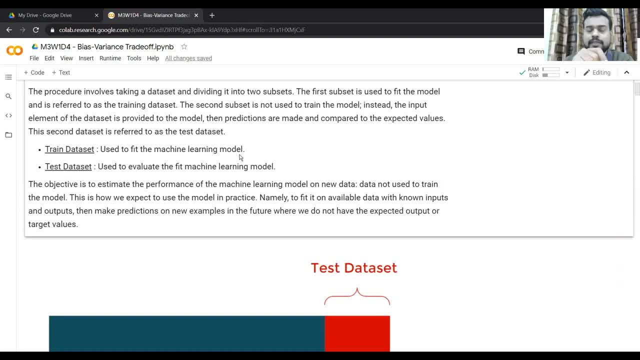 beta naught. beta 1 can take value to. beta 2 can take value something like 3 for a given train data set right. So once that model parameters learn and wonder, once that model has been trained, so that means our algorithm which is trained, or the machine learning model. 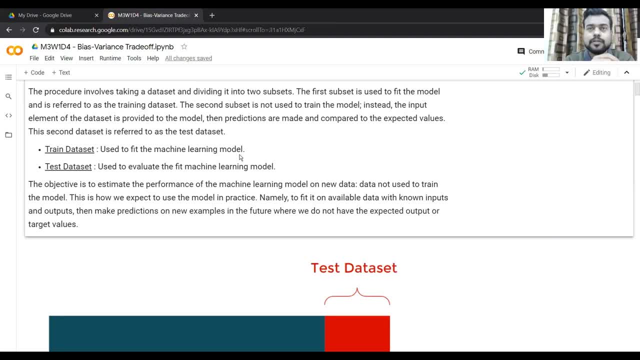 will now look. for example, in the case of linear regression that will look as: so I can say I can write that for you, Right? So I let's say that function can look like something to plus, let's say, 3.5 x 8 plus 6.5.. So this can be X 1 X 2, something like this, right. 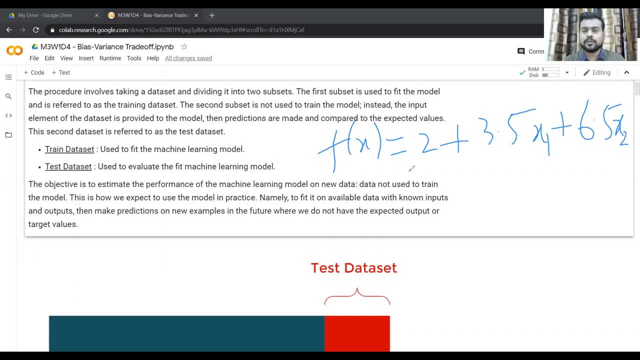 So this is our model And so for any input data in our test- okay, so we'll pass that into the here, So we'll file. We'll allow this function to take the values of x1 and x2 for a given test data set. Okay, so so of course. 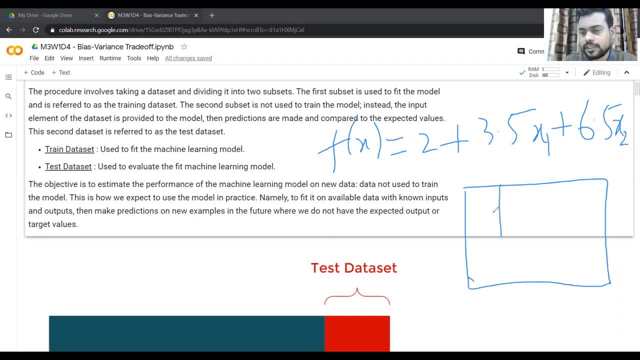 I don't think I need to re-emphasize over this, but let's say I have this test data set, something like this: So these are x1, x2, x3, x4.. So it will have some value. let's say 16, 10, 11, 12, right? So these values will be plugged in here, right? And then there will be a corresponding. 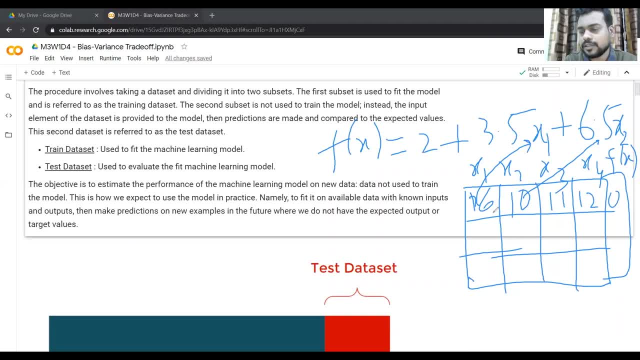 value for this FX right. So for these set of values will have some values- something like this or something like this- and then, of course, we already know what are the actual values in our test data set and we can then compare our predictions and the actual values. 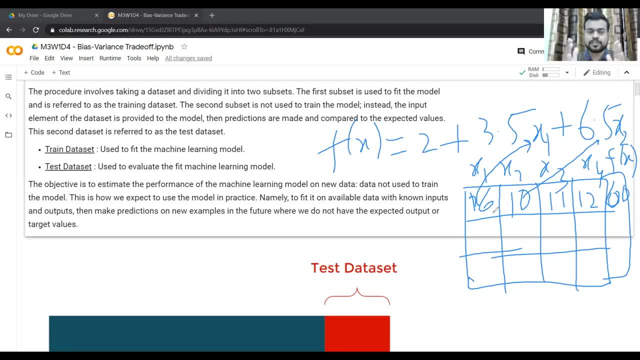 right by putting them side by side or in juxtaposition and then we'll be able to see how much deviant data Our predictions are from the actual set of values of y in our test data set. So I hope the this particular concept is clear to you. Can you let me know if this particular idea 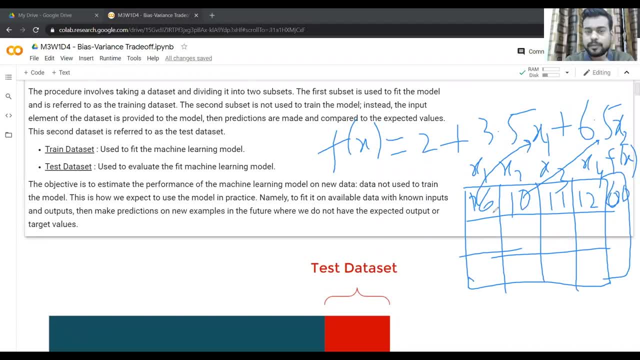 is. the concept of train and test is now familiar to you. If not, let me know what concerns you have and I'll try to clarify these, and then we can move forward. right? So this particular concept is very easy to understand, right? 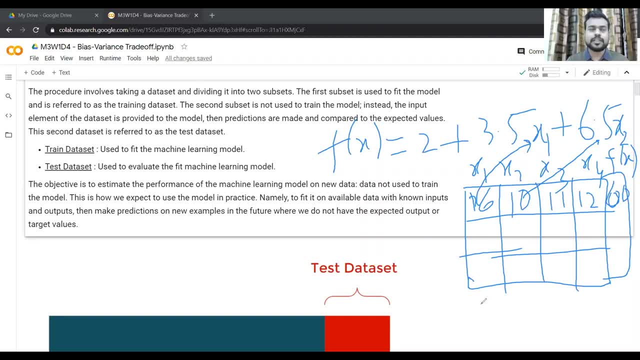 So when we're talking about training, any machine learning algorithm, as in so, will take any function. So, for example, in linear regression, we took this linear function which is linear in the parameters right And our objective would be to learn these parameters using the. 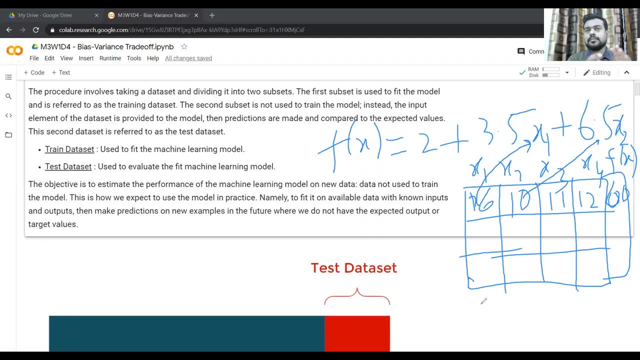 training data set. Okay, and so we have the set of independent input features and using this parameter, We're trying to sort of learn the dependent variable, which is why, okay, So using the training data set said, we learn these parameters right. So always consider this in mind that when you 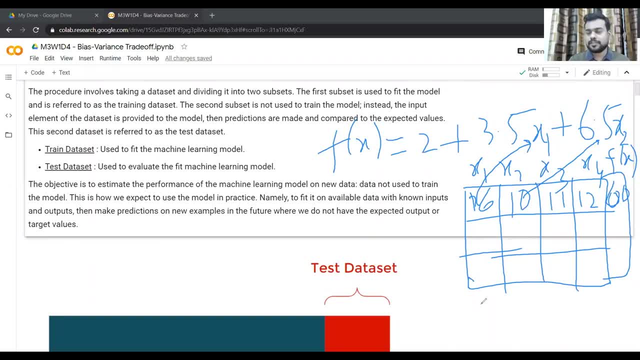 mean training. you are essentially learning the model parameters. So, in the case of linear regression, we have these beta naught, beta 1, beta 2, but for different algorithms will have different set of parameters to deal with. Okay, so so. yeah. so, once we have learned, 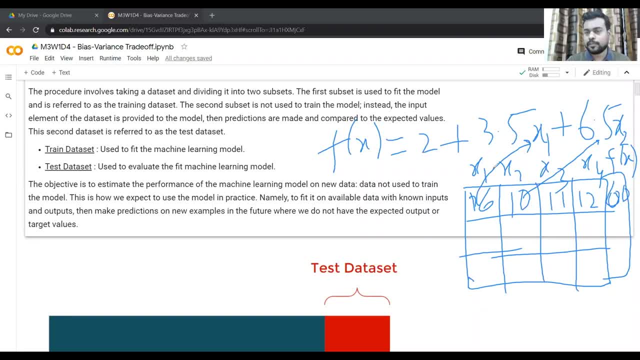 we have got in the learned parameters, as in these values, let's say 2, 3.. So, essentially, you don't know what these values are, right. So these are: beta naught, beta 1, beta 2 and, using the training data set you'll find, come up with this values: beta naught, beta 1, beta. 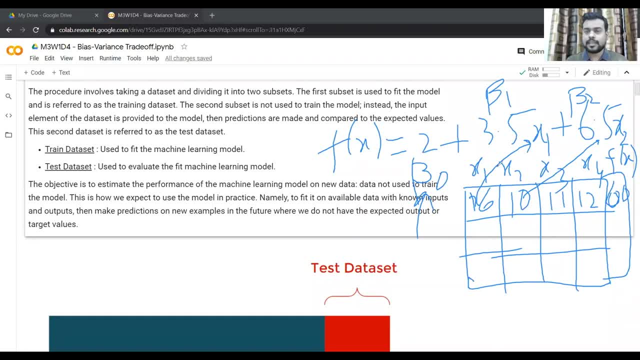 2, and how will come up these values? So, by using the gradient descent algorithm, in which so will minimize the loss function with respect to these parameters which are beta, naught, beta 1, beta 2 and something else, and then yeah, So once the 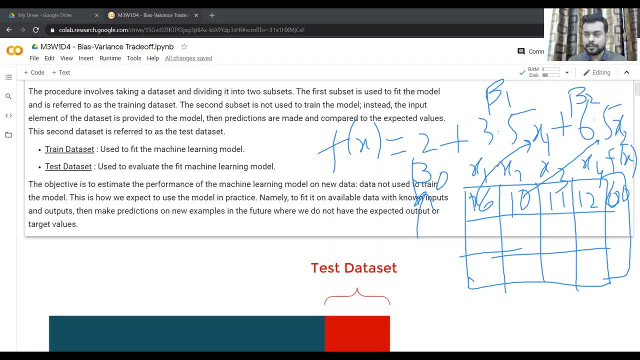 these beta naught beta 1 and beta 2. all these parameters are known using the training data set, right? So that's the best set of values which we can come up with by looking at that particular training data set. So we still haven't allowed the model to look at the test. 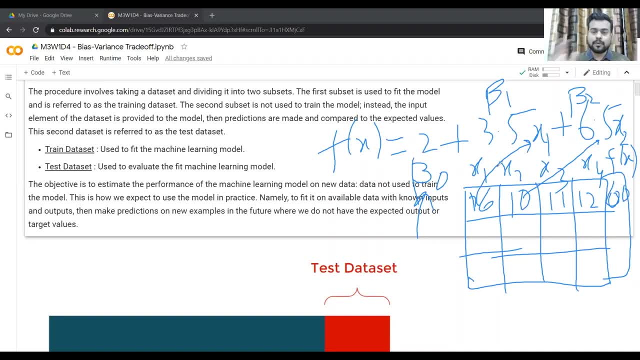 data, observations or test data set right now, once these, once we have a function, right, So we now pass each observation of our test data set into that function and for each observation we get a prediction, And then for each observation or test data, we already know the value of the dependent. 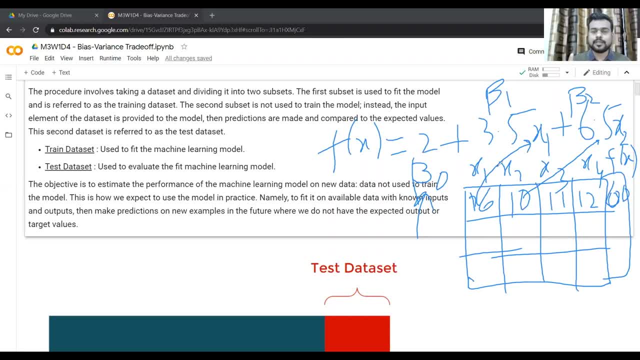 variable, and then we can compare the dependent variable value and or the Y value with our predicted value. And for R we take this result to see how much deviant they are. So we can look at the squared deviation from them for the two right. so 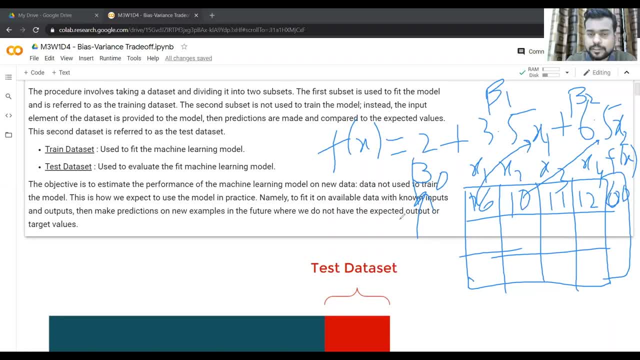 So Chinmaa is asking: if you want to find residual for vector mean of y test and y pret, is this important to? will it be zero or close to zero? so so, essentially, when you're calculating so the mean of residuals, we would expect that to be closer to zero. so when? 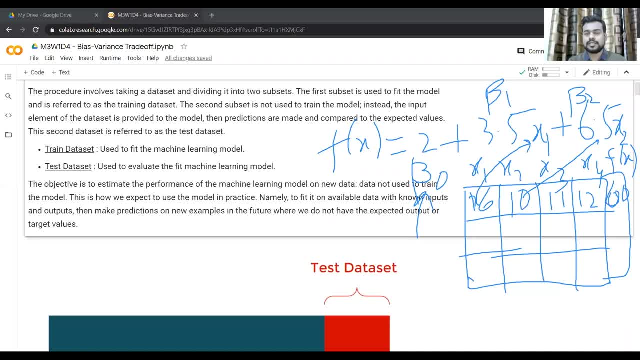 you're just taking the difference right. so we expect our model if, if that satisfies all the assumptions, so yeah, so I think the idea is clear. so the objective is to estimate the performance of our machine learning model on new data. what so, this test data? we also refer to this, this as: 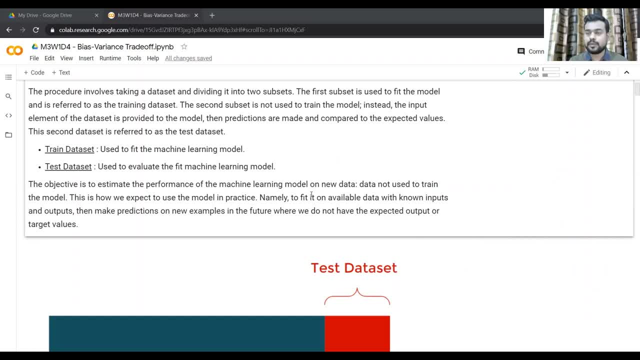 unseen data right or new data, so the data which is not used to train the model, right. so this is so, once we have trained our model, now our object to be would be to see how this model is performing on any test data set. So we'll make some sort. 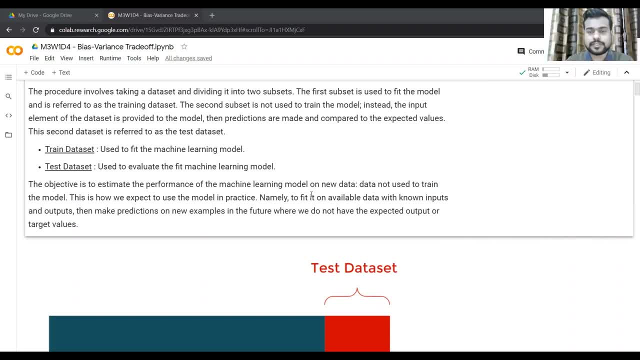 of predictions and we'll try to see how this fares right, So nice and so to. will fit it on available data with known inputs and outputs, and then we'll make predictions on new examples, right, So. so here what is saying that will make predictions on new examples in the future? 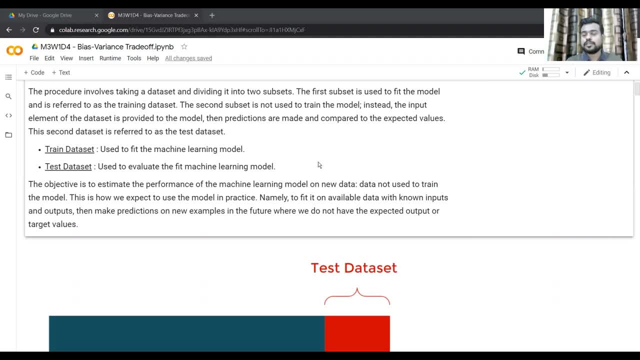 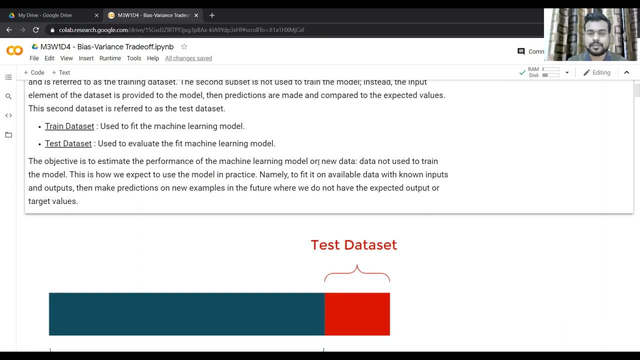 with we do not have the expected output or target value. So so let's say we build actually a built machine learning model, We trained our model and so we'll, let's say we put that in the production right. So where that model is based on any input set of features, it is. 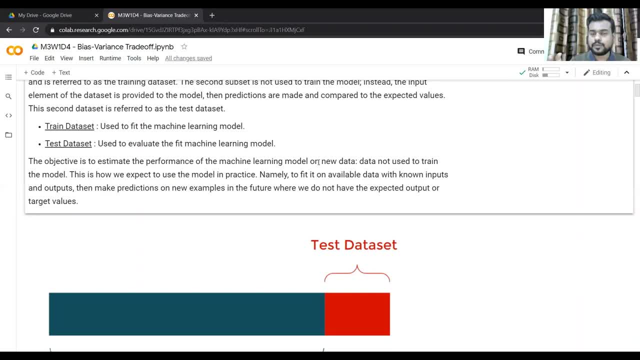 making some prediction, So whatever things which we're trying to predict. so let's say, in case of stock prices, So we want to predict today what will be. the stock price over means tomorrow, right. So today, when we are getting the predictions based on the observations which we have today, 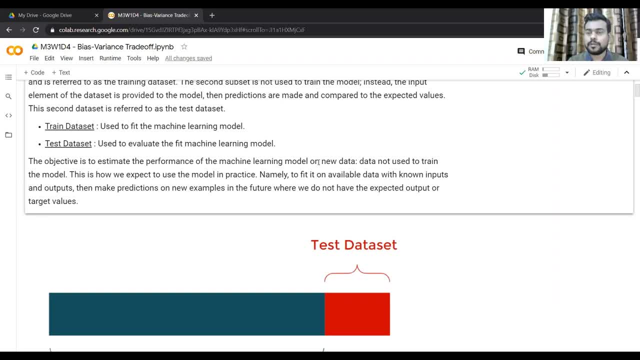 right? So we won't know what will be the actual value until tomorrow. right? So we have made our prediction. So let's keep that prediction with us. We wait until tomorrow, So we'll see what will be the stock price tomorrow and then we can compare how the prediction 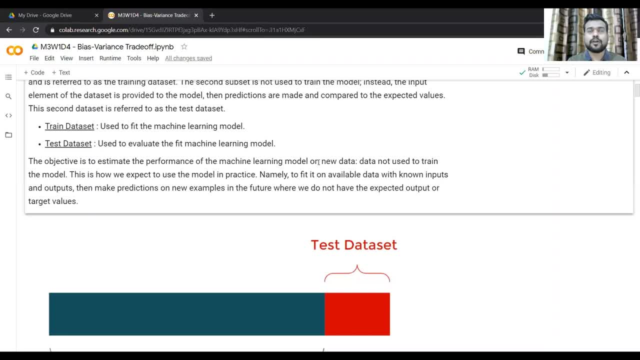 actually was right. So this is a talk, This is. this occurs when we are talking about the using our model in the real time environment, right, But essentially, when we are doing modeling, let's say when we are training our model in our system, we are not deploying in real time. 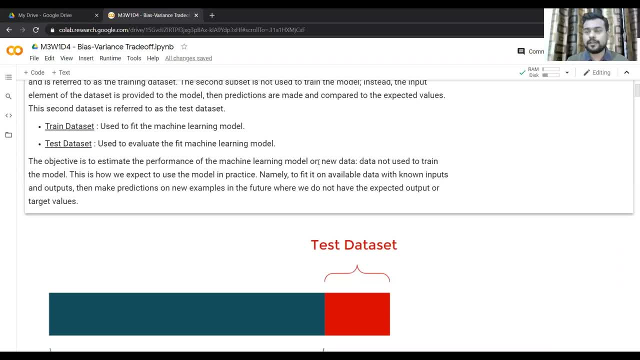 So essentially we want to figure out what's the performance of our model. So we'll have a test data in which the value values or the output variable will also be known. But the thing is, the test data set will not be the actual value of the model. So we want to figure out what's the performance of our model. So we'll have a test data in which the value- stable value of the model at some point in time- that's by using the control news in the variable problem- set, So we will be able to tell you right. here are five values of: 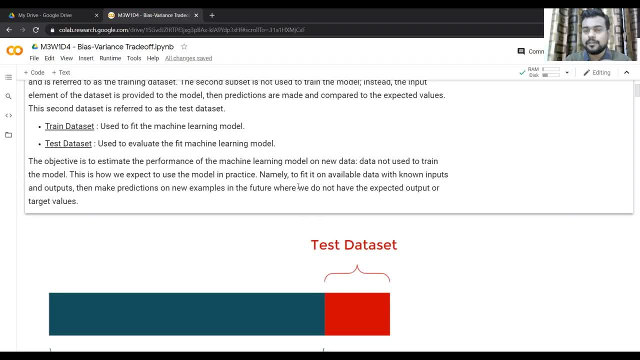 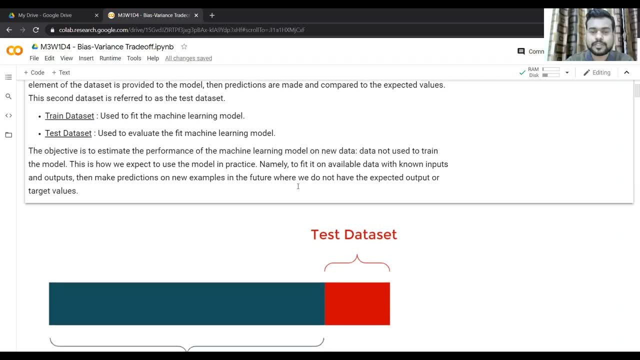 the model end with the output virtual data set that can be used during training right until at level four, And then we will be able to compare our predictions and the corresponding value values right. So, in general, what we do, so we take a major chunk of our whole data. 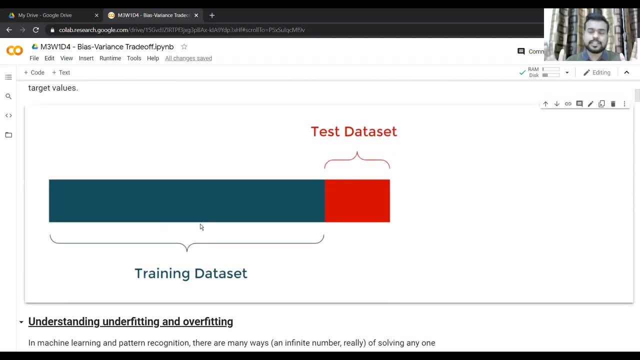 set which is available to us. so we take almost less 80% and 75% of it as training, and then we have some 25 PV, 25% of stress. Okay, that was 15%, So it differs. so whether it should be 80% or 75% or even 70% for train, that depends upon people to people, but in general practice it's: either you can take 80-20 split or you can take 75-25 split. 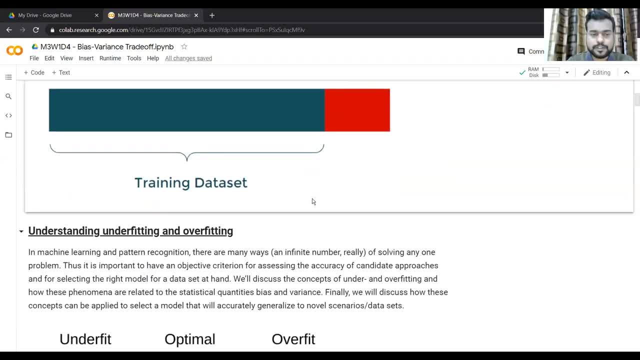 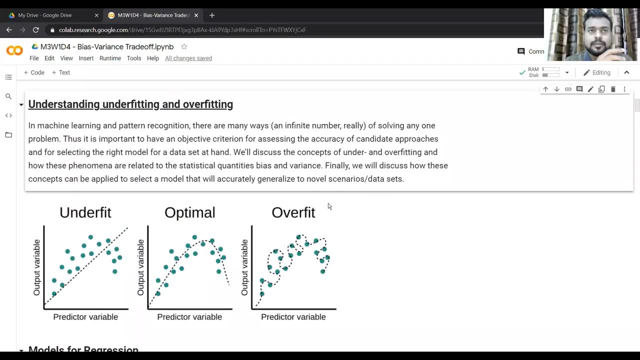 Okay, so that's upon you, Okay, So, yeah, so moving on. Yeah, So now we understand the importance of having, importance of doing the train test split, right. So we want to train our model on the train data set And then we want to see how the performance looks across the test data set. Right, 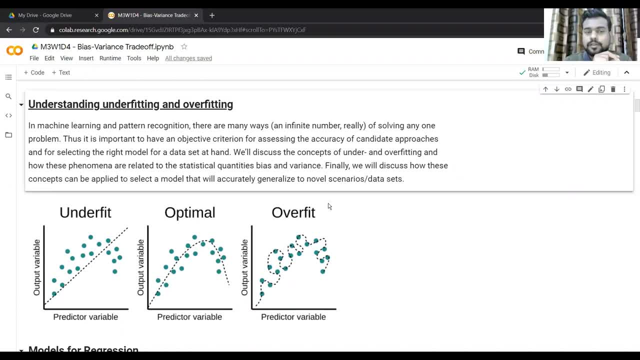 Now moving on. So there are two very important concepts Which I'll be covering today. So this is underfitting and overfitting. So when you are dealing with any machine learning problem, So there are many ways to solve that particular problem. So that's why it's very important to have an objective criterion for assessing the accuracy of all these candidate approaches that we can come up with and and based on this assessment, 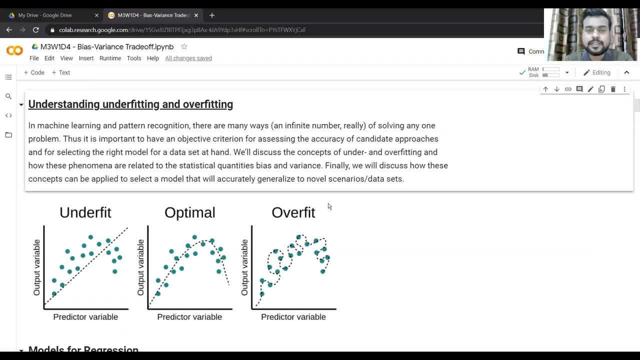 We can come up with the final write model for the given data set, Right? so how can we come up with the right set of model? which models are the best? right, So we can. let's say we currently were discussing linear regression, but we can have some SVM regression as well, or we can do regression using the neural networks or decision trees. 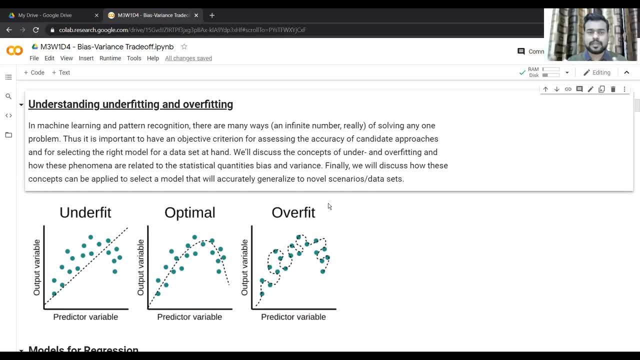 So we have all these different models at our hand, Okay, And for a given dataset, let's say, we try all these four, five approaches, And then we want to figure out which model we want to go ahead with. right, so the so to make this assessment, we'll need: 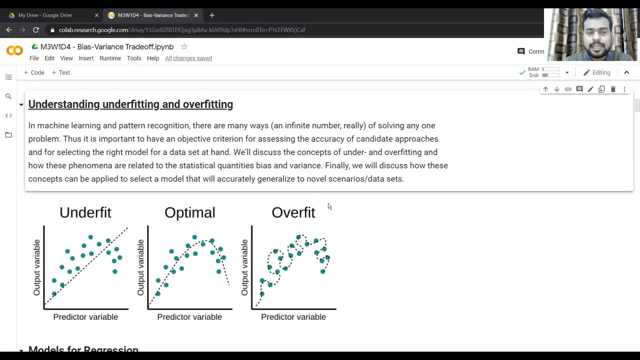 to understand, firstly, the concepts of under and overfitting, and we'll also get to know how these phenomena, that is, the underfitting and overfitting, are related to the statistical quantities which are known as bias and variance right, and then we'll see how we can leverage. 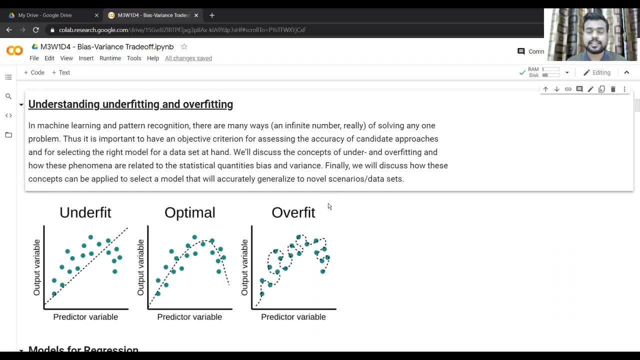 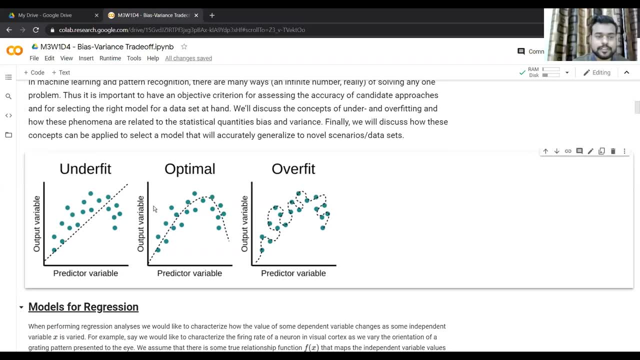 these concepts to generalize to any unseen data or new data set, right? so I'll give you a basic idea of what is meant by underfitting. so suppose you. so suppose I am just talking about a univariate regression, as in: I just have one single independent variable and the 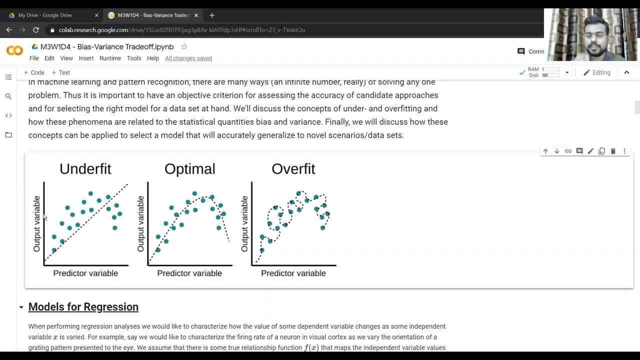 of corresponding dependent variable, right? so I have a pair of value, so one, the first value. so I have this pair of x, comma, y, right? so so let's say x is one variable and y is, of course your dependent variable or the output variable, and so we are having some set of observations. 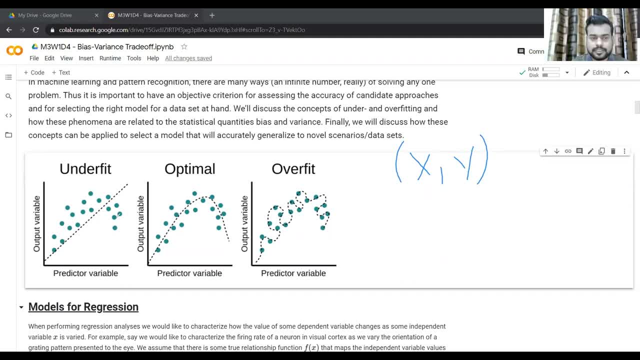 which look like this, right? so these observations in the scatter plot, so these are marked as these blue dots, right? so let's say, if I, if I just fit a single line, right, so for this one, so suppose I have y. y is equal to, let's say something like mx plus c, right, or I can, I should write it: the. 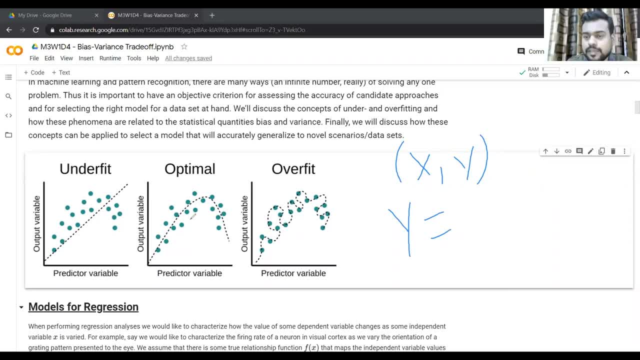 other way, so that that's consistent. right, so I can write beta naught plus beta 1 x, right? so this is how I can write my equation. okay, for this particular case. right? so here we have just created a line, but, as you can see, that this particular, for example, this particular, 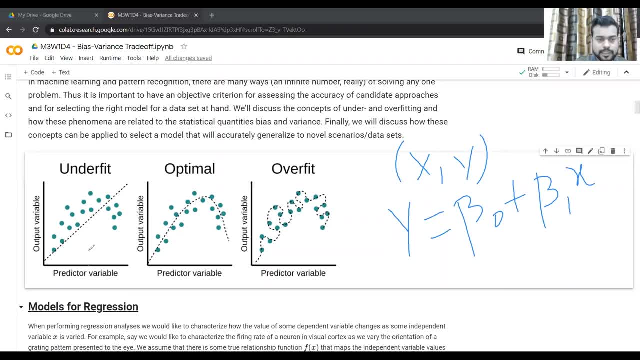 example, let's say for this particular x, right, so for this particular x, so we have this. so, yeah, so for this particular x. so, as you can see, so our predicted or value is this particular right, so, but we can call as y hat, that is, our predicted values, as you can see. 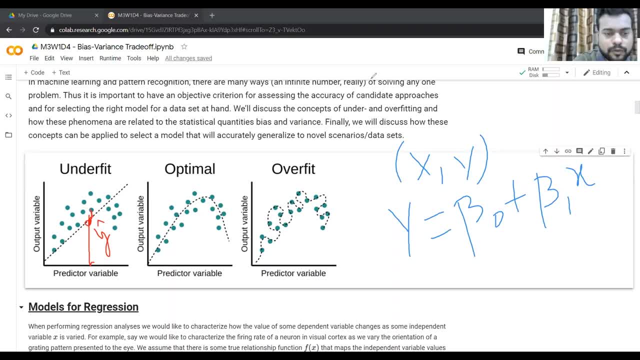 the actual values is somewhere here, right, for this particular x. our predicted value is this one, right? so this particular y hat for this, let's say, x2. so don't confuse between x2 with another variable. it's just another some value for x. so I'll rather write this: 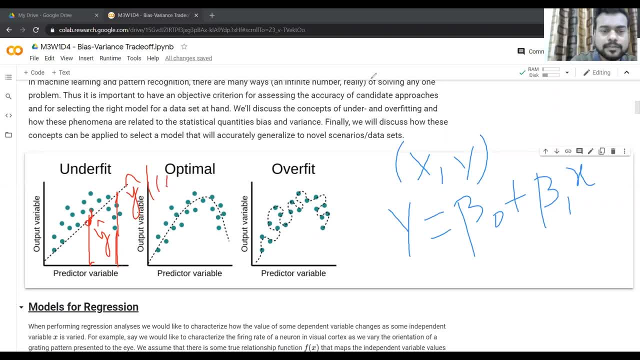 as some value for x. so let's say this could be 10. so what will be the value of this function if x over 10? so based on this line value and this value will be here. but the actual observation is here, right? So actual y value is there. so there is some gap there, right? so this is the gap here. so 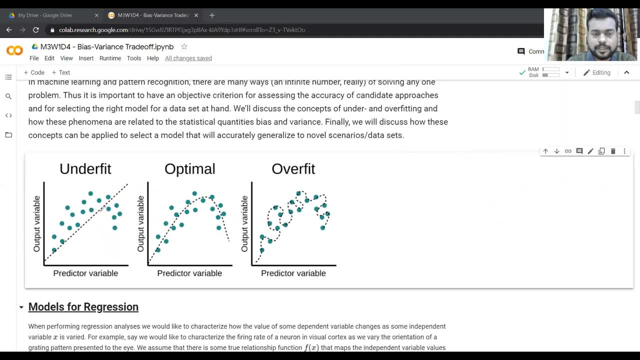 we'll call such a fit for this particular data as under fit. right, so it's. it's not fitting. well to all observations. okay, so, right, so this is known as under fit. now let's look at this particular scenario. so here also we have the same scatter plot right between these. 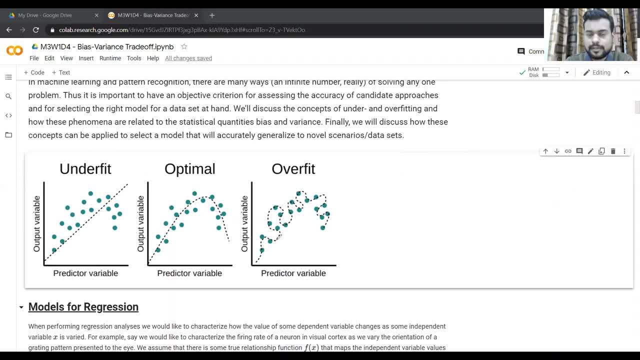 y and x. But, as you can see, This curve is sort of, yeah, it traces over all the points, right. so for each value of our x, right so we, we have a particular prediction, predicted value, or predict, or a value for our function, right, which through which we want to actually model our data, right, and 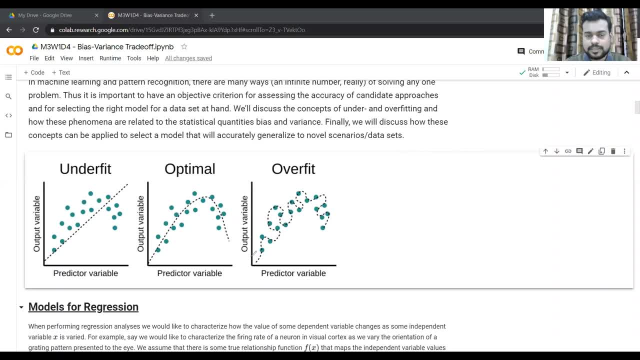 as you can see, that if you are using such a model, let's say: it's, this is some curve right, This is some function and, as we can see, the actual values and the values provided by this function, they're the same right. so so, as you can see, let's say: this is y hat and this. 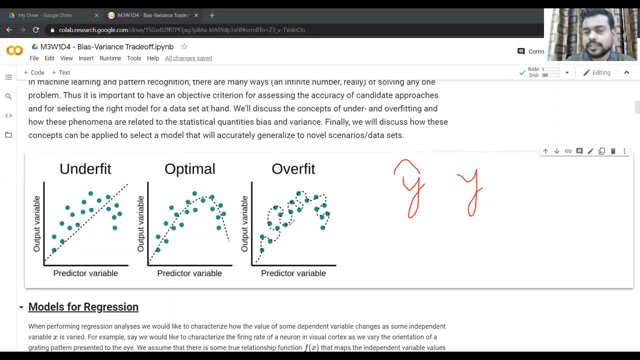 is y actual, so the deviation between this is 0. okay, so for these set of observations, so this is what we call as over fit. so, mind you, let's say, consider that these observations are part of your training data set. okay, So If these observations are part of your training data set, you are trying to learn the model. 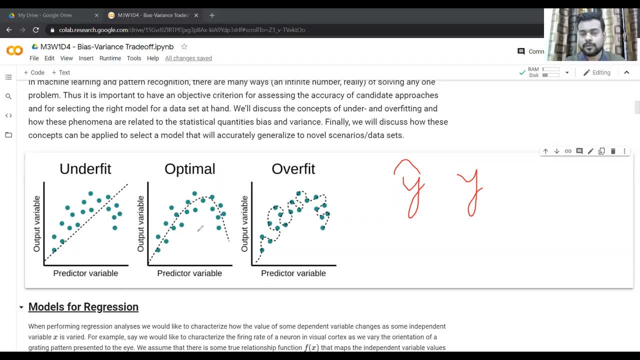 parameters on your training data set, and then you want to come up with predictions on your test data set. So, in this case, in our training data set, we have almost zero deviations in this case, right? so for each actual value of y, we have almost the same exact predicted value, right? so this? 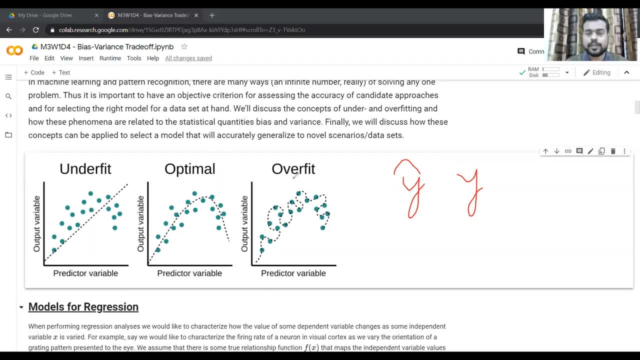 is what we call as over fit. and why is this called over fit? as in, let's say, let's say this is our train and in our test data set, in our test data set, let's say, we have some observations, something like this: right, so, but our model, if we can, yeah, if we allow this model to generalize. 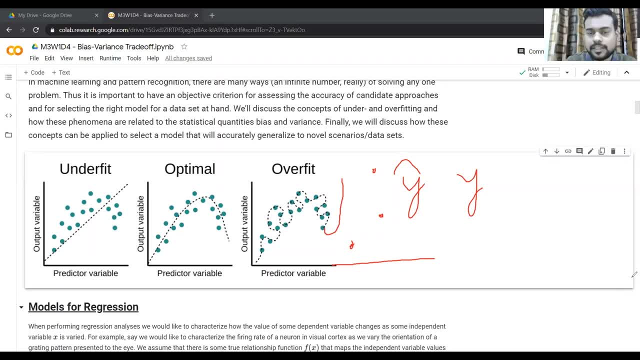 okay, so take on values for some new set of x, so this could be something like this, right, Or something like this. so we'll have a lot of deviations in my set test values for now. I'll come to this concept later on, but just keep this in mind. so better, yeah, not discuss. 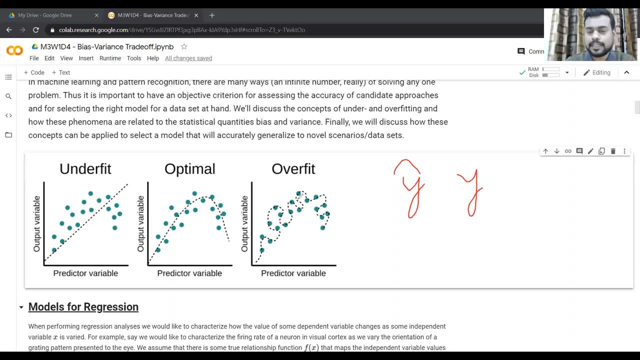 about the test part for now. but just keep in mind, let's say, if in our training data set we are coming up with a function or with a model which has some deviations in my test values, Okay. So if it has almost zero deviations in our train data set, right, so that will be called. 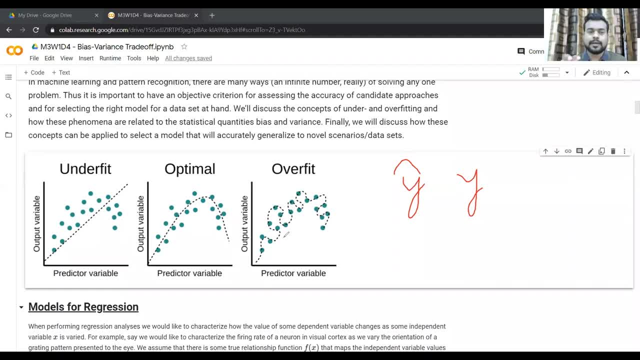 as a over fit, right, so it is trying to actually match for each value of the dependent variable, right? so it's trying to miss get the same exact value for a dependent variable. So that's why this is called over fit in under fit. it's not. this is not the case. but then 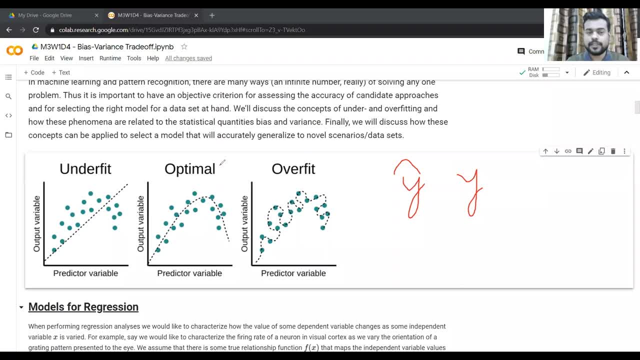 here we have something what we call it optimal fit, or the best fit, as in if you look at the distribution of observation. So this is the curve which, which is sort of an optimal fit for these given set of observations. So it's not exactly fitting on each value of our data set, but it's more or less kind. 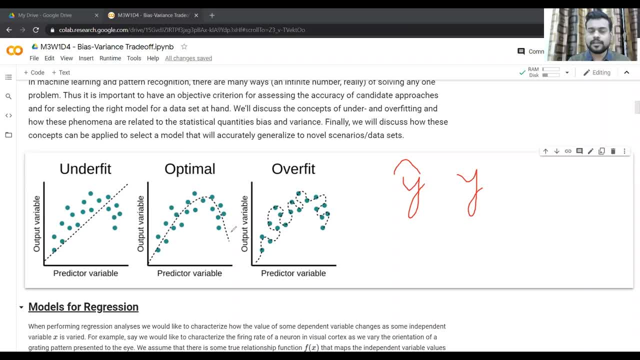 of gives us a very good fit for the observations which we have, right. So, as you can see, so this is not trying to exactly match for each values, but trying to find some set of, find a function, Okay, Which kind of maps the values more or less in a better way, right? 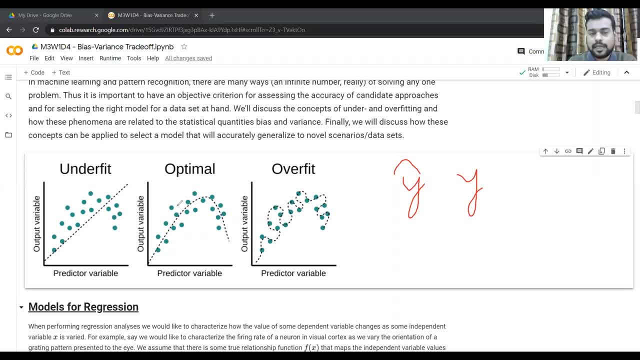 So we'll discuss today, right So, how we can combat this- under fitting and over fitting, right- and how we can come up with this optimal fit, right So, and in which cases will have an over fitting, in which cases will have an under fitting. so we'll be discussing these concepts, so these will become more and more clear when we look. 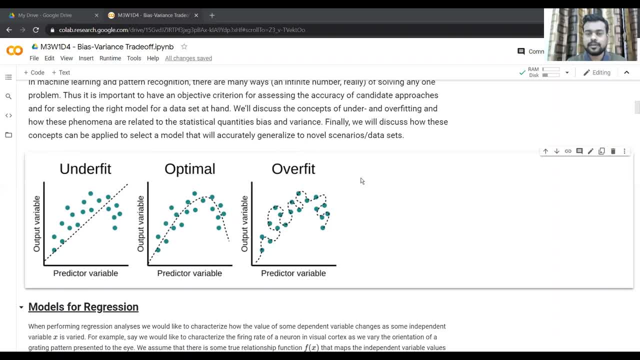 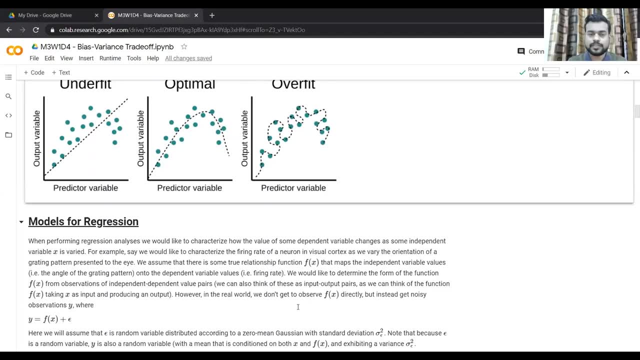 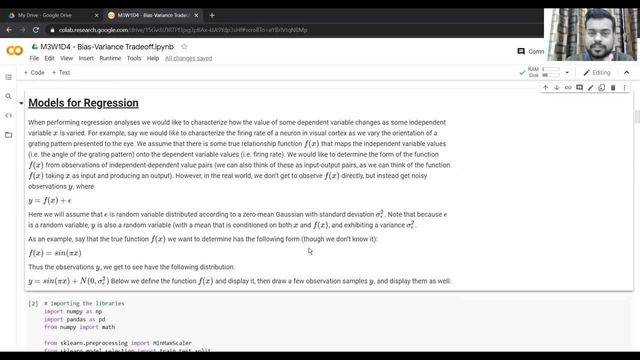 at some examples. So today we will be running some experiments, okay, and through that you'll get to know what I'm trying to, don't get to know what is under fitting and what is over fitting. So, yeah, So, yeah. So when we are trying to perform regression, we want to basically characterize or come. 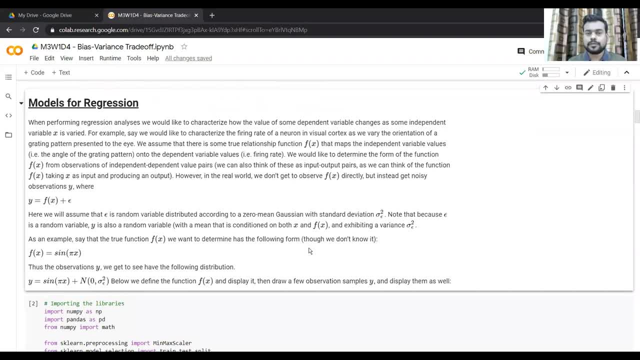 up with a function Which will tell us How it will give us a value of a dependent variable, as the values of X or your independent variable is varied, right? So essentially we assume that there is actually a true little relationship function, fx, which maps the independent variable values onto the dependent variable values, right? 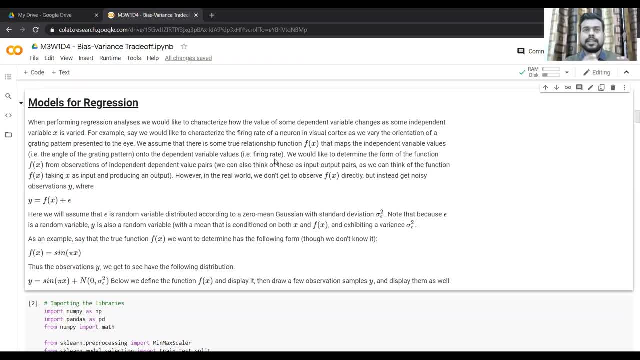 So this is our assumption, that actually this data actually derives from the independent variable values, So there, from a particular true relationship between X and Y. there might not be a true relationship, But we have will make some assumption, and so we'll try to determine this- of the form. 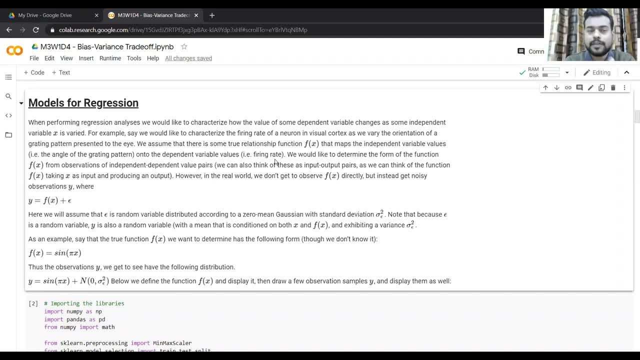 of this function, fx. from the observations which we have at our hand, that is, the training data set. So what observations do we have in our training data set? So these are essentially your independent dependent value pairs, right? So when I'm talking about univariate regression or a multivariate, 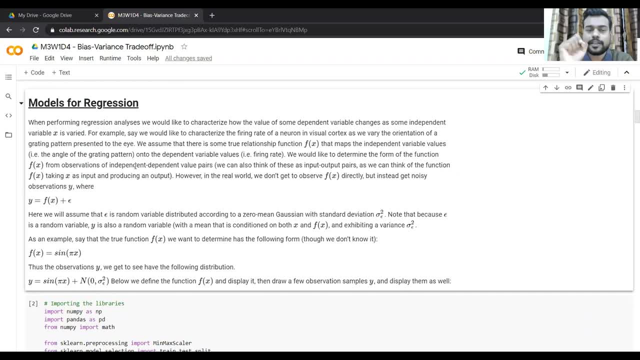 So univariate is single variable, multivariate is multiple variable- right. So we can think of these observations as input output pairs and based on these values we want to come up with a function f. we want to come up with a function which will closely approximate this true function fx right. 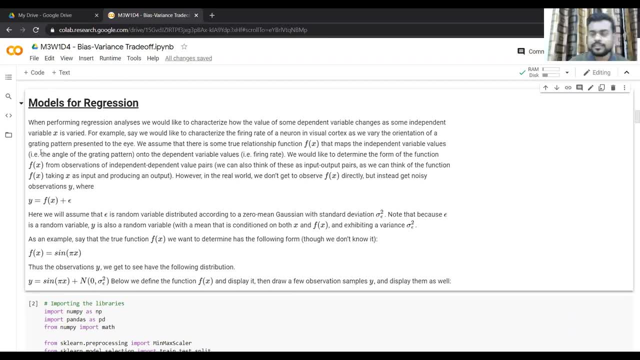 So in real world, Let's say, If you, if you're assuming that there is actually a such a function, fx, which maps your independent variable to your dependent variable, right? So that can be written as: y is equal to fx plus epsilon. So epsilon is some error which will evidently be there in our real world, right? 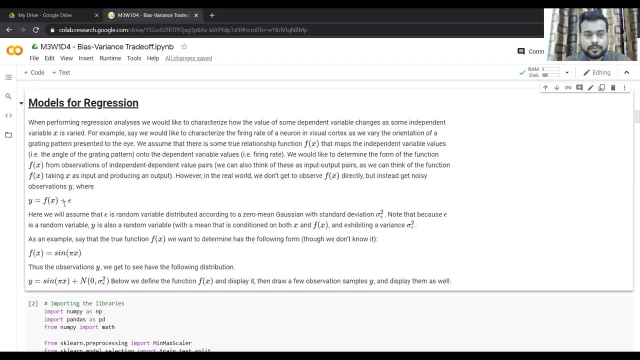 So our real world cannot have observations which are just like: y is equal to fx, right? So we'll have some error Which cannot be accounted for and that particular error cannot be removed Even when we are trying to model right. So this, this particular inherent error, will be there always. 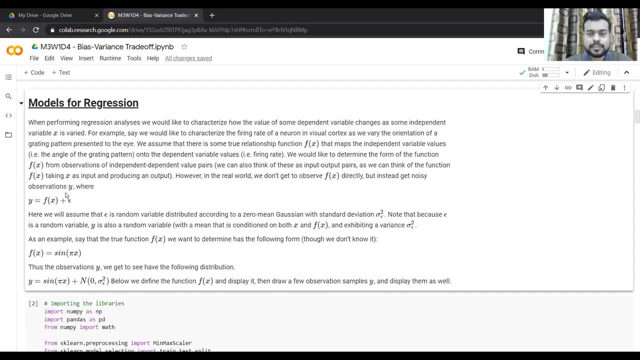 So let's say yeah, So these are our observations. why So? this we can call in real world problem scenarios. we can call this: y is noisy observation, right, Because there is some noise, Even though We were. There is a true relationship, function, fx. right. 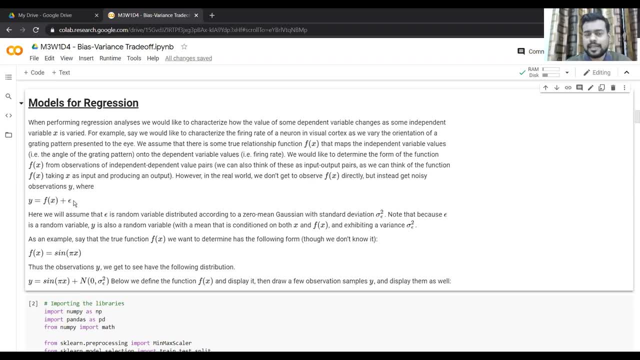 So y can be written as fx plus epsilon, where this error can be more or less. epsilon can be very small, but that will evidently be there. So in our case, for the experiments which we are going to run today, So we'll assume that this particular epsilon is a random variable which is distributed. 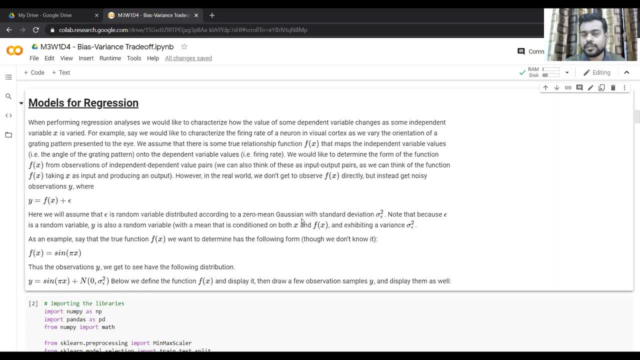 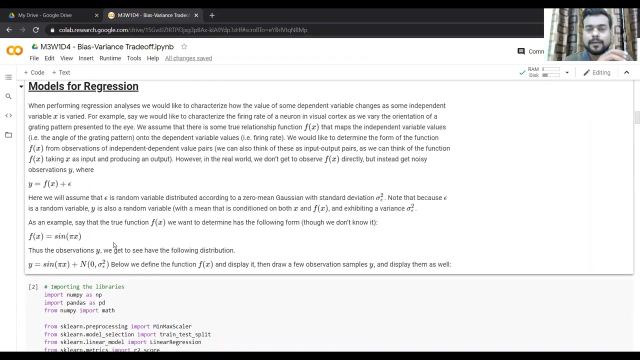 according to a zero mean normal distribution with standard deviation, Sigma E- Epsilon squared right. So we'll assume that epsilon is a random variable following the normal distribution with zero mean and standard deviation is some Sigma E- E squared right. So right now, what we want to do? we want to come, so we, using our train data set, we want. 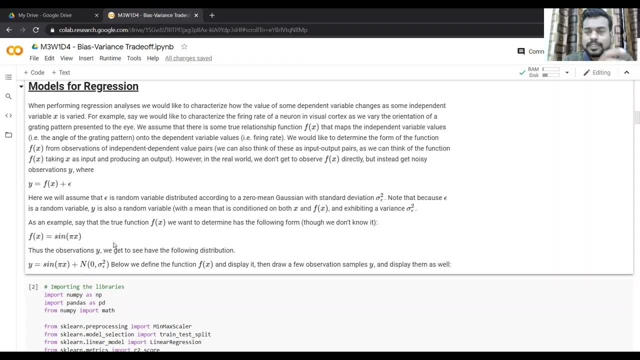 to come up with a function which will help us model this fx right. So this is our objective. We know we actually don't know what fx will be, But based on our training data set, we want to come up with some function, let's say gx, which. 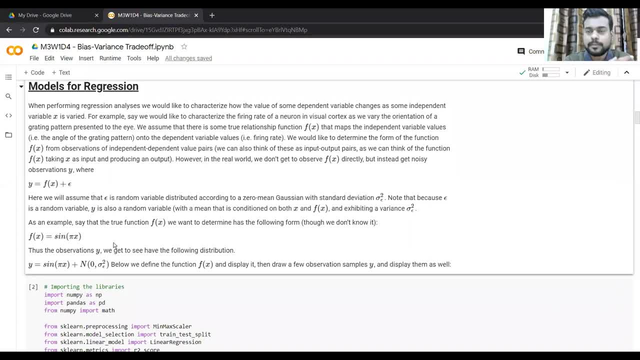 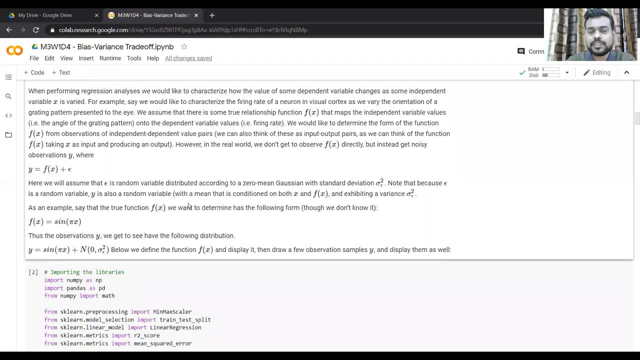 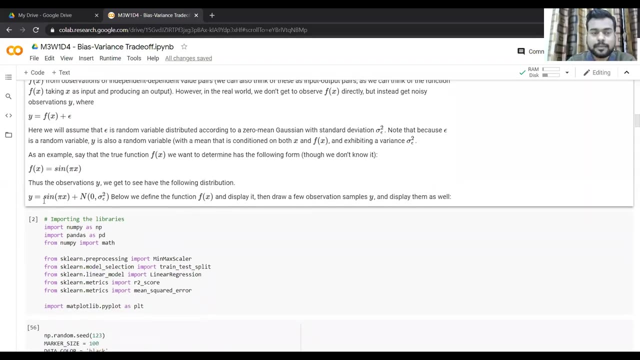 will estimate the fx in a much better, in a better way, right? So, for example, let's assume that this true function is some sine pi x. So this is, this is the true function. Okay, So then our observations, actual observations, can be: y is equal to sine pi x, plus this error. 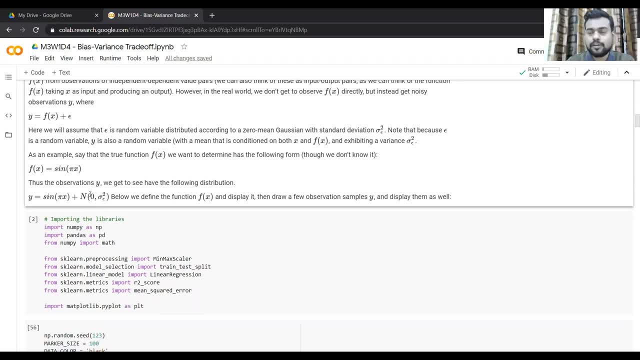 which can be defined with. define us, Okay, As the normally distribute with according to normal distribution, right? So so we'll see. so we'll assume that this sine pi x is actually some true relationship function for the experiments which we are going to run. 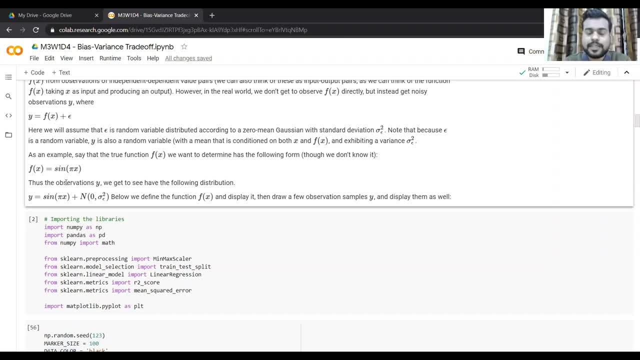 So don't think why we're just choosing sine pi, x, y, not other function. So we are. we want to actually do some experiments and we want to come up with functions which will help us. Help us come up with estimates of this fx right. 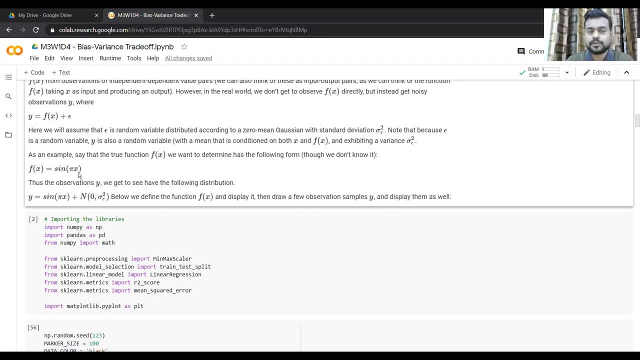 So this, this is the fx which we have right. so fx is equal to sine pi x with we are assuming that this function describes the true relationship between x and y value pair, right? We still don't know if sine pi x is the actual true function, but we'll assume this here. 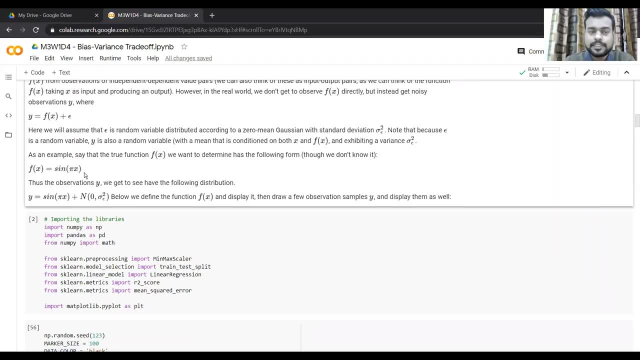 right and our objective is: given our train data set, We want to come up with a function fx. We want to come up with a function not fx, Some function gx Which will closely approximate this function f right, So we can create our observations for our experiment according to this particular equation. 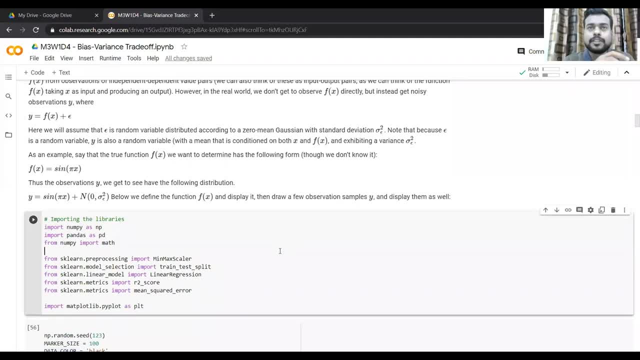 and then our objective would, we do come up with some estimates of fx, right? So these will be different functions. This will not be, let's say, trigonometric, some it could be less. a simple beta naught plus beta 1x, right. 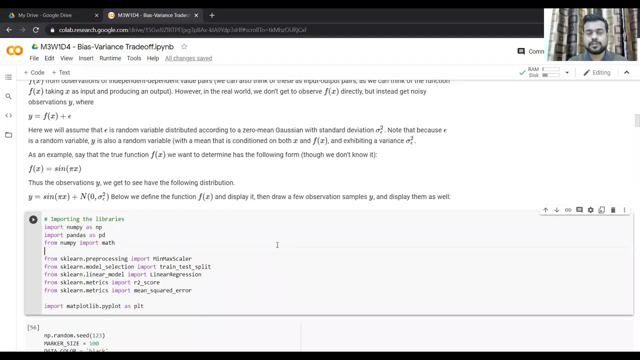 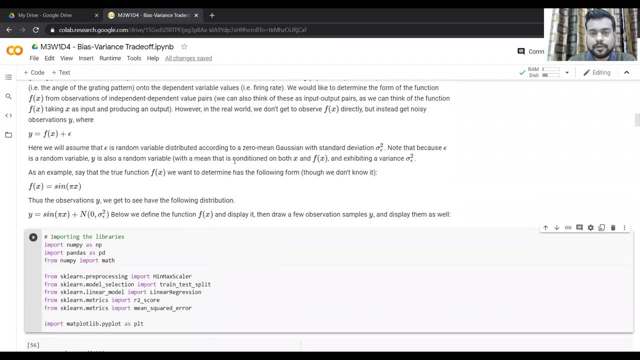 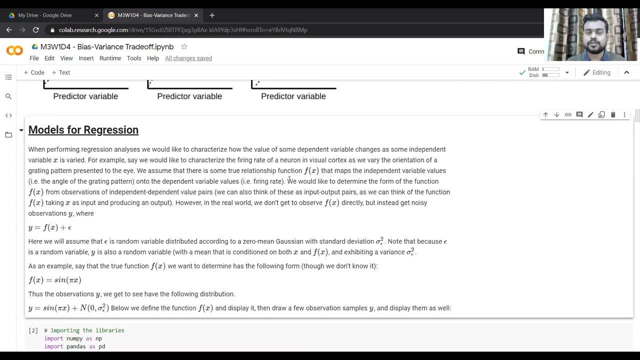 So that could be a very simple model which, using which we can, We can come up with some estimate of fx, right? So so, as I told you, we want to come up with a function g which will closely approximate this true relationship. function f- right. 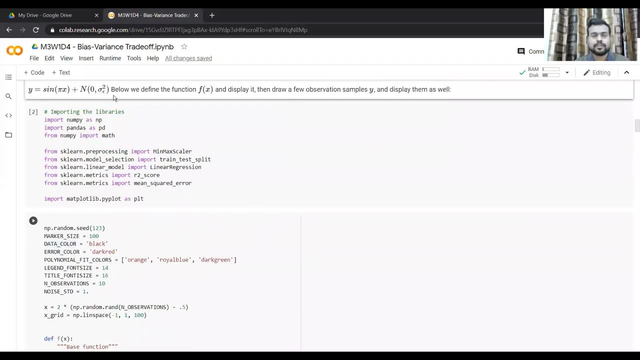 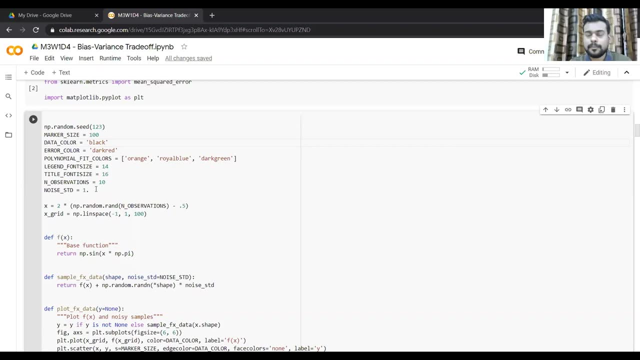 So let's do some experiment based on this. So I have written some codes here So you can. I'll focus on the important, Okay, Variables here. So so I'm I will be creating 10 observations. the standard deviation for the noise. 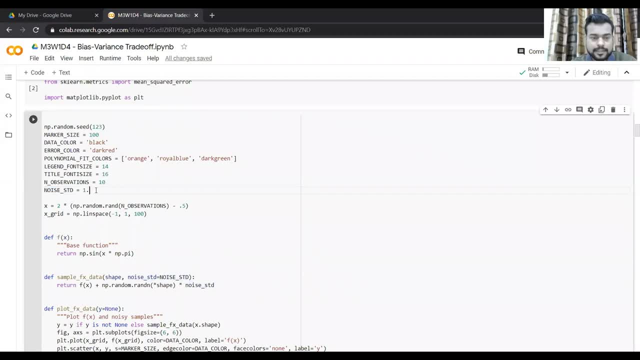 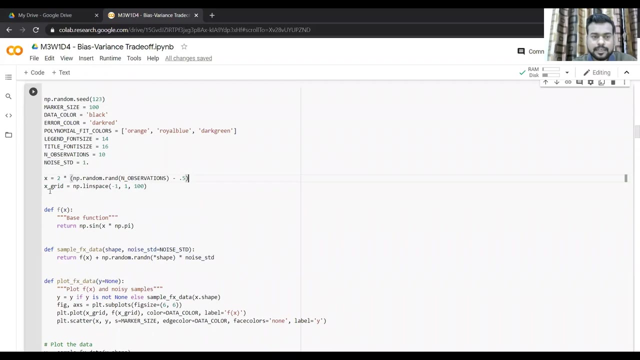 I'll be taking as one, Okay, and, and now, so I'm creating this variable, X, which will be which is defined by this particular function, right? So, in this way, we are creating X and then we are creating X grid, which will be sort. 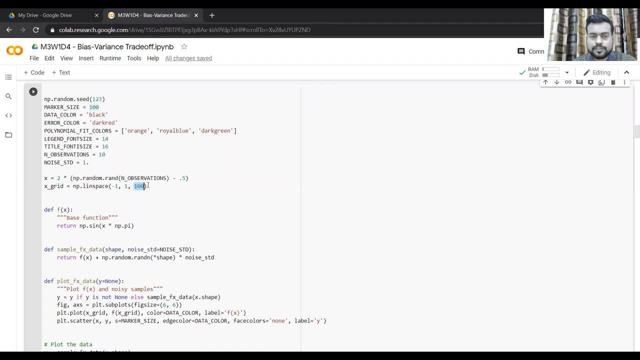 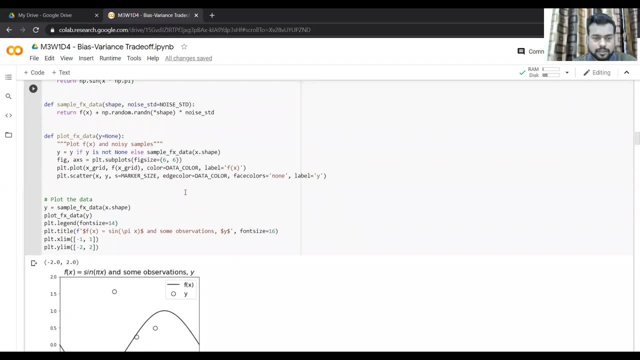 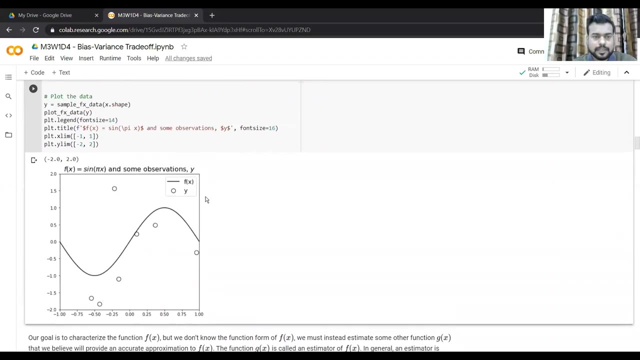 of hundred values Lying between Between minus one and one. So just keep this in mind, that. so we'll be creating X. so so one, two, three, four, five, six, seven, right? So we are creating some set of values for X, right? and then 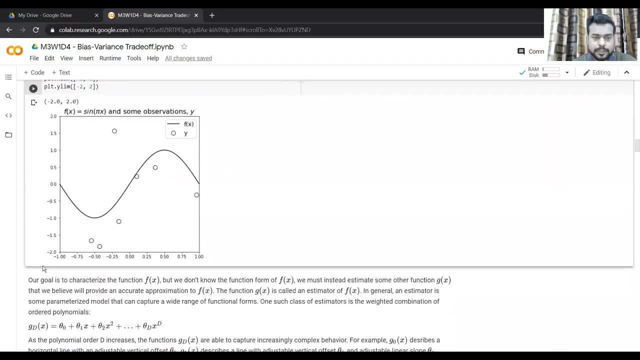 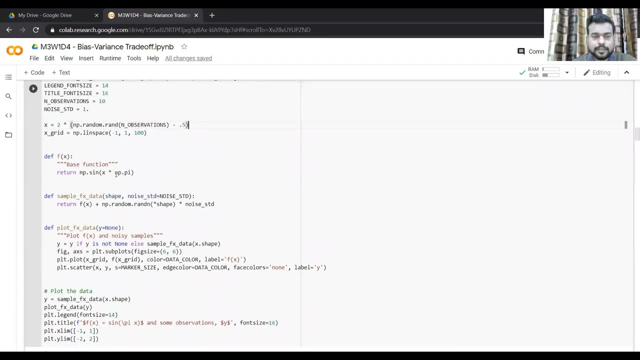 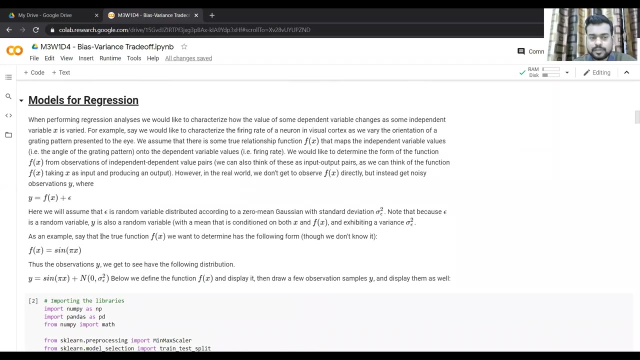 Right. so between minus one and one right. So we are creating these set of values. So, Okay, So I have written a function. This is the sine pi x. This is what we are assuming as the true function, right, So this is what we are assuming as this true function: sine pi x. 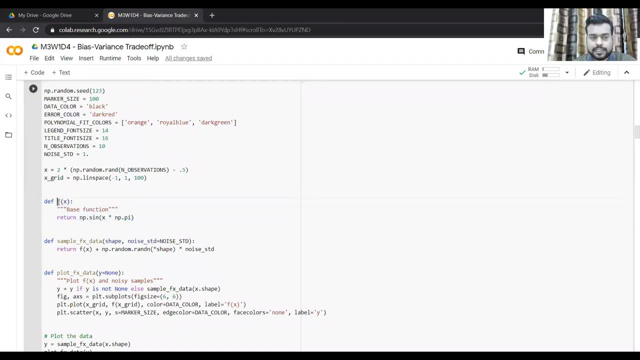 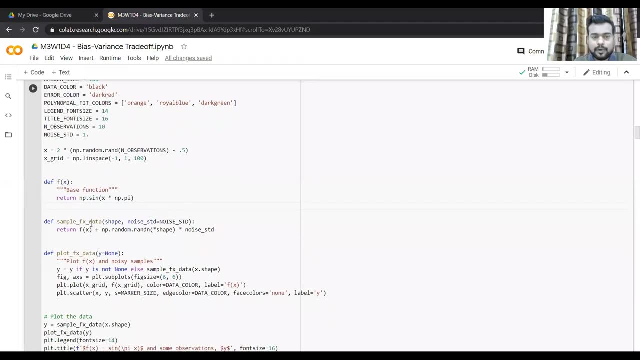 Okay, So this is the FX, So remember the function whenever you are seeing FX, that will correspond to this site by X, right? and then we want to generate a sample data, right? So what we want to do? so we want to return y. 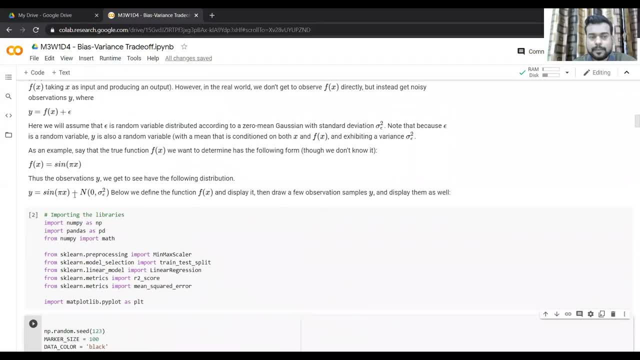 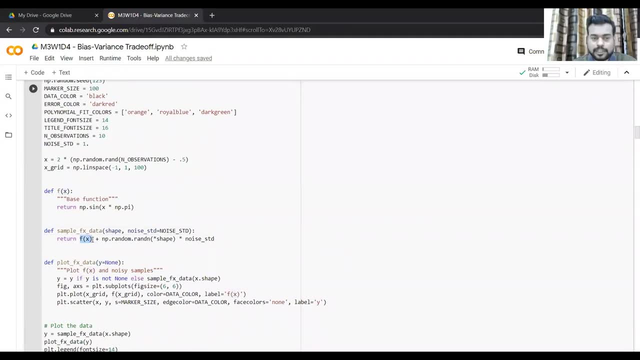 So how will we do that? will y be created? so y will be sine by x, plus some error which is normally distributed so in this way. so i'll call this function fx and then add some noise. okay, so i've already, uh, yeah, selected, uh, and my default value of noise, standard deviation of that noise is this particular value. 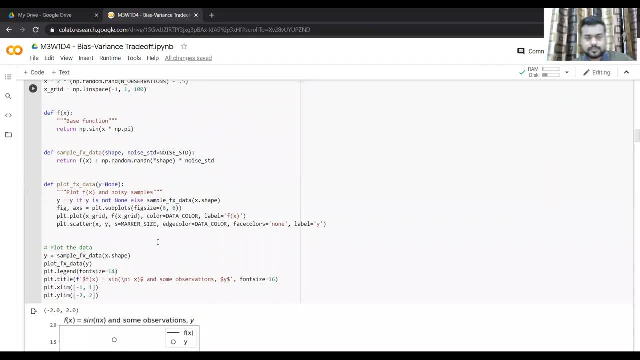 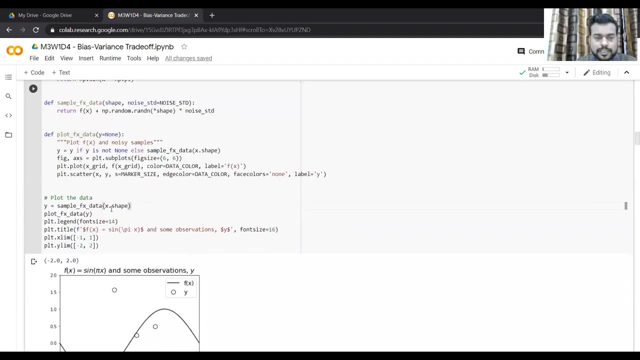 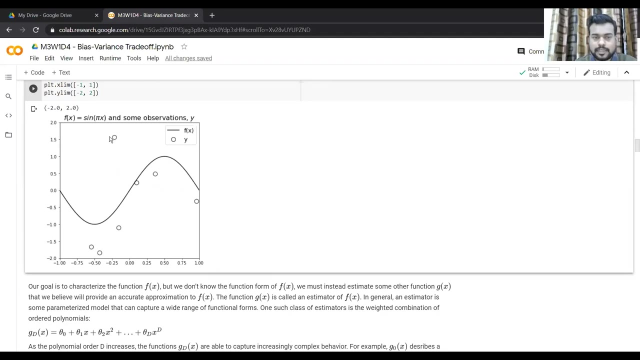 one, okay, so now, uh, i have created another function which is just to plot these observations. okay, so i'm just plotting these observations and so you can see. uh, so our actual y is are the dots here, and this is the fx, which is sine by x. right? so this is how sine by x looks like. so, for example, 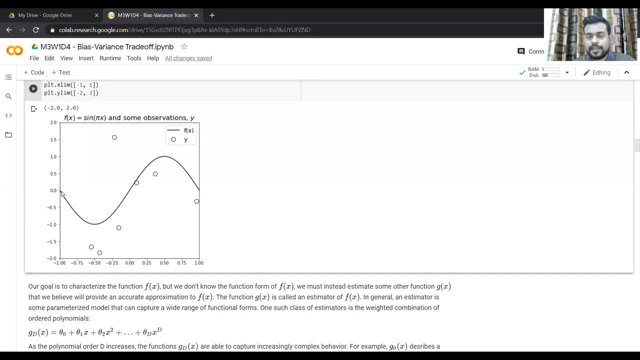 if x is uh zero. so what will be the value of sine zero? that will be zero. uh, what if uh x is one? right. so if x is one, then sine pi, sine pi is again zero. let's say: if x is half, so sine pi by two, right. so if x, x is half, sine pi by two will be one. and let's say: if x is 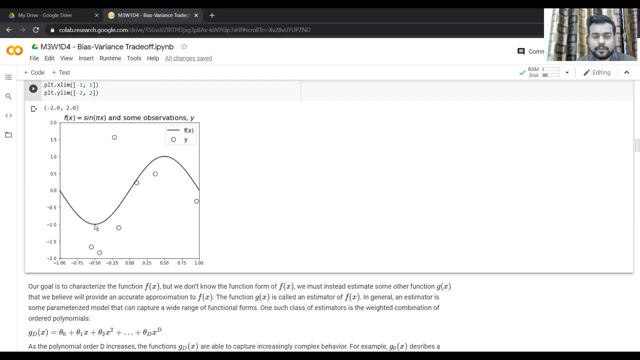 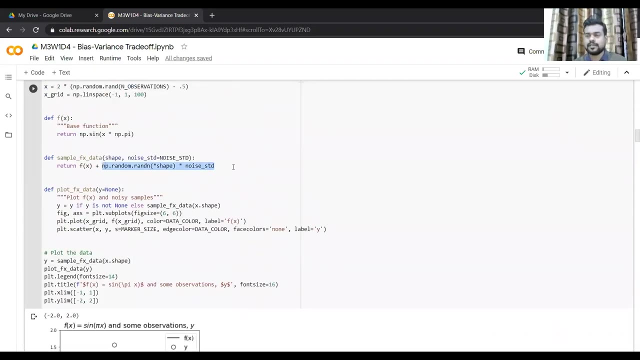 minus half. so sine uh, minus pi by two will be minus one. so in this way, this, this is what our true function, which we're imagining, and these are y. so why we are seeing deviations here? because i've added this noise term so that, uh, we're assuming that, uh, in real world there will be some. 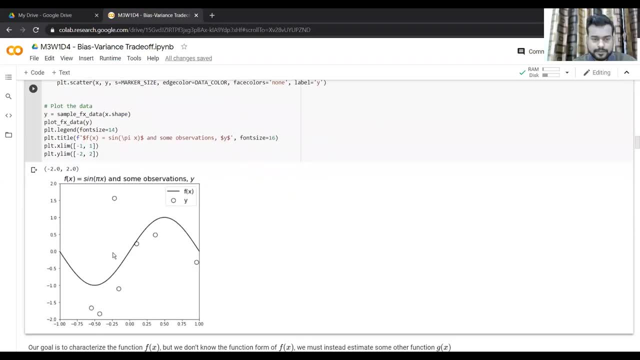 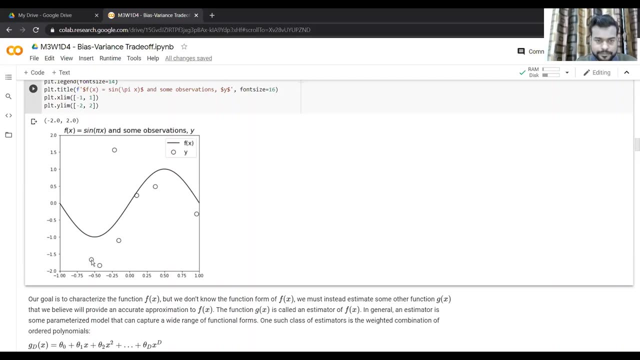 observations. so that's what we're trying to model here. okay, so these are our x and y value pairs, right? so this is uh, this is the y for this particular x, this is the y for this particular x, right? so in this way, i've created some set of uh observations, uh, some set of value pairs of x. 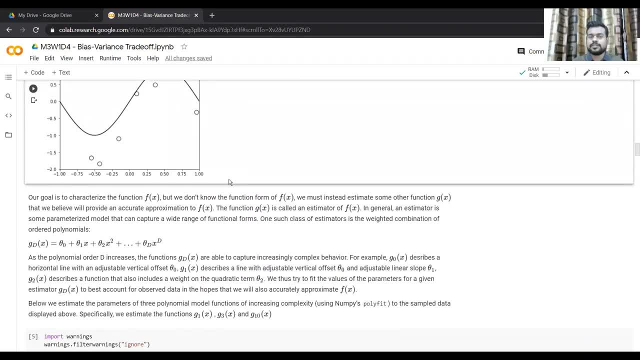 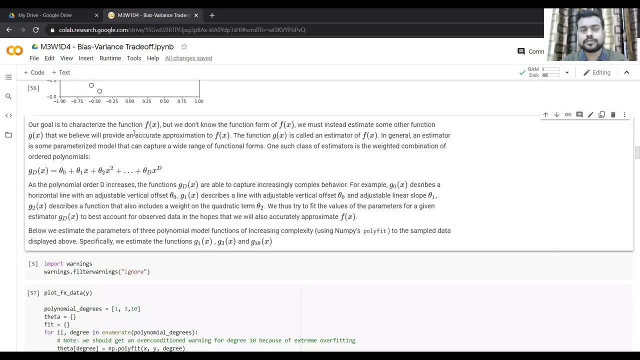 and y. okay, so this is uh. so we have just created a few observations here and now what we want to do next? so next, our goal is to characterize this function fx. right, so of course, we are given the sine pi, x, but in reality, uh, we'll never know what this function fx is. our objective view of 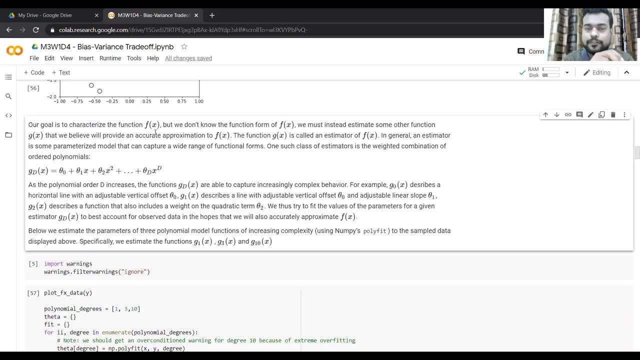 doing machine learning is essentially to come up with this function fx. uh, come up with an approximate uh estimate of this function, and we'll have to. so we'll assume that that is some accurate approximation to the actual function which describes the relationship between x and y. right? so i'll read: read this: uh, so our goal is to characterize this function fx, but we don't know. 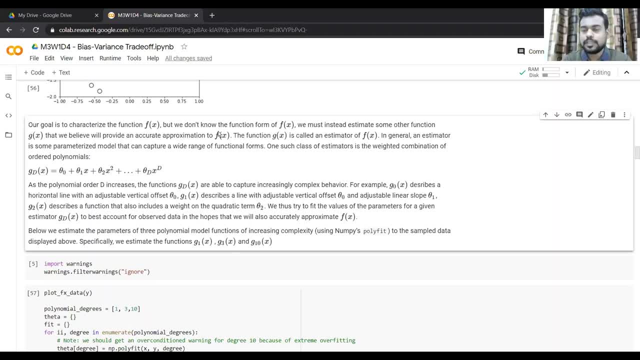 the function form of fx, right? we don't know that yet, right? so let's say, if you're given a data set, uh, train data set, and so we don't know this, what, uh, what is the relationship between x and y? and the whole objective of doing machine learning is to come up with that. 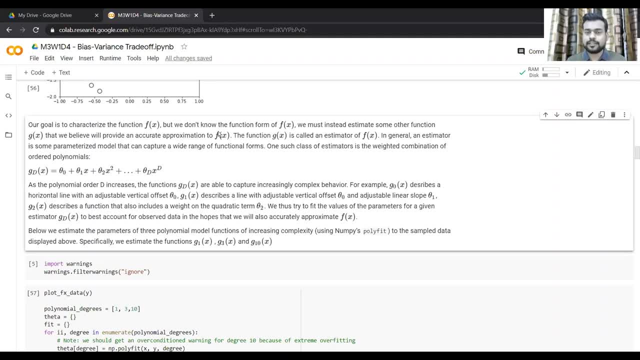 relationship between x and y. right, so we want to come up with some approximation of f. so we, uh, yeah, so we need to take some caution here, as in i'll be introducing some terms which you might be familiar with, but you just need to pay some attention. so of course, we don't know the function form of fx, but we must instead. 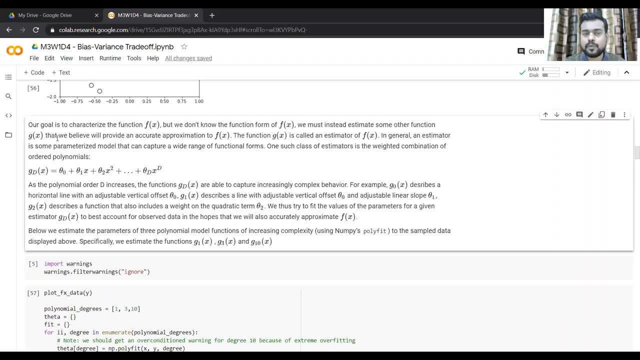 estimate some other function, gx, that we believe will provide an accurate approximation to fx right. so this is what we want to do. so there is some true relationship, fx, uh, which we don't actually know what that is, but given our data, we want to come up with this. 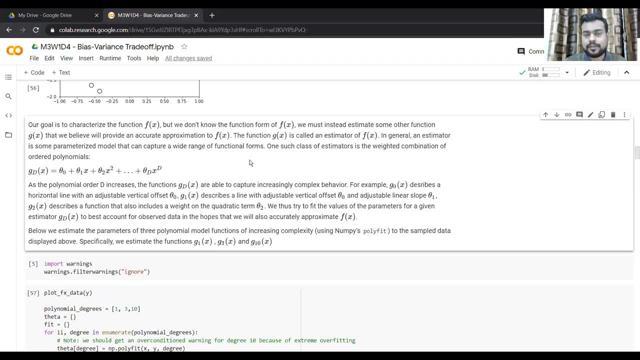 estimate function gx. uh, that will also call as estimator of fx, and we believe that will provide an accurate approximation of fx, right? so, in general, an estimator. so in this case, for example, gx is some parameterized model that can capture a wide range of functional forms, right? so don't? 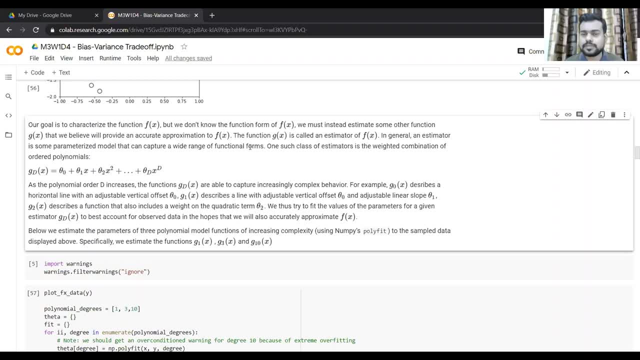 worry. what are functional forms? just, uh, just a little bit of information about the function form of fx. assume that these are some sort of functions. so one such class of estimators is the weighted combination of ordered polynomials, right? so, uh, you've already learned about one such estimator. 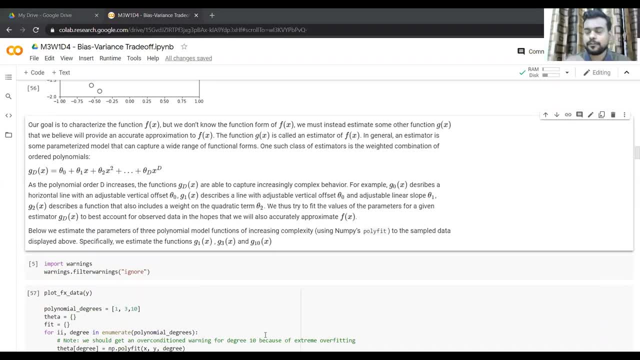 which is your basic linear regression. so let's say, if we had a single variable, so that function, let's say, i'll say that that gx was beta naught plus beta 1x, right? so this is, this is the function which we have learned from the last two classes. so let's say that we have a function which is: 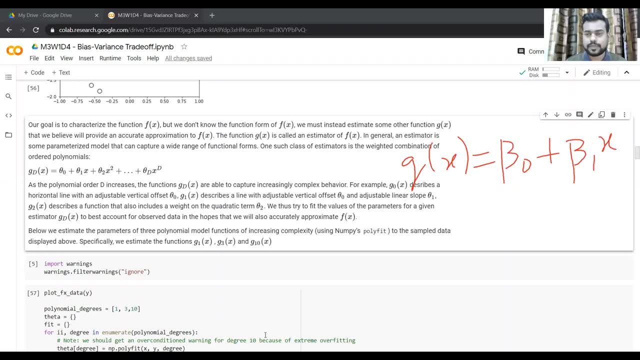 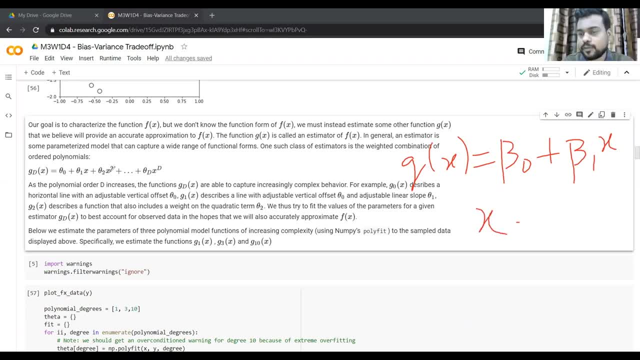 this one variable x, and i'm corresponding y. right, so i come. i can come up with, uh, an another estimator, uh, the gdx, which can be written as theta naught, uh plus theta 1x plus theta naught to x squared, plus something like this: theta d, x to the power d. so this d defines the degree of. 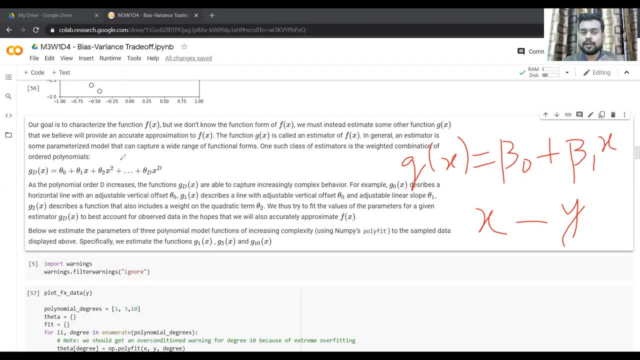 this polynomial. so i think you might be aware that this is how a polynomial is written. algebraic polynomial looks like okay and we're seeing. so this is this could be one class of estimators, right? so depending upon what is the value of d we want to take, so we can have different set of. 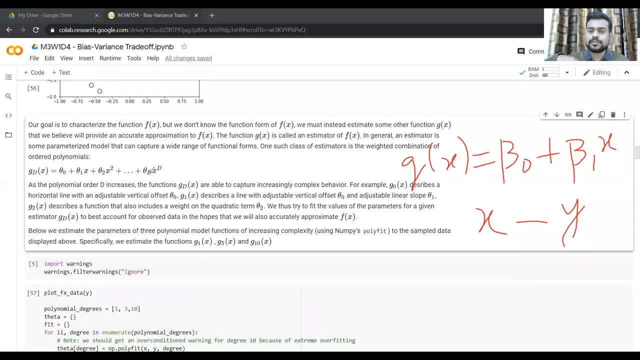 estimators, and these all estimators will come under one class, which will call us polynomial regressors of polynomial models. okay, so, as the polynomial order d increases the functions gdx, uh, yeah, so this just denotes the degree of your polynomial and able to capture increasingly complex behavior. we'll see how that happens. 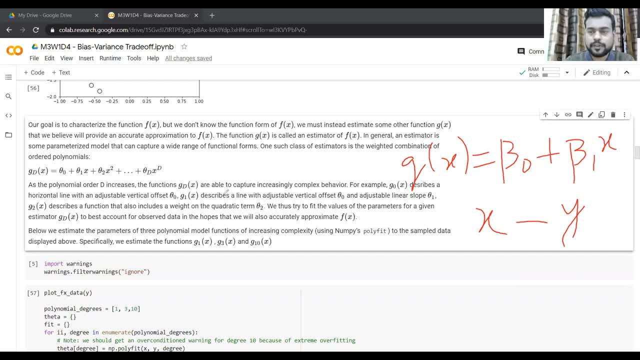 for example, g naught x. so based on this function. so this is how our g naught x looks like. i'll, in fact, clear the whole drawing. so how, how we can write g naught x based on our generalized polynomial function. so g naught x. 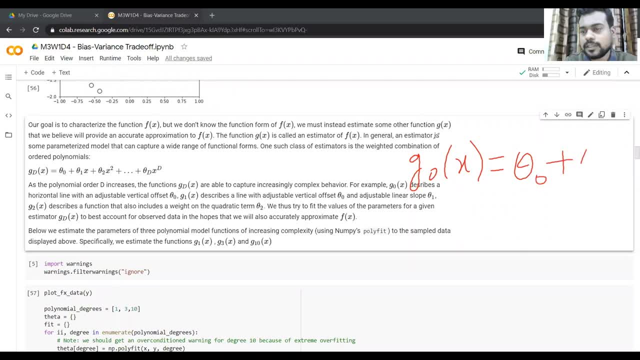 can be written as theta naught plus theta 1 x, right, what will be g1 x. so g1 x will be theta naught plus theta 1 x plus theta 2 x, squared right. so, sorry, one second. i yeah, so g naught x. uh, sorry, i made a mistake there. so g naught x, so put d equal. 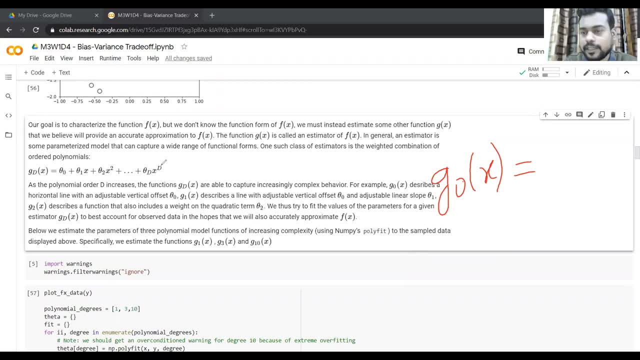 to zero, right, so x to the power zero. so we'll just have theta naught here, right, right, so we'll have theta naught, and then we'll have g1, x will be so theta naught plus theta 1 x. so as in, this is a first order polynomial, this is a zeroth order polynomial, right, uh, right, so we can have. 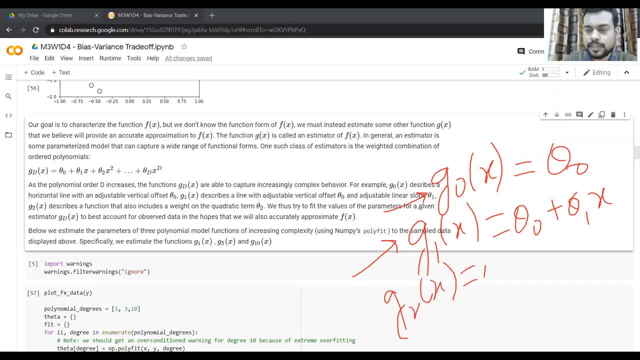 g2 x, so that will be a quadratic polynomial right. so theta naught plus theta 1 x plus theta 2 x squared, so one important uh terminology which you should uh be aware of. so let's say, when we're talking about the multiple linear regression, 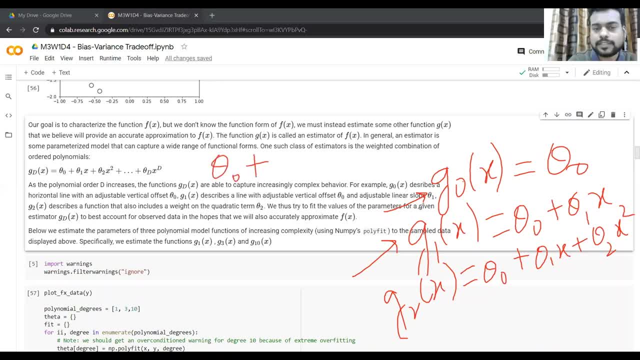 what was the equation which we had? so that was that we had theta. let's say, if i had two variables, so i i was writing that as theta 1, x1 plus theta 2 x2, right? so this is how, let's say, we were writing our multiple linear regression, so in this case, bivariate linear regression. 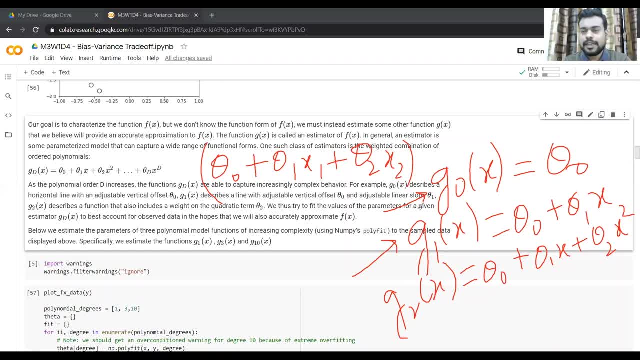 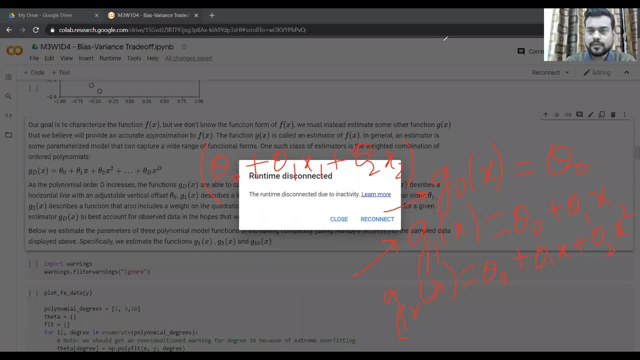 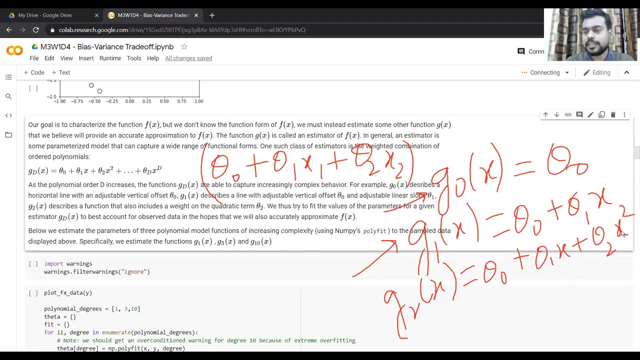 but here also you can find some similarity. so i told you that we have just single variable x, but i am writing one second. yeah, so i am writing theta naught plus theta 1 x plus theta 2 x, squared. so what you can assume that, uh, this x. 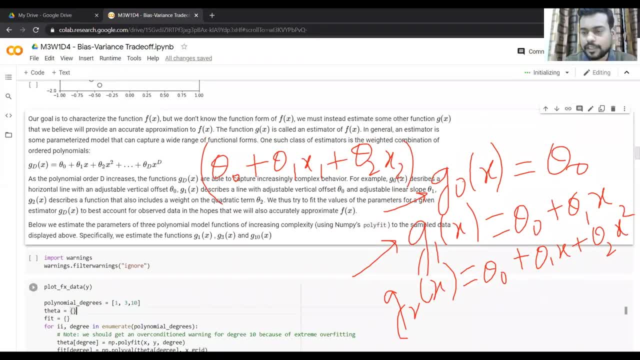 yeah, so you can assume that this x corresponds to x1. this x squared can correspond to x2, right? so let's say you are given a variable, you create another variable which is just the squared values of that variable. so you are given a variable, you create another variable. 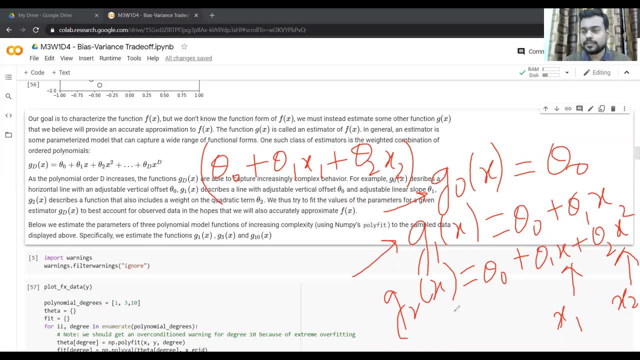 values of that variable. So that could be another variable, right? in this way You can see that this is also a function, what we can call as linear regression function, right? So this is as in when we are saying linear, these are linear in your parameters, Theta. 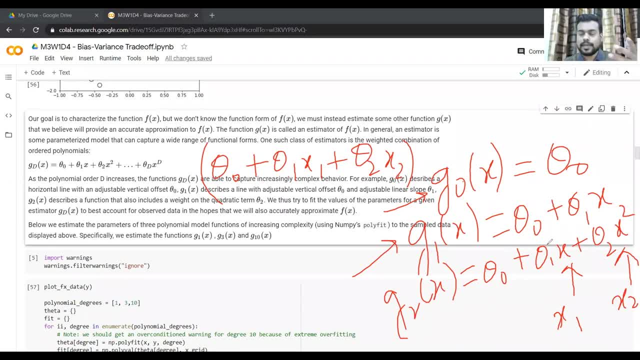 and Theta's right, So we don't have Theta 1 squared, Theta 2 squared, something like that. Okay, so as long as we have an equation which is linear in these Theta's, even though we have X, X squared, X cube, something like that, So we can say that this polynomial regression 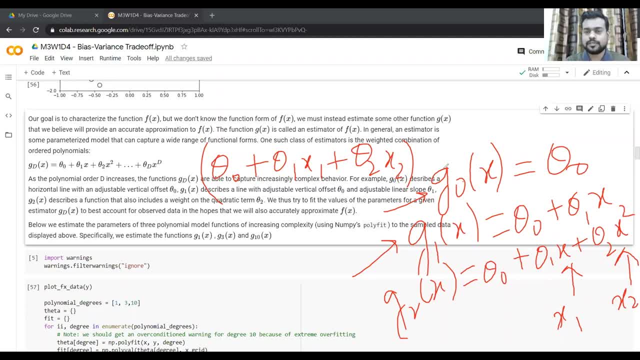 also is also a linear model. Okay, so that is just a terminology I just wanted you to be just familiar with. so, even though you will see, you say that we can have something like Theta 3 X, 1 X, 2.. Right, something like that as well. But yeah, we don't need to bother about that for now. 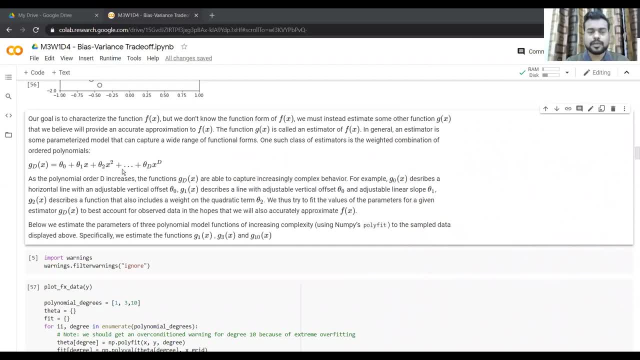 Okay, So. so this is how, this is what our, let's say, one class of estimators will look like, which is D degree polynomial. So so we'll, today we'll be looking, will be having estimators which are, let's say, one for one degree polynomial, three degree polynomial, 10 degree polynomial. 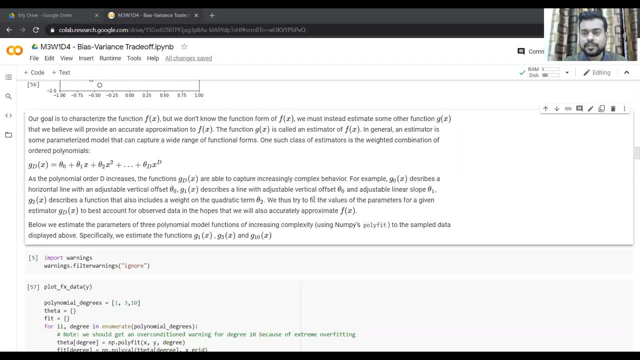 so we'll be experimenting with these today. So these are these. these could be our estimators of FX, right? So let's say, I can call G1 X, which is Theta naught plus Theta 1 X. So this is an estimator of FX, right? So this G1 X can be an estimator of FX. we can have G3 X. 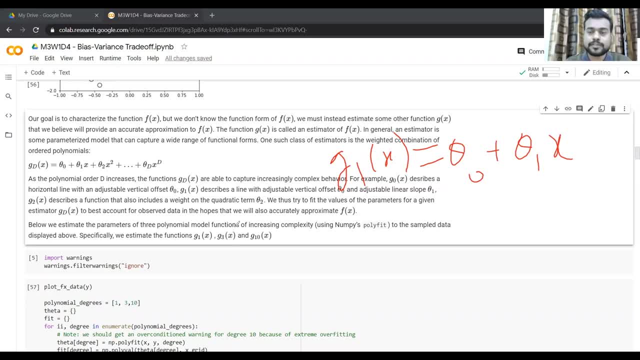 which is Theta naught plus Theta 1 X plus Theta 2 X squared, plus Theta 3 X square plus Theta 3 X cube, right, So that could be another estimator of FX. we can have more complex polynomial, as in, more higher degree polynomial, as in: we can have G 10 X, right, So we can have G1. 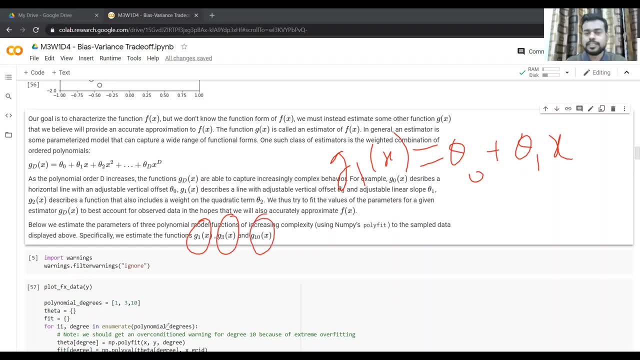 X. we can have G 3 X. we can have G 10 X. So these are our different estimators of X, So what we can call these as? so we can call these as estimators of FX, right? So these are the functions. 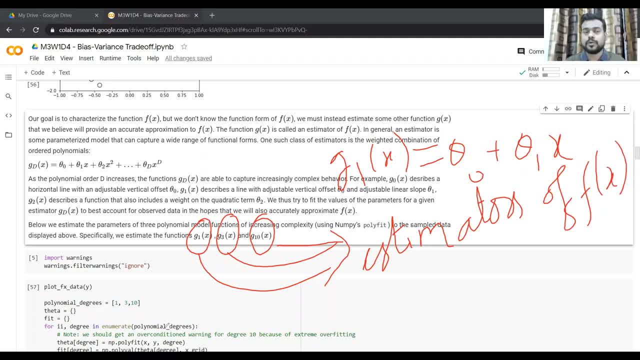 Using which we can estimate our true function, FX, which we don't know right, But of course in this experiment we have assumed that FX to be sine, pi, X, right. So these functions will be called estimators of FX and the objective of any doing machine learning, especially supervised. 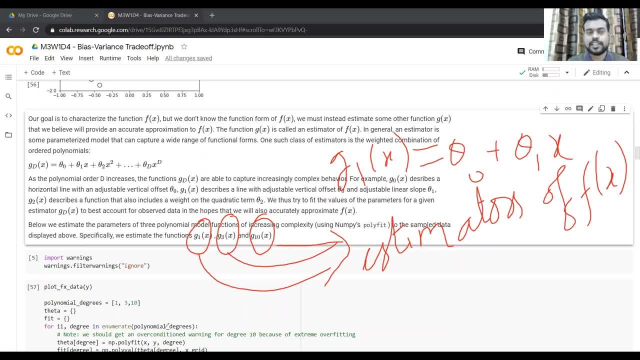 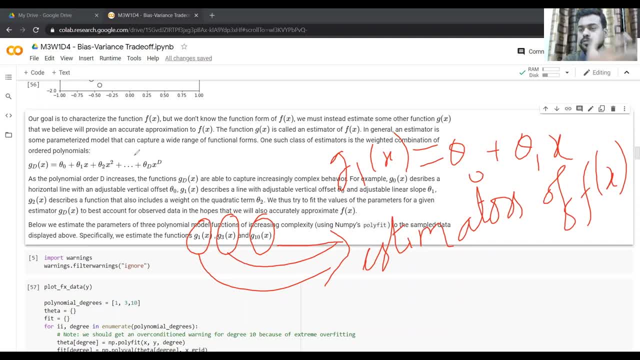 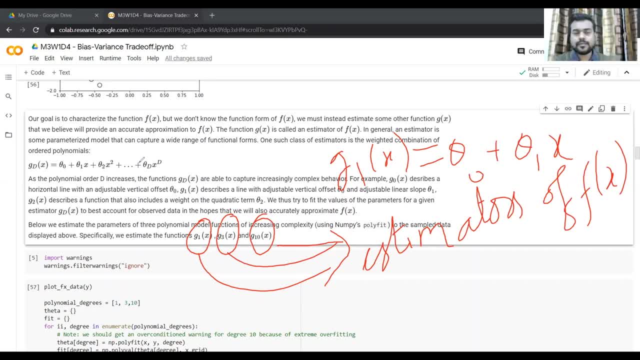 in the parameters Theta here, Right, So I hope you are. you now know what is and what refers to an estimator. So this is what we get, what we want to come up with, which will closely approximate FX based on our given data set. So is this concept of estimator clear to you people? 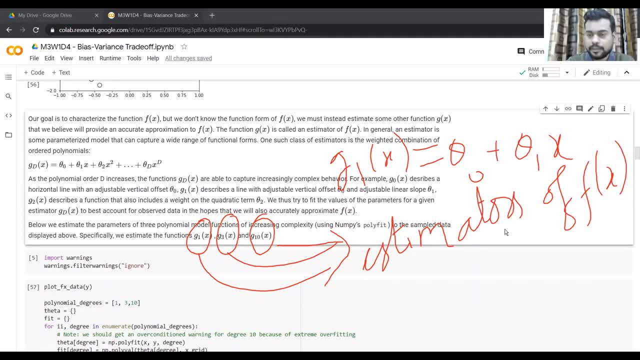 Can you let me know so that I can move forward and we can actually do an experiment with this? Yeah, so this concept of estimator should be- should now be familiar to you. All, right? So yeah, Okay, that's great. So yeah, everyone is with me at this moment at least. okay. 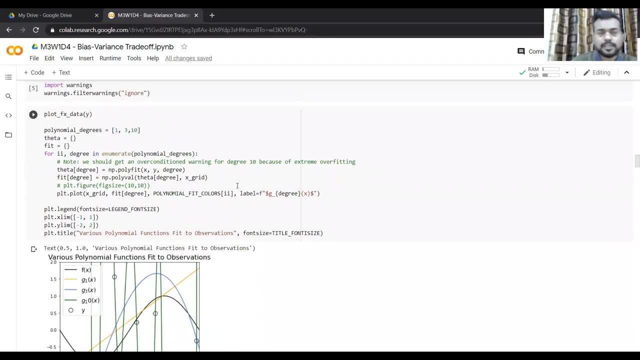 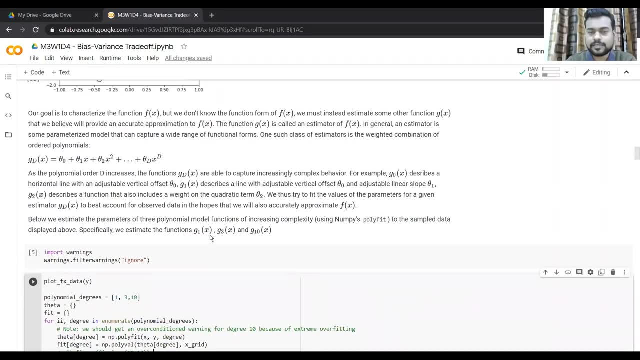 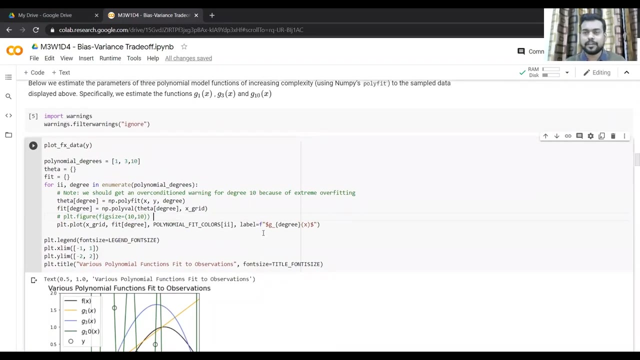 So okay, so let's do some experiment. Okay, So what we? so we are going to experiment with three estimators, as I told you. So this could, this will be g1 x, g3 x and g10 x, right, So one will be one degree polynomial. that is your basic equation: beta theta or not plus. 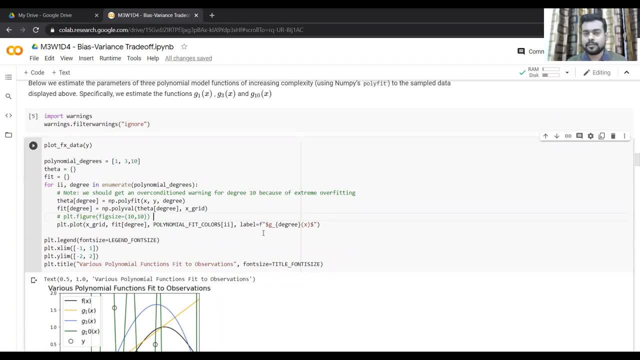 theta 1 x, then g3 x. this will be a relatively complex as in it will have a cubic term at least, And then we'll have a g10 x, right? so it will at least have a term which will be x to the power 10.. 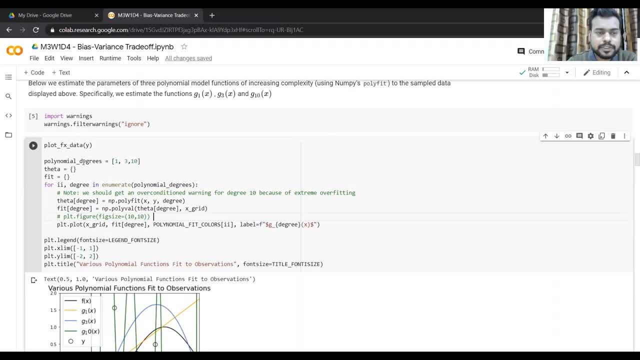 Okay, so so I'm creating a list, which is what I'm calling as polynomial degrees, and this list is taking values 1, 3, 10, right, and then I am creating a dictionary, theta, and then something called fit. now what I'm doing. so there is a function in numpy. you can use your. 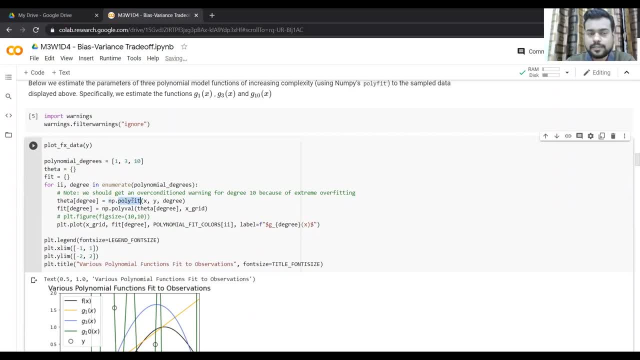 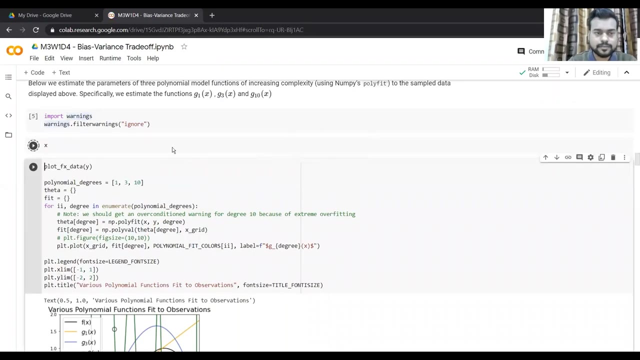 normal linear regression as well. but in numpy there is a function which is called polyfit which will do a polynomial fit essentially on your data x and your on your y right. So we can at this moment we can see what our x looks like, right? 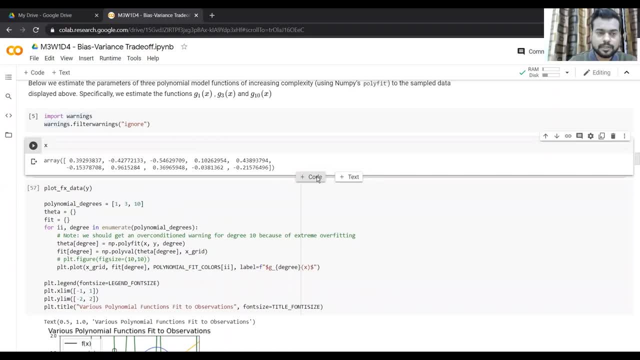 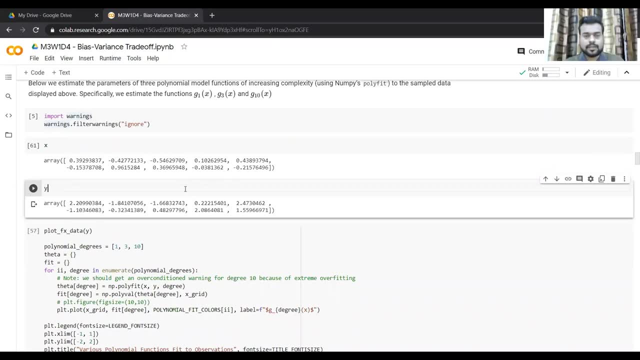 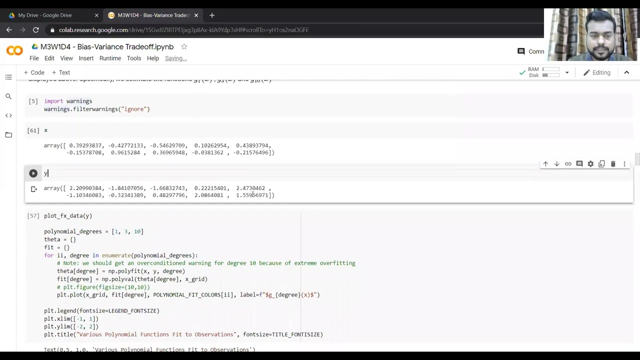 So this is how our x looks like and this is how our y looks like, or, in fact, Yeah, So for each value of x, we have some value of y, right? So this is our x and y look like, and let's say so. so I'm using an enumerate function. 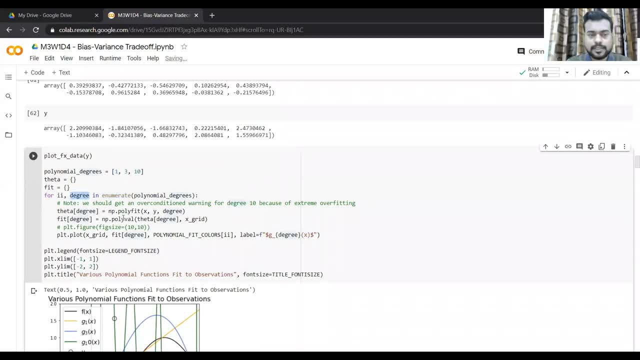 So of course II will be the index and degree will be the value right. So so I'm creating: so theta is a dictionary, so theta degree, So theta 1. so if for the key 1 we are doing a polynomial fit which will return the value, 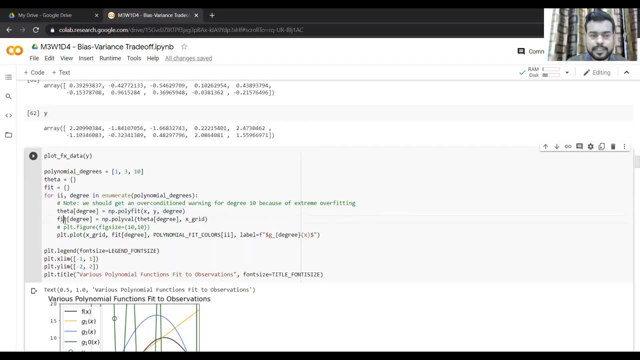 of the parameters, right, and then I have this fit degree. So now what I want to do. so I will be fitting this model on this data, x and y. okay, So on x and y. so these are what: 10 pairs of x and y, right? 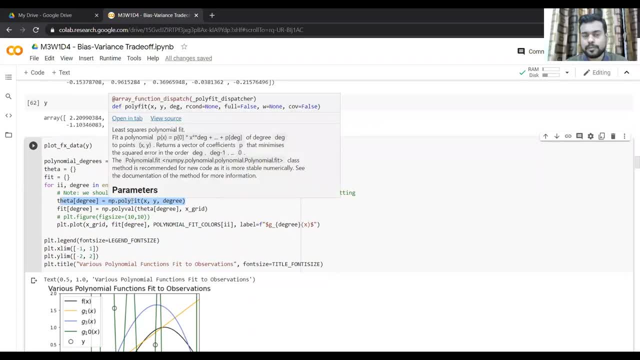 So I will be fitting this, fitting our polynomial model for each degree which you have in our list. So we'll be fitting Firstly 1 degree polynomial Right on this in data which is x and y right, and then we also need to provide the degree. 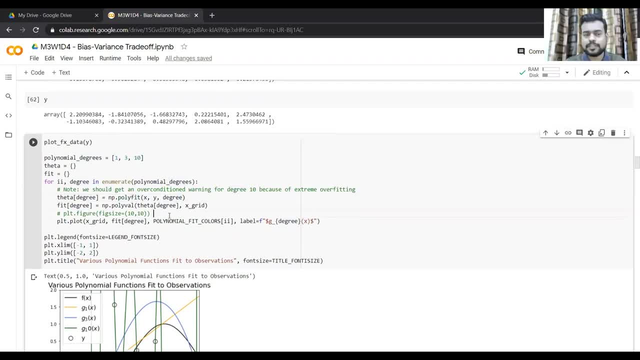 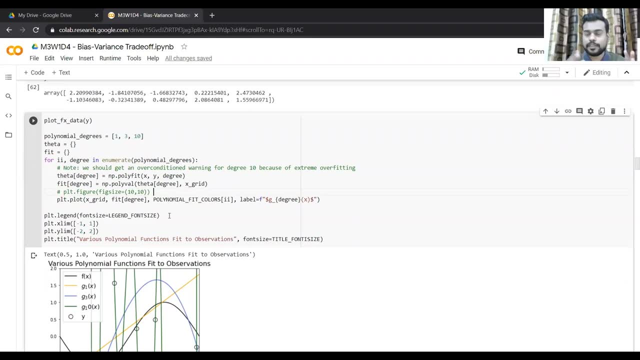 because this is a function, polyfit. Okay, So let's say, if this, these functions are new to you, do not worry about them as in they don't have a lot of concept involved in that, but you just need to understand what these functions do, right? 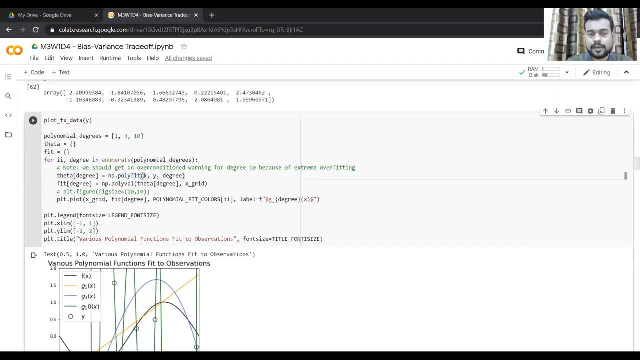 So this NP dot polyfit, it fits this, provided degree polynomial on this data, x and y right, and then now there is another function, polyval, what it will do. So, once we have fit, fit this polynomial, so as in for, let's say, for this 1 degree polynomial. 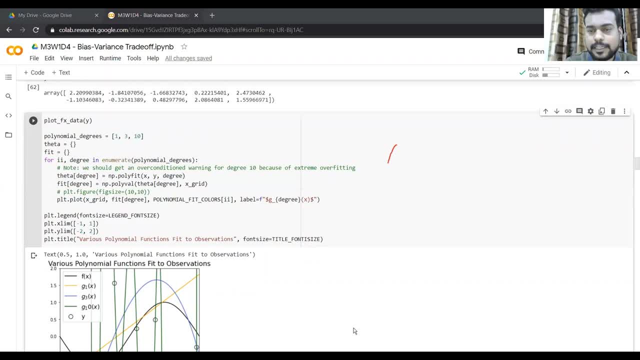 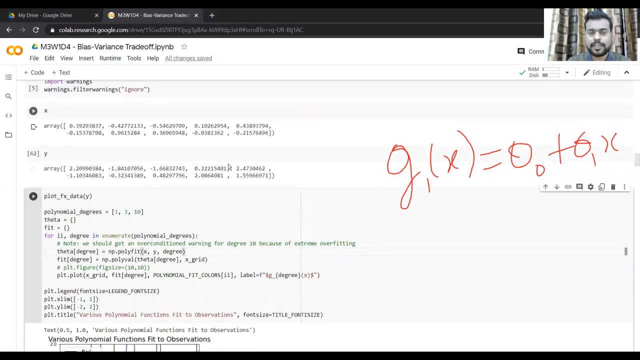 will have, let's say so. I'll just write: g 1 x will be theta naught plus theta 1 x, right? So for these 10 ones, So for these 10 pairs, We are fitting up 1 degree, We are fitting. 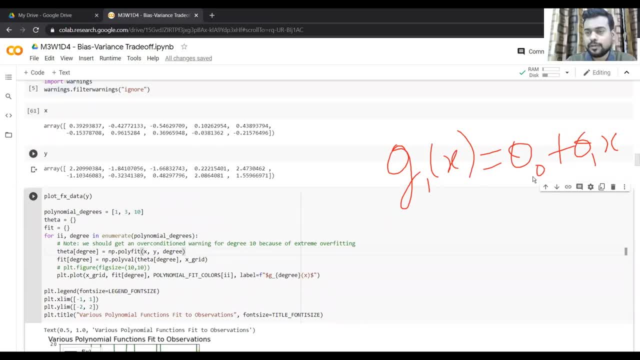 We are fitting this function, Okay and then? so for these, from these 10 x and y appears, will get some values of theta naught and theta 1, and that could be some value, right? So yeah, right now let's say this. this comes out to be something like, let's say, 0.0.. 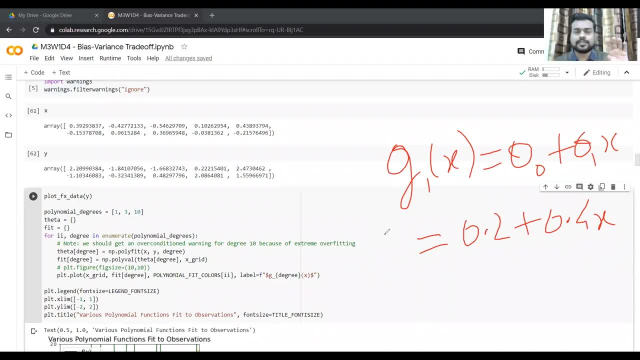 So this is our function. Let's say which we have gotten by looking at these 10 pairs of numbers, right? so 10 observations of x and x and y pairs, right? So let's say we can get these values: theta and theta 1. essentially we're getting these. 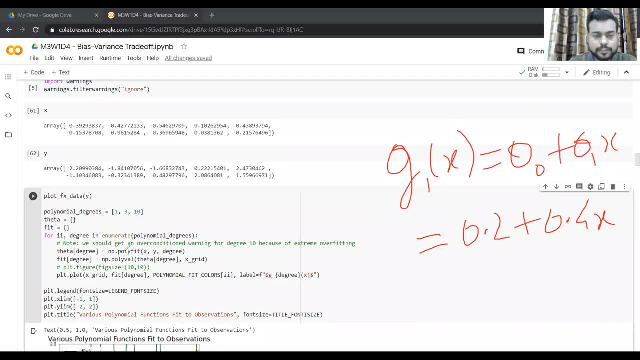 values 0.04 from this particular NP dot polyfit. right now, once we have the this particular function right, So this not necessary. It will be this way. Of course we'll have to print them and see what value it is having, but what we can do. 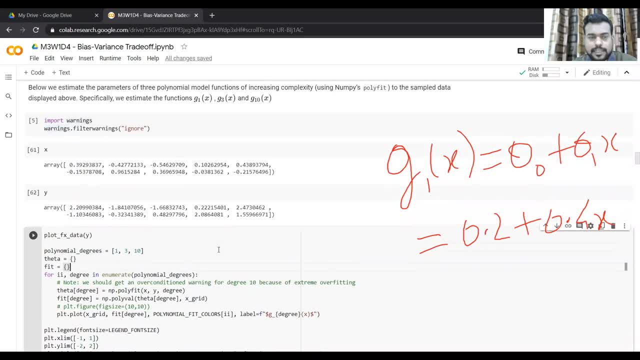 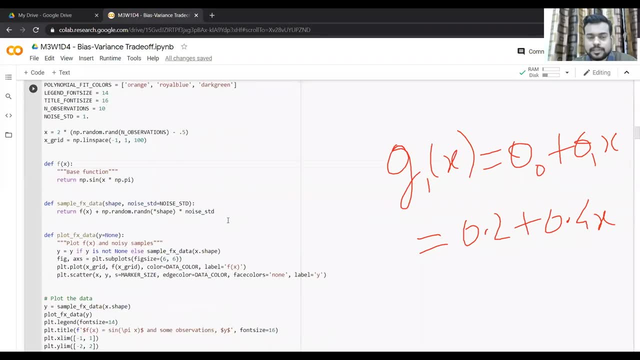 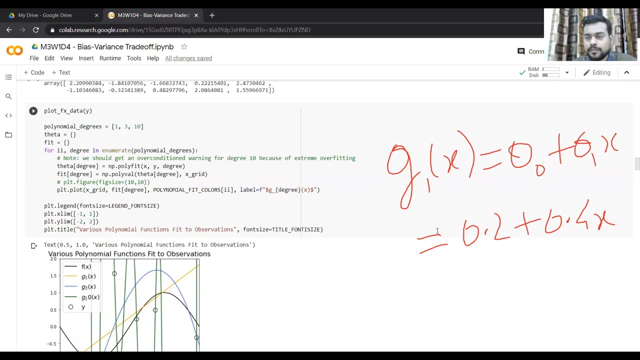 So we have this x-grade, which you remember from earlier what x-grade had right. So in x-grade I had around 100 observations between minus 1 and 1 right. So this is what our x-grade has right. So now, using this function, I will try to. yeah, so I'll try. I'll put all these values. 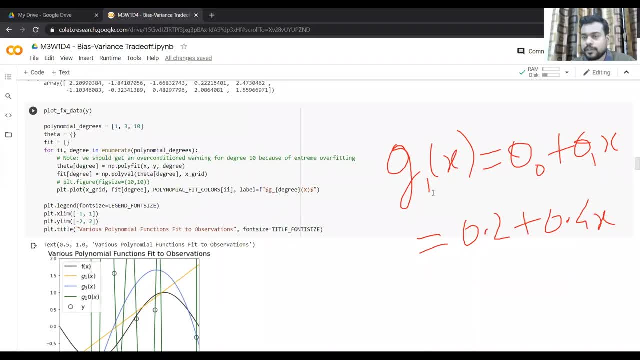 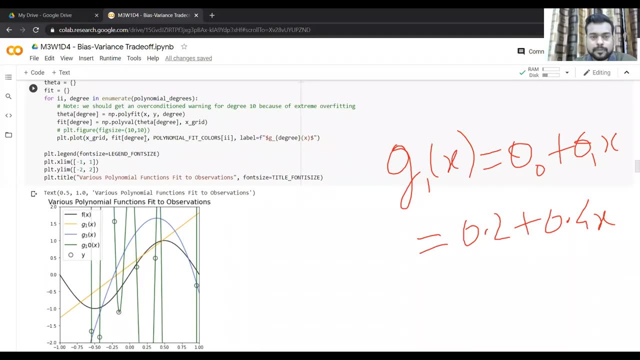 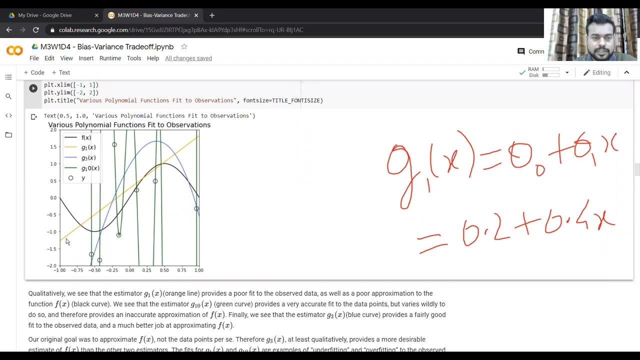 of x and see what will. what is the corresponding value of g1? okay, So, and that we can actually plot right. So this fit degree will give us that particular value and x-grade is the x, right? So for this g1, x, which is the orange line here. 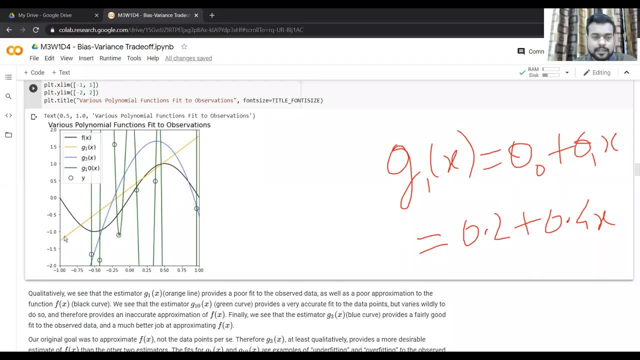 So for all these values. so we are getting this particular straight line right. So we have already come up with this function. Now We have these hundred values between minus 1 and 1 and so right. so, and seeing what is the corresponding value of g1 there, and then I'm just plotting that, all those 100 x values. 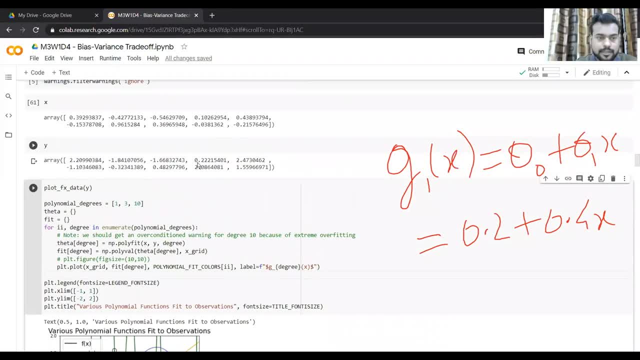 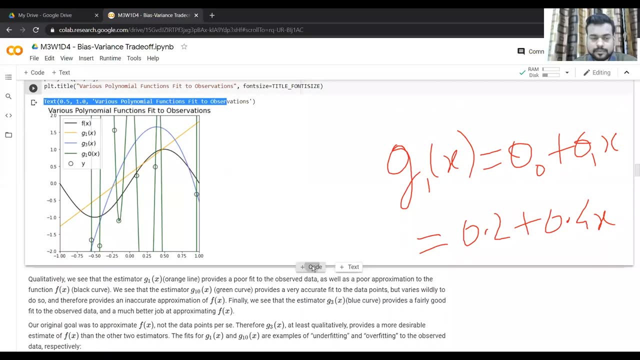 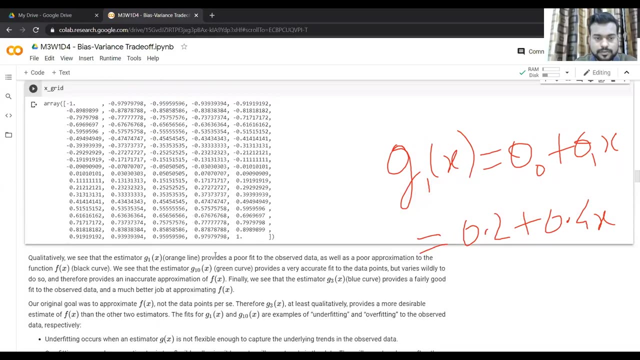 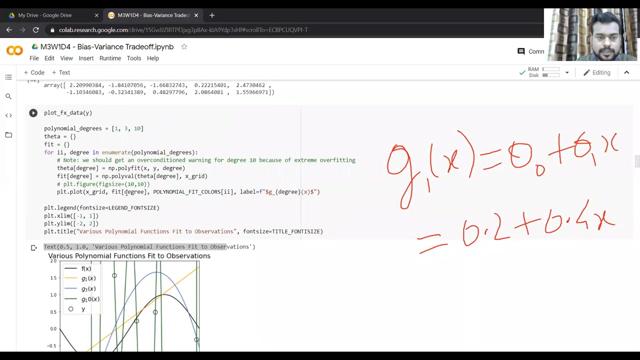 of x and y, right, so I can actually run this one, right? so so you can see what your x-grade looks like, Right? so these are some values between 1 and 1 and then right, so we can see what fit looks like, Sorry. 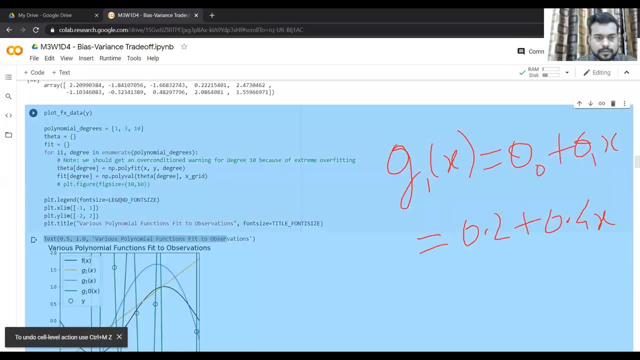 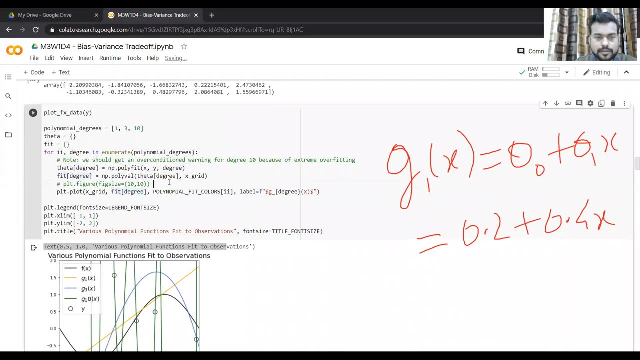 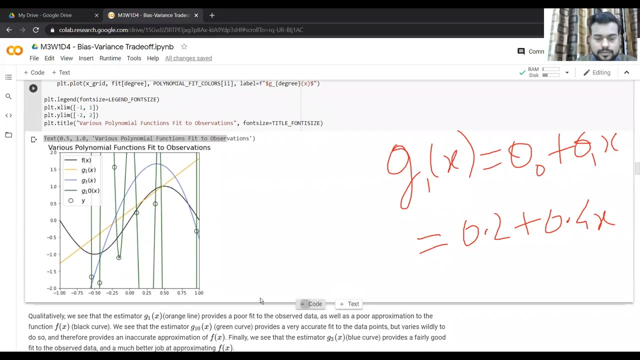 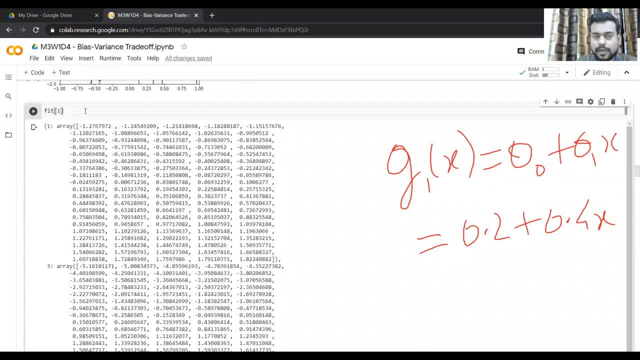 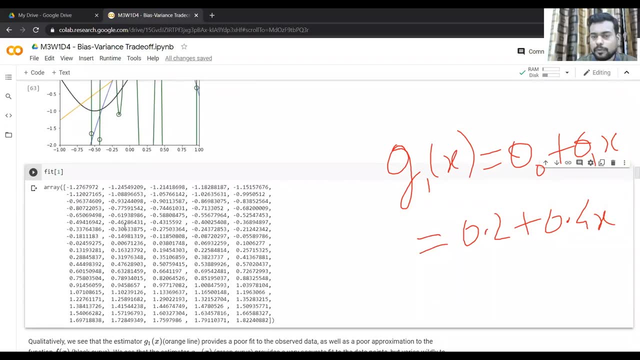 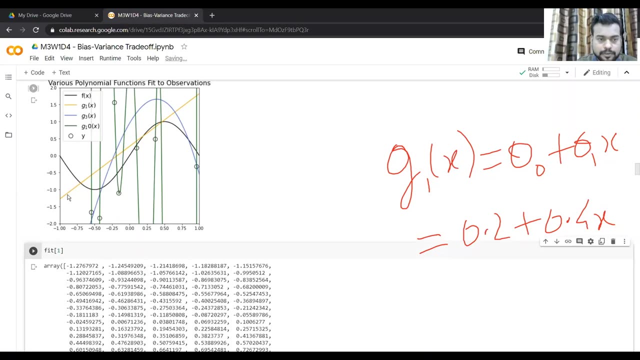 Okay, so so for one degree polynomial fit, one is for one degree polynomial, right? So it gives you corresponding values of y, so all these values of y which we are seeing here, right? So this is minus 1 point 26792, so it will be somewhere like this, and then we have this: 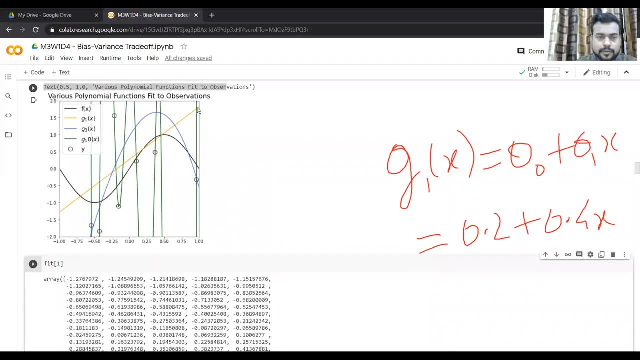 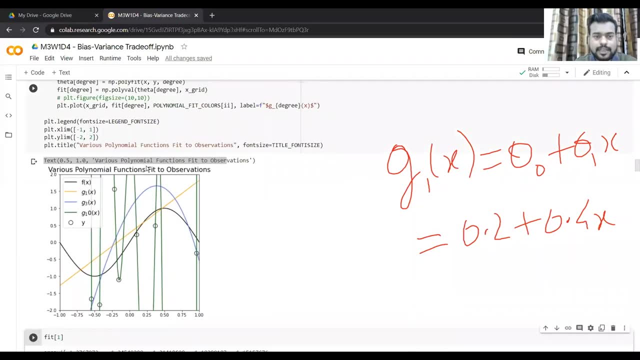 value less One point eight to two be somewhere here. 1.822 to something like this. So right, and so this is the g1x. So, just for now, focus on this orange line, which is this your g1x, right, and? 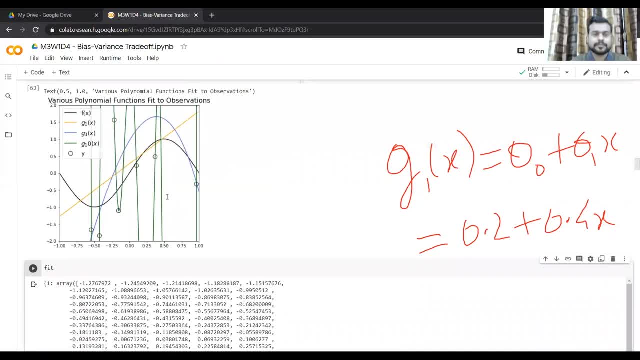 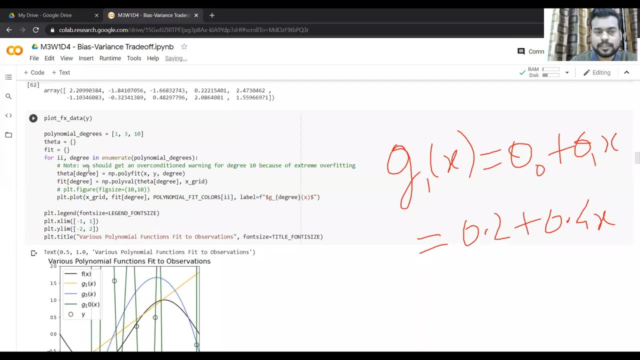 so you can see. now we will be repeating the same set of same experiment for another degrees. So here I have three possible set of degree value. So firstly I go, I did this experiment for g1x, then we can do this for g3x, right? So how our g3x will look like, so our g3x will. 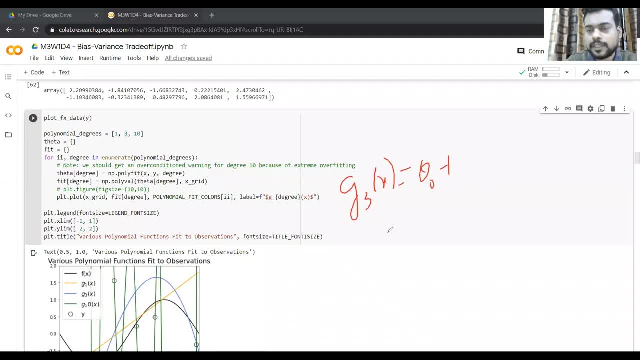 be something like: So: theta0 plus theta1x plus theta1, theta2x- square plus theta3x- cube, right? So this is your g3x. so we are again fitting this function on our given values of x and y. So those are only. 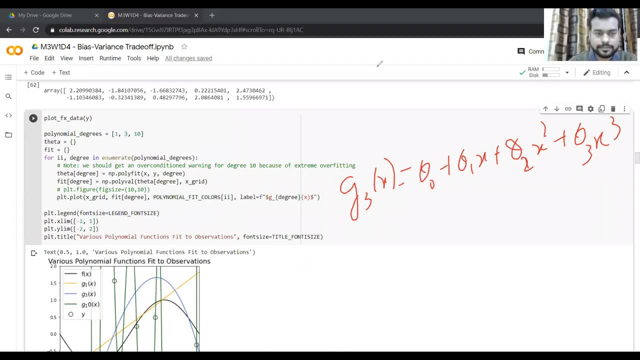 10 observations, right, and yeah, and then, once we have misguided these parameters, theta0, theta1,, theta2, theta3, from these, So So, so, these are. these are the previous 10 observations. We are making the predictions. you, on all those 100 x values, right, which is defined for your x-grid, right? So that's. 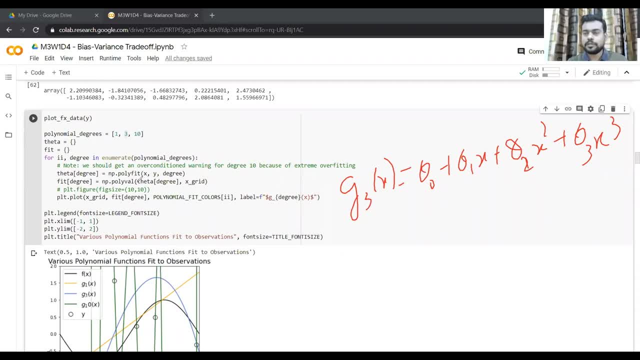 why this is called polyval. So here you are not quitting. So you come up with a model That's a G sum g3x, And then you're just plugging all those hundred values of x in your G3 and getting some value. So here, if you look at right so far, the term you know- you can find: 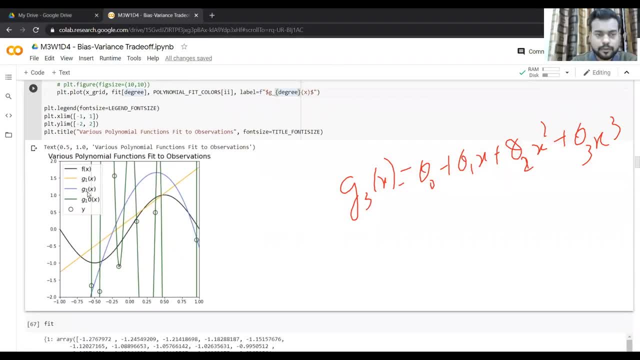 x in your g3. that's why this is called polyval. So here you are not quitting. so you come up with a model that's a G sum, g3x, and then you're just plugging all those 100 values of for this g3x, which is your blue curve here. So it looks like something. looks something. 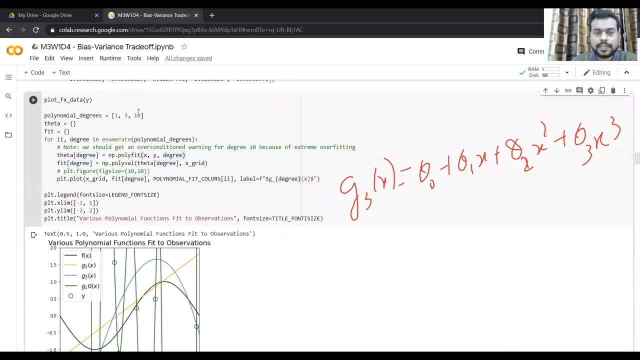 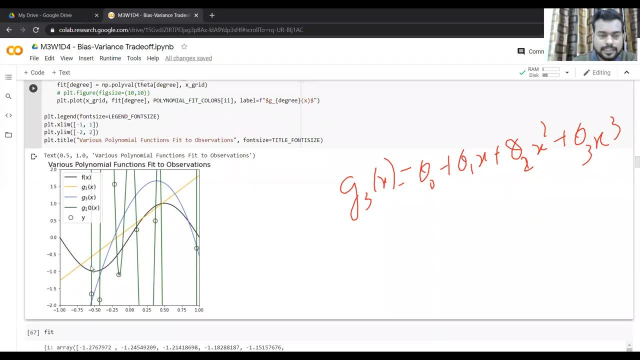 like this, then we can do fit a 10 degree polynomial. So what it will do? so, because they are 10 observations. So, as we can see that this green curve, which is the 10 degree polynomial, So it actually is passing through all these points here, all these dots, right, as you can see this blue. 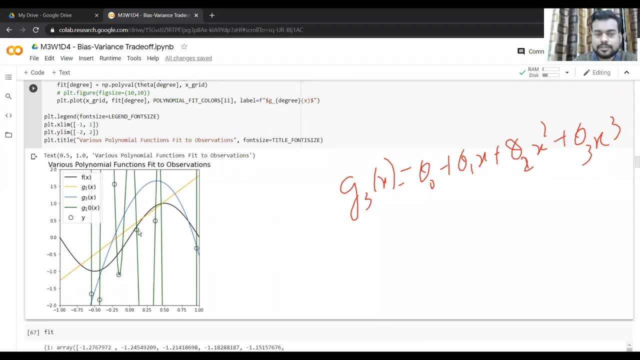 and the orange curve. This is not necessarily passing through each point of values, but this 10 degree polynomial is passing through each values of our X right. So so what this tells us? so this tells us that the high degree polynomial is overfitting as in it is trying. 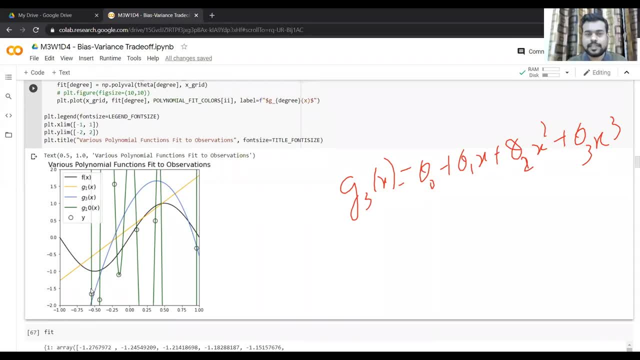 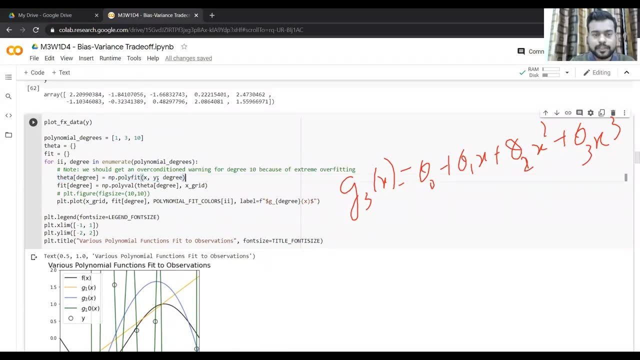 to fit to all the values of X and Y which it has seen during the training or during the fit in right. So this is the step Right. So it has seen 10 observations and it's trying to fit a 10 degree polynomial. 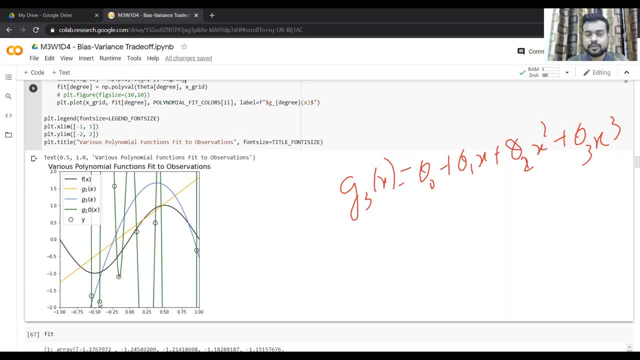 So, yeah, so it's, it will is at least be passing through all these points, right and then. but you, as you can see that this orange line, this is under fitting, so it's not passing through any of the values, but gives you some sense of idea that this is how your function should. 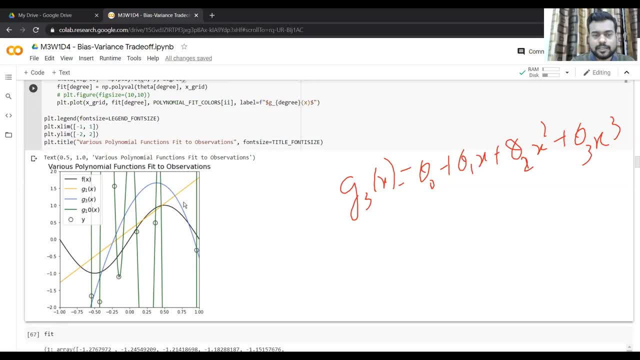 look like. and then there there is your g3, which is denoted by the G, Which is denoted by your blue curve, which is somewhere in between right, so it passes closely through some values. So, for example, this one, this one right, it passes through. 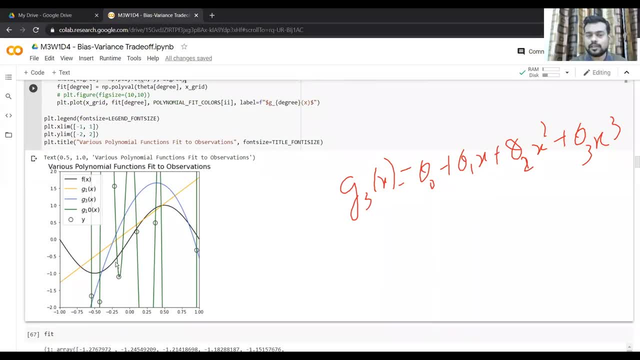 some values closely, but it's also not covering all those values, right? So so we'll say this orange line to be underfitting the data, and this green function, or yeah, the curve defined by the green line here, will call that this is overfitting the data. 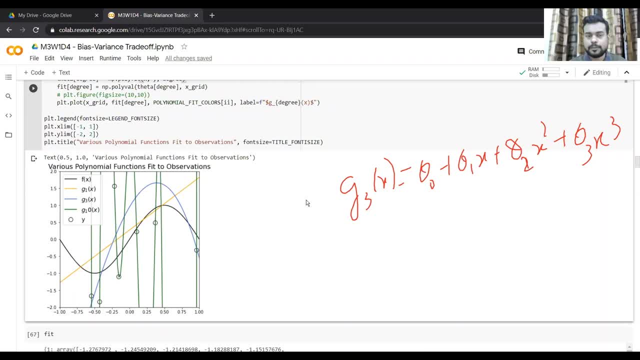 Okay, so I hope you are now familiar with why I'm saying underfitting and overfitting, right? so so as in when you are fitting the data, let's say, if your y value it's actually mapped to all it's the deviation between your actual values and your fitted values. if these 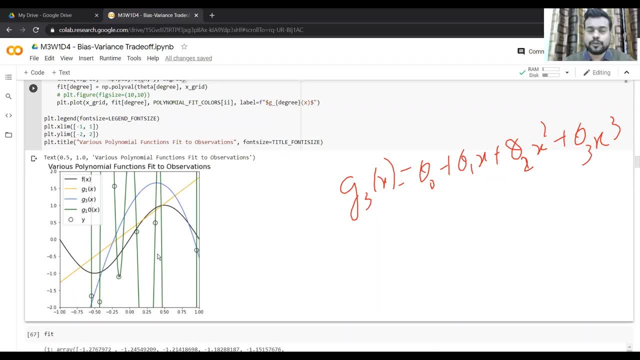 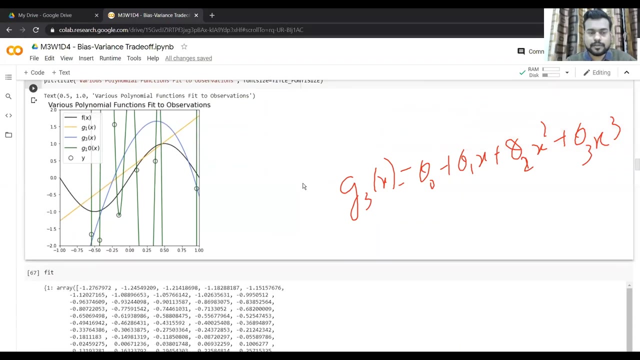 are very small, as in almost zero, so that will call is over fit. But if the deviations are quite Large, so we'll call that under fit, Okay, and if the deviations is somewhere between that, so it will be between an underfitted case and overfitted case, Okay. 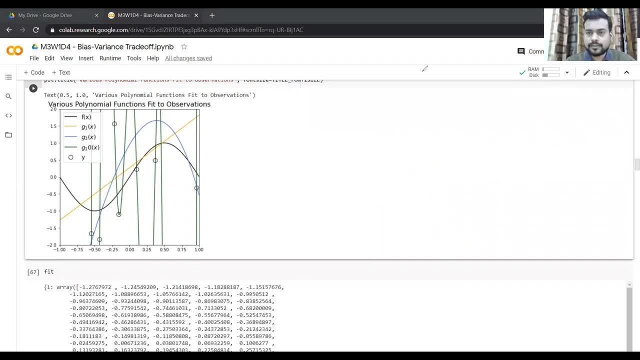 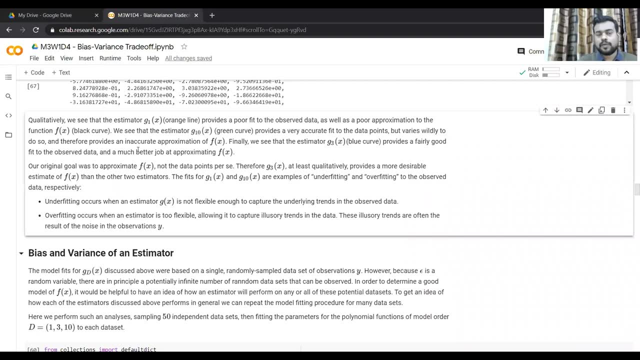 So, yeah, Okay, so so this is so. I hope you just got the idea. So what? so I'll tell you. yeah, I'll just read these out so that you can, yeah, misunderstand These concepts again. So, qualitatively, we see that the g1x line, which is our one degree, 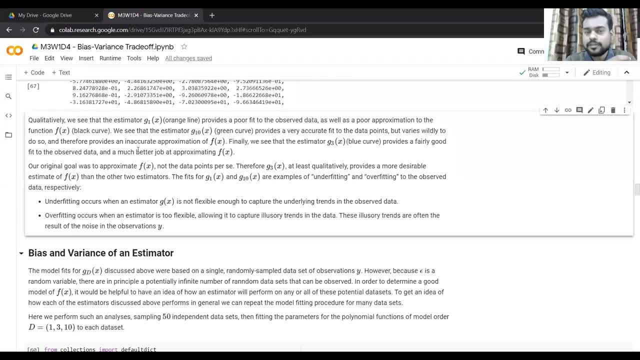 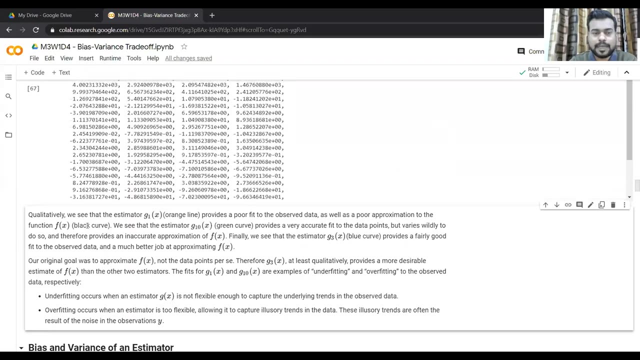 polynomial. it provides a poor fit to the observed data right, So it is not doing a very good task at fitting the observed data right And it also gives us a poor average approximation to our function effects, which is our black right. So remember, this black curve is actual. 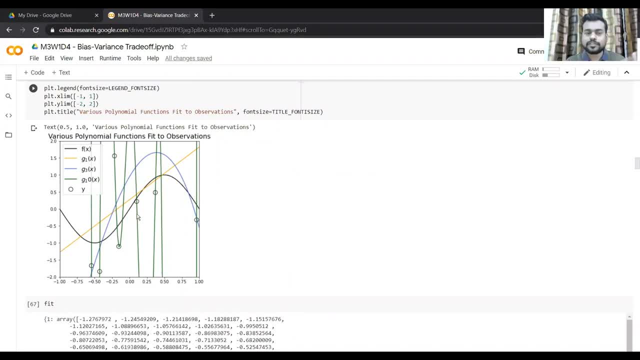 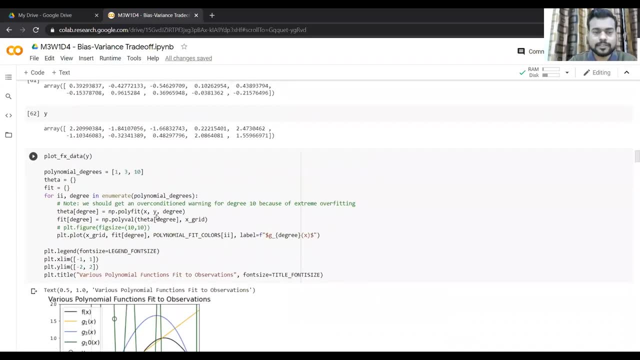 sine pi x. This is what we have assumed to be the true relationship Between x and y, right? So that is, that is how we have generated these xy value pairs, right, That is how we have generated xy value pairs, right, Using the sine pi x. and we are 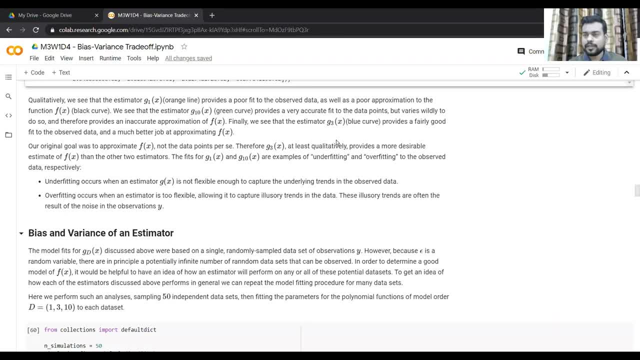 trying to come up with estimators which will approximate our effects, right. So these approximate estimators were calling at as G's. So g1x is one degree polynomial estimator, Then g10 is the 10 degree polynomial estimator, and then we also see that the estimator g10. it provides a very accurate fit to the data points. but 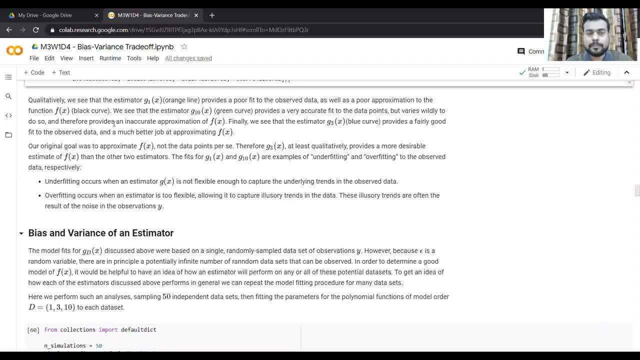 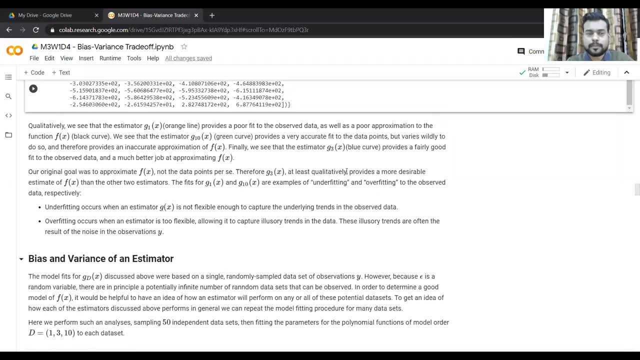 it varies widely to do so and therefore provides an inaccurate approximation of effects. right, And we see that g3x, which is the blue curve, It provides a fairly good fit to the observed data and it does a much better job at approximating effects. 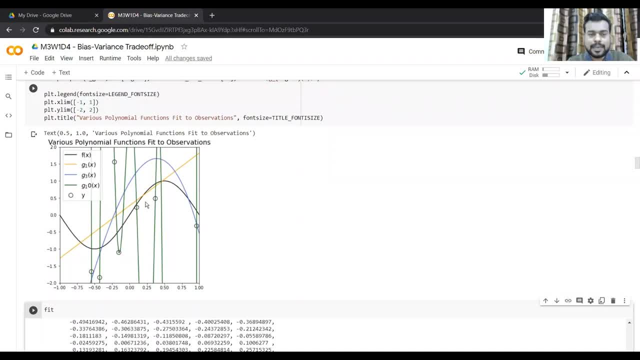 I want to, I want you to have a look at this. So this is the black function which we are trying to approximate, And so this orange curve is not doing a good task in approximating this black curve, but, as you can see that this particular blue curve is sort of doing a relatively better task, 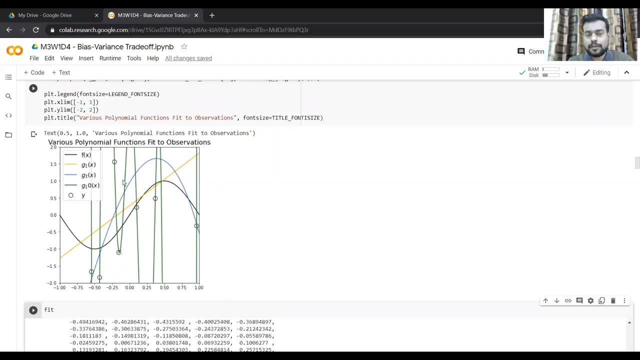 in approximating. and if you look at the green curve, or even though it has fitted all the scene values, but it's nowhere close to our, this black curve, right? So this is also not doing a good task At approximating effects, right? 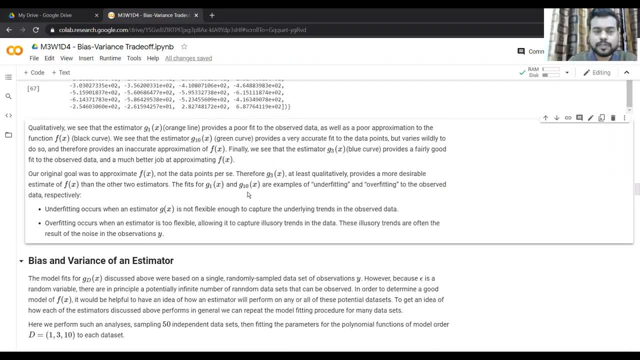 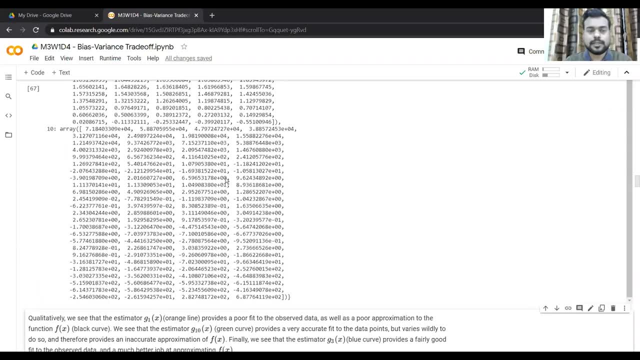 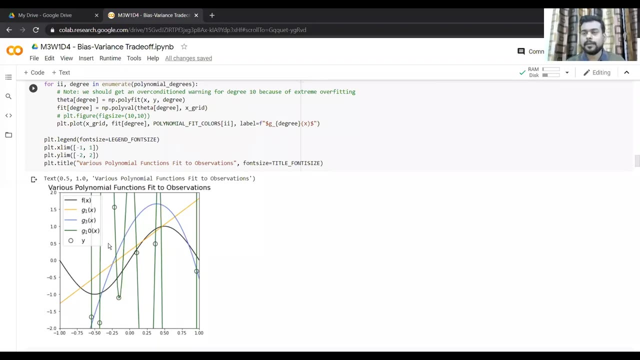 So you remember what our original objective was. So our objective was to approximate effects and not the data points per se, right? So of course, as you say, based on your 10 data points, right, You will see that the green curve has done the, or the 10 degree polynomial is doing giving. 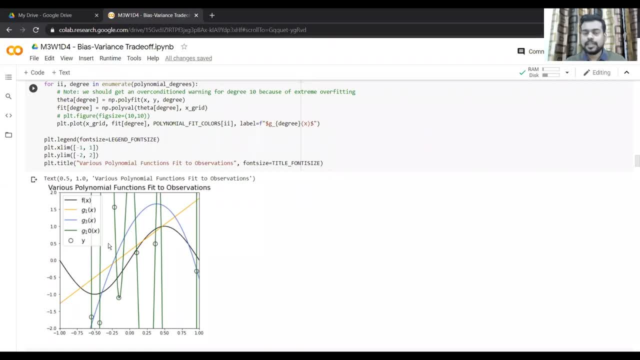 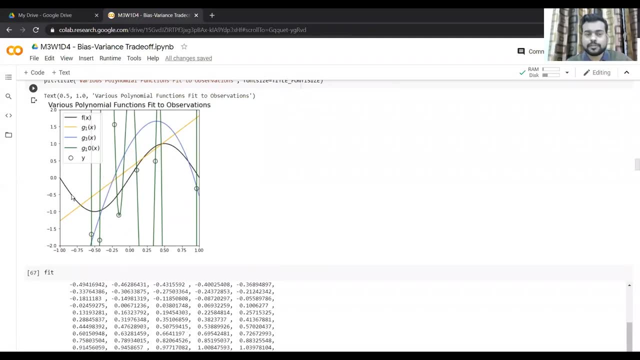 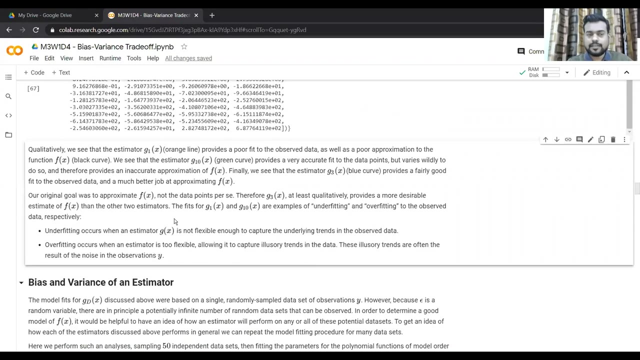 us the giving us the best fit. right, because it has actually fitted all the values, But we can see that this is not actually a very good approximation to our true function effects. Right, So? so again. so our objective was to approximate effects with some estimators. G, so we can see. 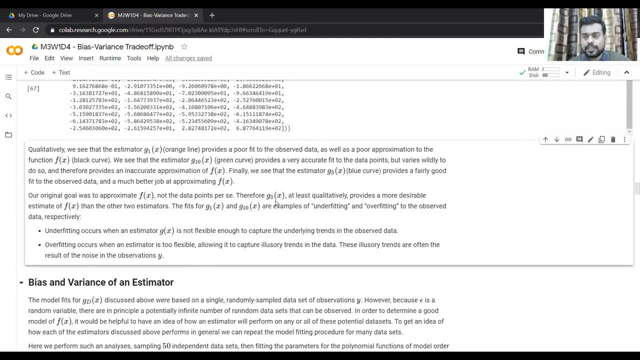 that at least qualitatively we can say. of course we have not yet quantified, but qualitatively we can say that G3 does the best job out of these three estimators Okay In approximating FX right, and the fits for G1 X and G2 X are examples of underfitting. 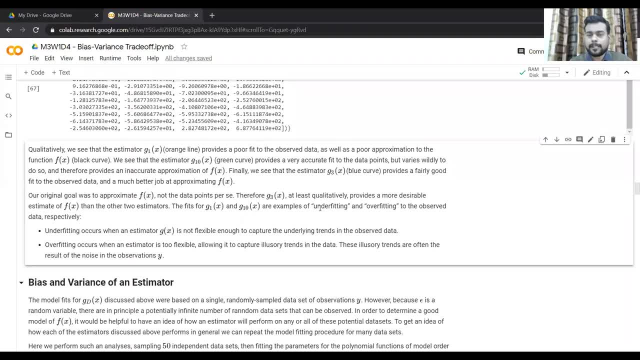 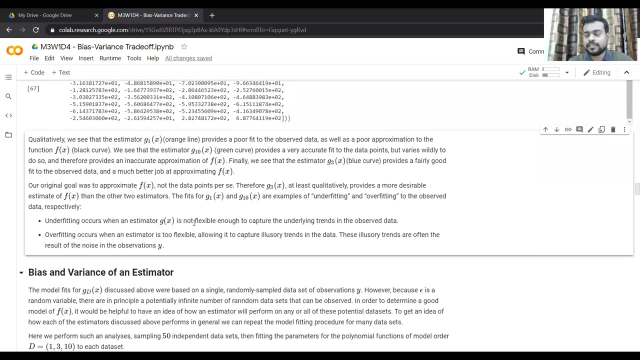 as in G1 X is sort of doing a poor fit and G10 X is overfitting, right. So it has fitted all the values but still it is not a good approximation to FX, right. So underfitting occurs when an estimated GX it is not flexible enough to capture the underlying. 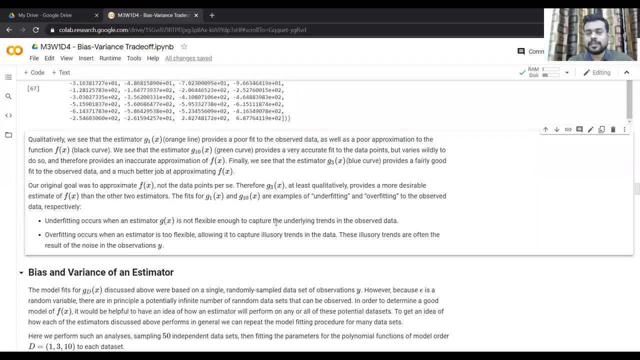 trends in the observed data. So it is not flexible, Right. so underfitting occurs when an estimator is not flexible enough, as in. the model is relatively very simple, It's not complex. Okay, It does not have a lot of parameters, does very few parameters. 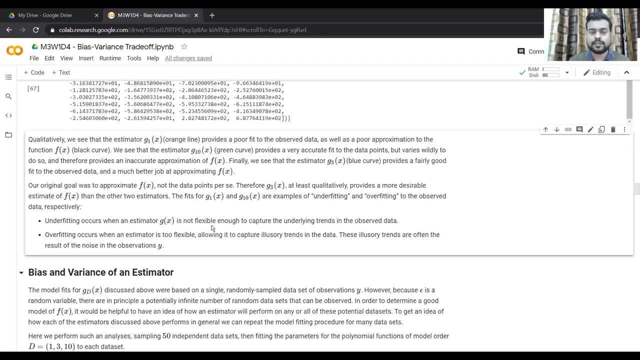 So in that case an estimator will under fit the data right. So that is what is meant by this particular line: that when an estimate is not flexible enough to capture the underlying trends in the observed data, that's when it is going to under fit your data. 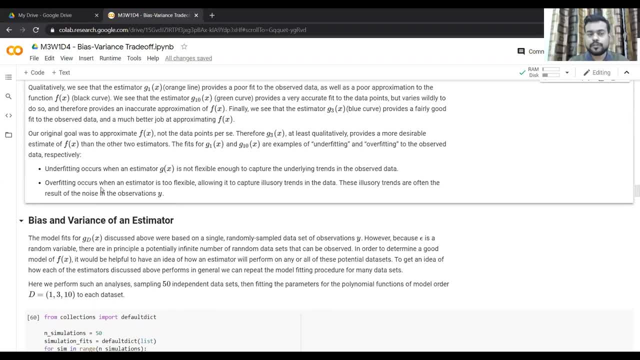 Then we have another case which is overfitting. So this overfitting occurs when your estimate is too flexible, right Of course. So when we had 10 data points and you're fitting a 10 degree polynomial, so you're expected. 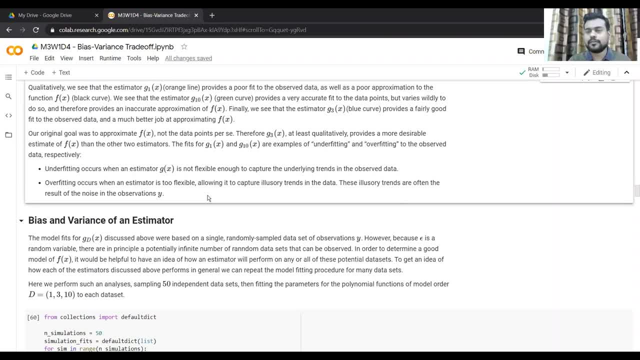 that it will sort of fit all the given values, right. But that was happening because your estimator was too flexible. right, It was too complex. It has a lot of more learnable parameters And that's why this estimate Is more flexible, as in your 10 degree polynomial right. 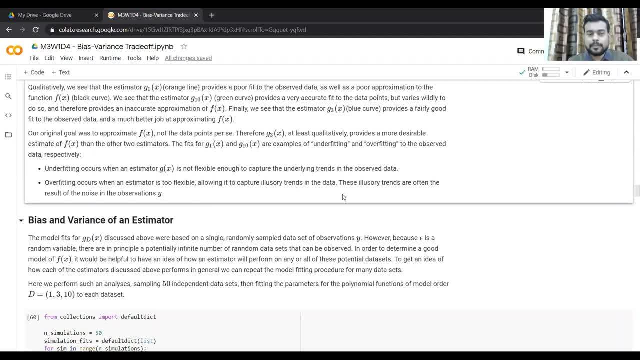 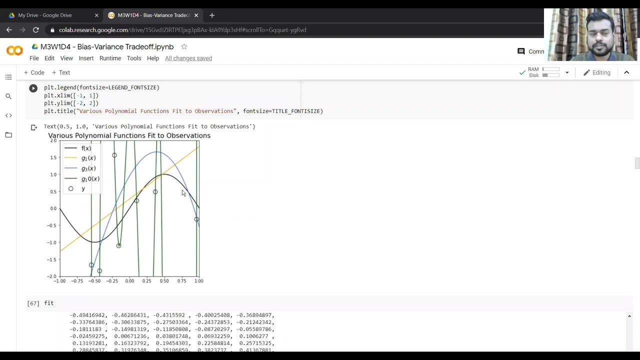 So allowing it to capture illusory trends in the data, but these trends could often be the result of noise in observations Y. So right, So that's why we are seeing that this particular green curve is does not seem like a good approximation to this particular function, which is your sine pi X in this case, but the blue curve 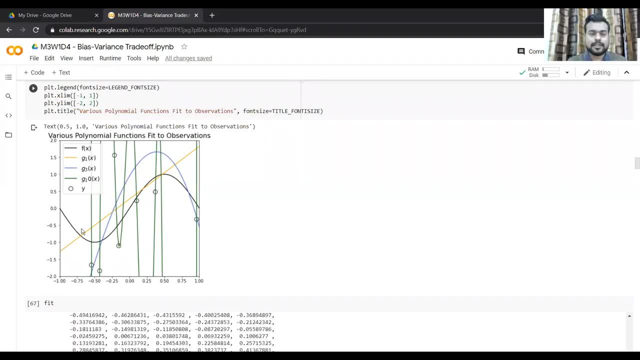 does a better job, So that is g3x, So so I'll write these here so you can. yeah, so this curve is underfitting right or doing a poor fit, So it's underfitting right. This green curve, this green curve is overfitting and we can say that this blue curve- right. 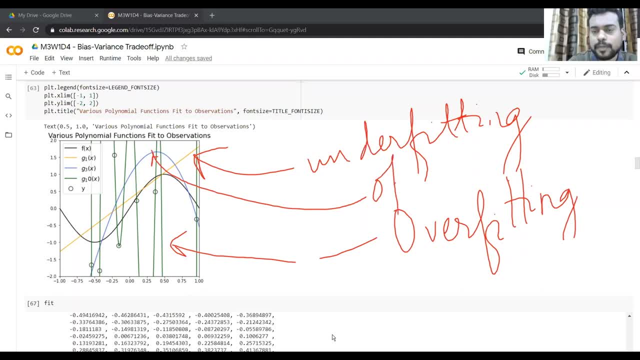 So this blue curve. So this blue curve is sort of giving us an optimal fit Right. So it is giving given, giving us an optimal fit right. So it's more or less at least out of these three estimated, We can also have a whole four-degree polynomial. that could give us much better approximation. 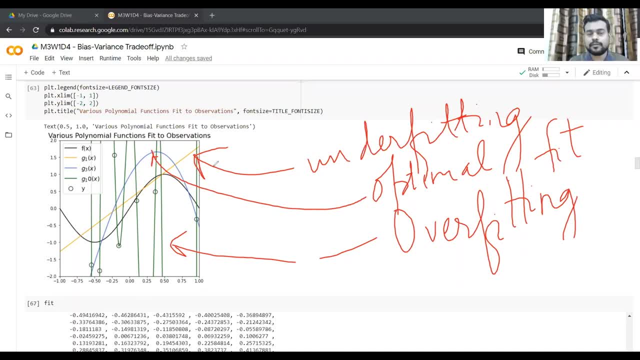 to the sine pi X. but out of these three estimators, we can flag them as so. this- this is the model, This is the estimated with very few parameters- is going to under fit, Okay, And this green curve, which is a model with too many parameters, which is flexible enough. 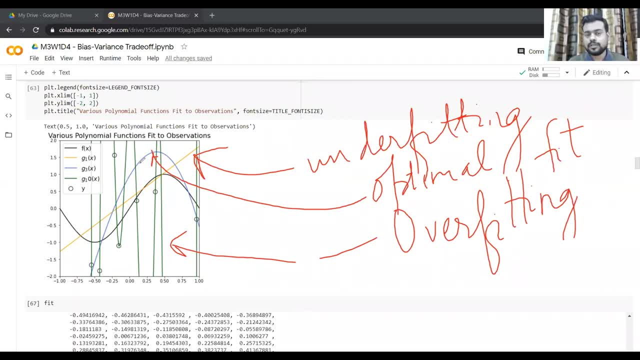 So it will overfit the data. but this blue curve, which does not have a very large number of very small number of parameters, but somewhere in between, so it will, it is going to give us an optimal fit. Okay, So I hope this concept of overfitting and underfitting is clear to you, at least with 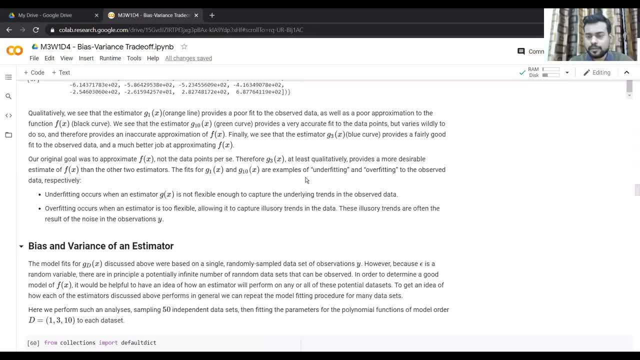 this particular experiment. Okay, So can I know from you if this concept is clear, The concept of overfitting and underfitting, right? So you, when you're choosing high-degree polynomial, that is a complex model, right? So a model with a large number of parameters is more complex. parameter model with very 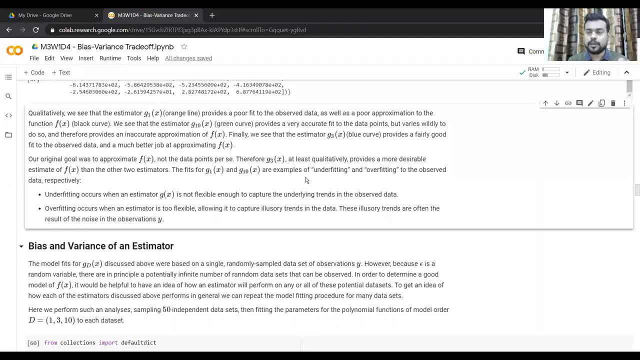 small number of parameters is simple, right, So we are going from simple to complex when we are going from degrees One to 10.. Right, So I hope, yeah, this is clear to you. Yeah, that's great. So, yeah, 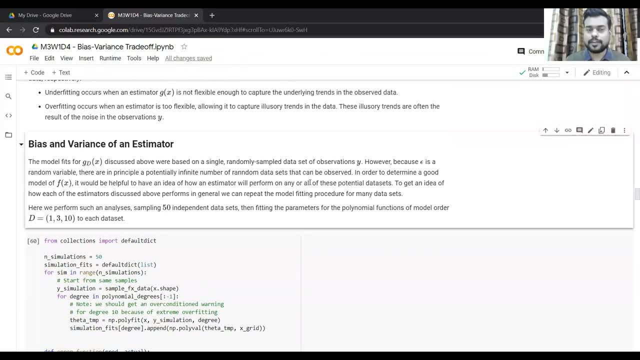 So now, once we have understood the concept of underfitting and overfitting, we will glance upon the concepts bias and variance of an estimated. so before I go ahead, so of course you know what is an estimator, right? So an estimator is again a function which we want to come. 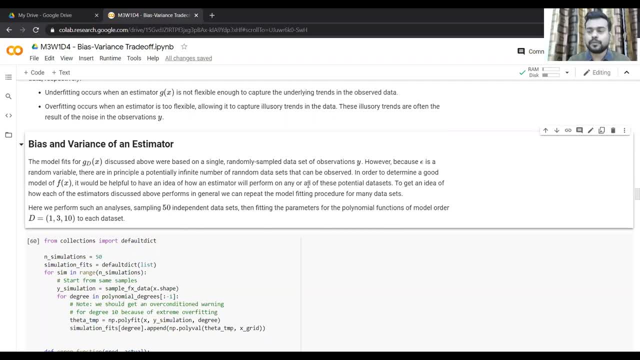 up with which will model the relationship between our observed pairs of X and Y. right, So this is what an estimator is, right. So the model fits for GDX as in D is your degree of freedom. It's the same function which we have seen above, So discussed above were based. 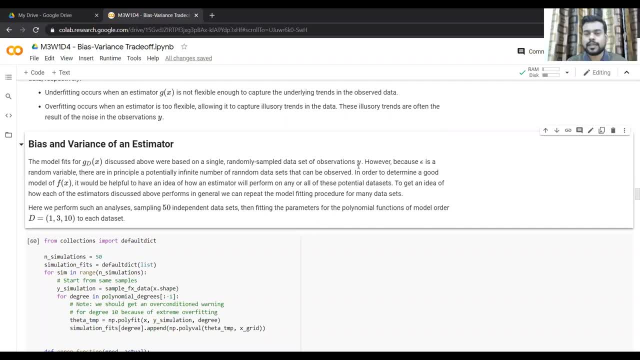 on a single randomly sample data set of observations. Y, right? So when we fit that model, so that was on some particular data set of 10 observations, right? So we had X and Y, So I can tell you that how our data there looks like. look like: right, So we have some 10 observations, right? 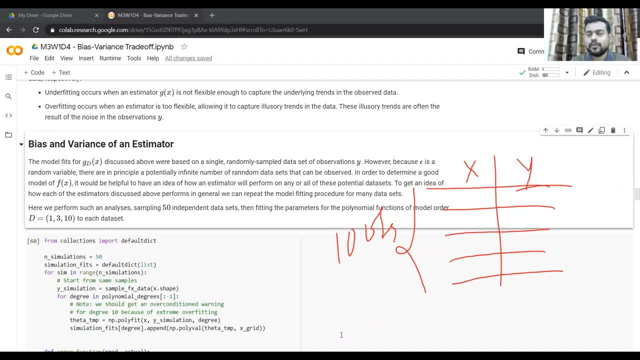 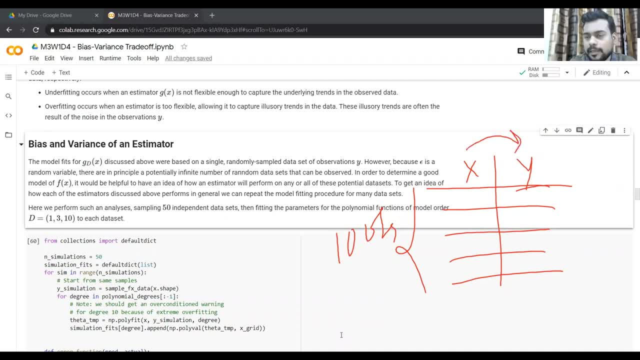 we were sort of trying to find an approximate function. We're trying to model Y with a function G. That is what we're calling as estimator, right? So this is 10 observations. So now, however, because you're epsilon, remember? we added some noise over dependent variable. 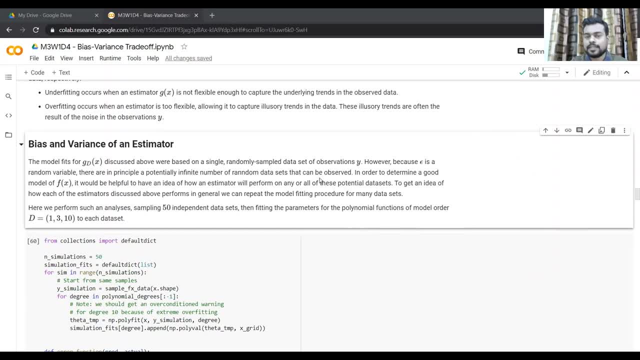 trees right. So we have some values that are not sufficient to see the kinds of improvement that we're going to have. So this is kind of the understanding end to end model of data set interesting. I would like to share with you a little bit of an overview of the different models. So first, 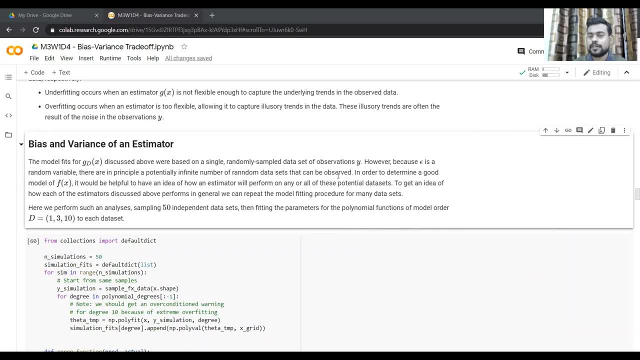 of all, we're actually going to have a data set that is stable. So my guess is that we have 4,, 5,, 6, and 8, right, So we have some numbers that we can save. We can come out. of the 2-D right, And then we have a number of infinite number of random data sets that can be observed Right. So I guess you would agree with this particular point that in principle, we can have potentially infinite number of random data sets right. So in order to determine, 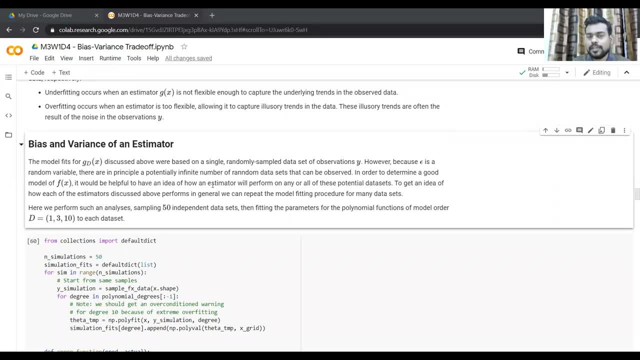 a good model of FX. it would be helpful to have an idea of how an estimator will perform on any or all of these potential data sets. So right, so we are just looking at one data set, right of 10 observations. So just looking at one data set, but we can actually repeat. 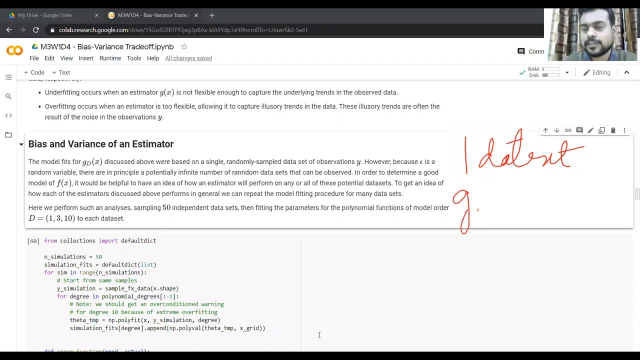 this experiment for a given estimator, Let's say for g1x. right, So we can repeat this experiment across a lot of data sets. right, So to get an idea of how each of the estimators discussed above, right, So how they perform in general, we can repeat the model fitting. 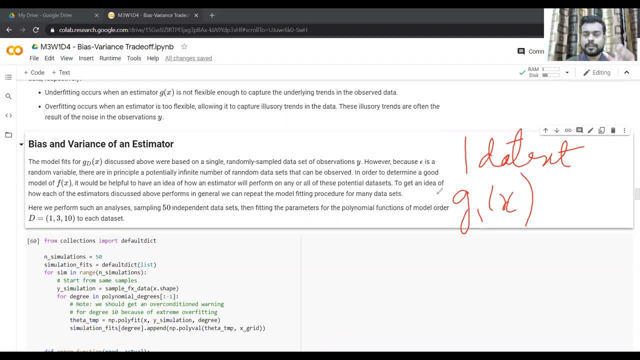 procedure for many data sets, right? So we just create a model for a data set consisting of 10 observations, But we can in fact repeat this analysis for as many data sets as we want. So in our experiment we'll do such fitting for a given estimator, right? So I'm 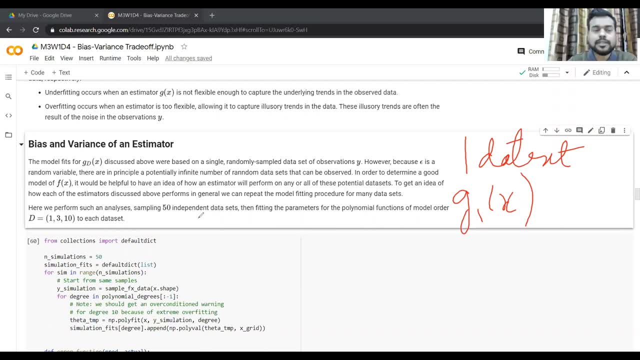 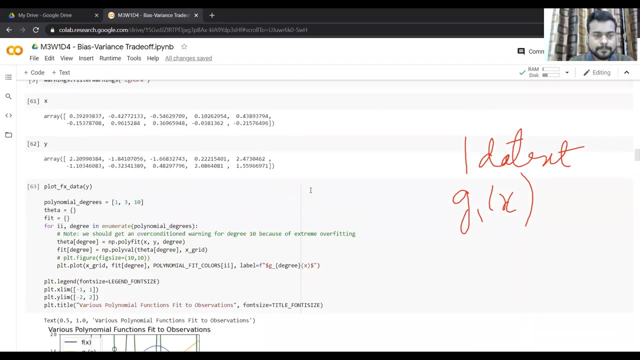 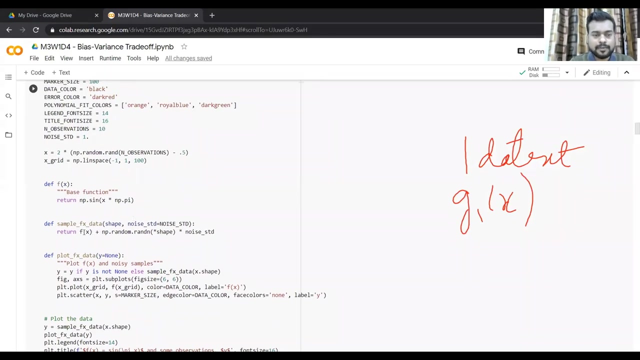 saying, for a given estimator, that is, let's say, g1x, We'll be performing an analysis of where will one will sample 15 independent data sets. So so, remember so, when we are written, x and y function. so so this thing will be, will be. 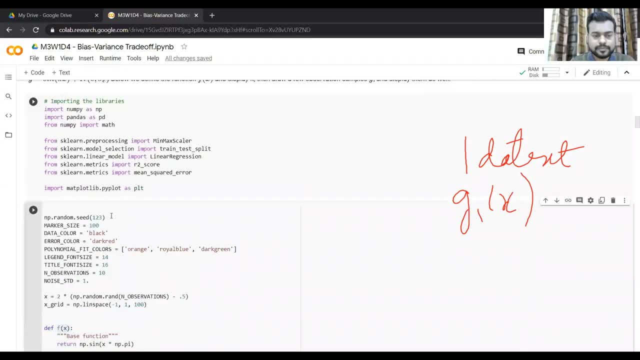 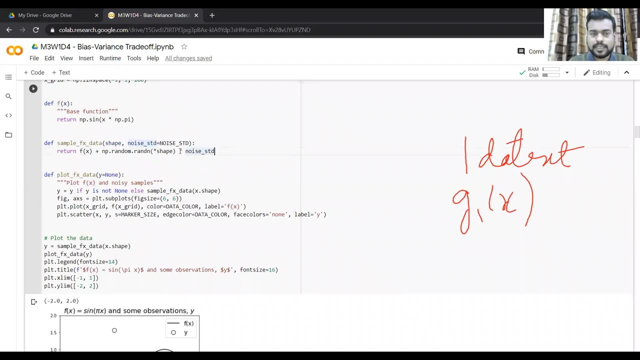 the same right, So fx will be the same because we have the same set of x right. So g1x, g2x, g3x, g4x are the same. But whenever we are randomly sampling, taking the noise, 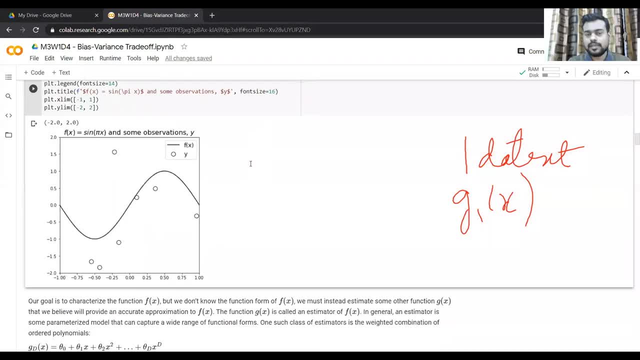 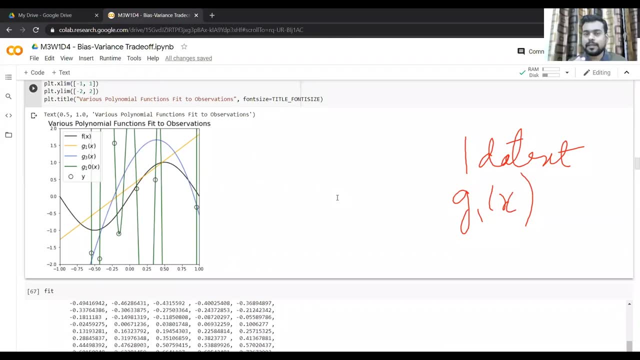 right, so this value could be different, So our data set will differ. even though the values of x are same, y can be different because we are sampling from a normal distribution for noise from sampling from normal distribution, And so we can have different values of y when 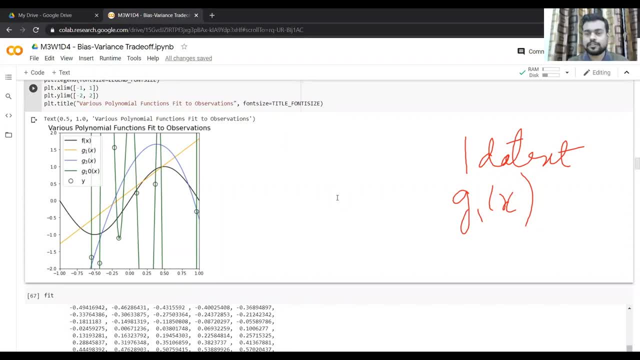 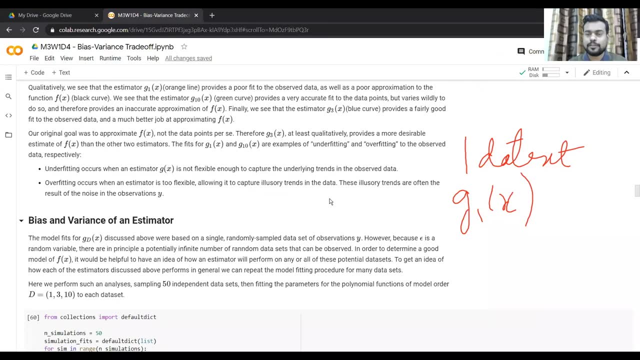 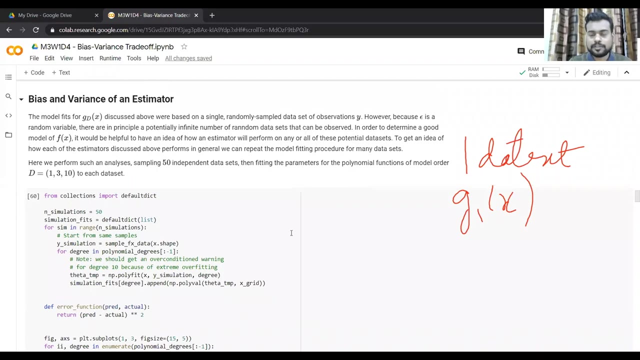 we're looking at different data sets, Right? So so we can definitely say that these are different. data sets are different, So we have a different set of values for x and y pairs, right? I hope that makes sense for our given example, right? So I'll just write this again. So what? 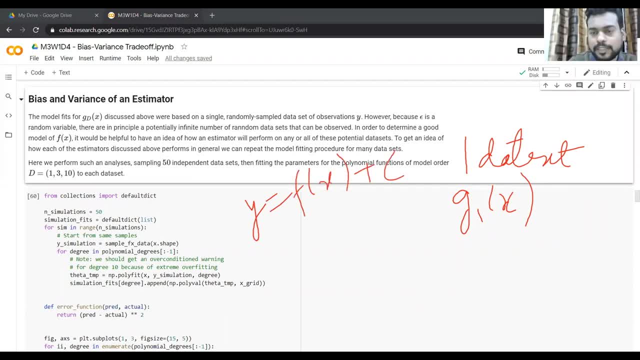 was y. y is equal to FX, plus some noise. So this is what will change. which will change the value of y. this will be more. this will remain the same. Okay, so x will remain the same, and, but the noise when we sample it randomly, so that might change. So this pair of, so this. 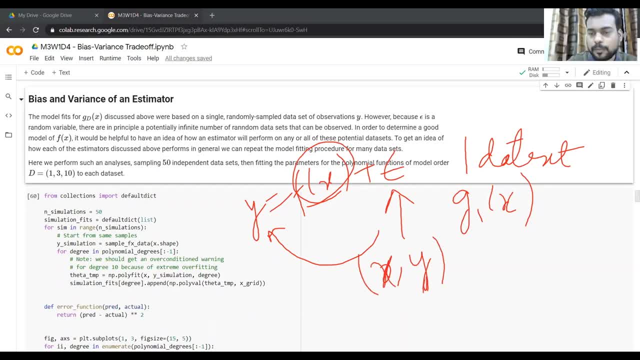 x comma y, right, This x comma y, So this whole pair will change because y is changing depending on the noise. So what we want to do, actually to do with this experiment, So we want to see how are estimated. So, for example, this g1x performs across all these data sets. 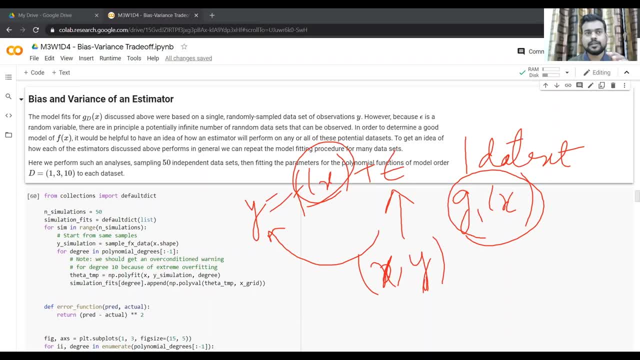 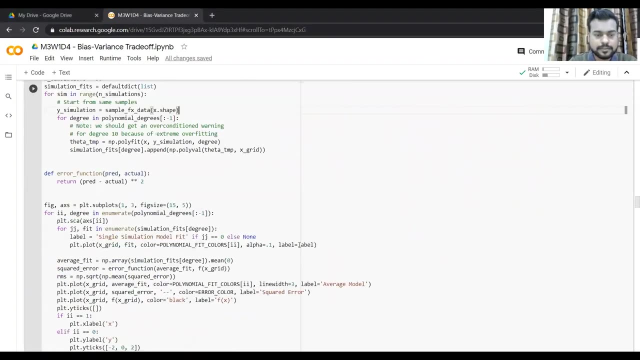 right, So we will have a data. So we'll have 50 data sets, each consisting of 10 observations, right, So? so, yeah, Yeah, that's clear, Yeah, So here's another function which I have written, So in this case, I'll. 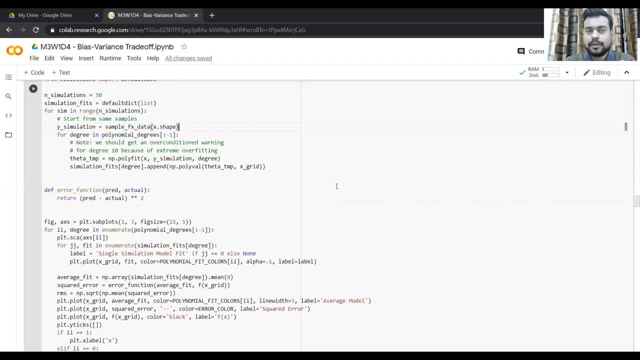 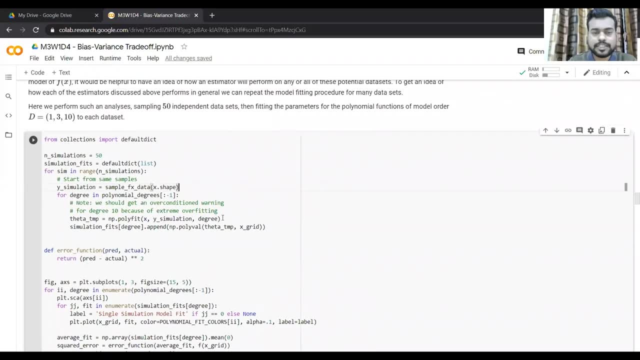 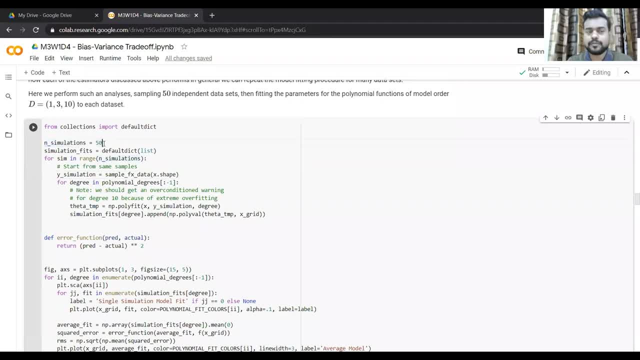 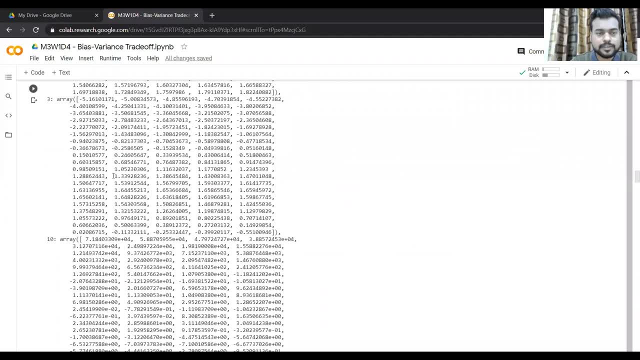 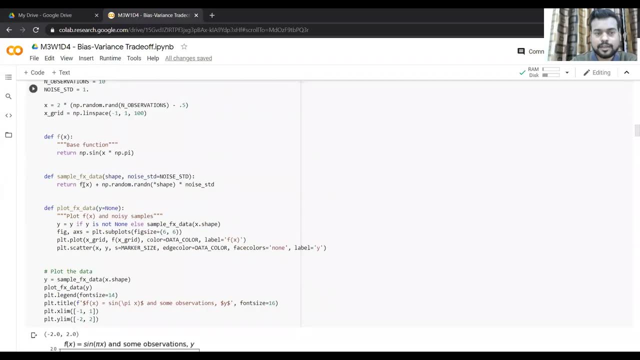 data. right, So remember your sample effectswhat How it looked like. Yeah, So there's a low flag, as we had written this particular value. Why So? So for our shows, whatever the xv is this box and it's high in sound isolation, Isn't it what this looks like? You know anywhere? 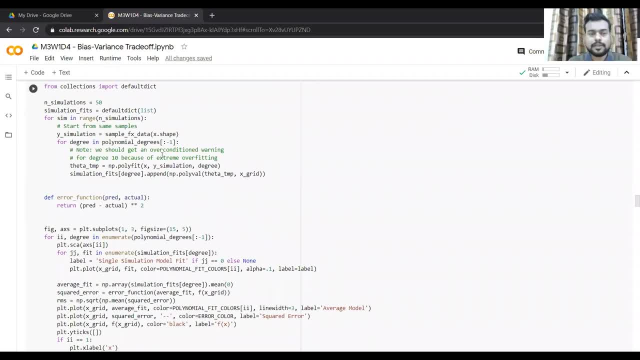 of the four values that different. All right, So the other virions. I'll just pass this now to given ybox plus some noise. So whatever the X we have will, yeah, for each simulation or, as in for you, for each data set will have a different set of values. for white: 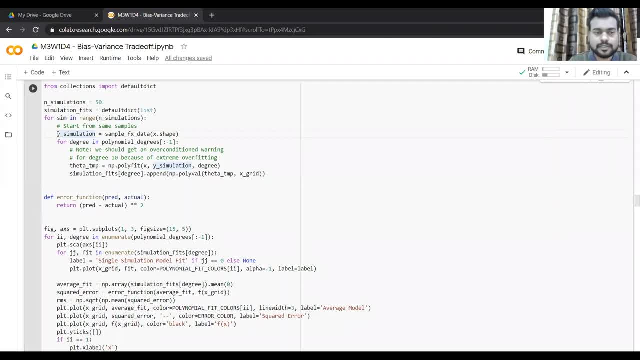 So of course we'll say that that's a different data set, for Y is changing right. So again, we are what we are doing, we are yeah, so we are fitting. so for all these simulations. So let's say, for one particular data set or where what we are doing we're repeating the 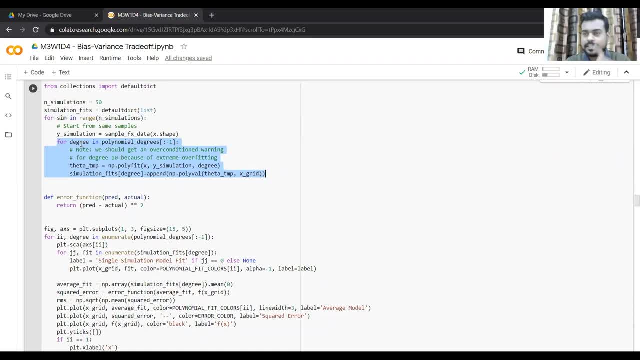 same exercise as we have done above. So for each data set we are fitting these estimators, which are g1 X and g3 X. So I'll just write this here so that you have this in mind. So we will be fitting these two estimators across. 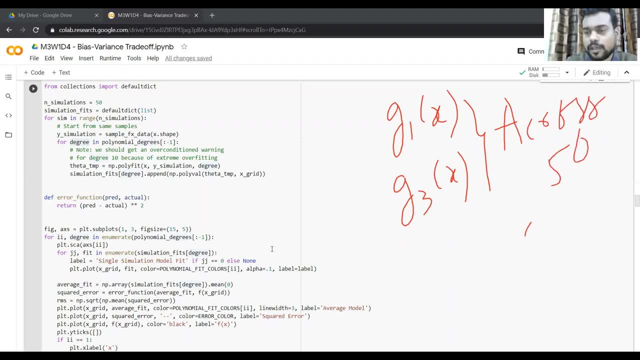 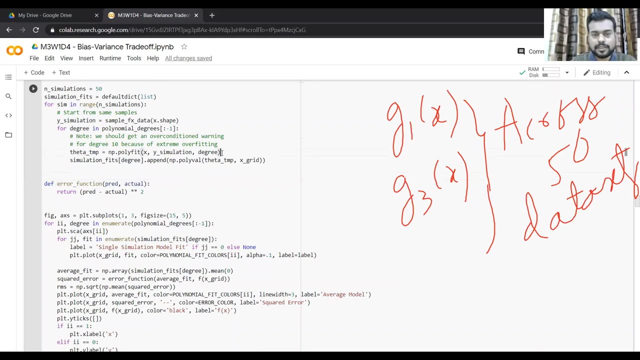 So across 50 data sets, or what I'm calling as simulations. So so, yeah, so I'm just, yeah, fitting this here, right, I am fitting this, and then, once I have gotten that estimated, so I'll just try to get the value of those estimators for. 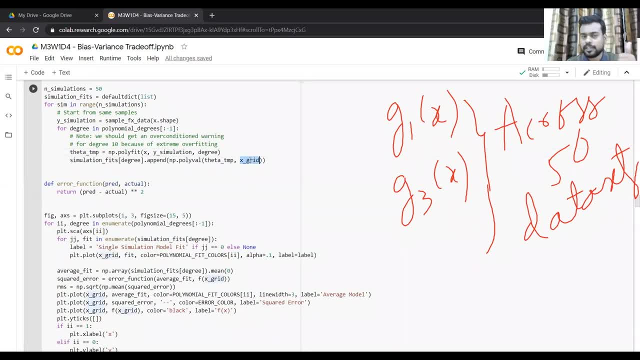 all the hundred values of X. so remember X grade from earlier. So this we are not changing. So of course it's not changing. Of course it has a set of hundred values between minus and one. So we are sort of predicting on all these set of values with our fitted estimator. 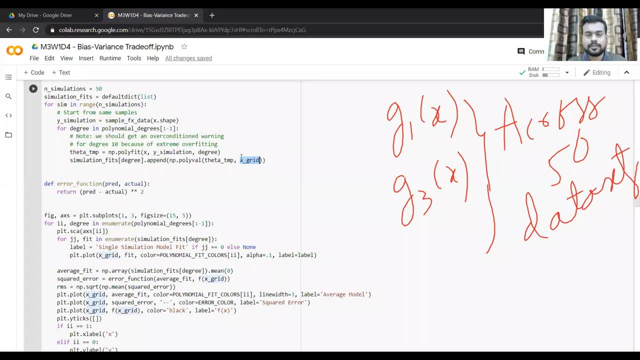 So for each degree we have, let's say, this line will give you all those set of possible values of g1, means it will give you a hundred values of g1 for all those X's in your X grade, right? Remember, we had a hundred such values. 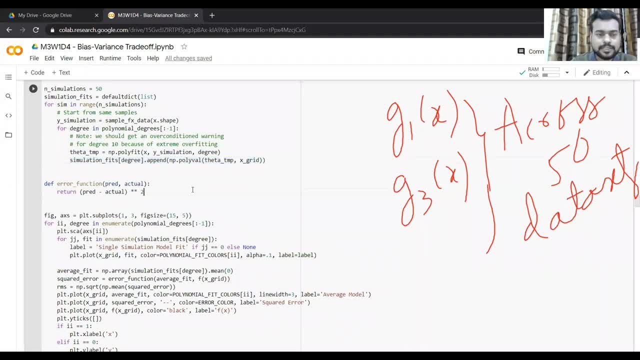 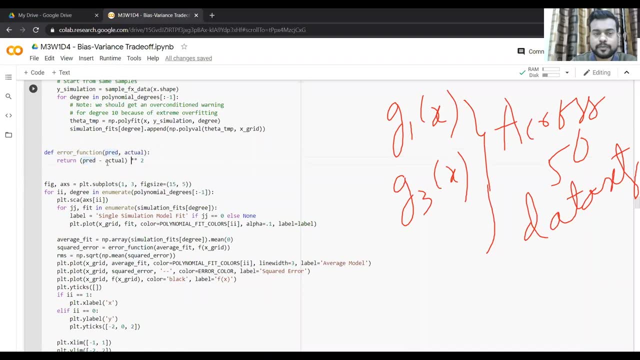 We intermediate this, So that's for of question. So I'll stop there with pretty quick. Next, I have calculated this error function so which will sort of calculate or return the square difference between your thread and actual right. So actually we know right. that is your sign. 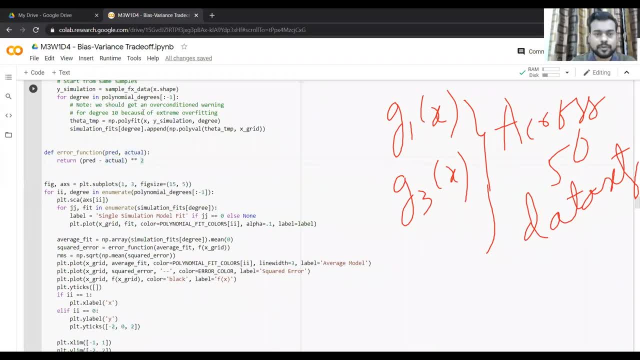 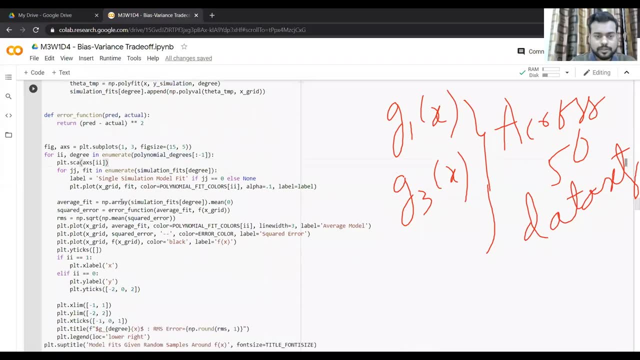 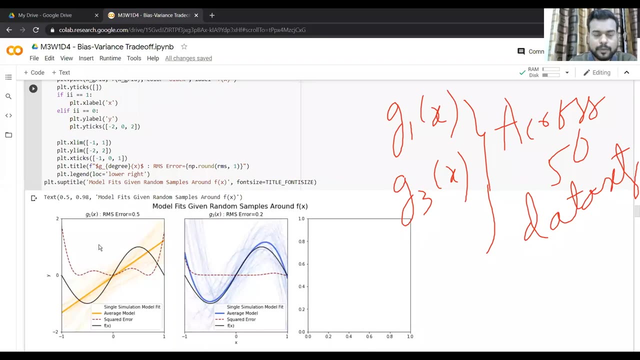 We actually know why. right, we know this Y. So this is our actual y. Yeah, so we are doing the same sort of things. And now, yeah, plot So what we are doing here. so we are running 50 simulations for, let's say just, 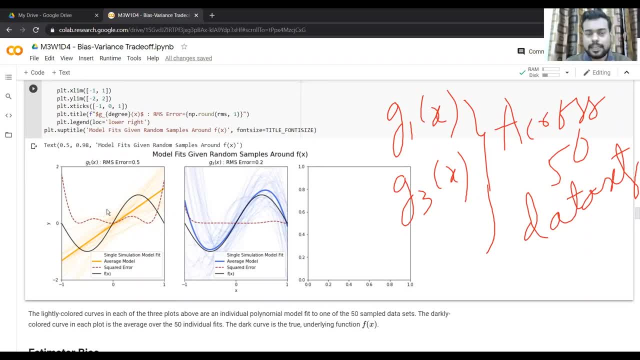 focus on g1x for now. right, So I'll tell you how what this graph depicts. So for this estimated g1x, that is when we are fitting g1x, that is, for one degree polynomial across 50 data sets, This is what it looks like. So this particular to all these light lines. 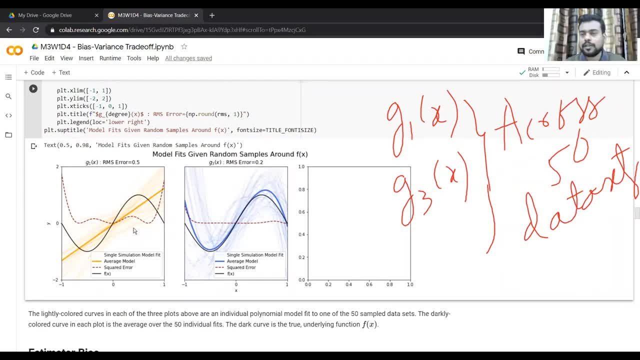 light orange blanks. So these are single model. fits for g1, right? So so we are doing 50 simulations where you can see there are 50 such single simulated line, right? So are you able to understand these light shaded lines which are here? So all these lines have been obtained. 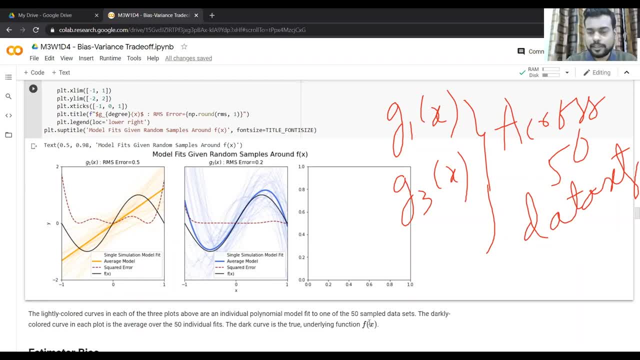 by so how these have been obtained. So I'll just give you the recipe for that. That's the same thing which we have done from above. So so I'll just give you. so just focus on this particular single line. So let's focus on. 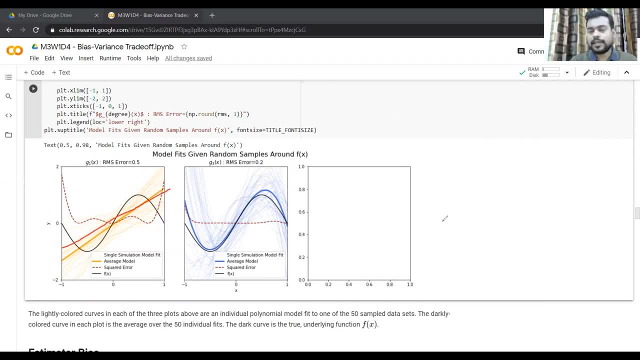 this particular line, right, So this particular line. so how we are getting that. so we are getting a data set which is your x and y value pairs. We are doing NP dot poly fit on this, Right? So we are getting some. so for this, I already know, Yeah, so we are fitting g1x. 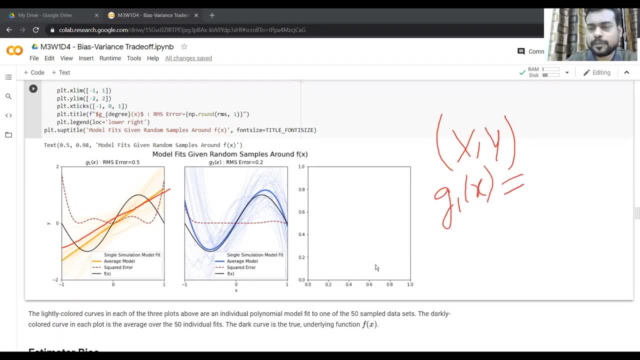 right? So let's say g1, this g1x for this particular data set, which is your 10 observations. Right? So 10 rows. So this g1x, let's say it was some one plus two x, it was something. 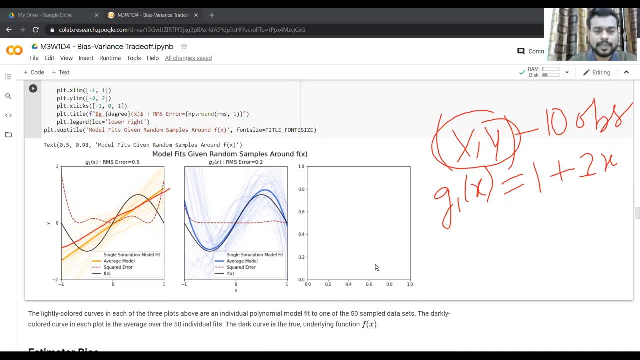 like this, right? So, for all these values lying between from minus one to one, all those hundred values. So I'll calculate this g1 for all those hundred values and I'll have some value using this function, Right? So, for example, this minus one, so I'll have this value minus one then. 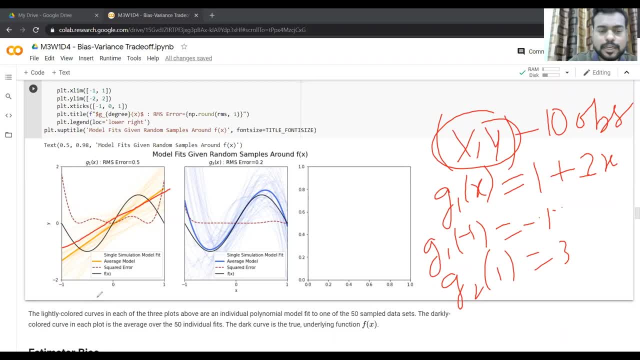 g 2, one will be three. So for all those hundred values lying between here, so all those hundred values, I'll have a corresponding value of g1, right? Okay now. so let's see for all those hundred values, Right. 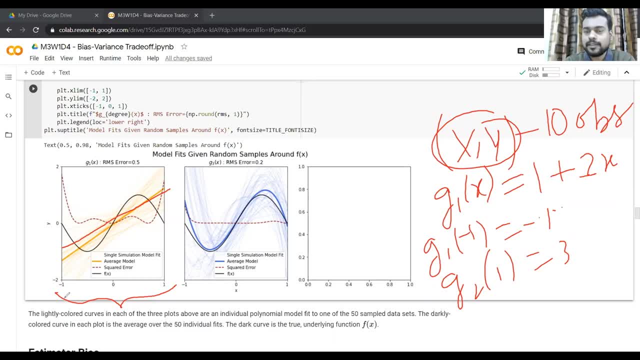 that is what we can also call as predicted values. right, so we have fitted our model by only looking at 10 observations for each simulation, so i'm just talking about just one particular simulation as of now, and then we'll be repeating the same set of procedure for all these simulations. right? so for 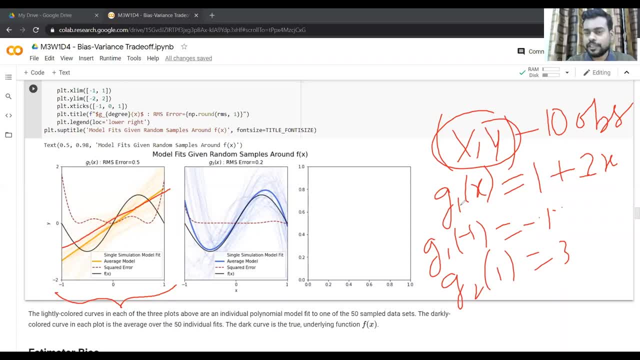 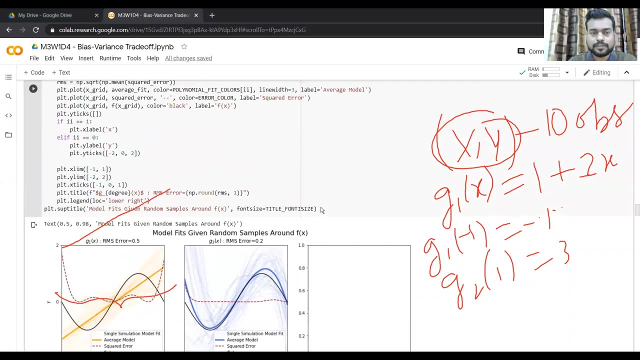 a particular simulation. we are training this g1x right on 10 observations. we are getting some values of theta 1 and theta 1 and then for all these 100 values we are generating the corresponding function values, right, the values of our estimator, for all those values, right? so you can see, this is. 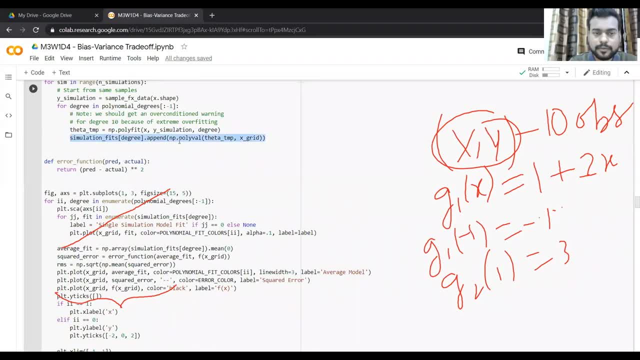 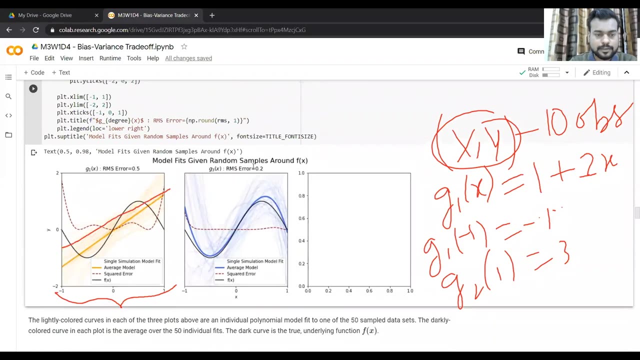 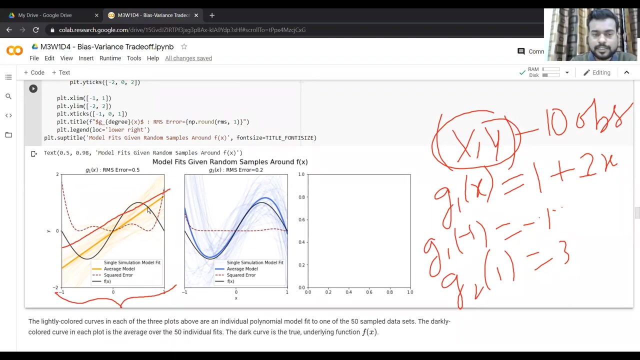 this step which gives us all those 100 values. right so here we are writing nppolyval as in: we are calculating the values for our fitted model across all these observations, right so? yeah, right so. this is one simulation. so for one simulation you will get a function like this, right so? 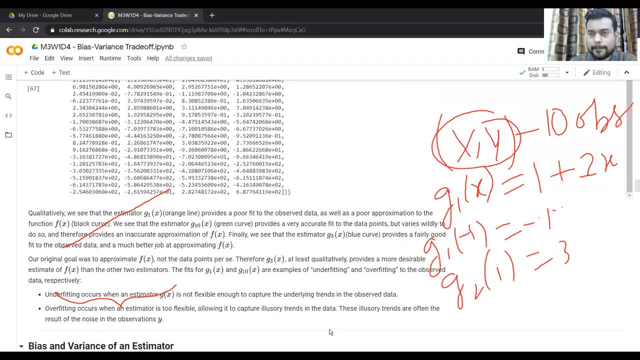 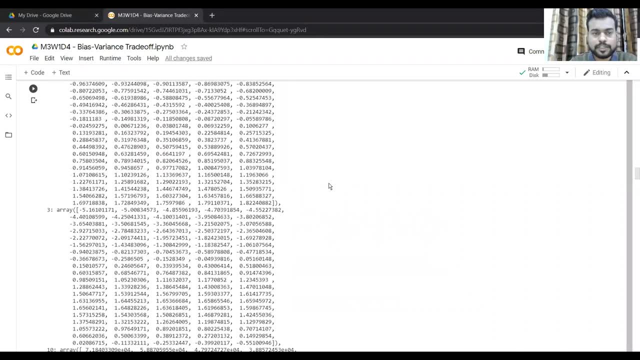 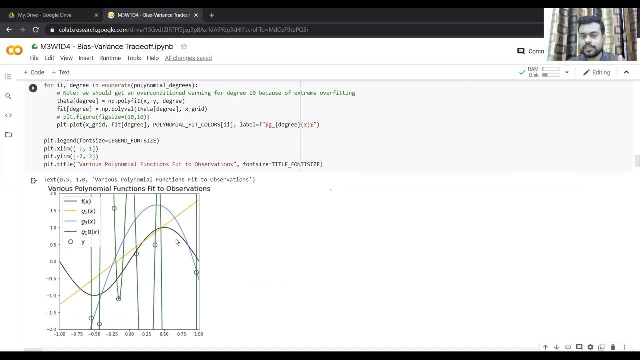 remember from, i think so from above, uh. so one simulation looked so for, so for, so for, just think of this particular orange line, right? so this was just one simulation for a given data set which consisted of 10 observations, uh, where we had two variables, x and y, right, and we have we. 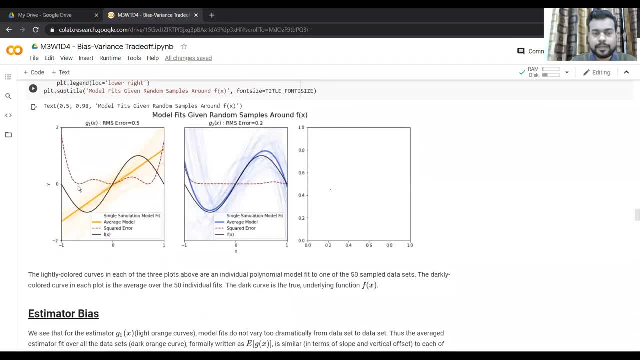 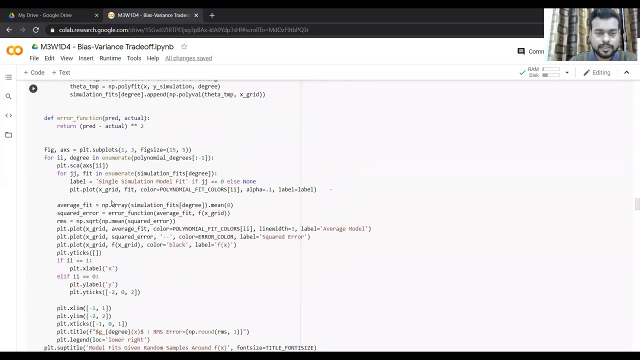 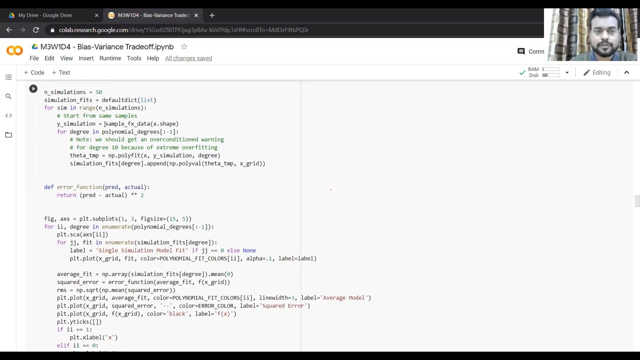 want to model y, only right. and let's say, we repeat this experiment, uh for uh, 50 times with, uh different data sets, uh of 10 observations each, but our y values will be changed then, right, because, as you, you can see from here, right, so when we are calling in this function, so we are adding a noise part. 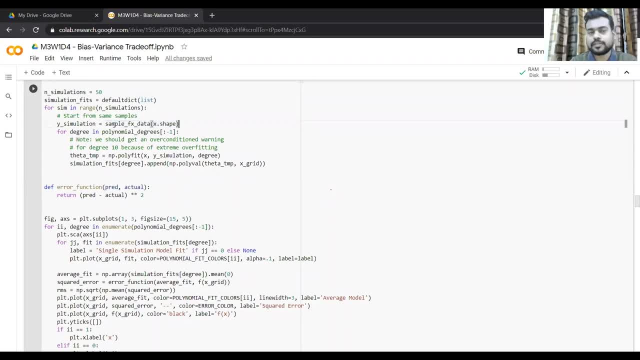 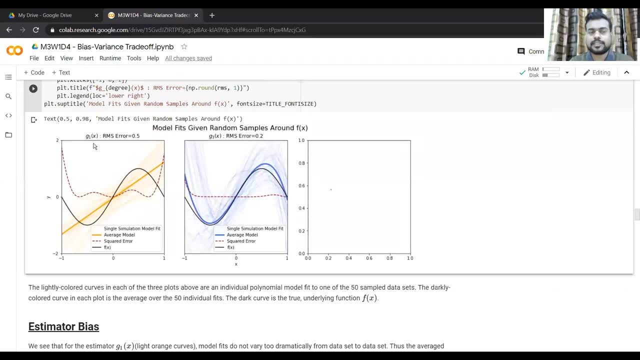 which will change whenever we are calling this function right. so this is how all the simulations uh for a single estimator, which is for this estimator g1x, looks like right. so these are 50 lines uh which we have gotten from uh fitting this g1 estimator for 50 data sets. so i hope this is. 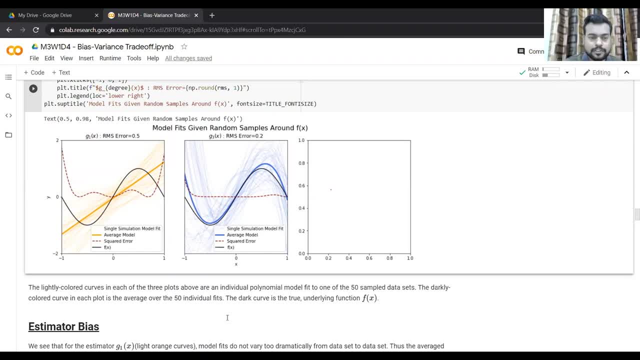 clear. uh, can you let me know if you are able to understand what each of these lines corresponds to? so can you tell me if that makes sense, or else i'll? i'll just repeat that. so i think yeah. so so each line is a single model for a given data set. right so, but because your data set is changing across each simulation, 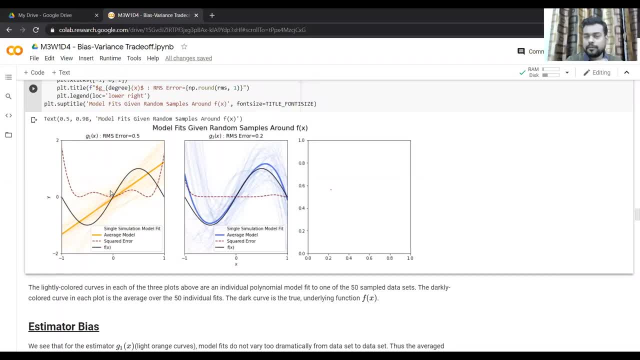 as in our y values are at least changing. x could have changed, but we have kept x fixed for all the data set. but our y values are changing. and all these uh, this light, uh orange colored lines, they are uh, 50 different fitted uh, g1, x's right. so, yeah, that makes sense. uh, for everyone. and now yeah, 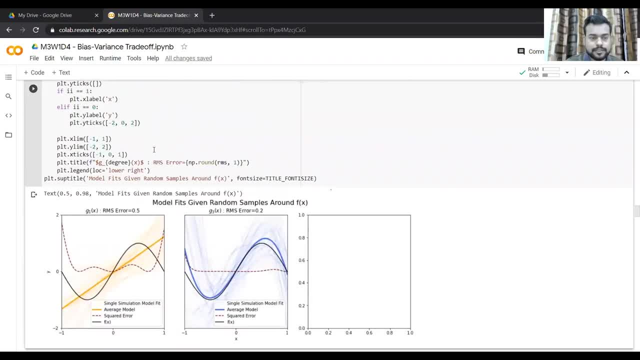 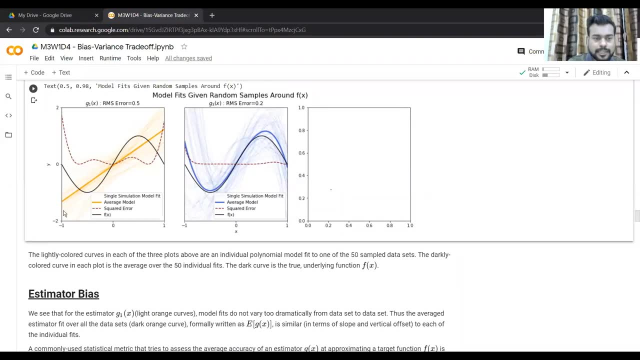 so now, what we are uh doing here? uh, so we also have something called the averaged model as in for each points, uh, where we're taking the average values right. so this is this, uh dark orange line. so this is giving us the averaged model as in for each set of, for each x. 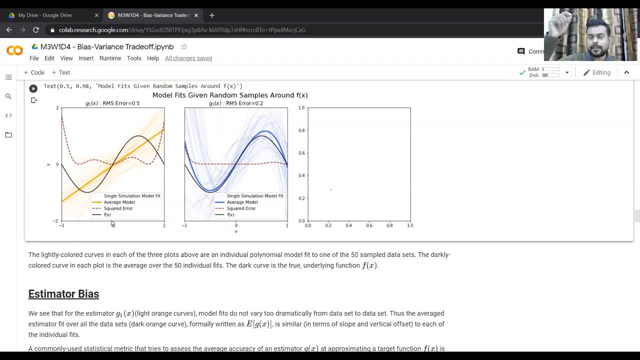 uh, i'll take the average of all those uh prediction of y's for all across all those 50 data sets, right? so let's see, let's think it in this way. so we have 50 different uh g1 x's, right, because we had different, 50 different data sets. so we have 50 different g1 x's and for each value. so all we'll. 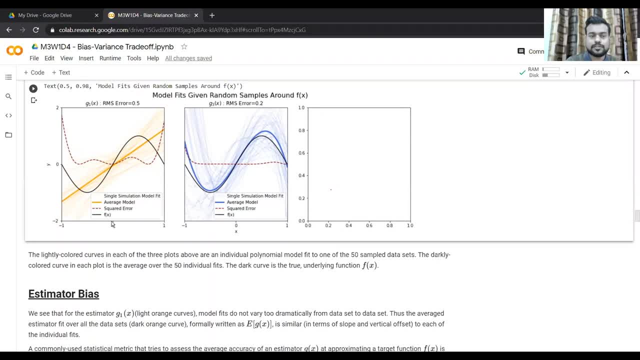 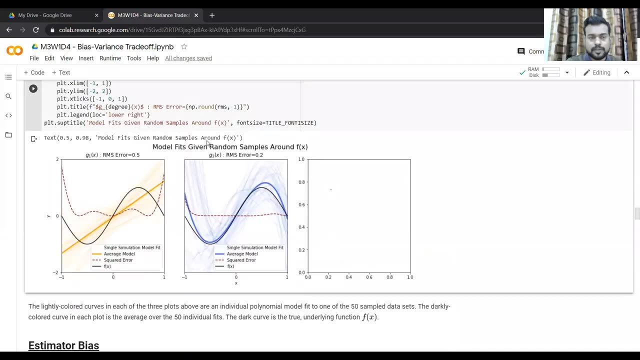 get 50 different values and if you take the average of that, so that will correspond to this dark orange line. okay, so this is just the average of all these lines. okay, so you understand what's the recipe for getting this averaged model. so i i can show you here. 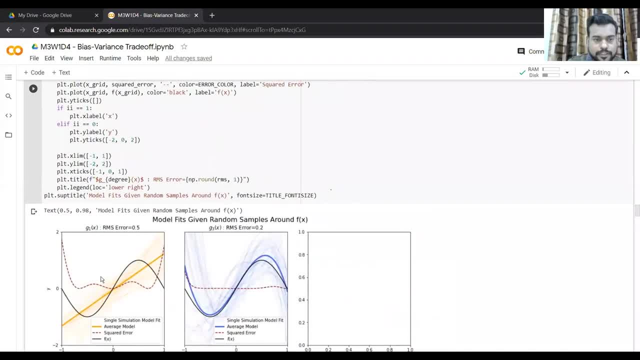 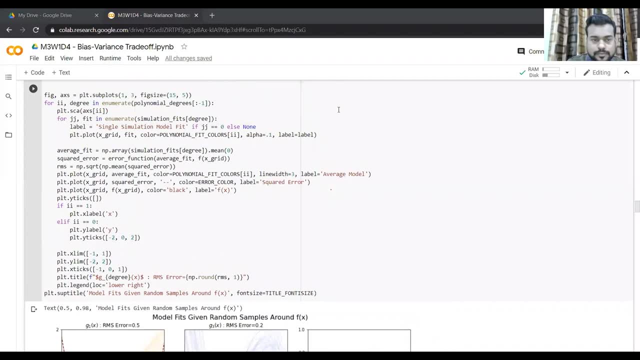 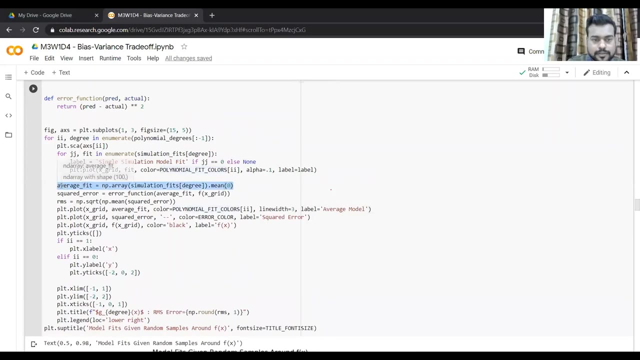 so where we are calculating this uh averaged model. okay, so, yeah, right, so this is how we are creating the average fit. okay, so this is how we are creating the uh, miss uh, creating the average fit. so how we are doing this. so we're taking the mean uh along the first axis. so we're taking the mean along the first axis. 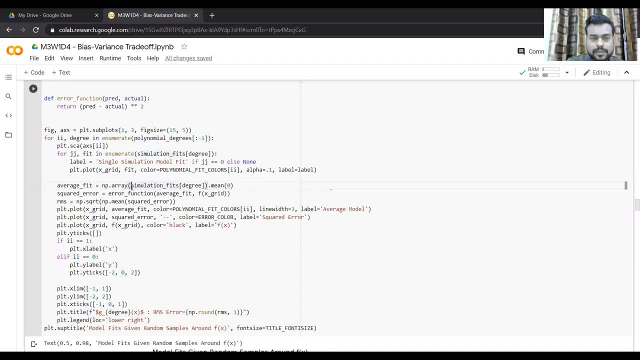 uh, right, and so so this is, uh, the y values. uh, across all those data sets, and we take the mean along, the x is zero, so this will give us the average fit, right, so, so, so you have, let's say so, let's say this is x. 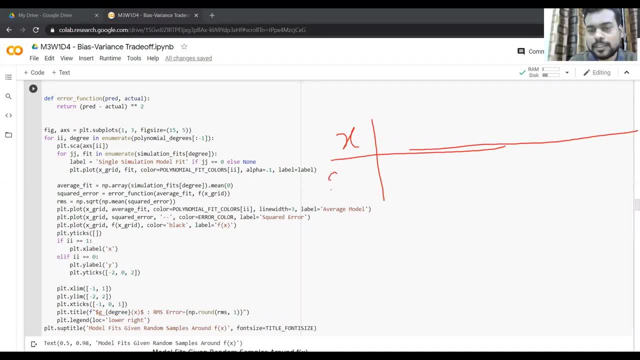 right, so yeah, so this is, let's say, uh, g1. let's say so, let's say this is g1. on the first data set: okay, uh, let's say this is your, uh, g2. for the second. i think i should do it. no, So let's say: I have X is here. Okay, so for the first simulation. so I get a function. 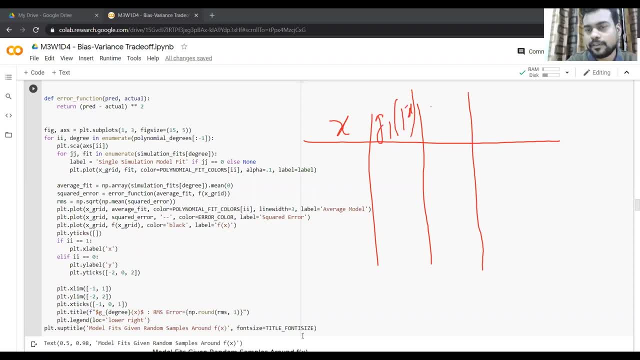 which is, let's say, I call this G1 first. then I get another function which is: I call G1 second, something like this, and I do this 50 times right. So for each value of X, so let's say it ranges from what one right. So they are a hundred values on which we are predicting. 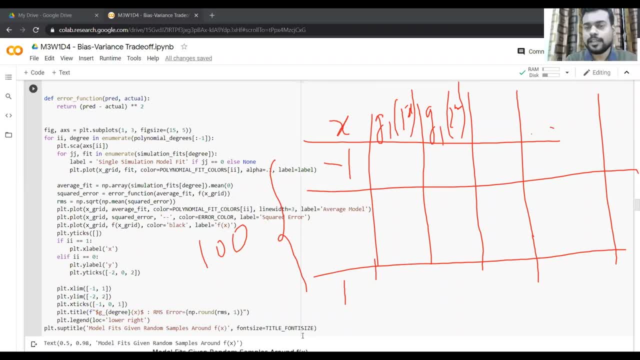 or predicting our fitted model. right, So G1 X will be something. So when I plug minus one here, so it will give me some value. So let's say that is 0.5, G2 will put some, G2 will give me some. let's say 0.6, right, So all these fitted models will give me some. 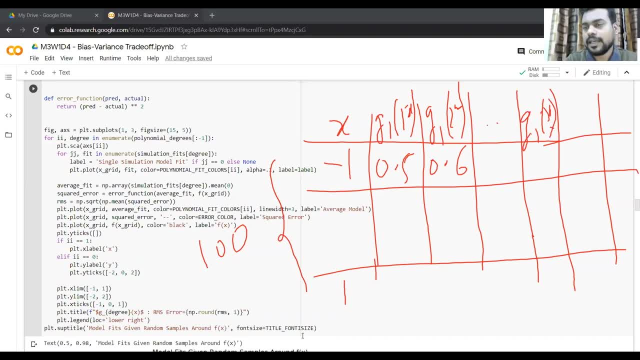 value right. So let's say this is G1 50.. And now this is, let's say, average across all these models. So for minus one I can get some value. average values. Let's say this could be 0.7.. So for all these X's, I get all. 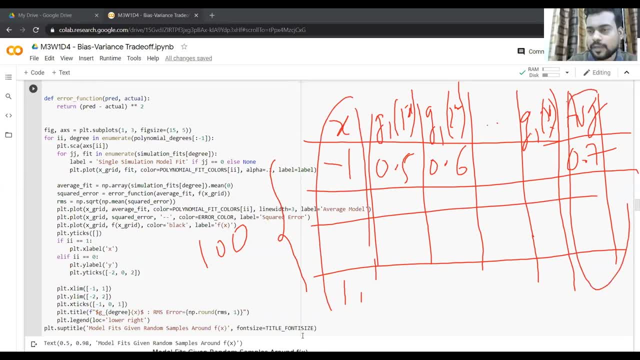 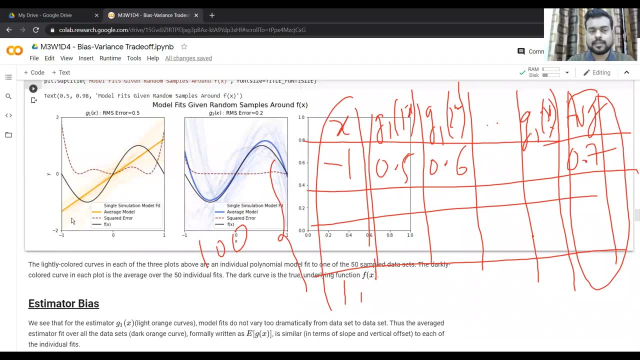 these average values. So if I plot this one and this one, so this is what our this dark colored orange, bold orange line looks like, right? So this is how we can get the bold orange. So you now know the recipe for miss creating all these individual light orange. 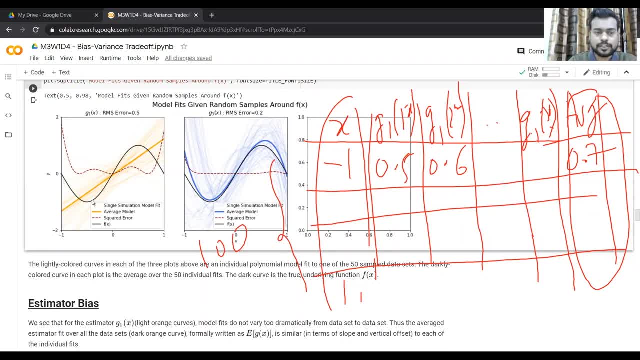 lines and the dark shaded line And, of course, this black line is your true function FX, which we want to approximate. So our first choice was this: G1 X. right now we can do the same set of experiment, but now with G3. right, So now just replace this with G3.. We'll do this. 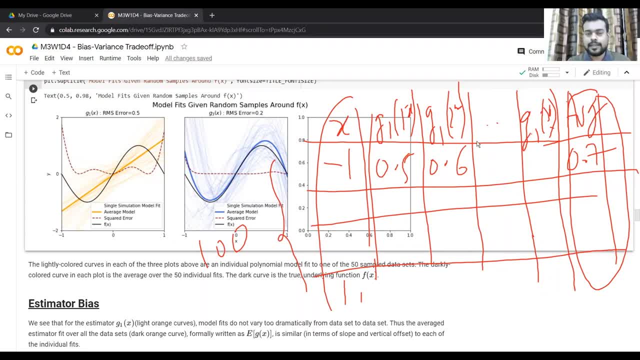 experiment 50 times for G3, right? And then yeah, so again we all these light blue colored lines. So these correspond to a single experiment, right? And this dark blue line corresponds to this particular average value of all these predictions of G3, for a particular value of. 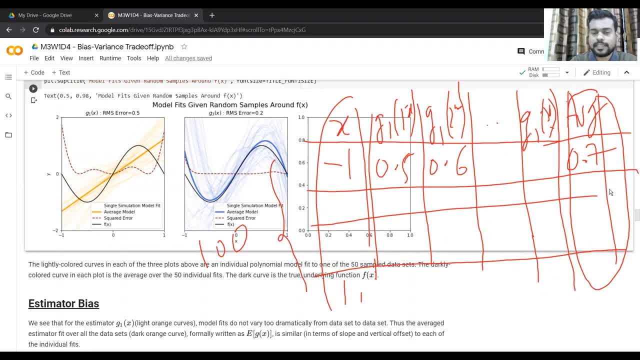 X, right, So the recipe is again the same. right Now we can see that Here this function, this average estimator, So let you can see that this particular estimator, So this particular estimator, I'm just talking about this one. So so let's say I focus on 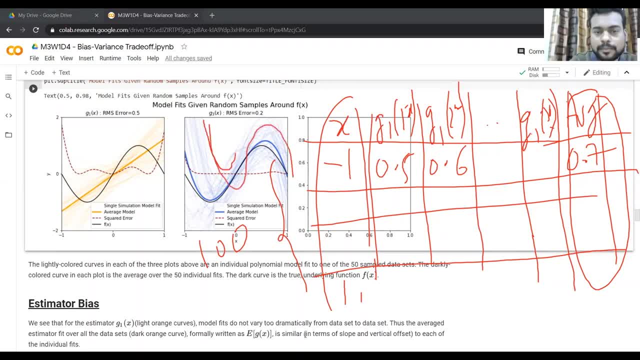 this some. so this particular parameter, this particular curve, right. So this is, this was one experiment which we have gotten from some simulation. This does not approximate this black line which we want to approximate, right, That's our objective, You remember. but if we do this simulation, 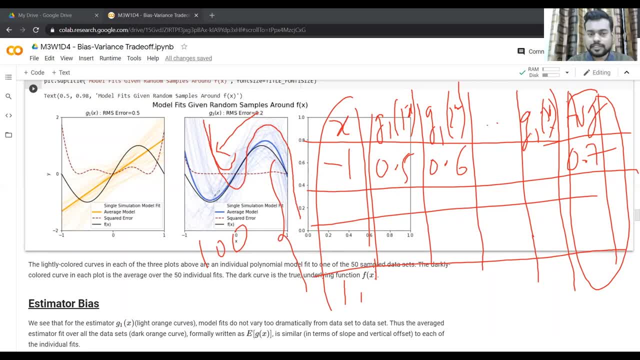 large number of times and average them. so you can see this average, this one, So you can see this clearly. So now you can see if we repeat this experiment 50 times. So this average model is very closely resembles to our true function right FX. So this is: 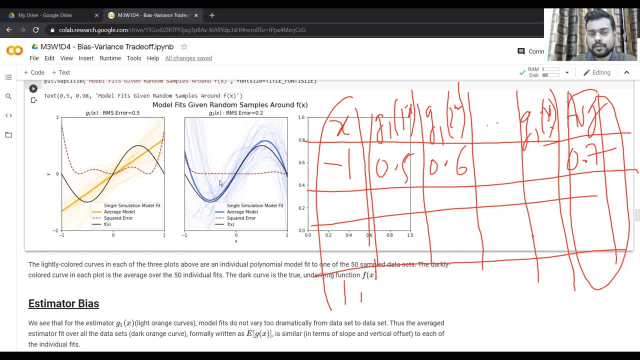 a good estimator of FX, right? So we can see that this looks like a good estimator of FX, right? So for a single simulation you might not have gotten, you would not. you might not have told that, Yeah, this looks like a good approximation to FX. But when we repeat, 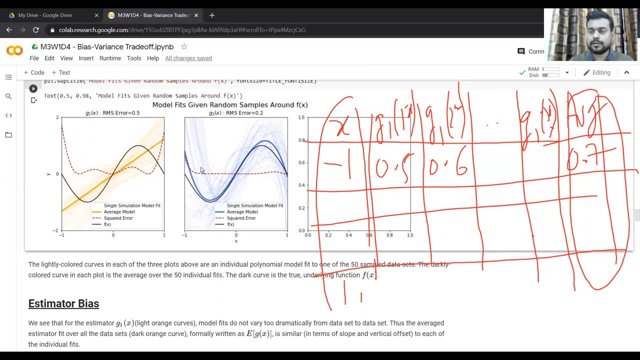 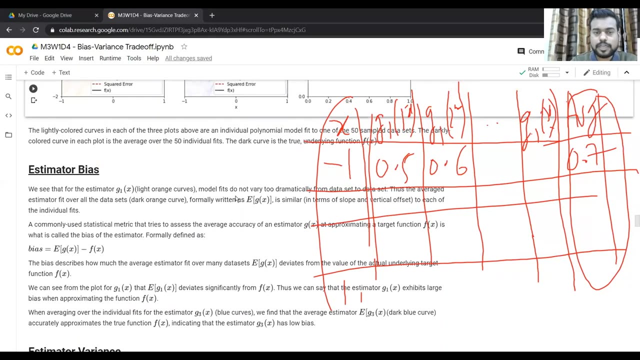 this and repeat this for a lot of different datasets and take the average model so we can say that, yeah, this looks like, yeah, good approximation to FX Right. So sorry, tell you. So this is what we refer to as E of expectation of GX right. 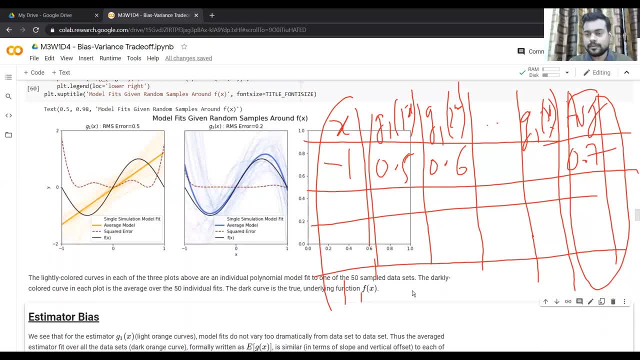 So we had different GX, right? Yeah, so they will see this. asking that we can create the data set here. What do we do with real data? So, in real data, of course, we'll see that we can create the dataset here. What do we do with real data? So, in real data, of course. 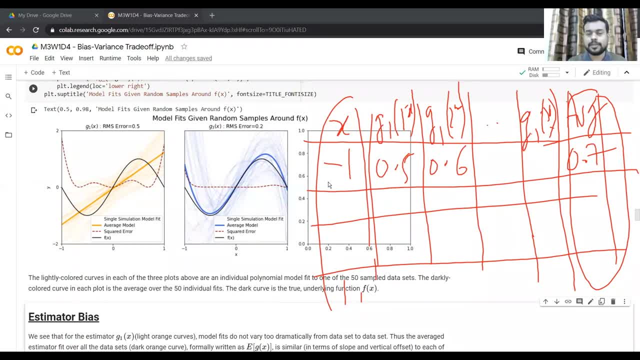 this is. I'll tell you what is the objective of carrying on this experiment. The objective is we want to understand the concept of wander, fitting in, overfitting, And once we know these concepts, so these are. this is actually a theory, and we are trying to understand this. 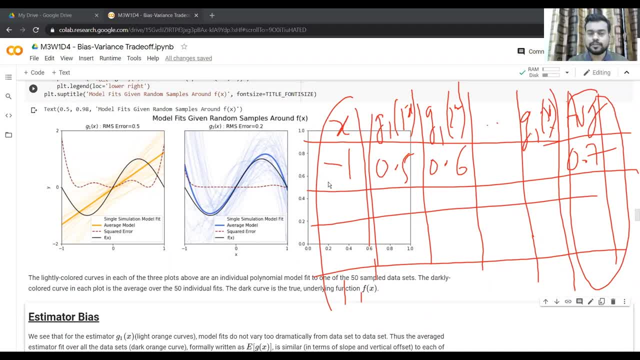 theory by doing some experiments Right, So by using some synthetic data. but when we actually do the machine learning, modeling on data, So by looking at the performance across tests At roundtable, and train will be able to ask you about that mins and get it to your back. 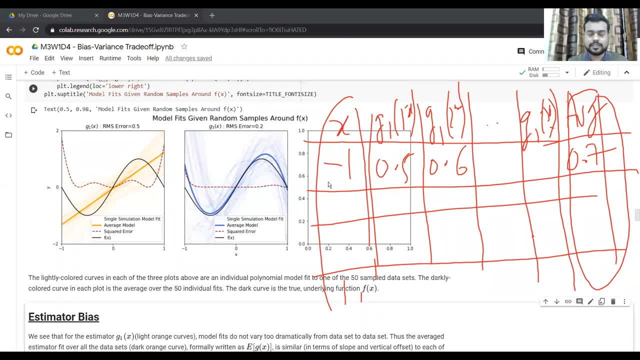 across tests and train will be able to explain to them to what? well, and then didnttalk. you say that, yeah, this model, seen this is underfitting or overfitting, right, So there, we don't have to repeat these experiments, But when we're training a particular model of a base for 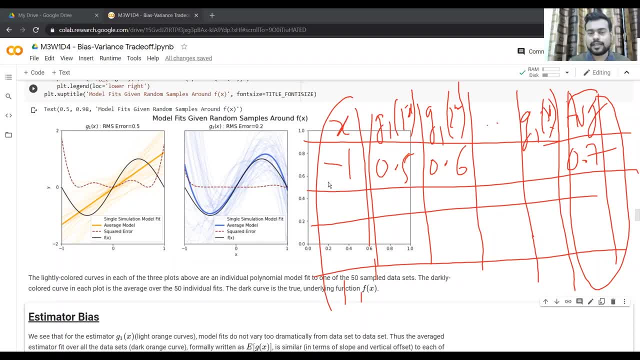 any chosen algorithm so we can say that. right, So this is to just understand the concept of underfitting and overfitting and the very important concept of bias and bias variance. right, So this is what I'm getting into it And yeah, so just bear with me for a while. 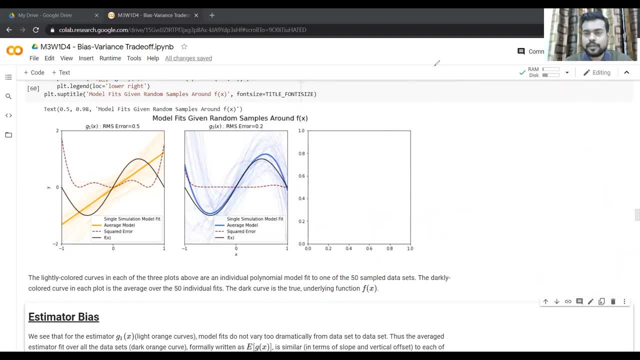 and these concepts will become clear. right So we're doing a lot of experiments now so that we just understand what is actually happening. right So we have a lot of theory which someone will, as it, tells you, and you will just accept that on face value, right? Yeah, So anyone. 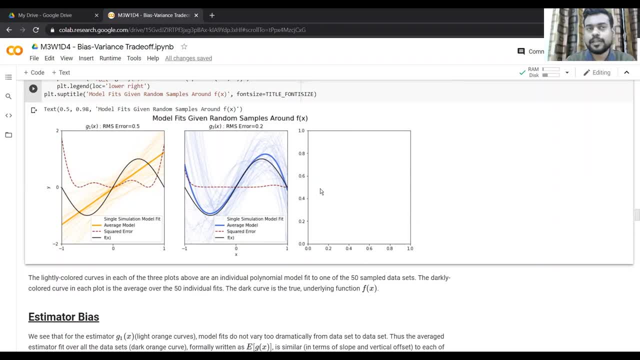 someone can come up and say that, yeah, simple model Underfit, but a complex model will overfit your data. So of course you can accept this statement, but here we want to- actually we're just trying- to validate that particular statement. 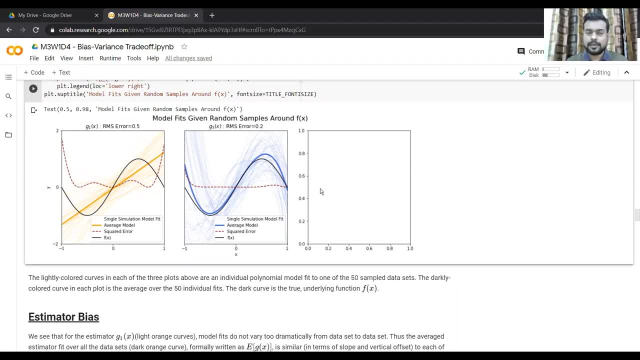 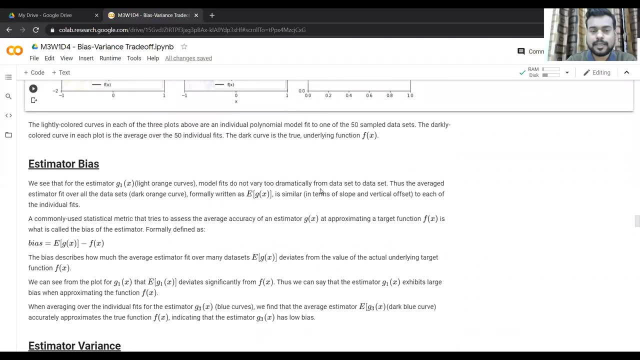 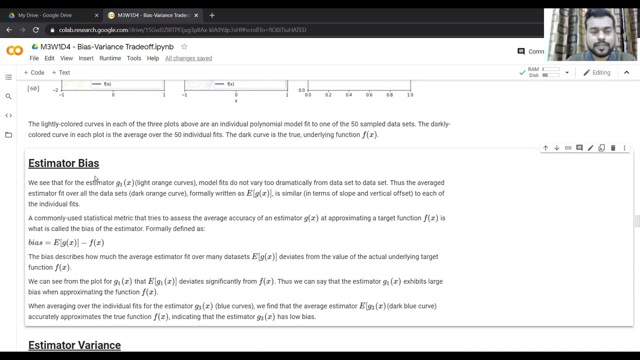 right. So that's why we're carrying out these experiments and using this, we'll be able to understand this concept of bias and variance. So I haven't yet come to the concept of bias, but, yeah, allow me to. Yeah, So now we want to introduce the concept of. 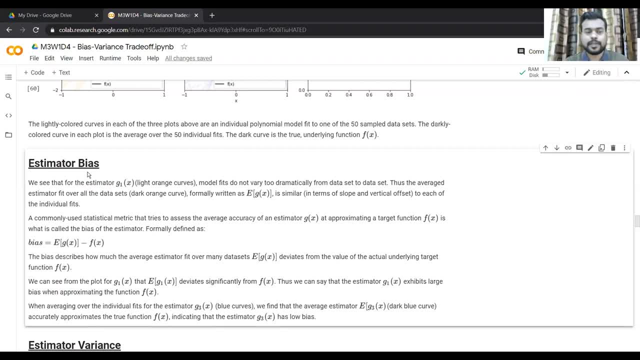 estimation Estimated bias right Or a bias of an estimator. So we saw that the estimated G, one X, which is your first degree polynomial, this model fits. do not vary dramatically from data set to data set right. So the average estimator fit over all the data sets written as this: 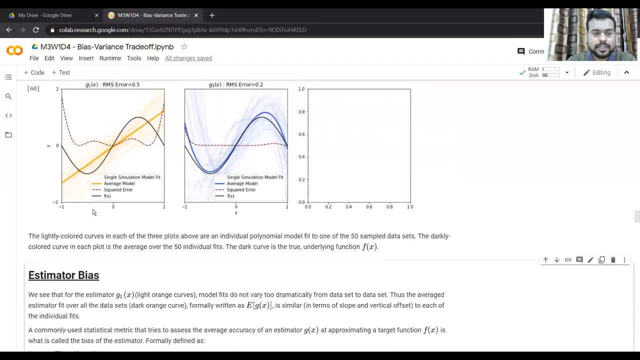 one is similar to each of the individual fit right. So these are the fits and this year this is your average fit, So you can say that more or less there They're not automatically varying from your data set to data set or simulation to simulation. 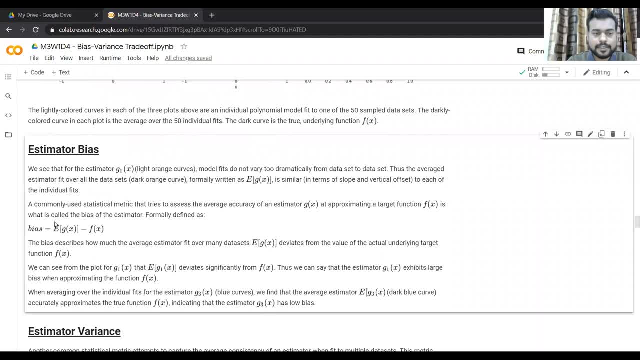 Right So right, a commonly used statistical metric that tries to assess the average accuracy of an estimator G X at approximating a target function. FX is what is called as the bias of the estimator. right So bias is formally defined as expectation of GX minus FX right. 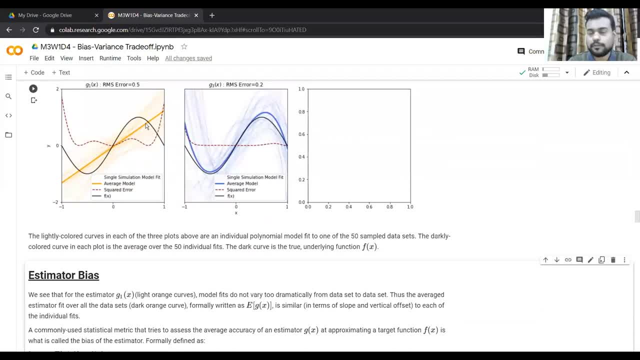 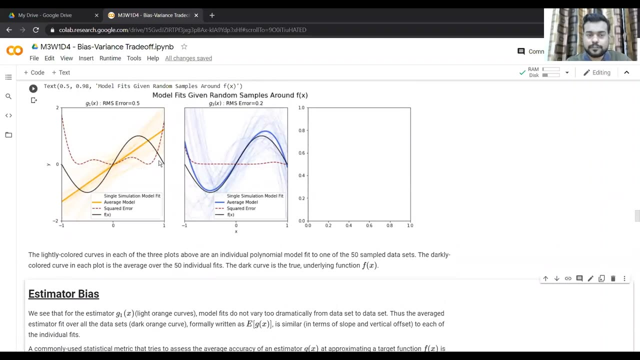 So, in this case, your expectation of GX for 50, right. So the expectation of GX for 50, 50 simulations was: is this one, this dark line, right Or the bold line, I should say right? And so the bias in this case will be the difference between your true function, which is FX, right. 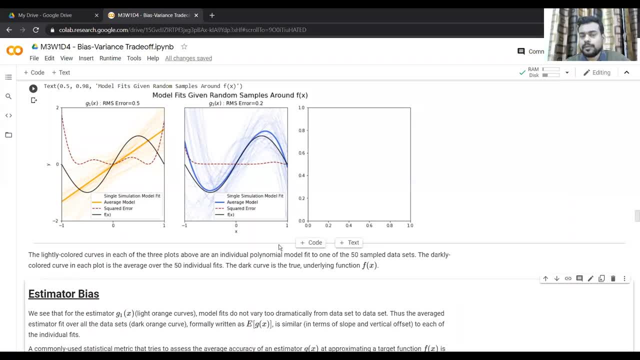 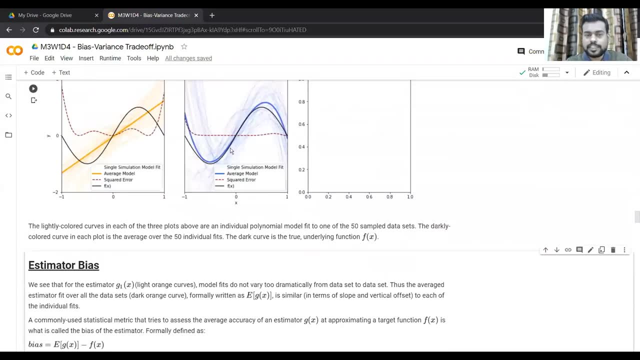 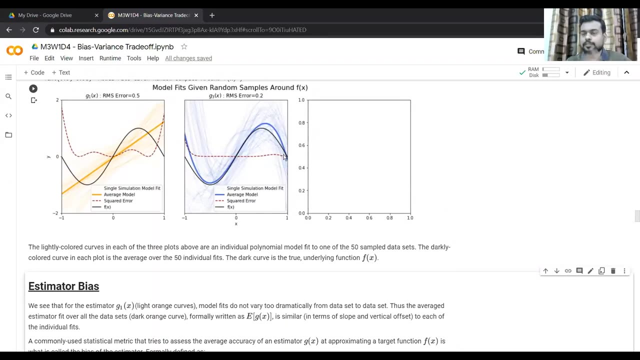 And this line, right. So the difference between this will be known, will be, which will call it as bias Again. so for this, G three X, right? So this is the expectation of G three X across all these rights. So, expectation of G three X. what is the meaning of that? 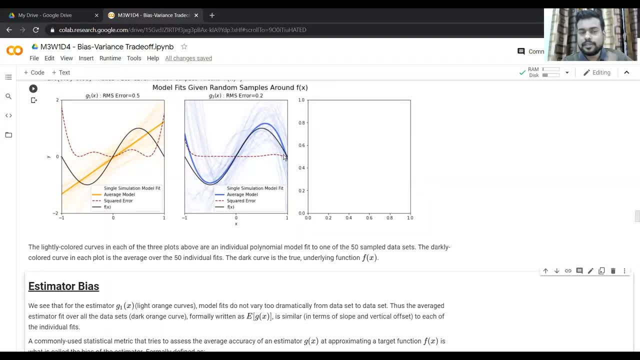 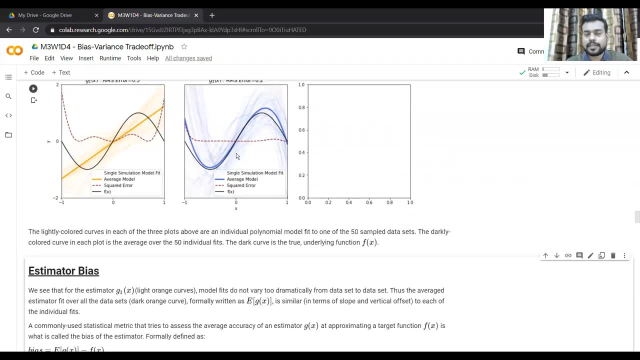 I just want you to know this. Tell me, do you already know this? but tell me what this means, right? So let's say I've done 50 simulations, So what would be the expectation of G, three, X? Right? So can you tell me privately? Right, So there was this. right, So there is a critical. 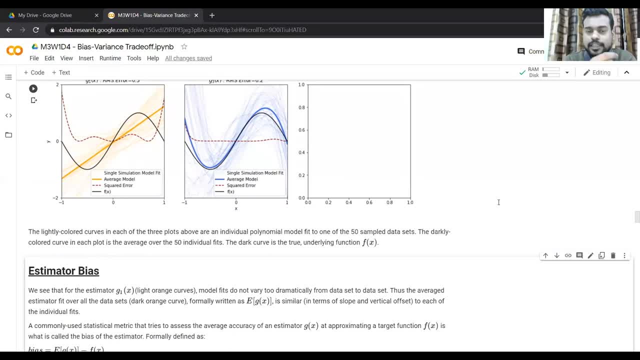 curve, which corresponds to a expectation of g3x right from here. So what is that line? So, yeah, so red is again right. So yeah, I just hire people, whatever you are. Yeah, So which one? Yeah, so that is the average model. Okay, Yeah, you're correct. So this: 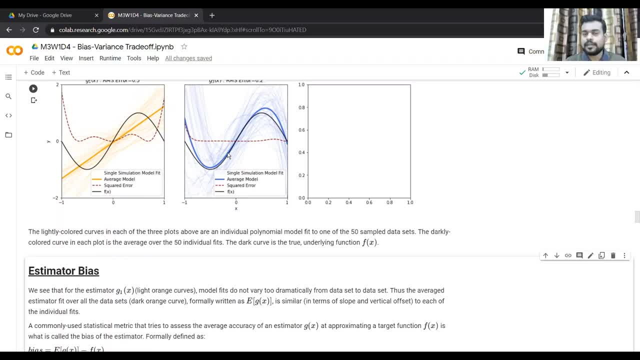 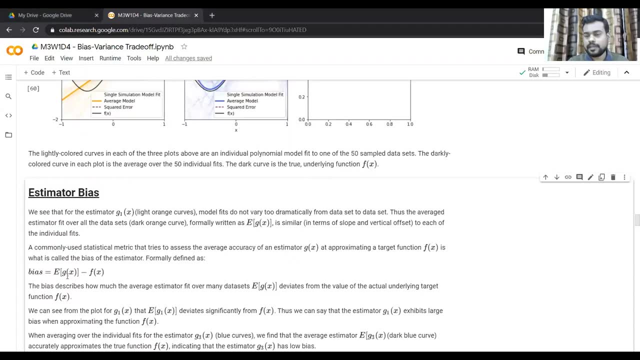 is the bold blue line which we are seeing, that we can call as the E of gx. right, Remember, expectation of gx is essentially the mean of g3x And because we have carried out this example, we have carried out 50 simulations, So E of g3x, for that will be the average model. 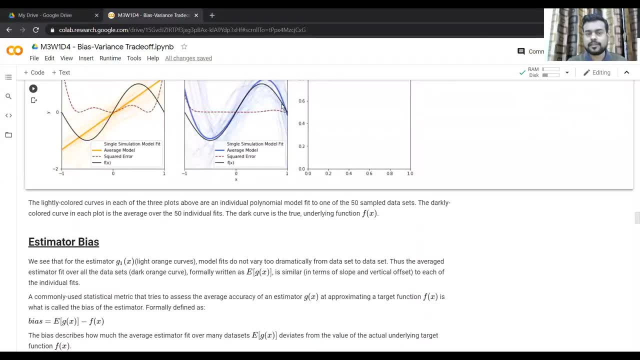 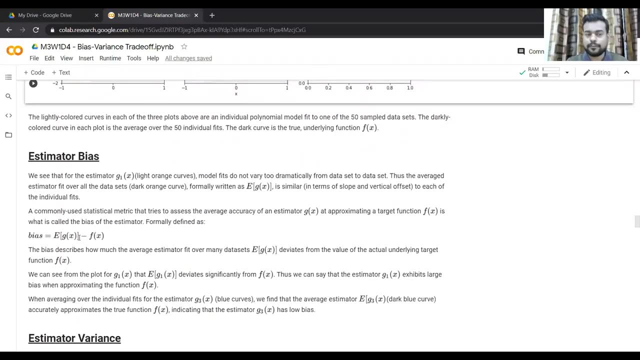 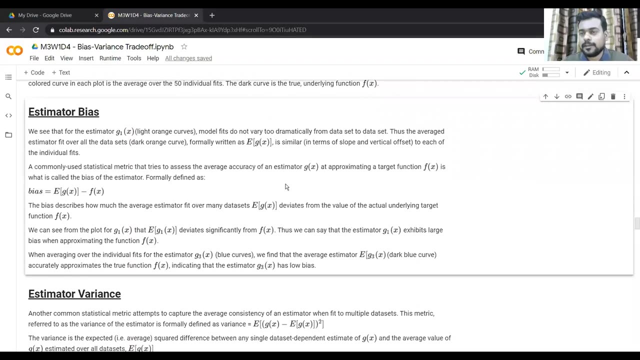 that is what we have here as this blue line, right? The solid blue line. Yeah, So bias is essentially the difference between your average model and your actual true function. Okay, So in reality, we don't know our true function, right? So that's why. 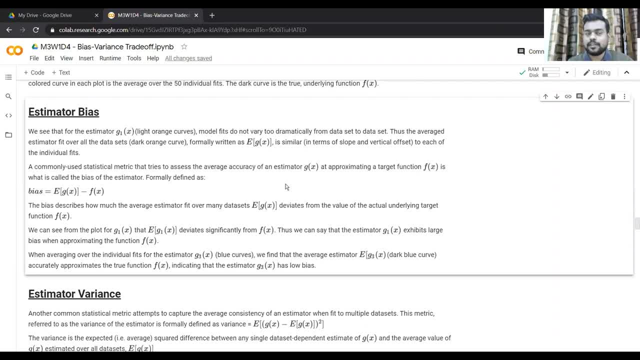 we are trying to do these experiments and understand the concept of bias and variance, right. So in when you are given a data set- x and y- you don't even know the true function, but you are, you're trying, So there is a. 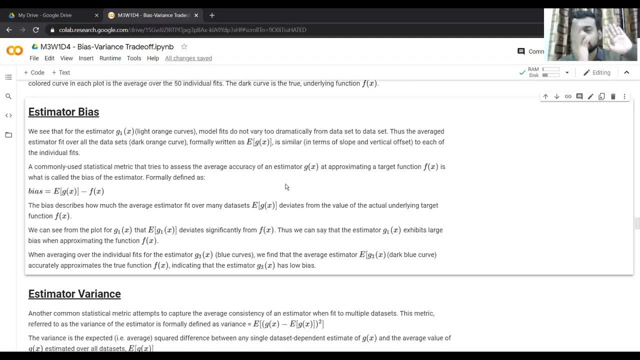 some true function which would define the relationship between x and y, But at best, what we can do with it without even knowing what that fx is. we can come up with some estimated gx which will closely approximate that fx. Okay, So, and that approximation? 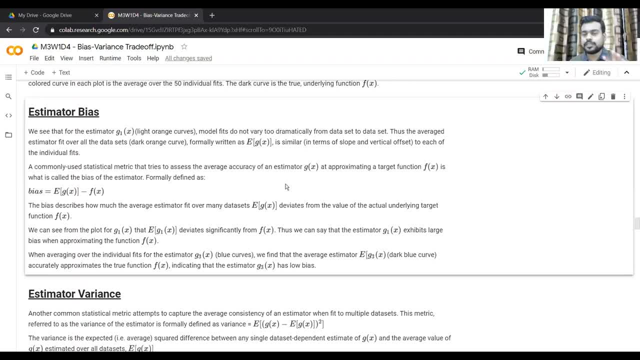 we will judge by looking at the model performance across train and across test. Okay, so this is how we'll do this. Okay, Yeah, So we can do that in real, with real data. So I hope your question gets answered, Right. 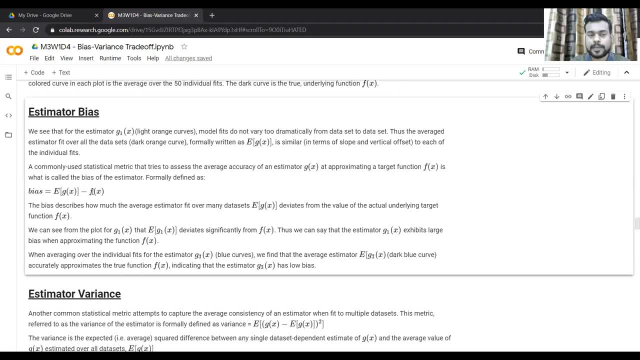 So here, of course, we're defining this with respect to some true function fx, But in when we're dealing with real data, we'll never know what that true f is right? So yeah, So yeah. so, even see, whatever we are observing in nature we are, we don't know how much we. 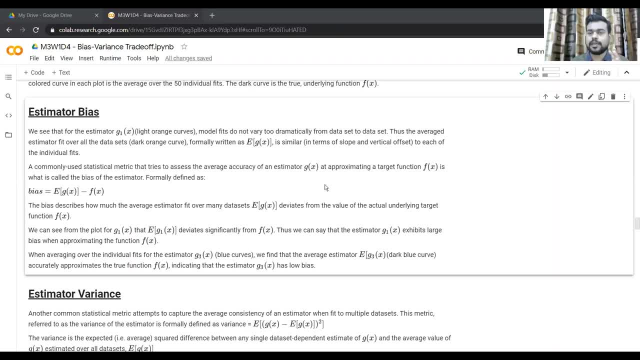 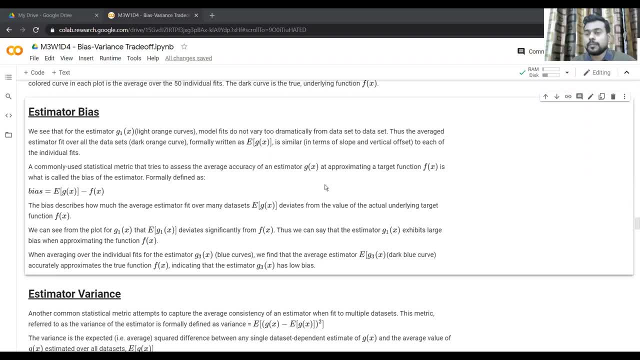 that Newton's laws of motion might not be the actual f right, It is only g right. So it is the best estimator that we have come up with, based on whatever experiments we have done, So that we're telling that, yeah, that is the best approximation we can come up with. 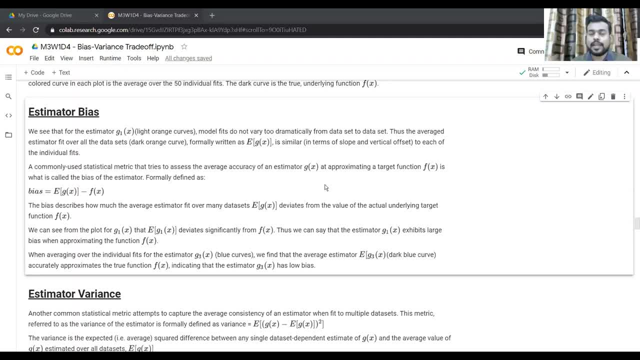 with approximating, when approximating fx right, But we actually we never know what f is right. So, even though it's called a law, but it's actually not a law right, It is just a model right. So in physics you have something called a standard model, which is very famous for. 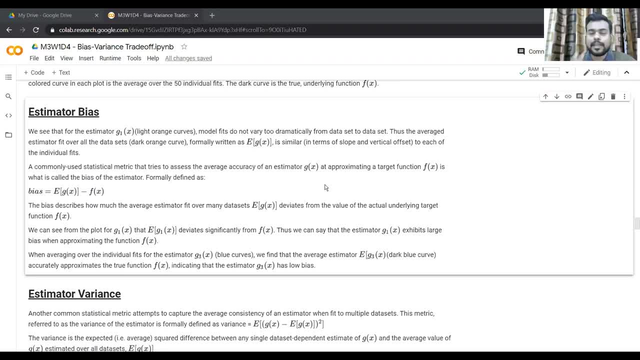 particle physics And that's also tries to govern all the behaviors we see around, all the particles we have in our universe, like electrons, protons, something like that. But again, a standard model, that is still a model right. That is not the true f right, That's. 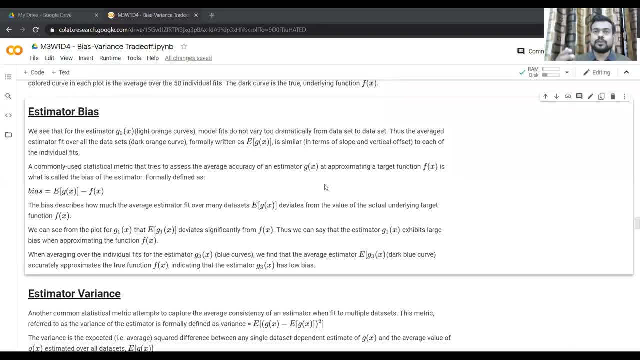 why the research is ongoing? because we want to actually come up with. we want to come up with the best approximation for our function f, which will describe whatever we are seeing in our environment, which we're seeing in our surroundings. So yeah, theory of everything. 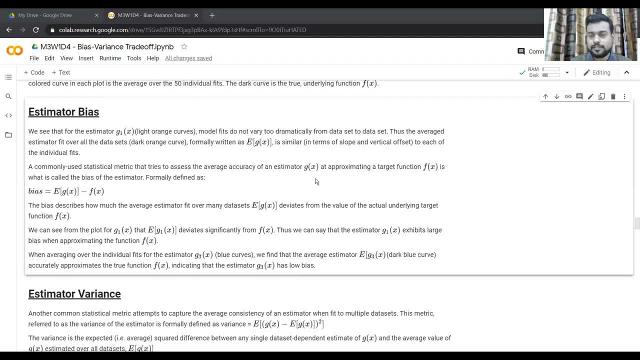 in fact, right, So, yeah, so see, as human beings at most, what we can do. we can conduct experiments and come up with an estimated g which will describe the relationship between the variables we have in our experiments. right, So this is how we define bias. It's the difference. 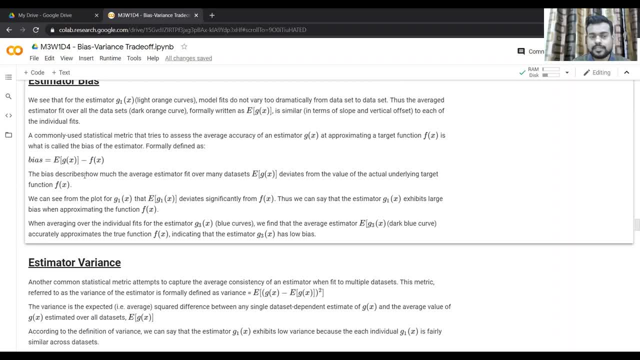 between the. this bias describes how much the average estimator fit, which is your expectation of gx deviates from the value of the actual underlying value, Right. So we can see from the plot for g1x that this deviates that expectation of g1x. 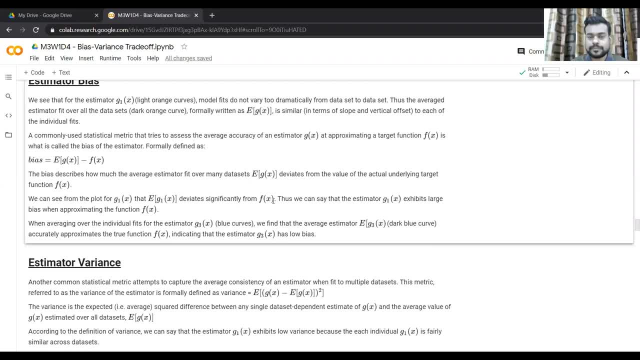 deviates significantly from fx right, And thus we can say that this estimator exhibits large value bias when approximating this function. fx Isha is asking a question. This is the bias we studied in inferential statistics, So so there also what we are trying to look. 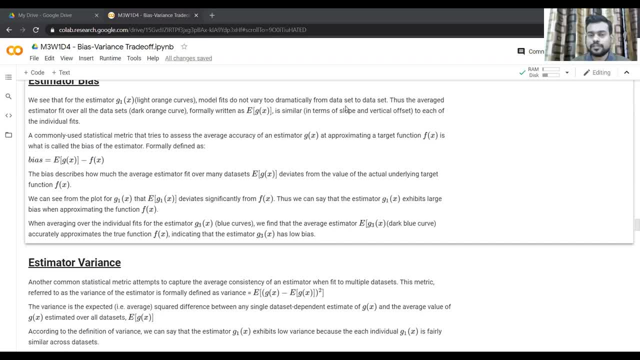 at here is that we are trying to come up with the best estimate for a parameter right. So let's say, if theta were a two parameter right, So we are trying to come up with right this one, So something like this. So this was known as the bias right. So this is theta. 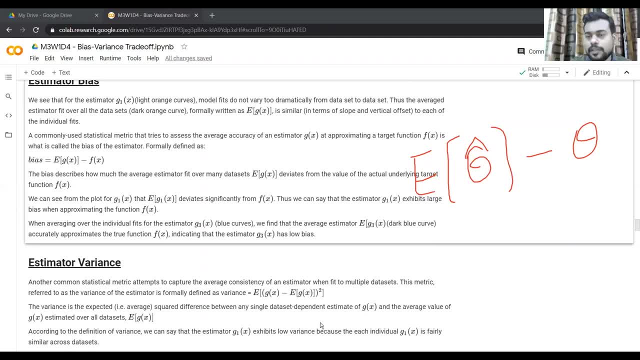 hat, right? So this is what we wanted to come up with. In fact, we can call this as g of theta, theta hat or something, or maybe I'll just restrict to theta hat. Okay, So this is what we are referring to as bias of an estimator. So there, the estimator was theta. 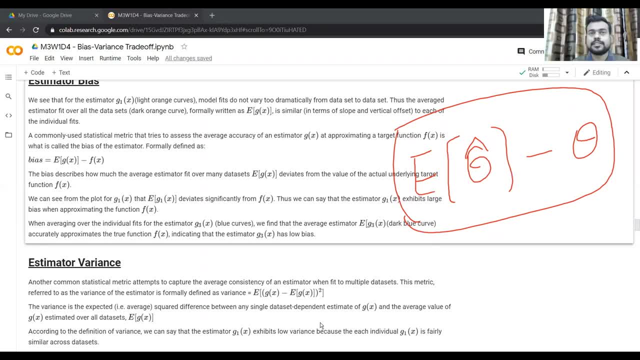 a single parameter. So there we are standing. let's say a particular distribution, binomial distribution, So it had two parameters, And so let's say: theta, is your proportion there, right? So when we discuss bias in inferential statistics, we were looking at the bias of 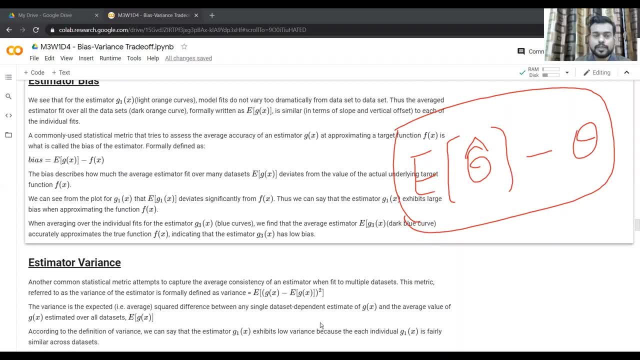 a parameter of a distribution. Okay, Here also we are using the same formula, but here, instead of theta, we are. we want to come up with an estimator of a function, right? So we want to come up with an estimator function rather than an estimator parameter, right? 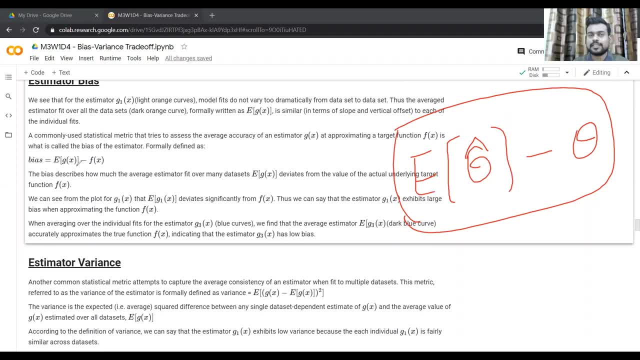 So, of course, estimator function in this case is a set of model parameters, right So? but I hope you realize the difference between these two, right? So of course the bias formula is the same, but earlier we were that we'll call it a set of model parameters, right So? 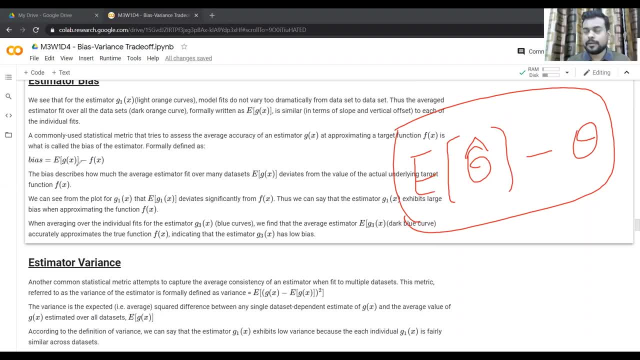 this is what we'll call as the bias of an estimator: bias of the estimator for parameter theta, And here what we'll call as bias of the estimator function g. right, So I hope that difference is clear. Yeah, that makes sense. Okay, So this is what we'll call as: 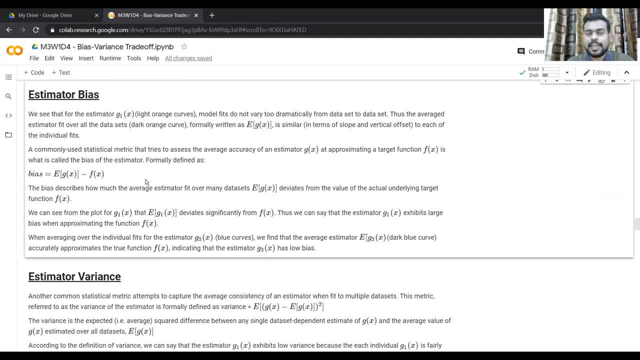 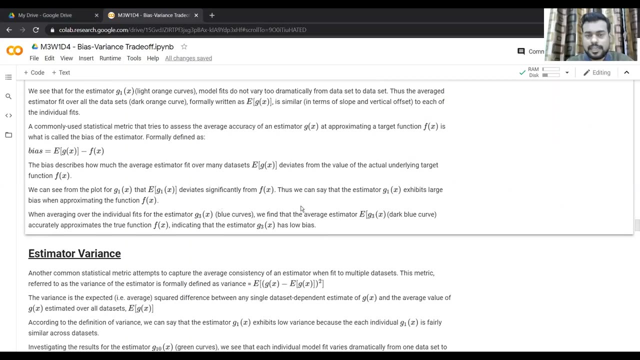 bias, as in this bias tells us how the average estimator fit, deviates from the value of the actual underlying target function, which is effect, which is what we want to approximate. right, So we can. we saw that g1x exhibits large bias as it deviates, deviates a lot from. 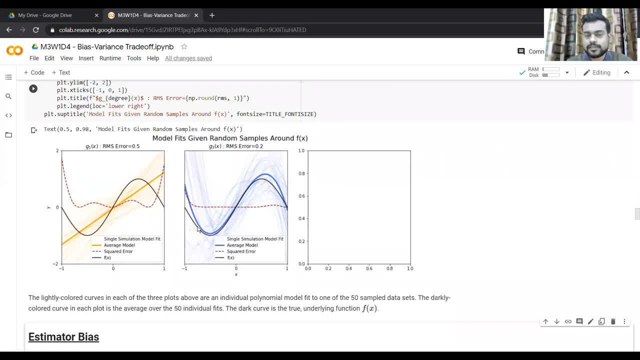 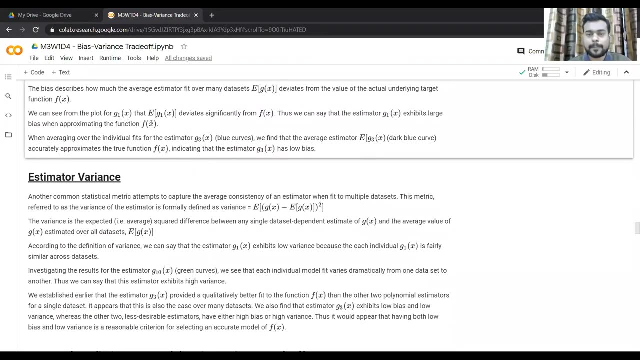 the actual true function. but g3x has low bias. Okay, As in, it is closely resembles. as in, the deviations are very small between the average fit and your true underlying function, Right? So g1x will say that it exhibits large bias and g3x will call that it exhibits low. 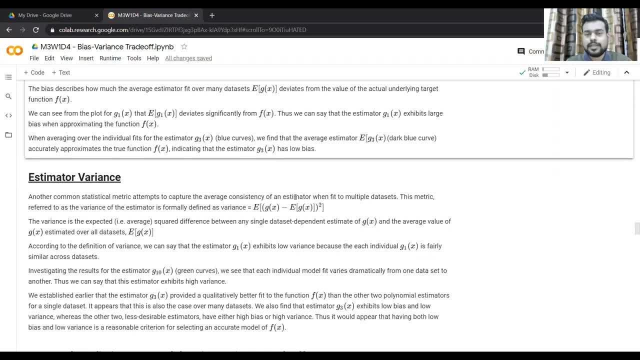 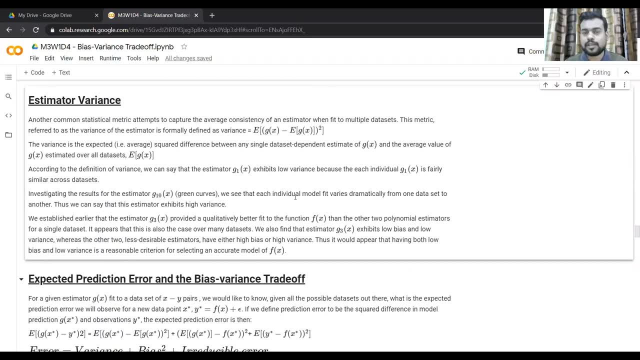 bias. Okay, So a simple way. or you can say that because g1x was a simple model, so simple model will have large bias and let's say, a relatively complex model will have low bias. Okay, So we'll get to this as in how the bias will be. 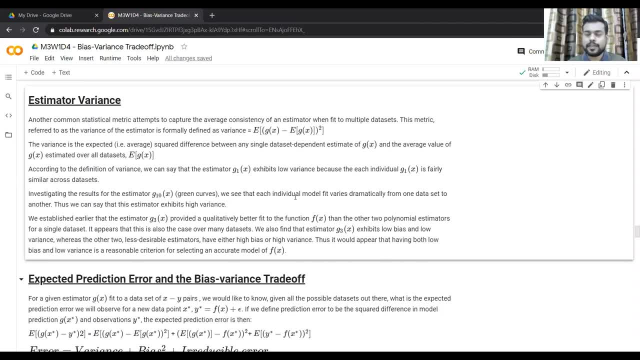 So what bias looks like if you vary the model complexity, as in we vary from, let's say, polynomial degree one to, let's say, polynomial degree 10.. So how the bias will look like. So we'll come to that, So we have done that experiment and we'll be discussing that. Then there is 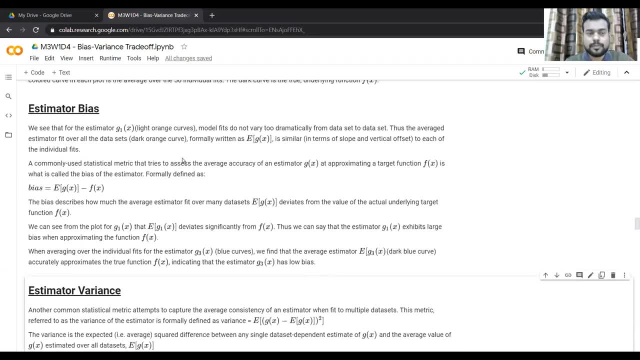 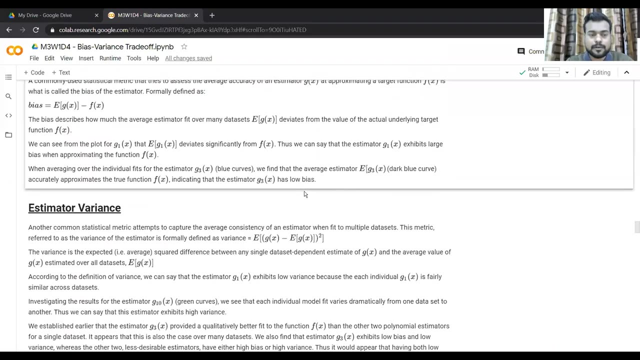 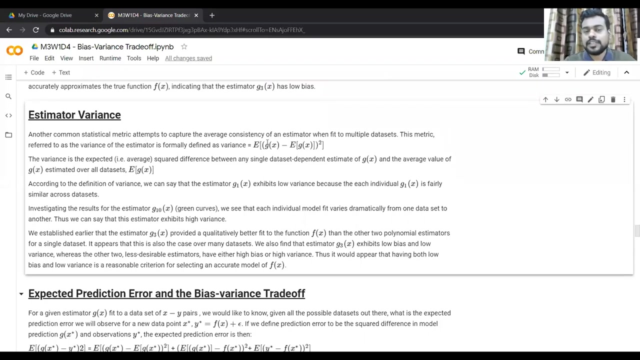 another estimator variance. Okay, So remember so: in statistics, your estimator was the estimator of parameter theta. here The estimated term is- this is meant to Describe the estimator function- gx. Okay, So now what is estimator variance? So another common statistical metric attempts to capture the average consistency of an estimator when. 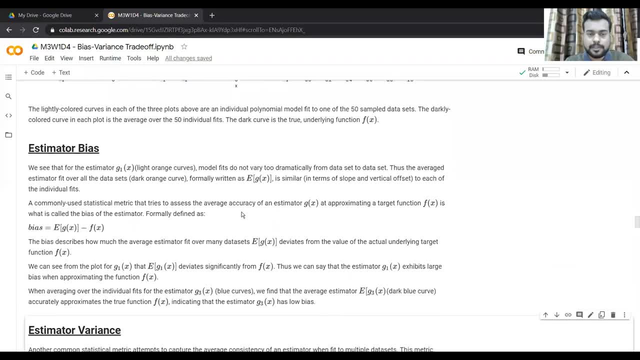 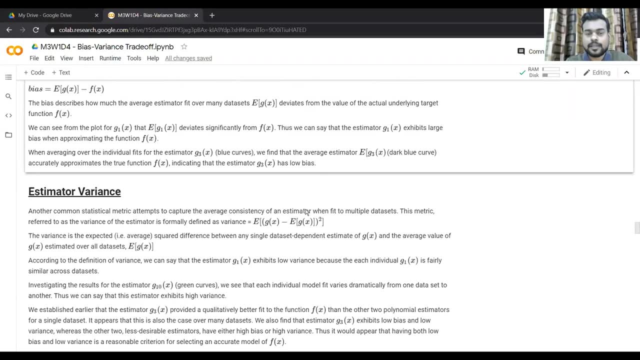 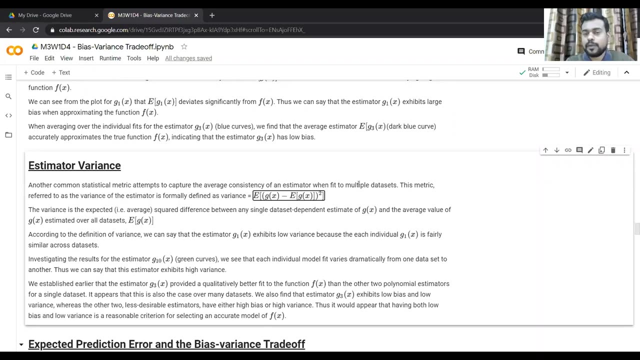 fit to multiple data sets. So remember the in bias, we wanted to assess the average accuracy of an estimator at approximating a target function. But here, in variance, we want to capture, capture the average consistency of an estimator, The average consistency of an estimator when fit to multiple data sets. So here now we. 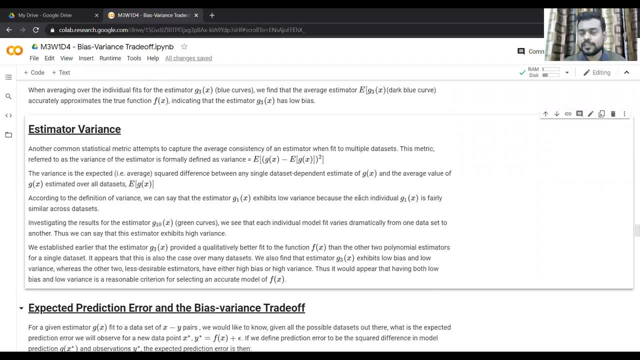 are not concerned with the actual, true function, but we want to see how the estimators look across all these 50 simulations. right, So this is how the variance is defined. right, So you remember how variance is defined. So when we when X was a random variable, right? 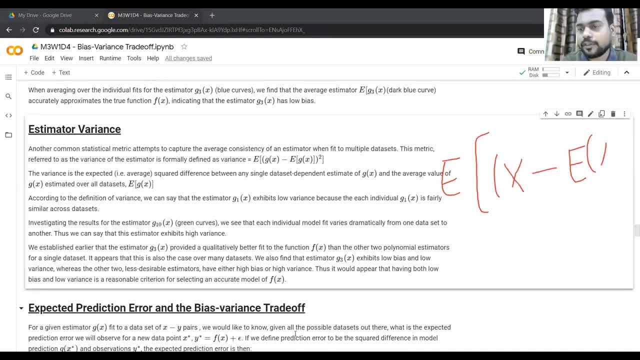 So we had X, expectation of X, So we use the square this and This was the variance, right? So this was the variance We had studied in statistics. This is the same variance, but instead of X will have gx, right? So so what this tells? 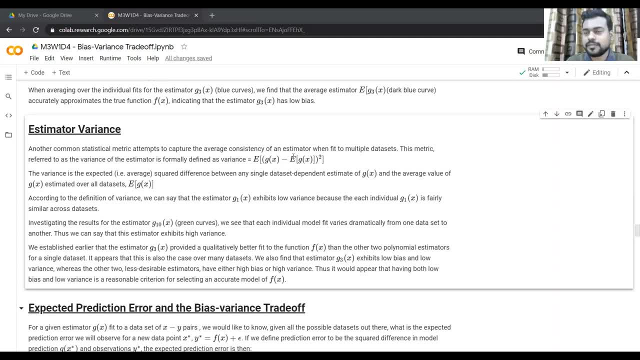 you. Can you tell me what this tells you? So, so, in the in the square, within the square brackets, so ignore this square term. Just tell me: So this is gx minus expectation Of gx, and then we are squaring this term and then taking the expectation for that. 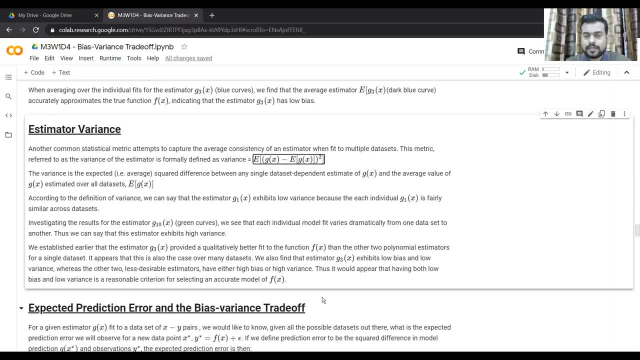 So what does this tell you? Yeah, so this is pretty bang on on this. I want to get answer from other people. So it's a straightforward concept. It's the same concept of variance. What does variance tells you? Right? So it tells you how it varies, about the mean. 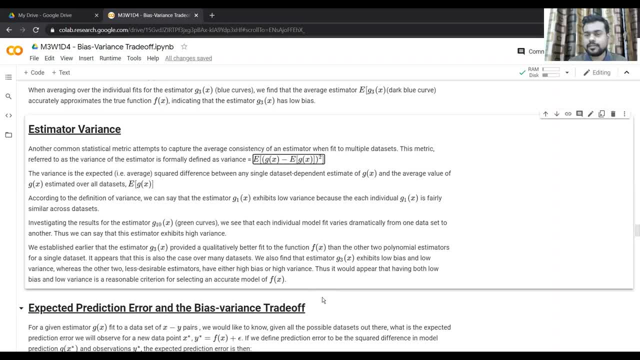 Right, So it tells how the values are, we are spread, or varies around, mean Right, So Yeah, exactly How much it varies from average model, right, So how much it so is saying that, how much it varies from average model. 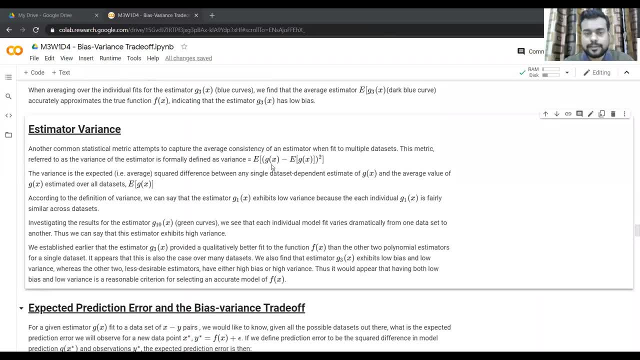 So what does it mean? So see, So we have done 50 simulations, So I'll just write this here. So we have done 50 simulations, right? So each simulation had a different data set, So we had done 50 simulation. 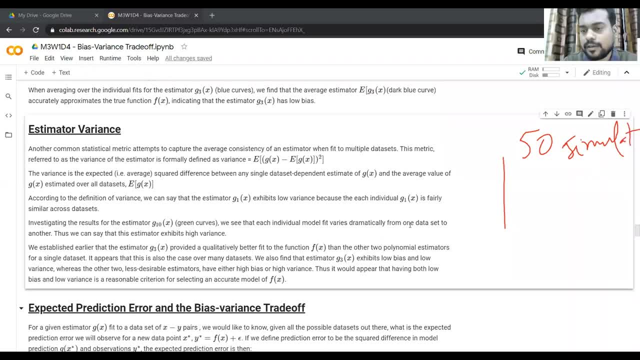 Okay, so So for all these simulations we are getting some g of x, right? So we are getting some g of x for all these simulations. So I can call this one, two, and then I'll have some g of x. 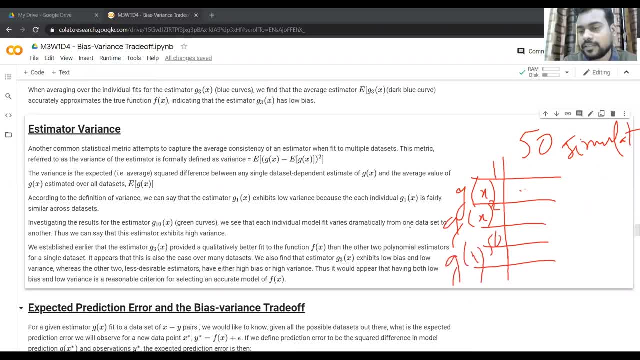 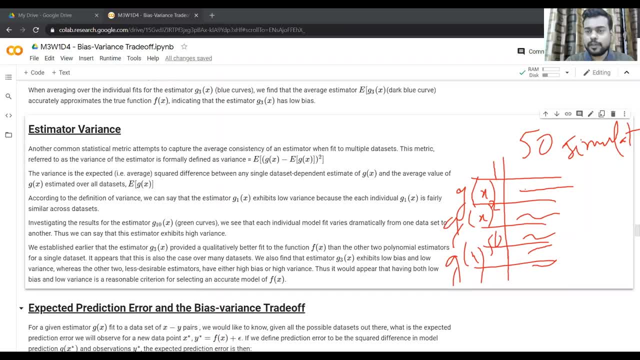 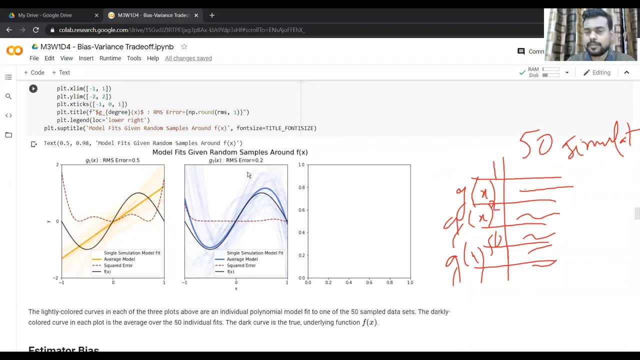 Right. So if we go back and look at our plot, So in this case, so all these light colored lines are individual estimators, like these ones, And then we have the average estimator, which is the expectation of g of x. So, in this case, expectation of g of x, Right. 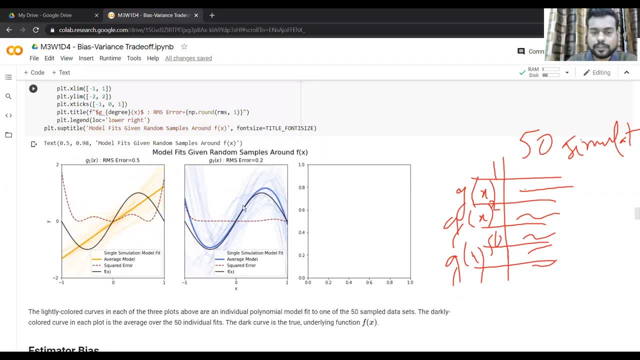 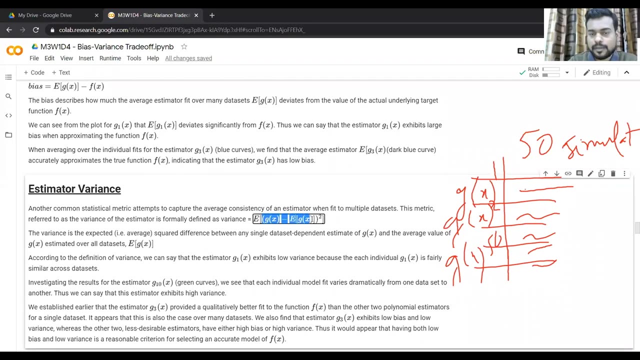 So how these are sort of spread around the average fit, Right. So if we find the expectation of g, of x, Right, So we have the expectation of all those 50 values, Right, So we'll have 50 such values. And if you take the expectation of that, so it is just, this video is telling you how consistent your estimated is, or how consistent your estimator is. 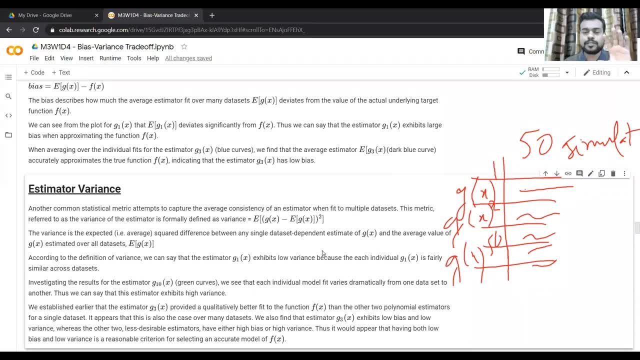 Exactly Right. So you, we have an average fit Right. And we want to look at each Right So, at each estimator, and see what's the deviation from the average fit Right. So if the deviation is small, for all those fits. 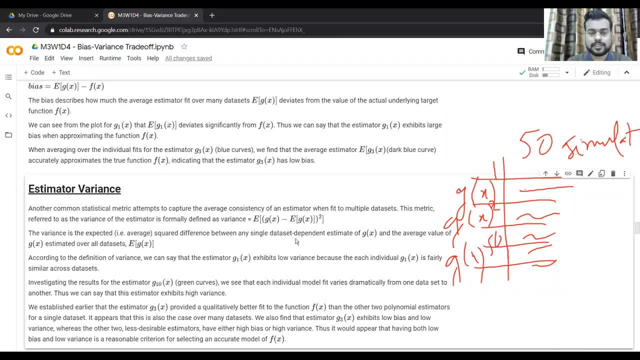 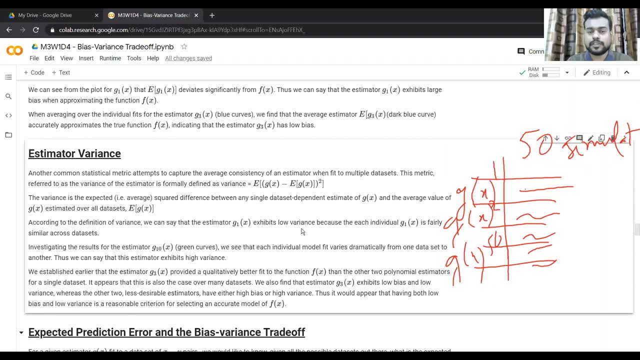 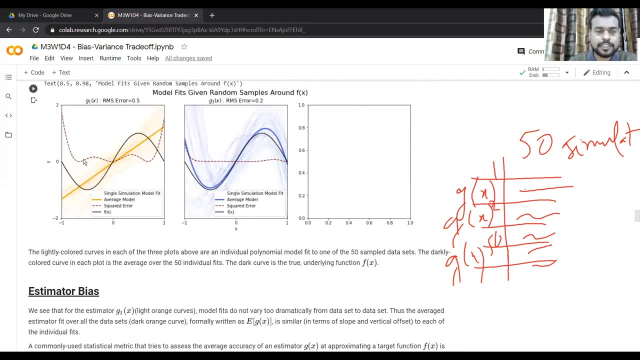 So we'll say that it looks more or less consistent, Right? So this is what is captured by variance. Okay, So you already, you're already familiar with the concept variance. It's the same thing here, Right? So we can see that g of x is sort of. it does not. it does not exhibit large variance. 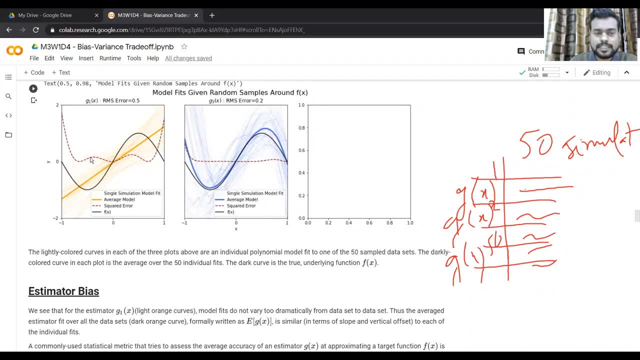 Right. It has a small variance, as in: these lines are sort of closely packed together, Or you can say that these are closely spread around your average fit, Right, But for this one this is more spread, Right, So we have more variance actually in this case. g3x. 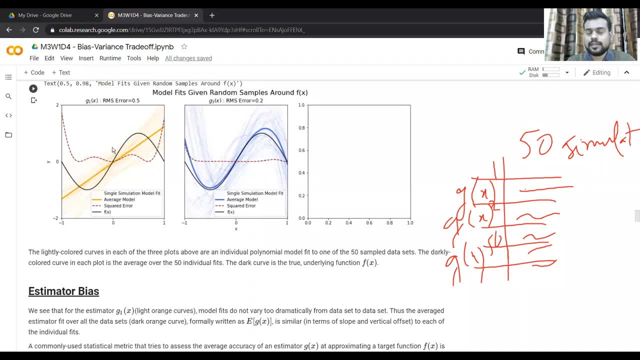 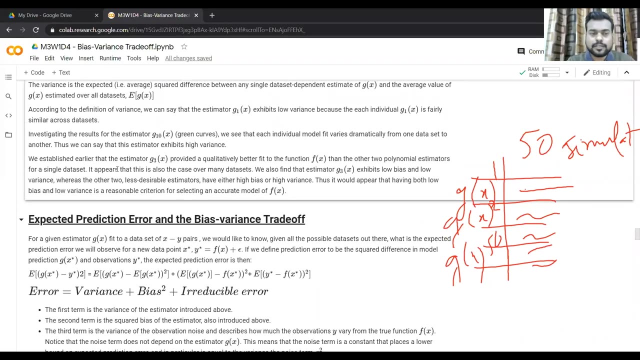 But in g1x we have a small deviation Right- Small- So this is what we call a small variance here. But here we have relatively larger variance, Right. So this is so we established earlier Right That the estimated g3x provided a qualitatively better fit to the function fx than the other. 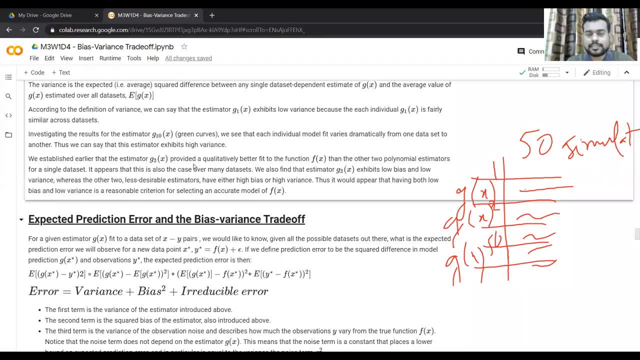 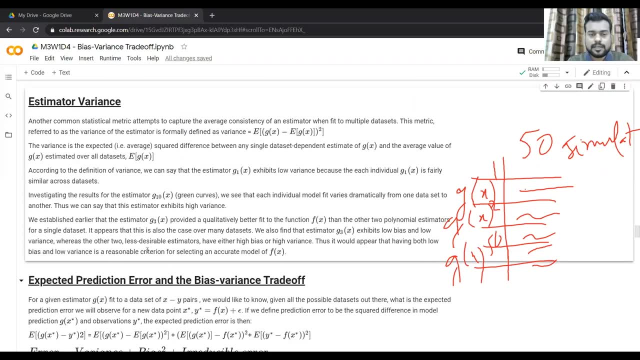 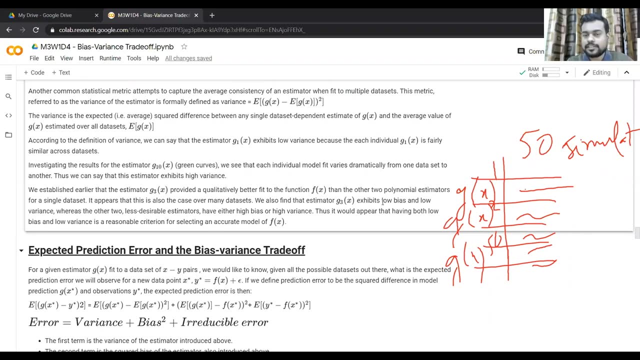 two polynomial estimators for a single data set- Right, So g3x. we saw that it provides a better fit out of these two Right, But it appears that this is also the case over many data sets. We also find that estimated g3x exhibits low bias and low variance. 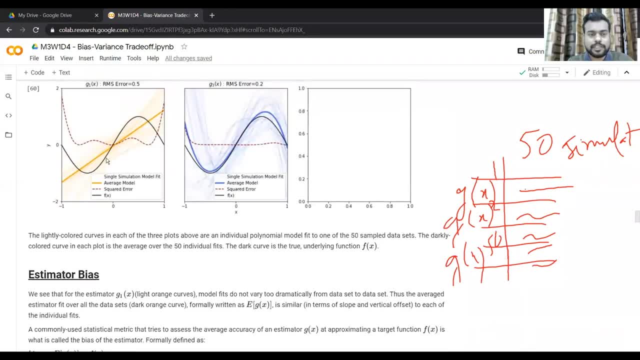 Whereas the estimated g1x. so it has high bias but it has low variance here. So here also the variance is not that large, but I think it's relatively larger than in this case. But this particular estimator it has low bias And low variance. 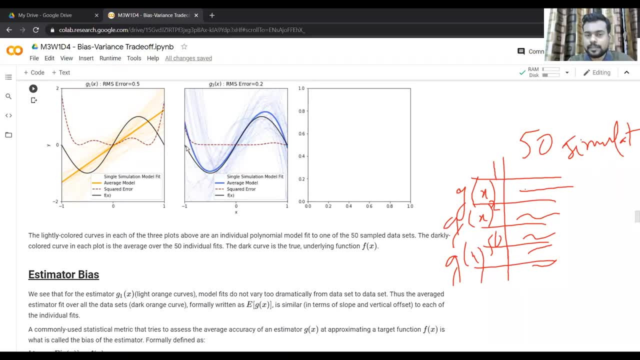 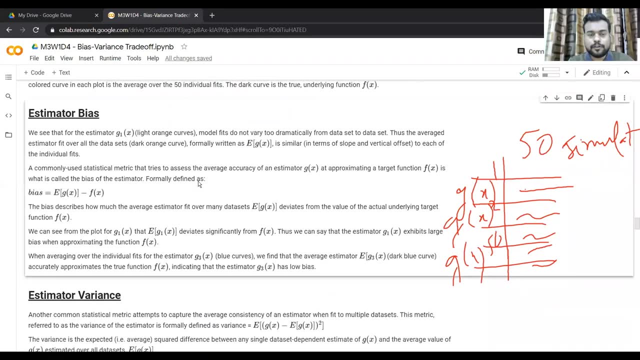 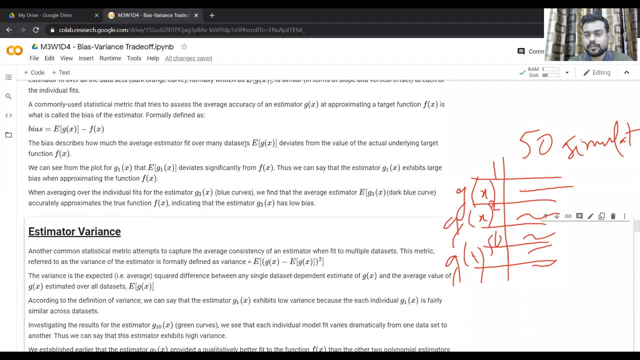 Why low bias? As in it is very closely resembling the black curve here, Right? So this is what the definition of bias is, And then and for variance is sort of how we want to look at the average consistency of each estimator across multiple data sets. 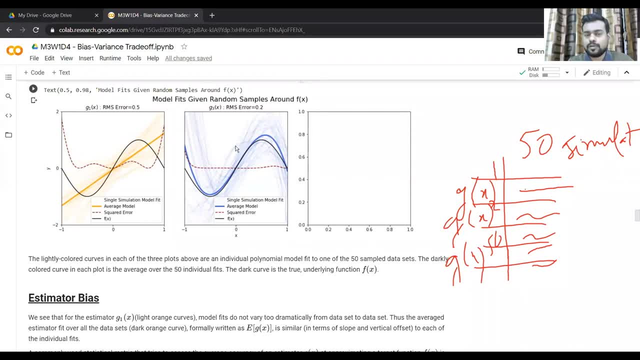 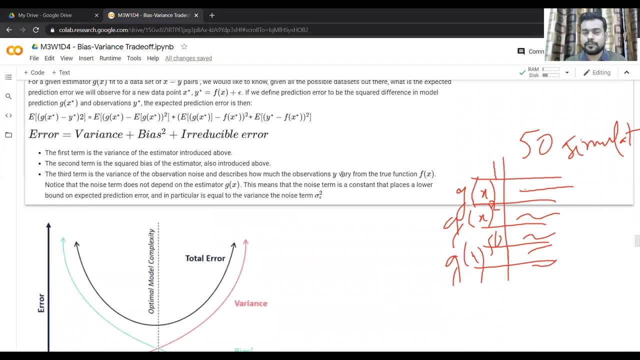 So this also sort of it has low variance and low bias, But in this, for this estimator, we have High bias but low variance. Okay, So we'll see an example and we'll familiarize ourselves with this- the whole notion of the bias variance across strain and test- and we'll get to know why these concepts are really. 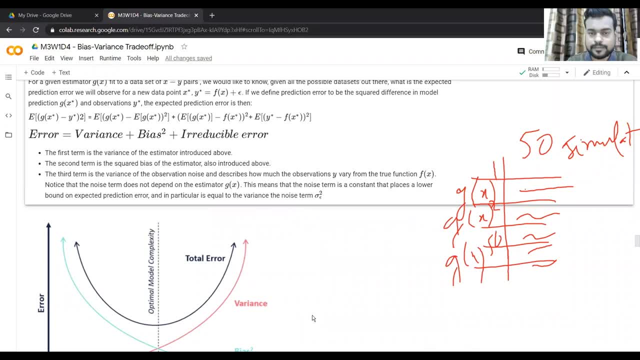 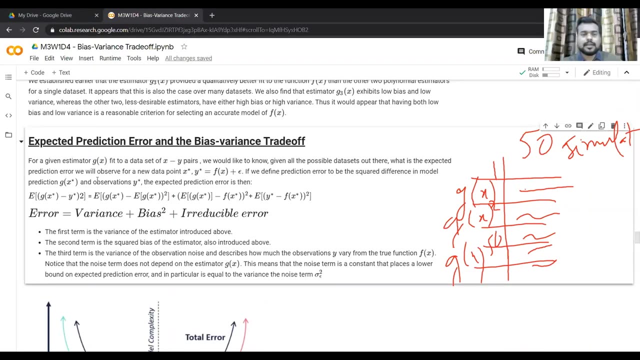 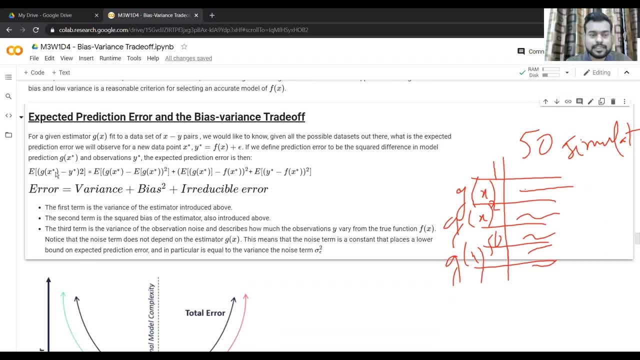 So what we actually want to do, so let's say this is: this is the function which we want to come up with, which will closely resemble our fitted, Our actual values. Why Right? So for a given estimated gs, which we want to fit to a dataset of XY pairs, 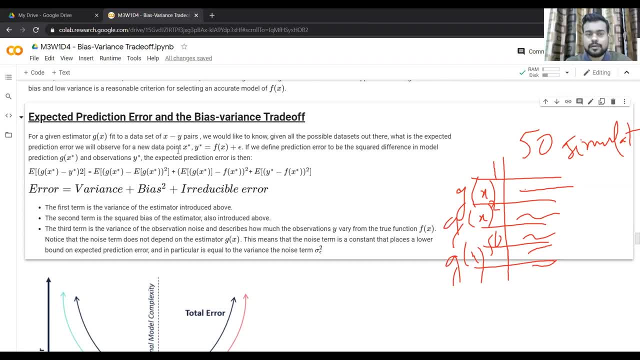 of X- Y Pairs, right? So what? what will be the expected prediction error when we observe new data points- X star and Y star, right? So let's have written estimated GX by looking at these X- Y Pairs, and I want. so what will be the expected prediction error when I look? 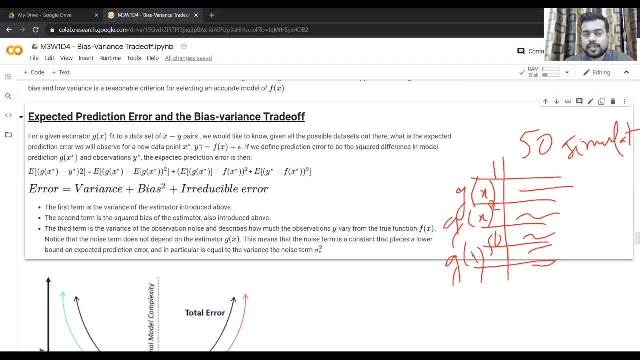 at new data point: X star and Y star. So this is again a pair, right? So our GX star minus Y star and, if I square this, so this is the expected prediction error which will expect- and this can be a lot probate here, but this can be written in this way, right? So so this: 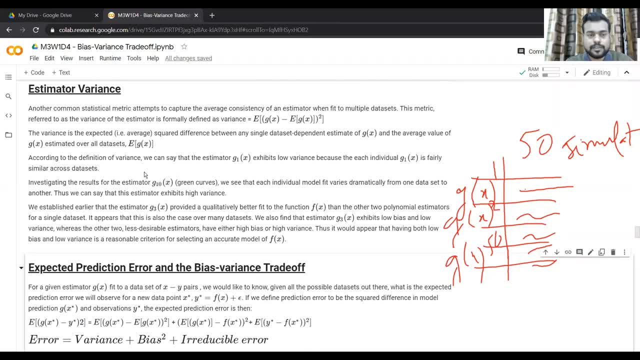 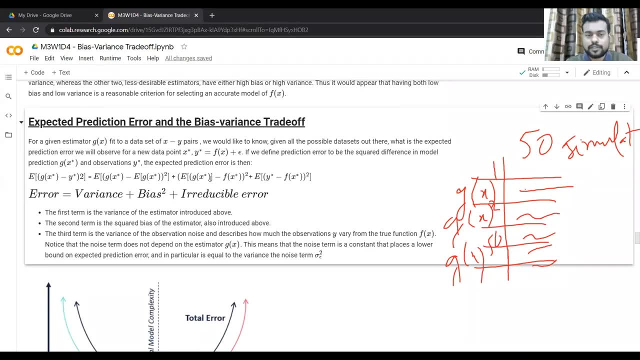 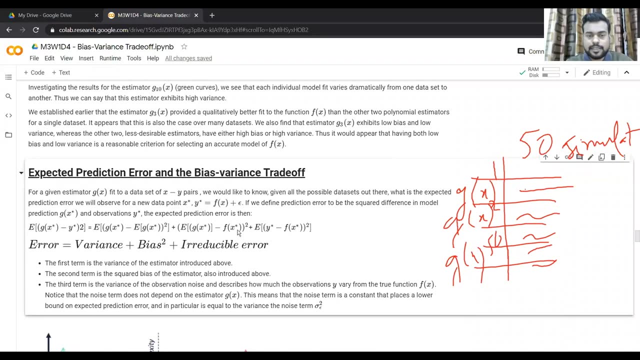 is the variance term which we have seen from earlier. right, So this is the variance term. then the second term Can be written as the bias, squared, right. So remember what is bias. So it's the average fit minus your true function, right, So right this and then plus this particular value. 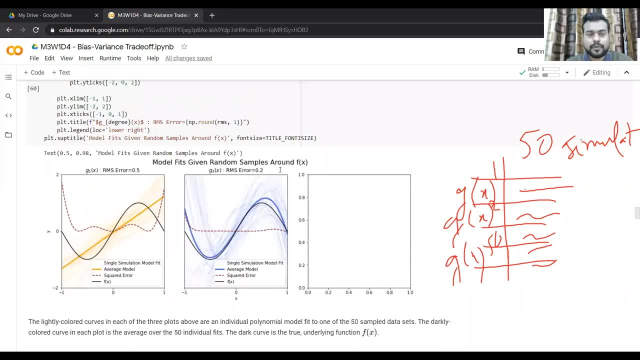 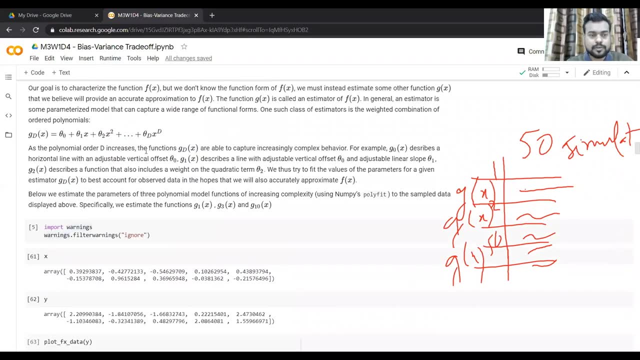 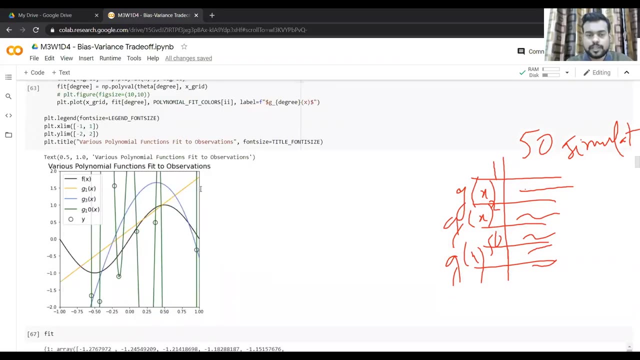 right. So Y star minus FX star. So if you remember Y star minus FX star, what will that be? So that will be our error term, right, Remember? so right, So Y star minus FX star will be some noise. Okay, so in general. so this is a very important equation in all. 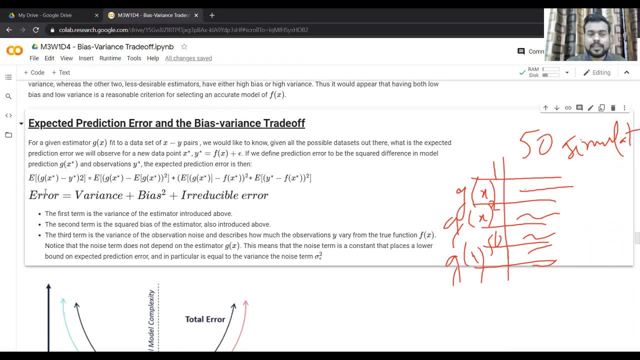 of machine learning. This is one of the most important equation as, in the total error which will get when we're trying to, which will have between our predicted values and the actual values, will comprise of three terms. One will be your variance. Yeah, so this will. 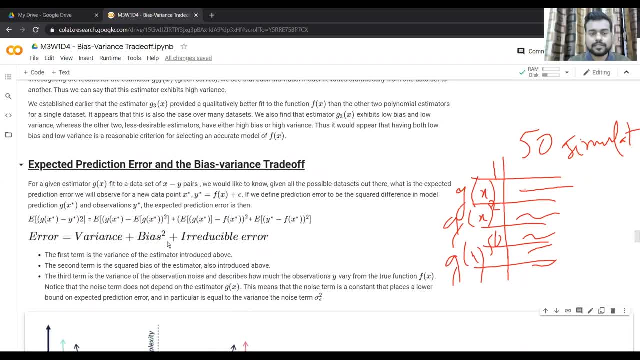 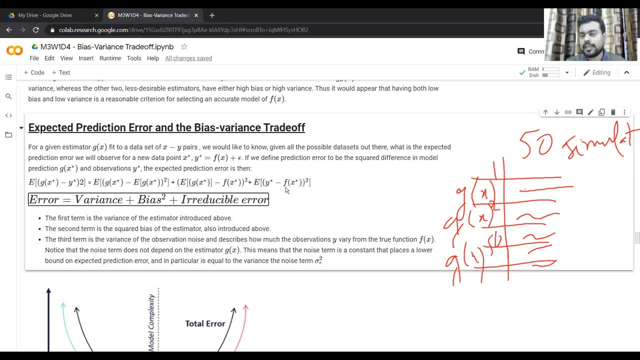 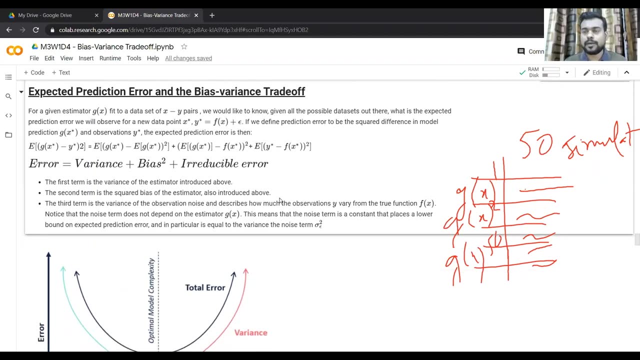 be your variance, So one will be your variance under will be your bias squared and third will be irreducible error. So in this case, this is your epsilon squared right. So so the point here is, whenever we are doing any modeling, whenever we are doing any prediction using our estimated G, 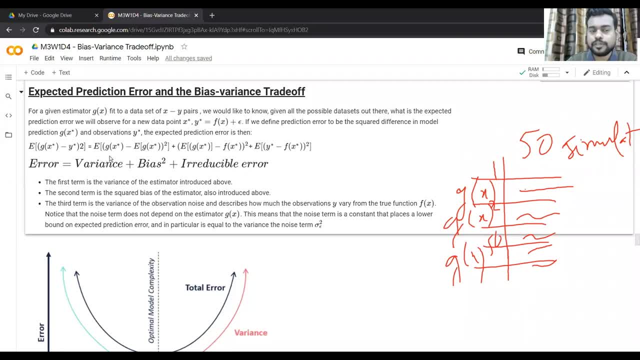 So we'll have an error introduced due to variance, will have an error introduced due to bias, and there will be another component Of an error about which we cannot do anything right, because this error will be inherently present in data sets and cannot be removed right? So this is what we call it: irreducible. 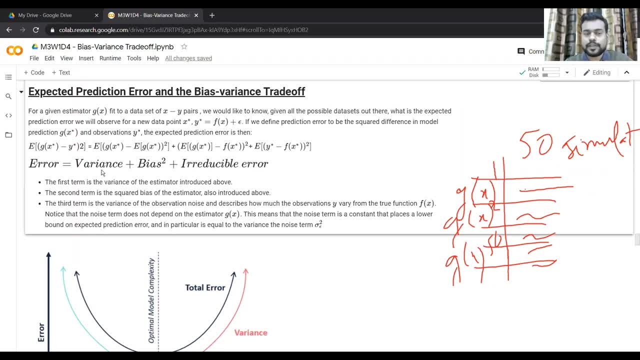 error. So the only two sort of sources of error which we can try to work around with is variance and bias squared. Okay, so variance is given by this term, bias is given by this term, Of course. So that's why I've written Y is squared, So the first term is the variance. 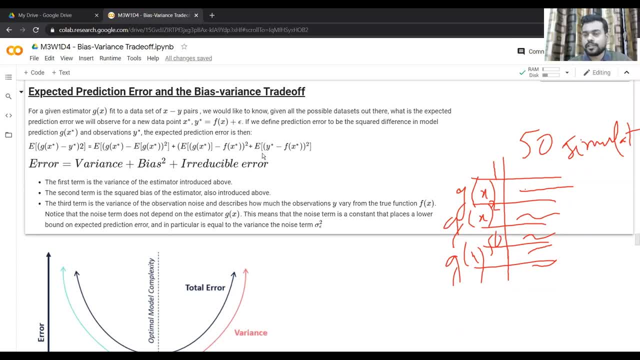 The second term is the squared and the third term is essentially described in noise, which is which will always be present, and we so this is the least error which will have when we are, whenever we are modeling relationships between X and Y. This is what we call as irreducible error, or also called as Bayes error. 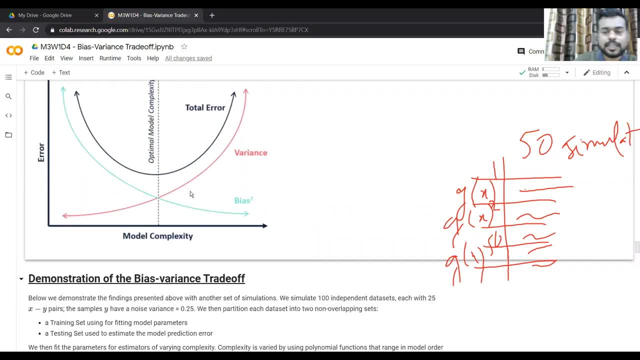 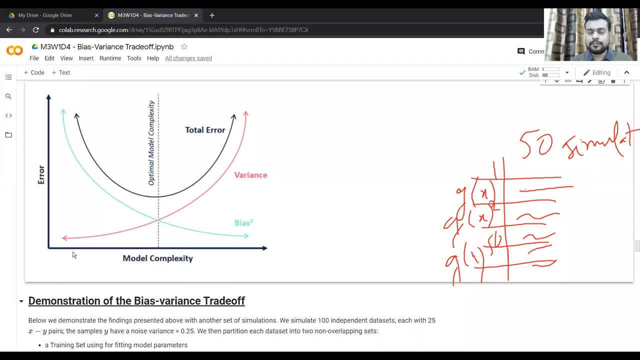 Okay, So this is how the curve looks like when we increase the model complexity. So let's say, if you're moving from relatively simple model to a more complex model, So for a simple model. so if you look at the bias term, right. 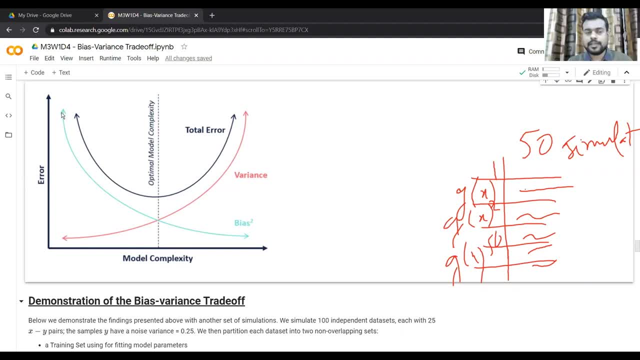 So the bias will be high, as we saw in our for saying g1x. So bias was high for g3. It will be low and then it will be low for if we increase the model complexity, as in if we have, if we allow our model to be flexible enough. 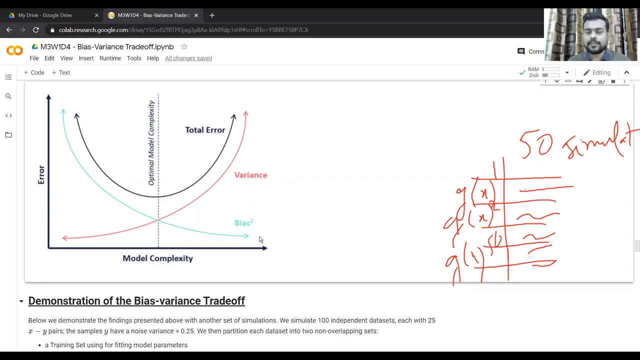 it will fit over all the values in your training data set, Okay, and eventually it will have low bias when we are talking about complex models, So they will have low bias as well. They will try to fit to all the given values which they'll see in the trading data set. 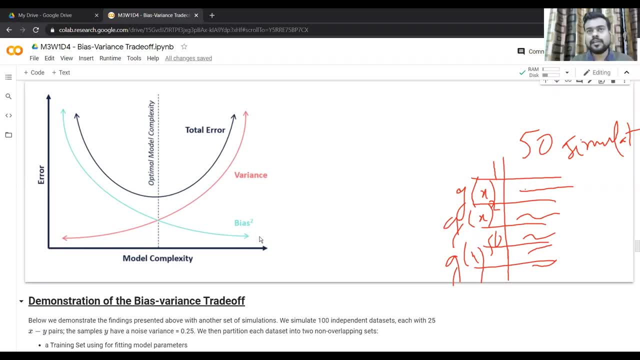 So bias, we can also say that a low bias will tell you how well your estimator has fit the training data right. That is what we call as low bias. And then if you look at the variance, so if your model complexity is low, 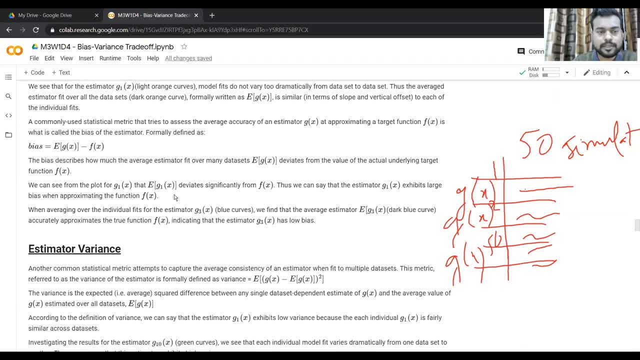 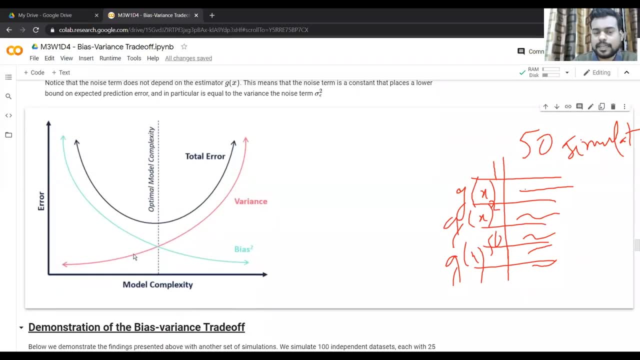 okay, so we'll have low variance. So, as you saw in this particular for the experiment, so we had low variance. for g3 also, we had relatively larger variance, right, And if we increase the model complexity we'll have a lot of. 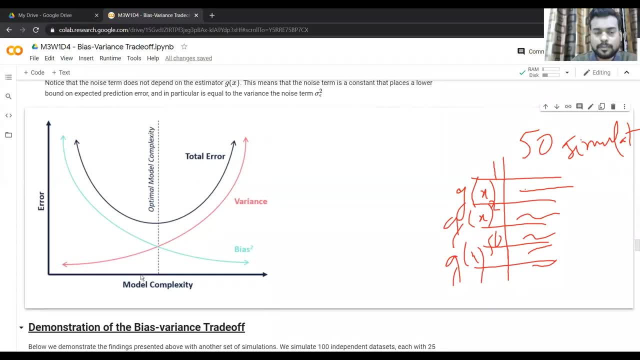 a lot of variance, right? So if you talk about error and model complexity and think of these two terms, bias and variance, so if we go from the relatively simple model to relatively complex model, so we see that bias is increasing, decreasing, but variance is increasing. 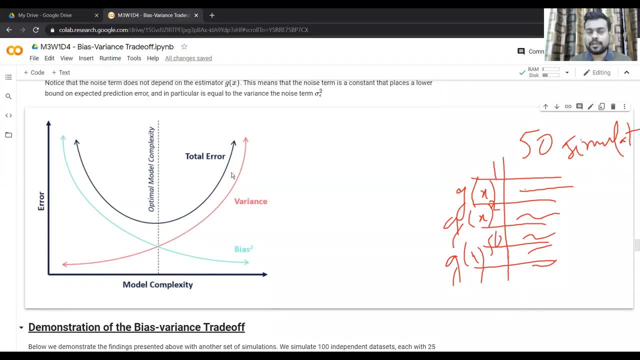 and that's why there is this term which you're encountering, that is, bias, variance, trade-off. to find our optimal model, complexity or optimal model, Or the optimal fit, will have to find some values in between for which will have a relatively low bias and relatively low variance. 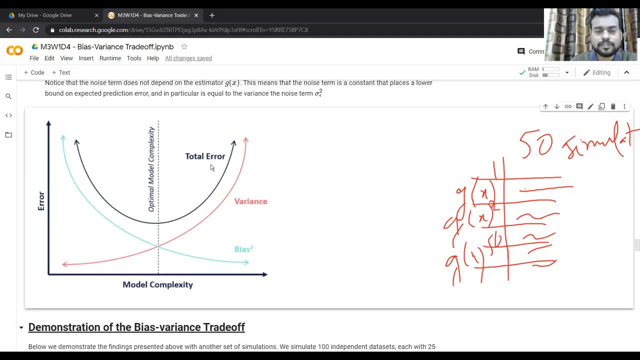 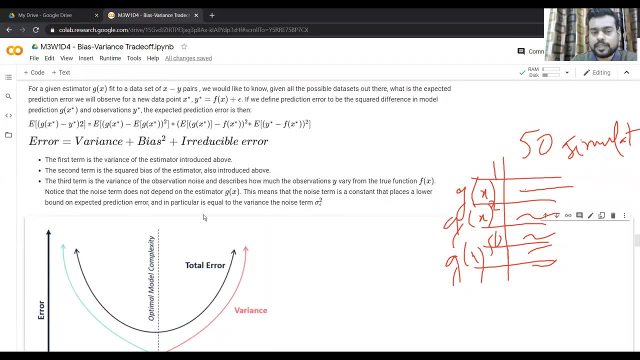 Okay, and this is what the total error looks like, right? So, totally you remember. this is the sum of these two terms: bias variance, plus bias squared, plus this particular term, right? So if we add these two curves together, so you will get something like this: 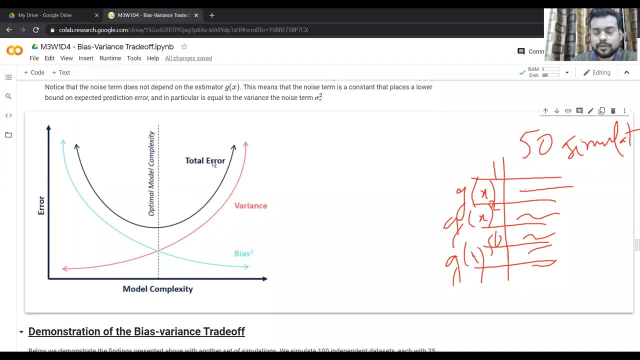 right. So the minimum value of this total error lies somewhere here, somewhere between, somewhere for this mid-range complexity, right? So we never want to go with a very simple model. We'll never also want to go with a very complex model. We'd want to go with a model which is somewhere in between. 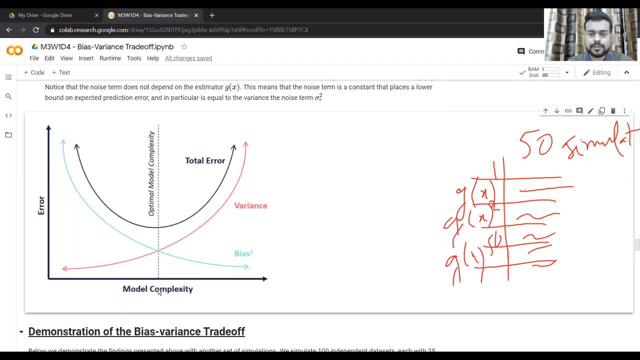 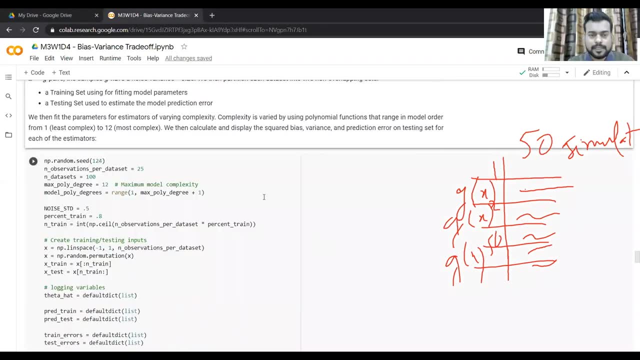 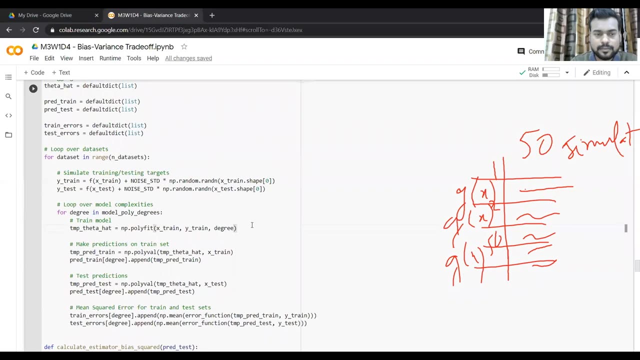 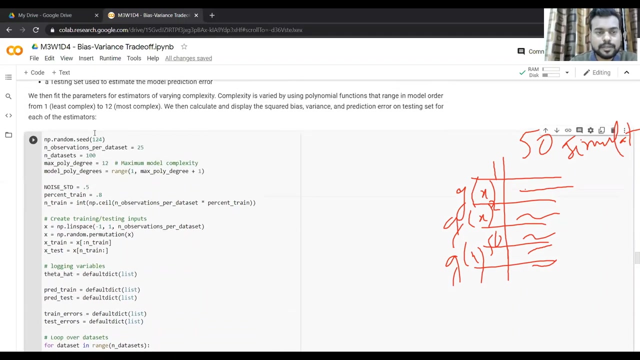 Okay, So let's do an experiment. I think we are running out of time, So, but let's do an experiment on our data, and yeah, well, so here also what I am doing. so, So we are focusing on three polynomial degrees: one, three and ten. 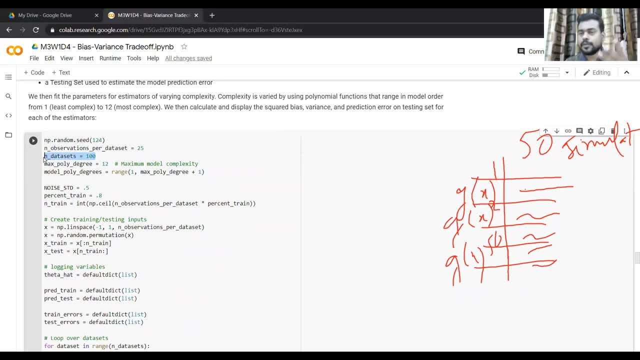 Okay, and we have hundred data sets. So earlier we are doing the simulations on 50 data sets, So but now we have 100, okay, and noise of standard, standard deviation of noise is 0.5.. And this is the important concept, which is percentage train. 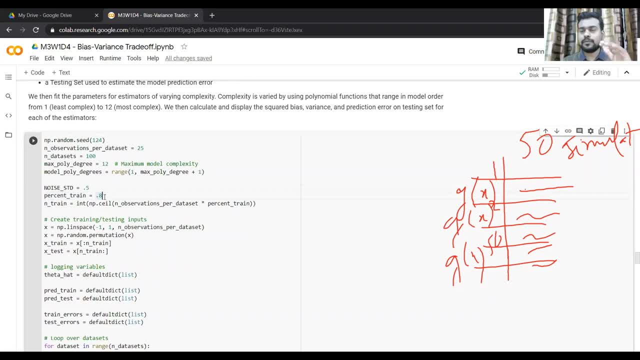 So it is pointed So in our data set will will divide into train and test. So we'll keep 80% as a train and 20% as test. So this is what is meant by percentage train And this is how we'll get the number of training examples in our training. 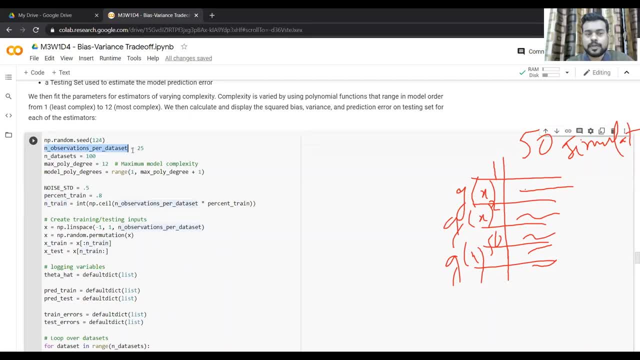 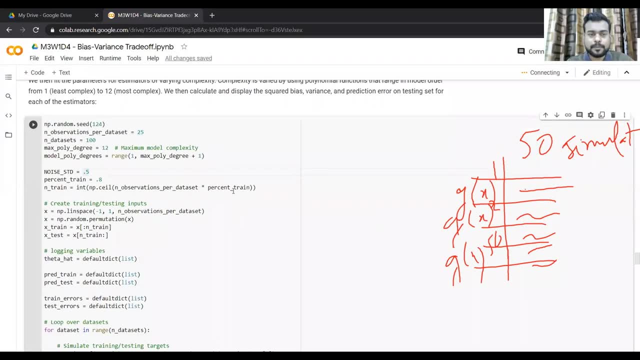 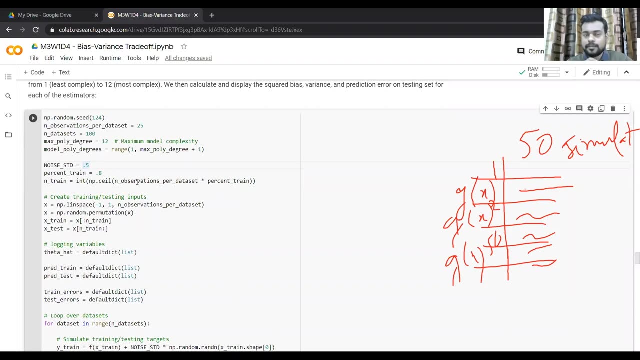 Data set and the number of observations per data set will be 25.. So just take 80% of 25.. Okay, so just take 80, 80%- 25.. So that will be for one. simulation will have that many observations in train and for test will have the remaining one. 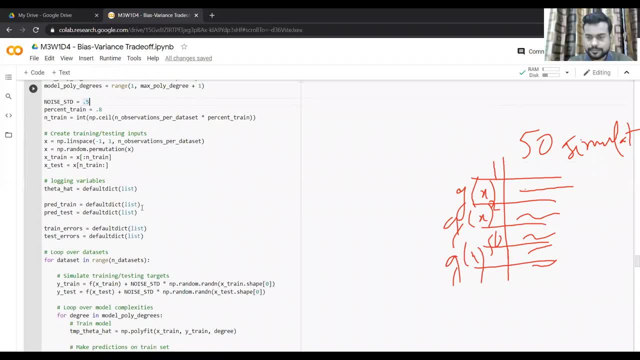 Okay So, and we don't see, is basically saying the ceiling Of X, right, So it's the it is. it leaves integer greater than or equal to that particular value. So let's say, if this comes out to be 18.6.. 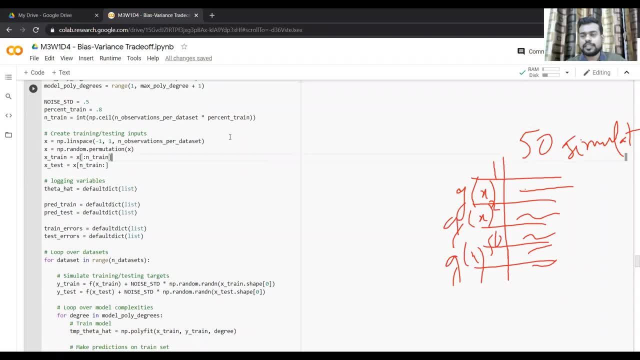 So then n train will be 19.. Okay, So, ceiling of X. Okay, So there is floor of X. So floor of X is the greatest integer less than or equal to X. ceiling of X is the least integer greater than or equal to X. 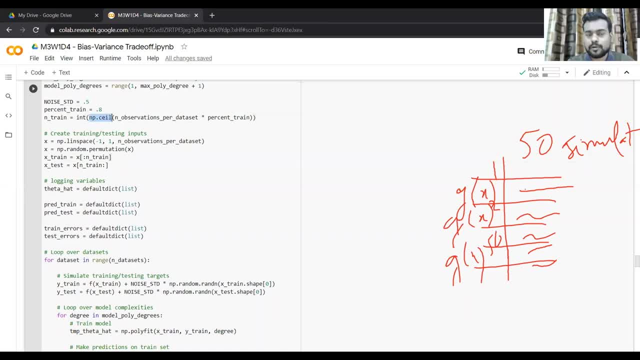 Okay, So I think when you go through the codes, you know free time. I think you should be able To figure out most of these things, because these are not something new which you are seeing, but I will describe the overall procedure of this particular experiment because I want to identify. 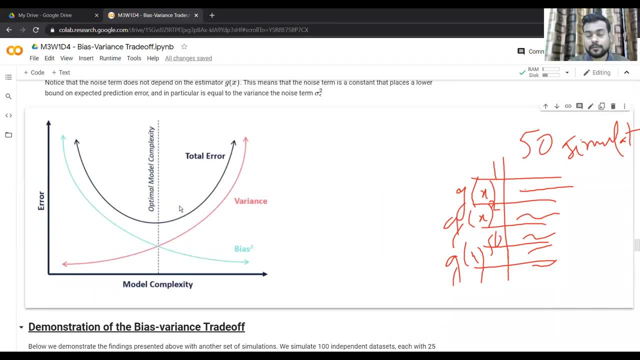 I want to validate this particular assumption, particular concept. So if you vary the model complexity, so here our estimator is a polynomial estimated. So we'll vary the complexity from degree 1 to degree 10 and we'll see how the train and test error looks like, how the total error terms looks like. 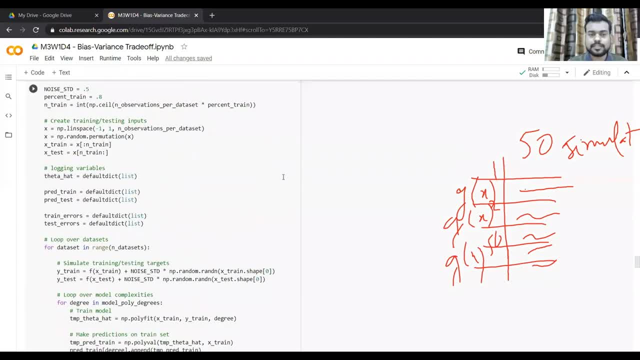 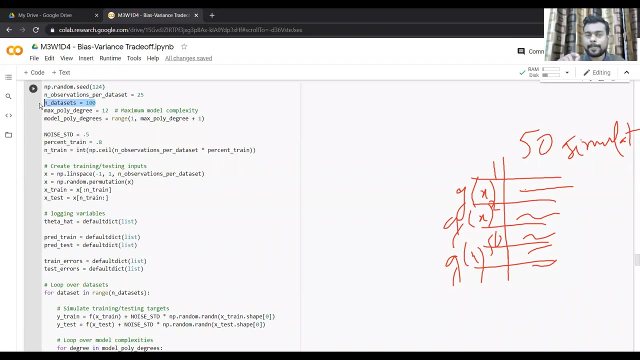 So we'll be seeing those things. So I just describe you the recipe for doing this experiment, but you can go through the codes and understand what's actually happening. So, yeah, so for each data set. so we'll be doing hundred simulations for each degree and in each simulation will have a data set with 25 observations. 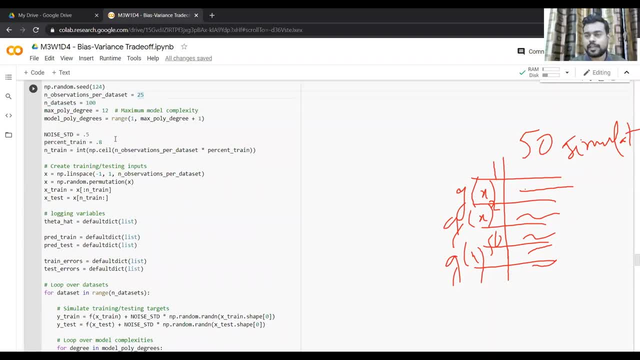 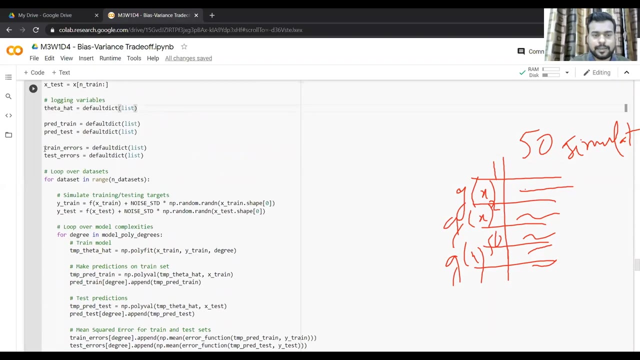 And we're keeping 80% of train observations, 80% of observations in train and the rest 20% in test. Okay, So this is how I create the train and this is how I create the test. Okay, and I'm creating some dictionary is of lists, as in my values. 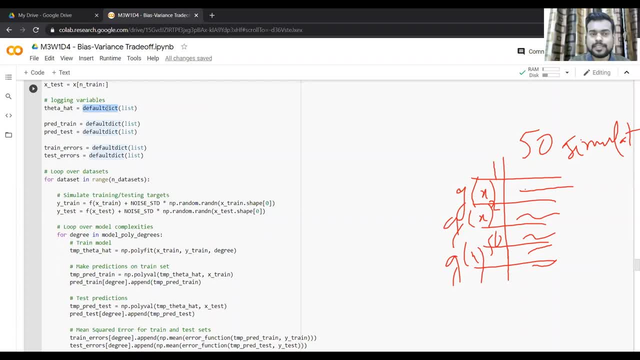 So this is a function. I don't think you have encountered this, but this is a similar to date, But here we can Provide a function as well, So my value will be a default list, right? So if I don't have any value right now, 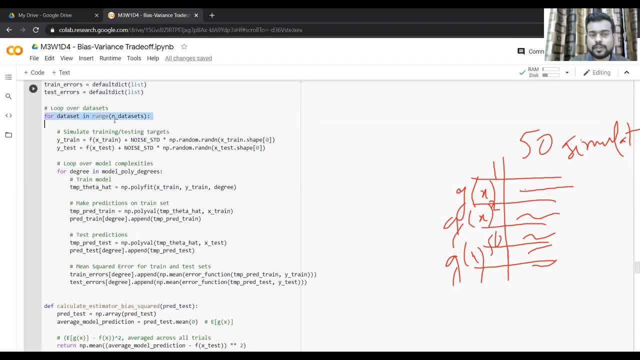 we are moving ahead. So for each data set so far, that is, for each simulation, So remember, and data sets is a hundred. and then so for each data set, of course, our Y train and Y test will differ, even though X train and X test are the same. 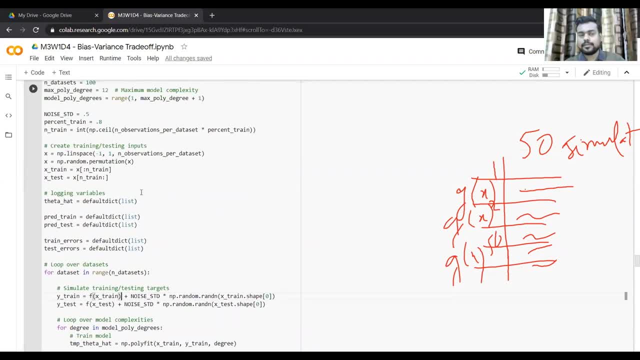 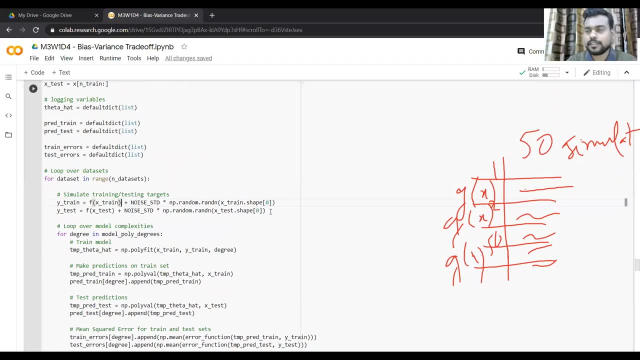 right, So X, train and X test will be same for all the simulations, But Y, train and Y test will differ because we are randomly sampling the noise from the new normal distribution and so will of course have different data set because the valued pair, which is XY, that will differ for each data set. 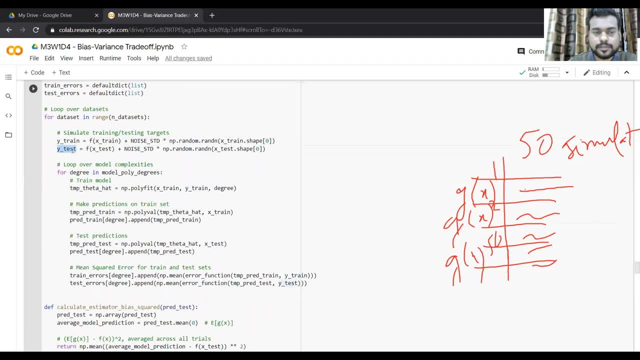 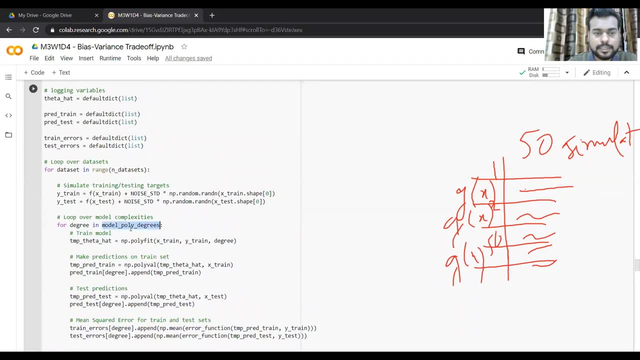 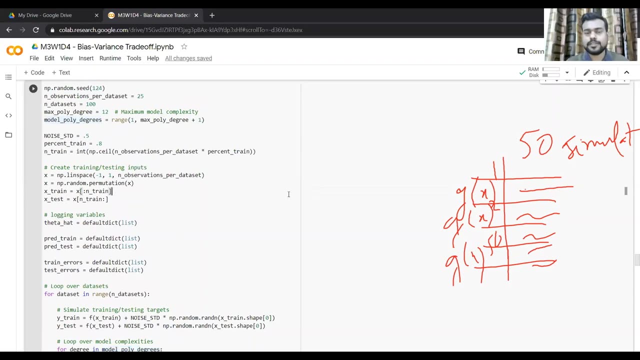 So Y train is this and Y test is this one. Okay, So now for each degree of the polynomial. Okay, So this is the model poly degrees. This is the list, which is from 1 to 12.. So this is from 1 to 12.. 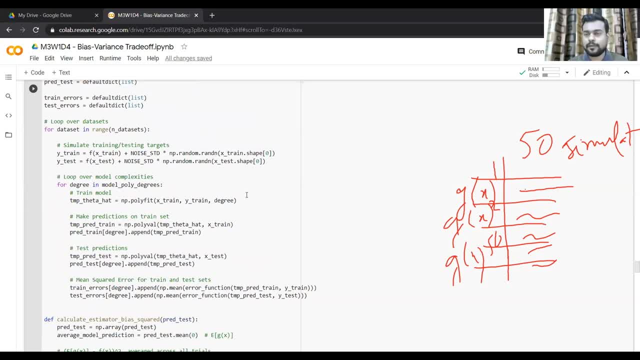 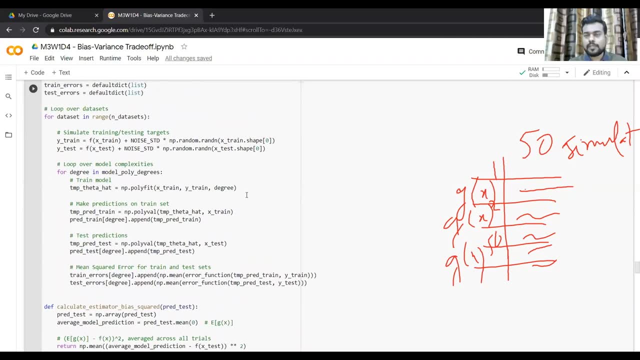 So repeat the experiment for all the degrees, from starting from 1 to 12, right, And for each degree will be doing the experiment across all those simulations, That is, across these hundred data cells. Okay, So what we are doing here. So for each degree. 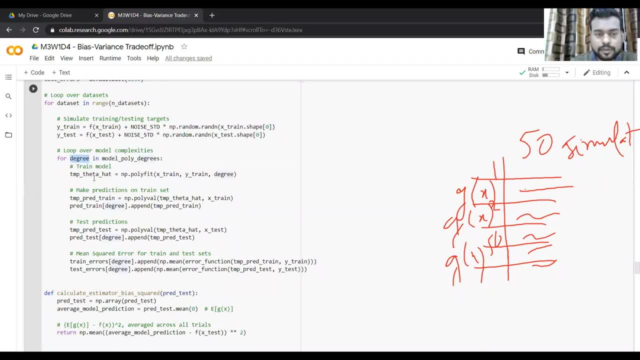 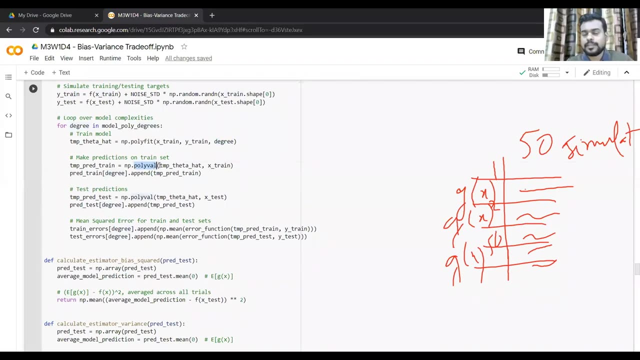 so let's say for the degree one, right? So I'm doing a poly fit, which is X train, Y train on X train and Y train providing the degree, and then I am validating this, or basically taking my fitted estimated and I'm trying to predict the values. 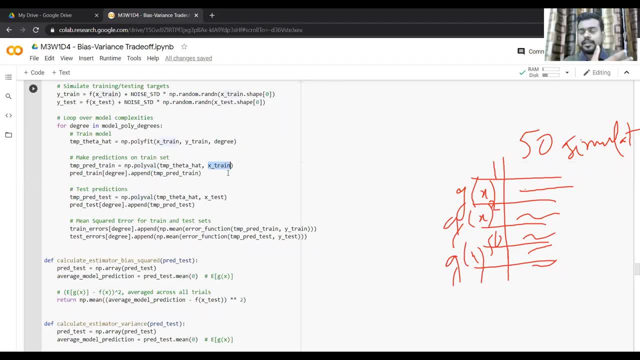 Firstly on train, right. So of course earlier we had seen that we are just doing that on a whole set of values, between all set of hundred values, right, But here what we do will predict that on the values of train, and then we'll predict that. 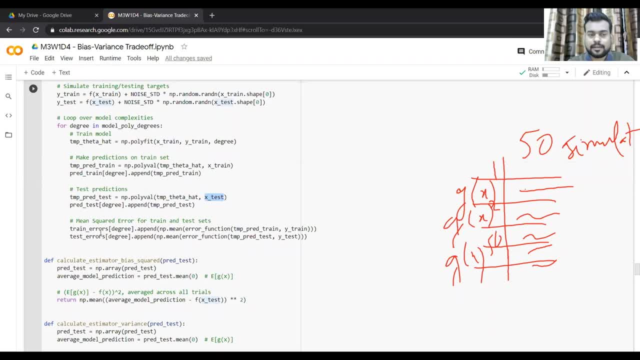 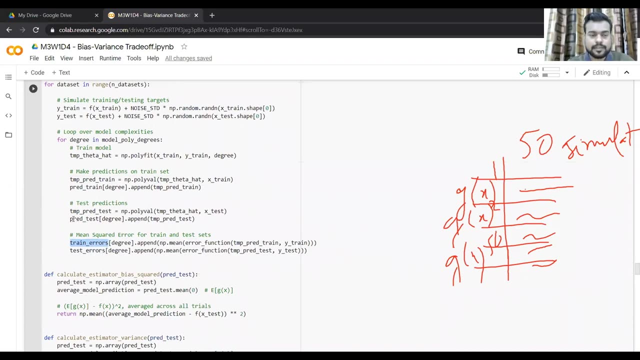 on the values of test. Okay, and then we'll: yeah, so we'll calculate the train errors and test errors. So how do we calculate the train errors? So for a fixed Yeah, so for a given degree. so we are calculating this bread test and pray a bread train. 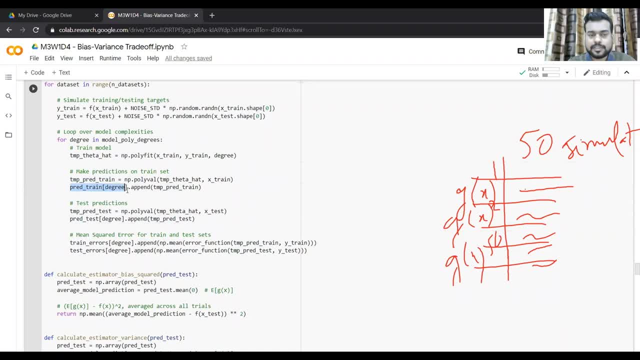 right So? so for each degree. so this will generate a dictionary, isn't degree will be your key and you'll have the list of values for your train, right? So train predictions and here also you'll have the test predictions. Now we can calculate using the error function. 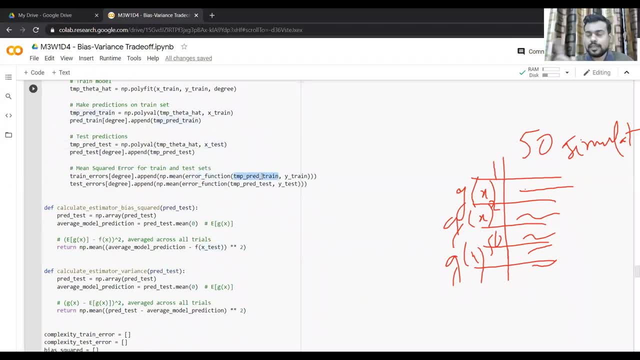 We can calculate the difference between your train and actual predicted train and the actual train. and also for the test we can do the same thing: predicted test and the predicted test value of actual test value in this will be calculated train and test error. And then, if you want to average this over all these simulations, 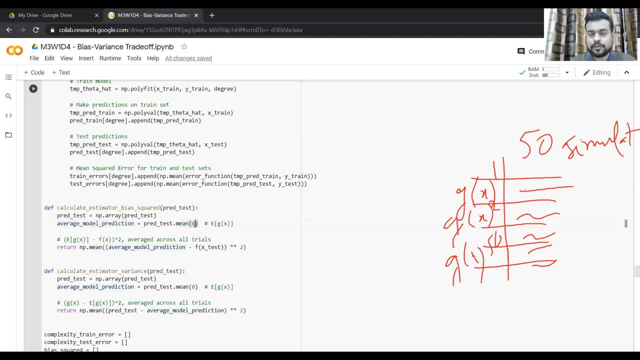 so we'll take the mean across the axis 0.. Okay, so this is, this is how we'll get the average model prediction. Okay and then. so our bias squared will be average model prediction minus my, our actual the five Function for test squared. 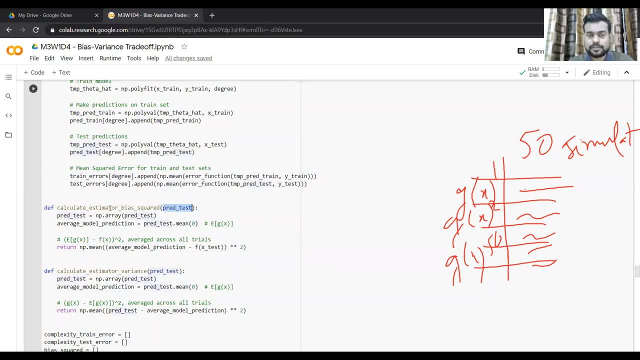 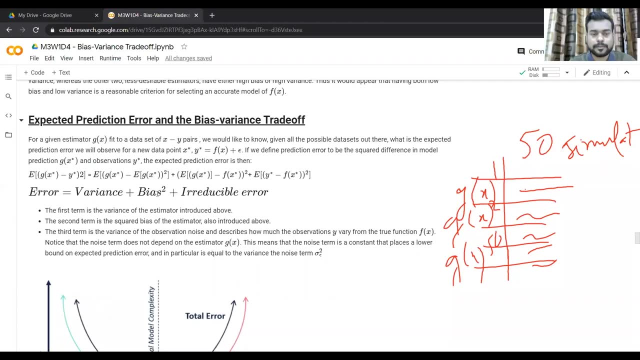 right. So this will be calculating over the test data set, right? So this, so this term is calculating the bias square term, Remember from above. So this is calculating the bias square term, right? And then we have another function, which is which is calculating the estimated variance. 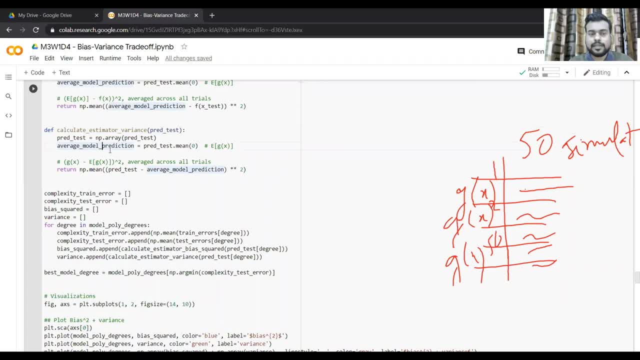 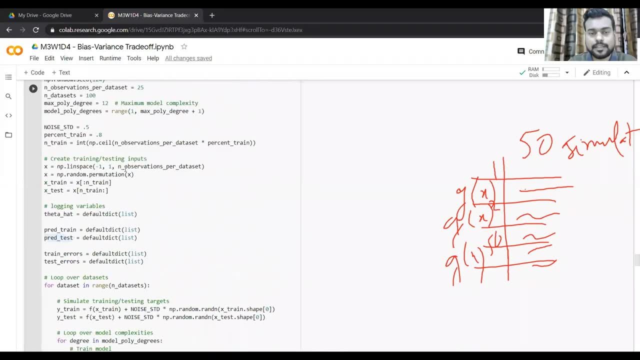 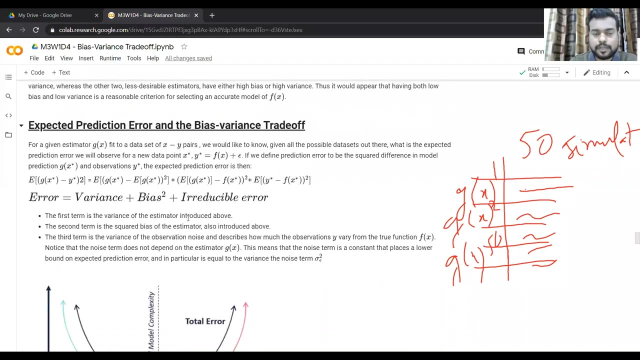 So here also we are calculating the average model prediction and then for each model prediction we're taking the expected values. So we are calculating this particular value right. So this one right, this value. So for now we are doing this on print test only. 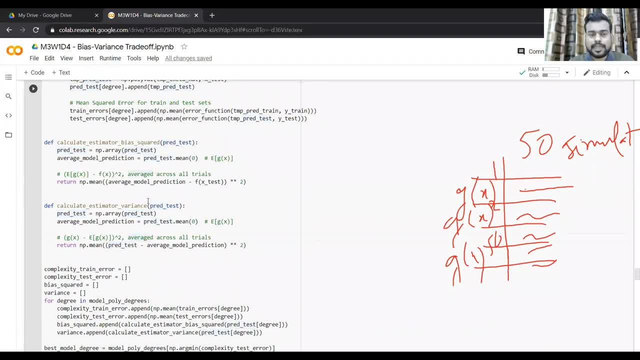 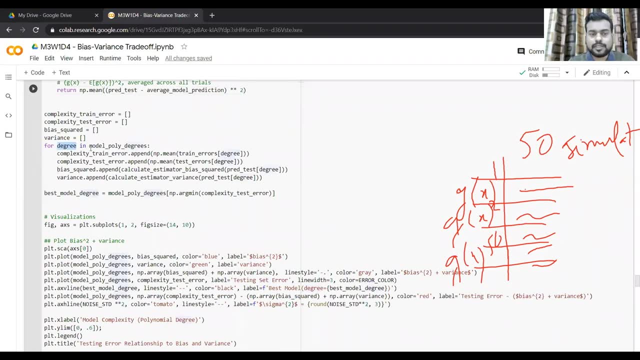 right, So this will help us give the bias and the variance across our test data sets. So now so for each polynomial estimated, right? So what we can get? Yeah, we'll have a list of complexity train error. We'll have a list of complexity test error. 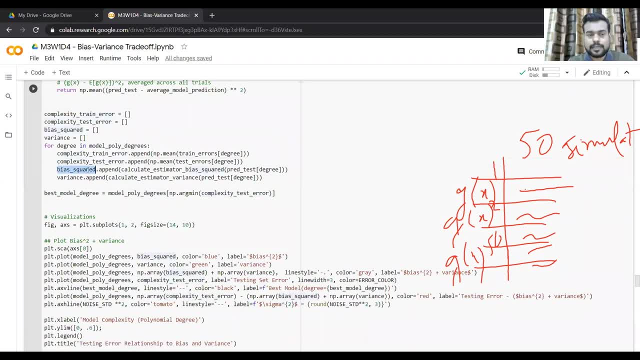 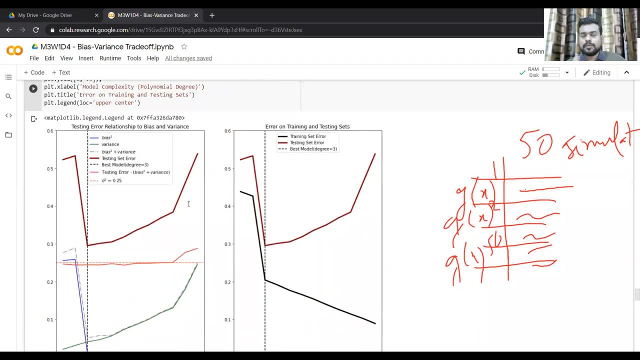 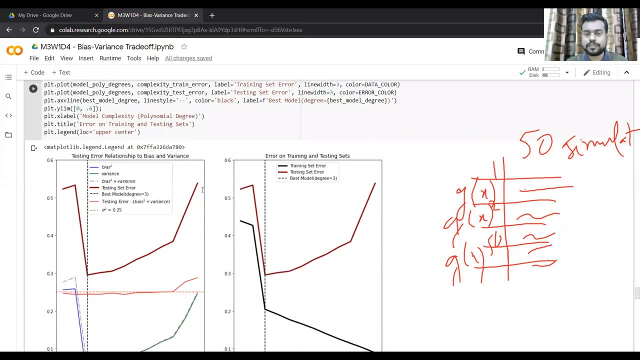 Okay, and then we can calculate. Yeah, append all the values for the bias squared and the variance, right? So if you plot this, so if you're not getting all the codes here, but don't worry about that- the important concept which you should understand, that if we vary, the model complexity, 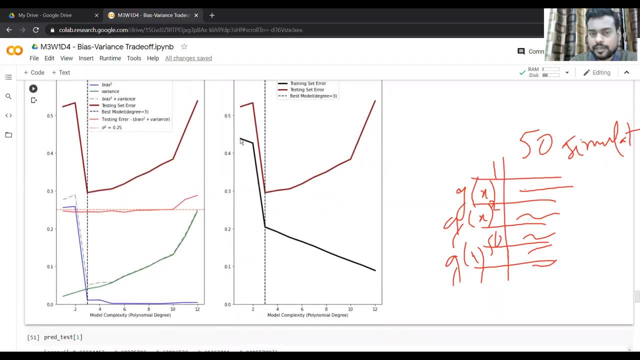 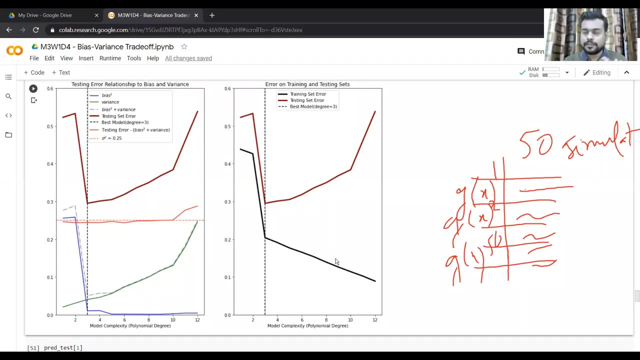 right. So you train error will decrease your train error. This is the training center, right. So if you vary the model complexity, so if you go from a relative of a simple model to a complex model, the error which will have on our training set that will decrease. 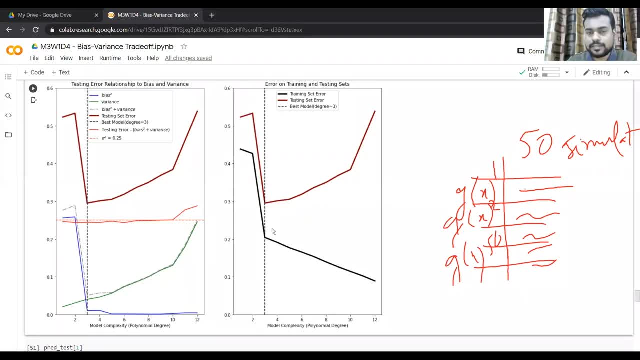 So for this particular experiment, this looks like this black line, but if we calculate the test, set error, this sort of decreases and then increases. Okay, so right. So this is test. There is a data which is not seen by the model. 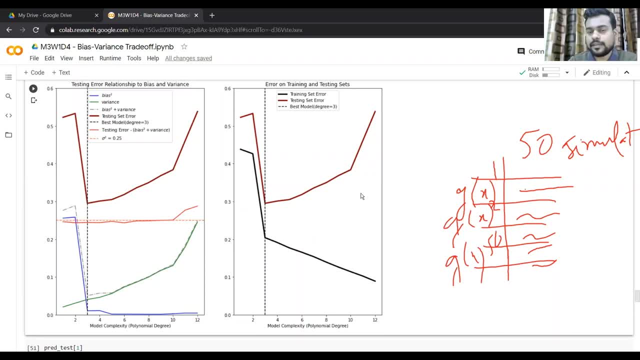 So model is not performing well. So I will say that a simple model or very complex model They are, they will evidently produce high errors on test. set right. So a model with, let's say, an optimal complexity, So it will have the least error for your test. 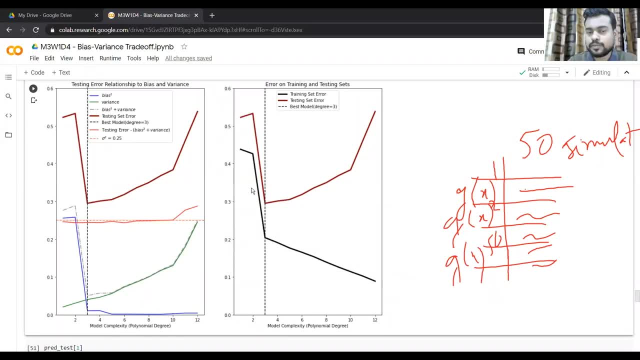 So see why this trainer looks like this one. Why the trainer is reducing: because if, when we are increasing model complexity, we are allowing the model to be flexible enough so that it can miss. look across all the observations on which it is getting trained. 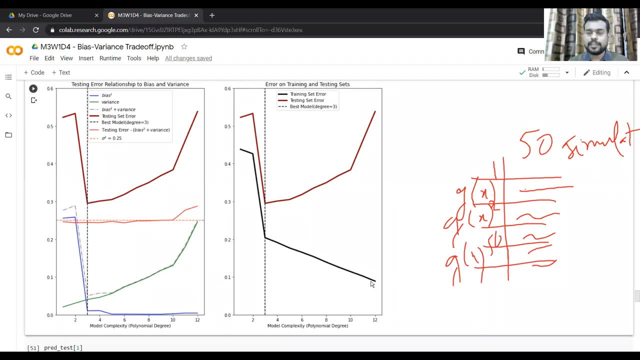 And that's why there will be very small deviations in your a tray, Mr Train, why values and predicted train values right. So that's why this train set error is very small. It decreases when we increase the model complexity, but this test error it increases. 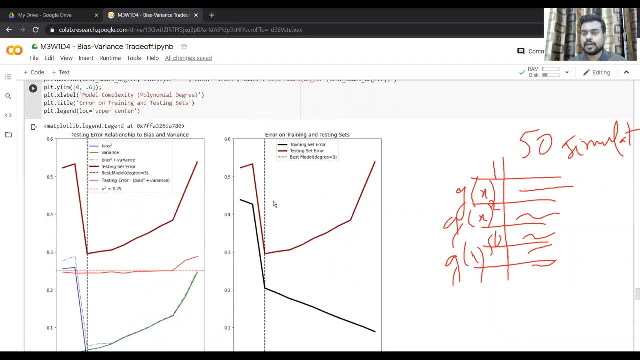 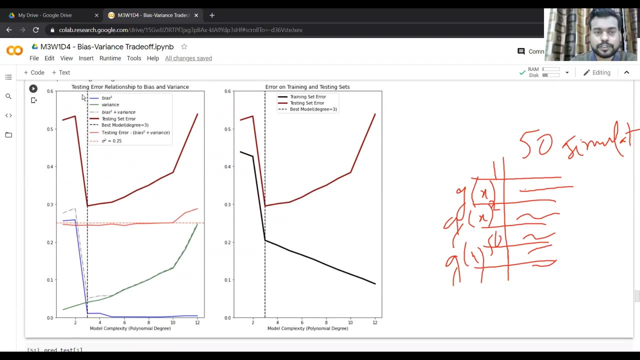 right. So why so this test error is the sum of the components, of some of the two components- right bias, squared plus variance, And then, of course, there is an irreducible error component. So if you look at this particular graph on the left, so let's say, if I'm just focusing on test data set, 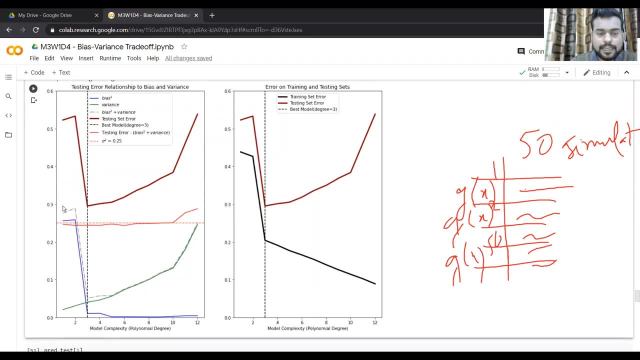 Okay, so if I increase, if I increase the model complexity, so see, bias is decreasing, bias is decreasing, right, This blue curve, This is in fact the bias squared, the variance in fact, but variance is increasing. very pleasing the model complexity. 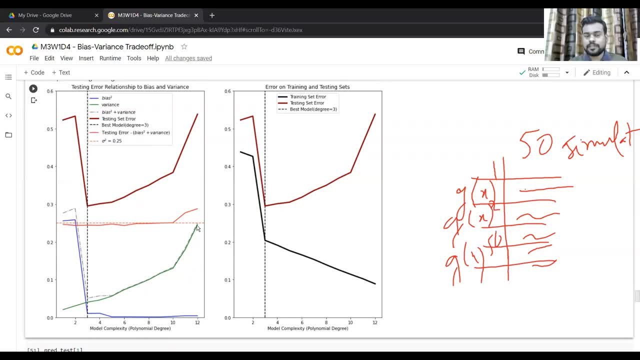 Right. So so far as you can see that for each value on this test data set, because model is really complex, So values are sort of very fluctuating and that's why we see, I variance Right And then test error is of course some of these, some of the blue and the green one. 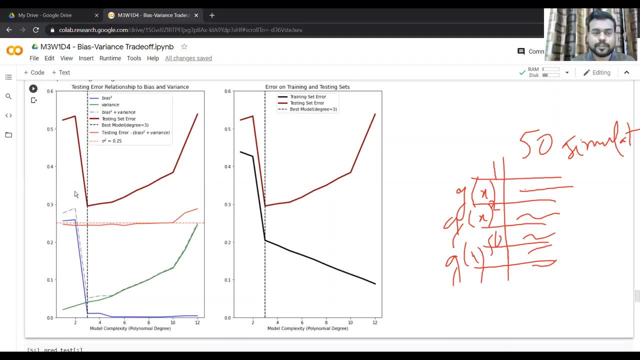 And this is your, this particular maroon colored curve here right, And we, our optimal model, which will select, will be here right, Which will give us the least error, least total error across test, Right? So this is what we are saying. 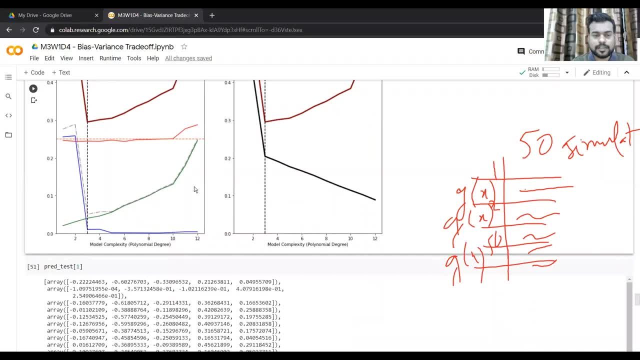 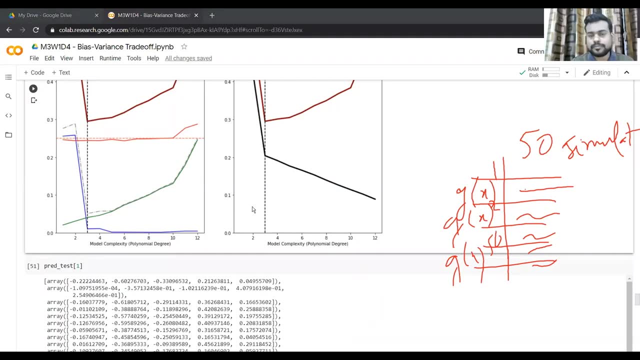 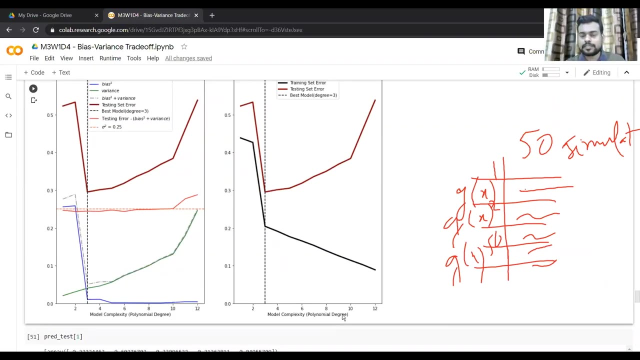 Right, So this is our optimal model in this case. Okay, so, yeah, so. so we can again say that polynomial when we are increasing the complexity of the model. So this is overfitting. So when we are overfitting. 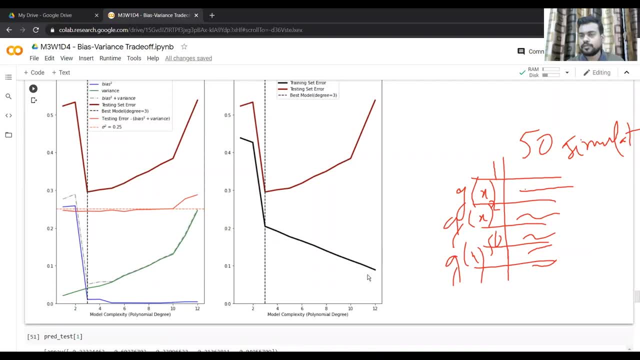 so it's essentially: the training error is quite small because we are overfitting, but the test error will increase a lot. Okay, in a model when we had a very simple model, the train error was large and the test error will also be large. 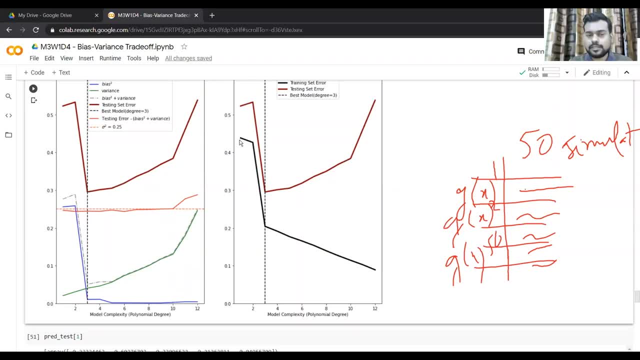 Okay, So, so, this is so, this model, the model with a low complexity. So we'll call this, call this model with high bias and low variance, right? So this is high bias, rates of blue curve is high bias and this is the variance. 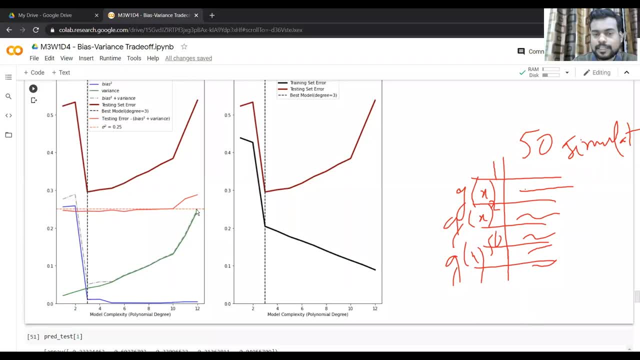 So this is a high bias, low variance. and but if you're increasing the complexity of the model, so that model will be high variance, high variance, but low bias. right, So we'll have to. there will be a trade-off between your bias and variance, because these are acting in opposite directions. 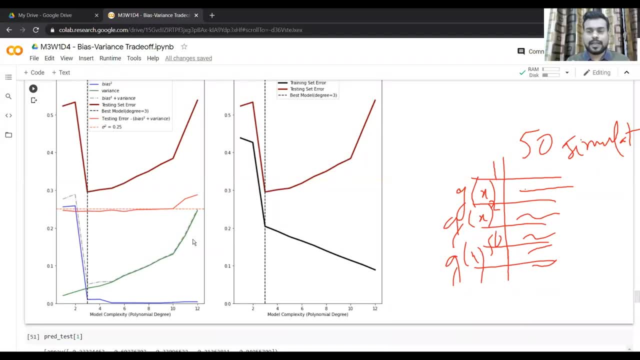 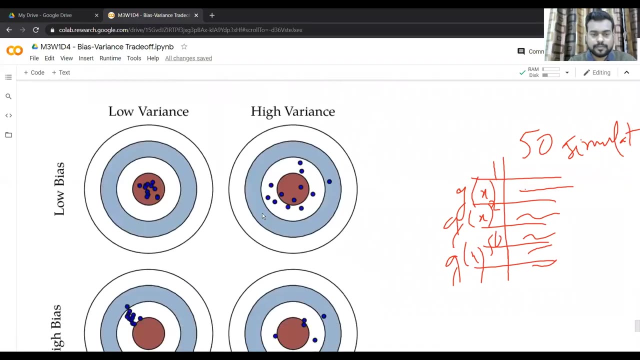 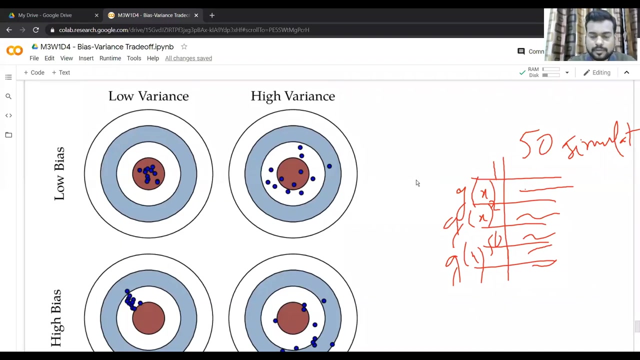 When we increasing the model complexity right and we'll have to find a middle ground to choose our optimal model right. So in this case I will go with polynomial degree three. Okay, So so this is. this is one photo or image with you. 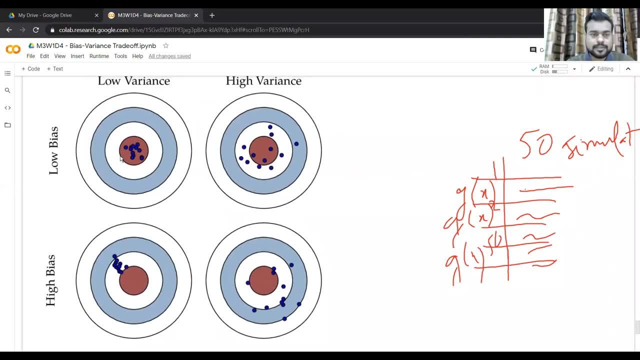 Yeah, Yeah. So how does the lower bias and low variance looks like? Okay, So, typically what happens? that a low bias model will have high variance and your high bias model will have low variance? Okay so, but how the how the four combination looks like? 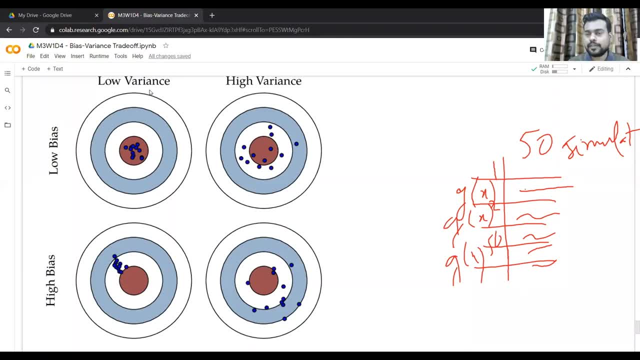 So you have low by the so suppose you're playing a game of dart and you are throwing your darts Okay, in the bull bull's-eye right. So if you have got this situation where you're, let's say, you are throwing 10 dots and they're all clustered in a very close point and yeah. 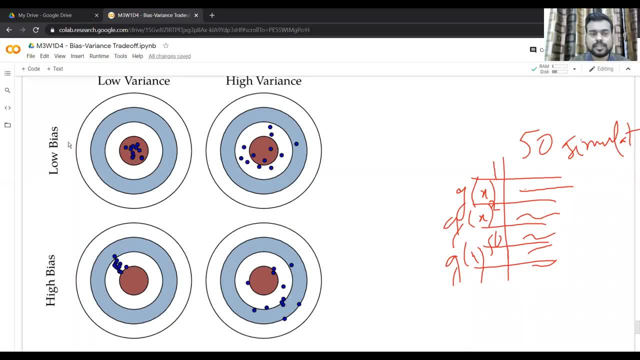 and they're, they're all hitting the bull's-eye. So you'll call this as low bias and low variance. but let's say, the darts which you're, which are thrown, So they are mostly around the bull's-eye, means that they are closer to the bull's-eye. 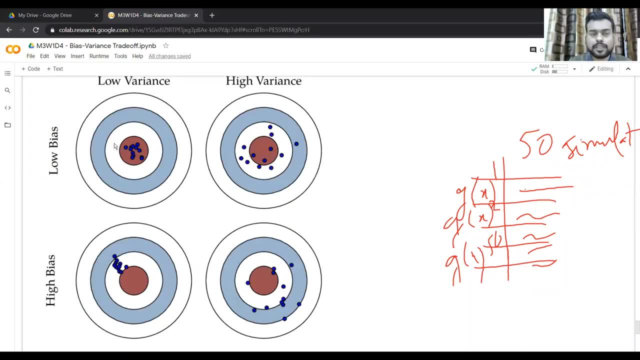 but they are sort of relatively spread around. So this, what we'll call, is low bias and high variance. but let's say another, consider another situation where we have high bias and low variance, right? So let's say you're not hitting the bull's-eye with your. let's say: 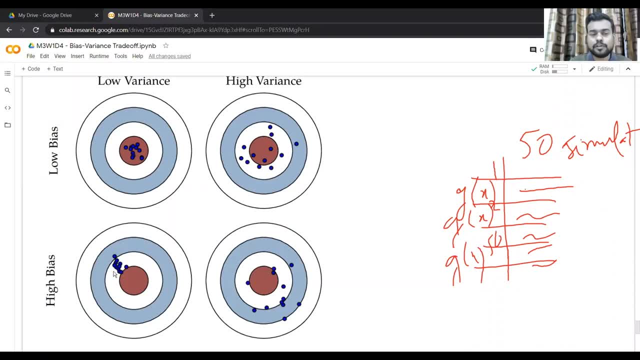 a bit away from your bull's-eye, but all your throws are sort of centered, are very close together. So we'll call this scenario as high bias and low variance. And then another situation is high bias and low variance. So you're doing the worst, actually, in this. 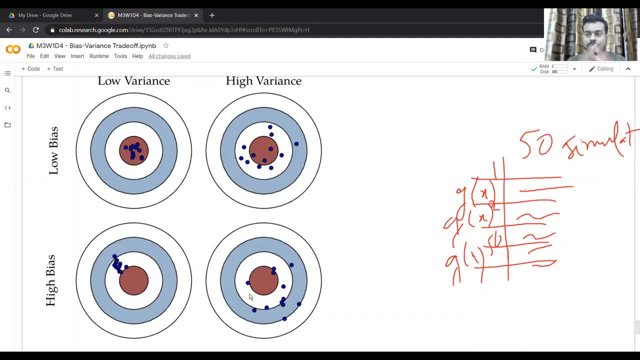 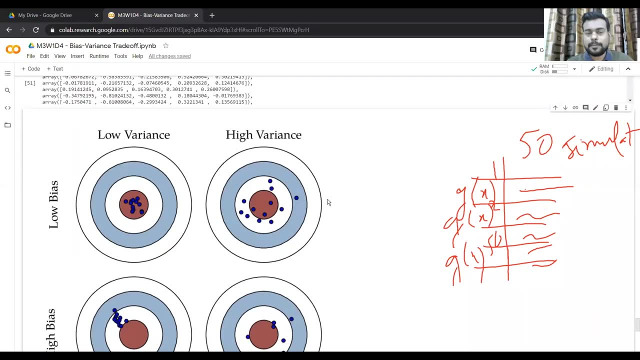 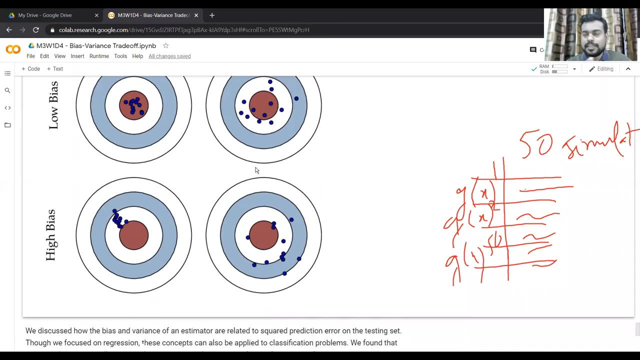 So of course you're not hitting the bull's-eye and you're sort of very spread across, right? So in this case you have high bias and high variance, right? So typically what when we increase the model complexity, so for a relatively simple model will have high bias. 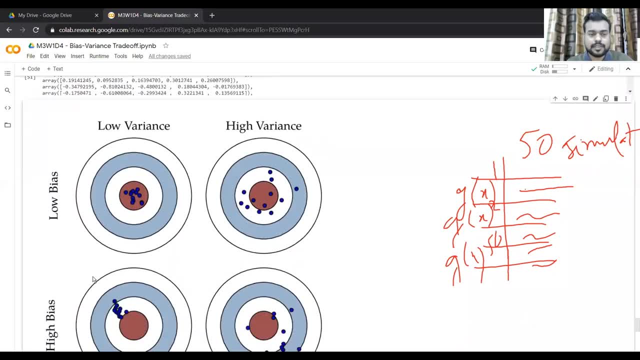 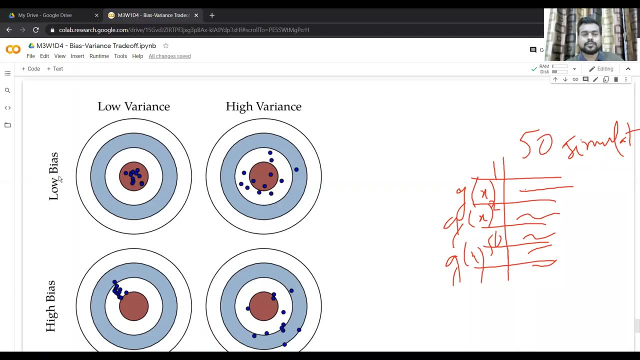 but low variance. right, Something like this. But if we increase the complexity of the model will have low bias and high variance. So low bias, essentially. So the decrease of bias tells you that we are moving from underfitting to overfitting. 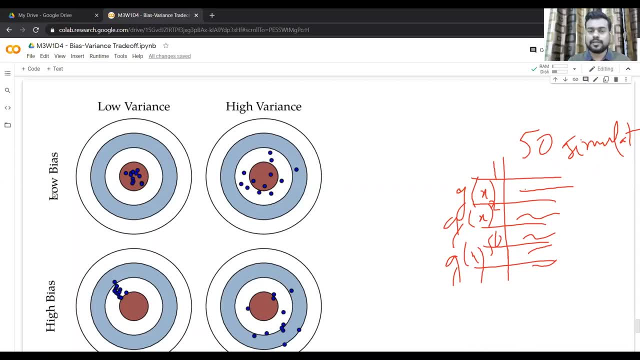 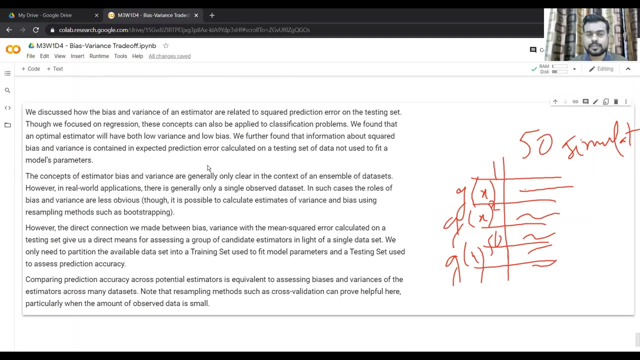 And the increase in variance will also say that we are moving from underfitting to overfitting. So I hope this particular concept is clear. So just to recapitulate, before we conclude this session and have the quiz, So we discuss how the bias and variance of an estimator related to squared prediction error on the test data set. 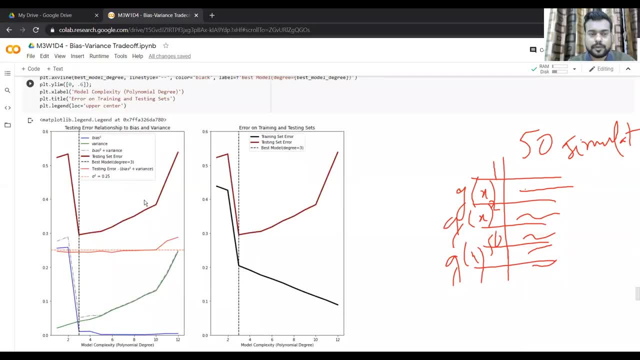 Okay, so you should remember that we're looking at the error Terms across the test data set, at that data set which we have not included in the training right. So we are training our model and then, using that model, We are making predictions on our test set and then looking at how our model is very at the making predictions in this test set. 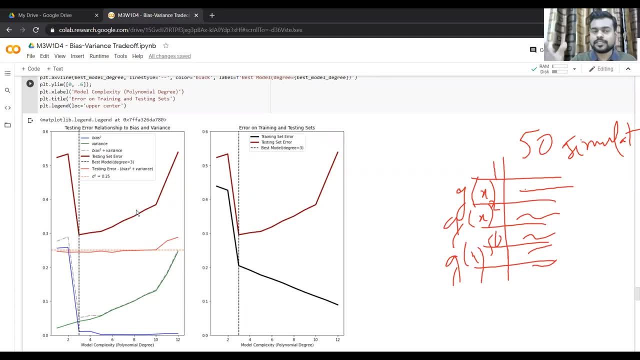 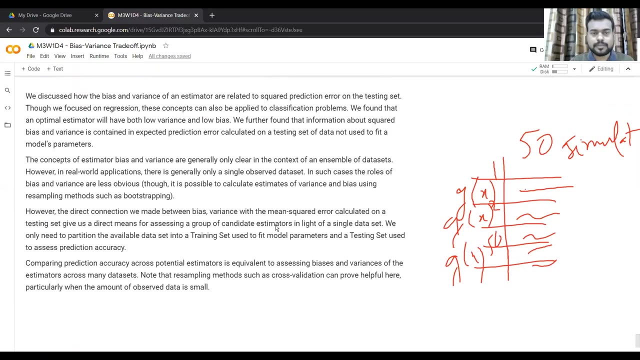 right. So we actually know the true function in this case. So we can sort of calculate all these terms by a squared variance and all these stuff And we can see how the error looks like Right, So again. so of course, in this particular class. 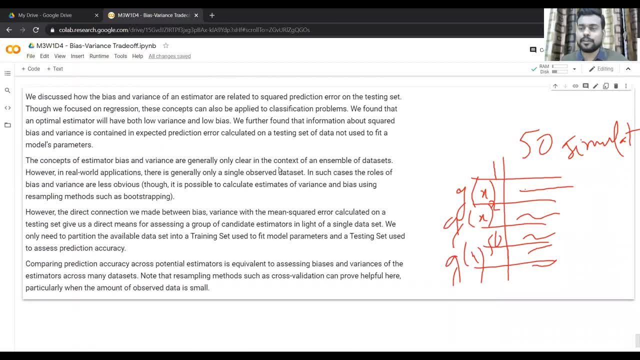 we focus on the regression model, but these concepts can be carried over to the classification problems as well, which will focus on the next week. So so, for an optimal estimator, we want to have sufficiently low variance and sufficiently low bias Right. 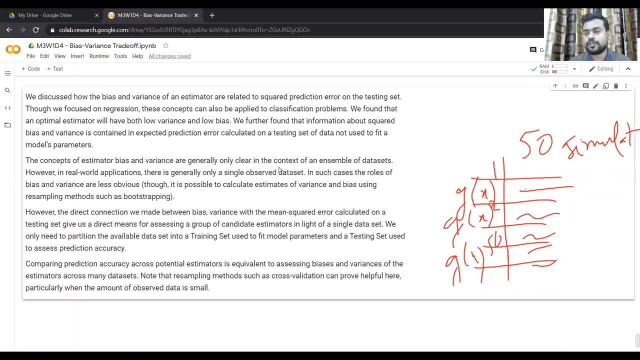 So this is what an hour, What An optimal estimator should look like, right? So so, at the cost of the increase in decrease in variance, right, We'll have a increase in bias, right? So that's how these factors are sort of working opposite direction and we have to find a middle ground. 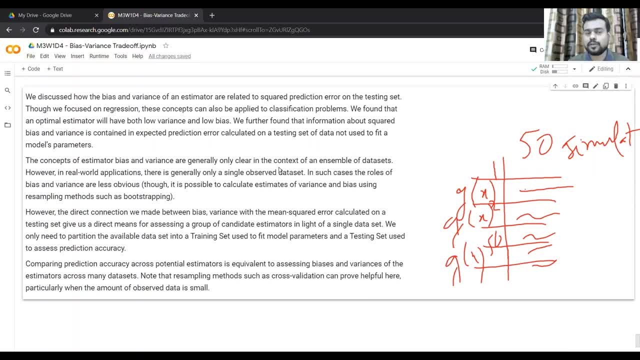 But ideally, will want to have an estimator which has low bias and low variance, So it's not very complex enough, Right, So it has an optimal Complexity. So that's how well, that, that's what the kind of estimator We are kind of, we want to come up with. 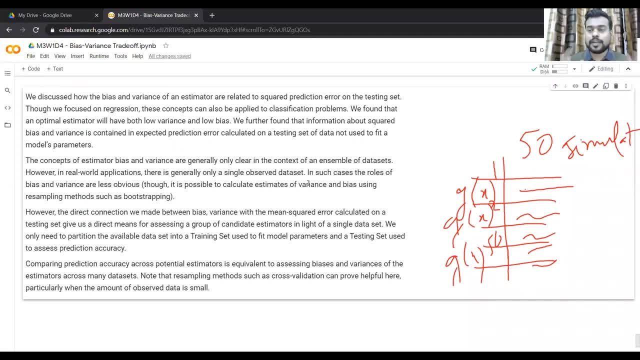 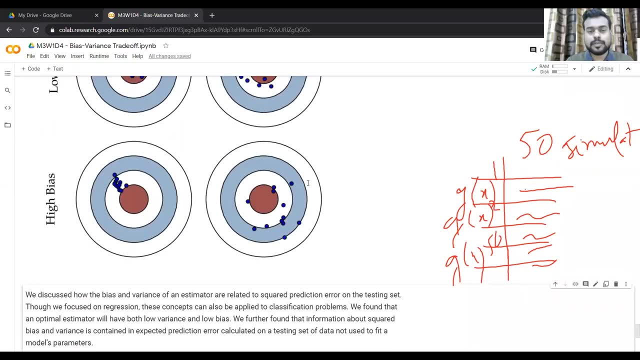 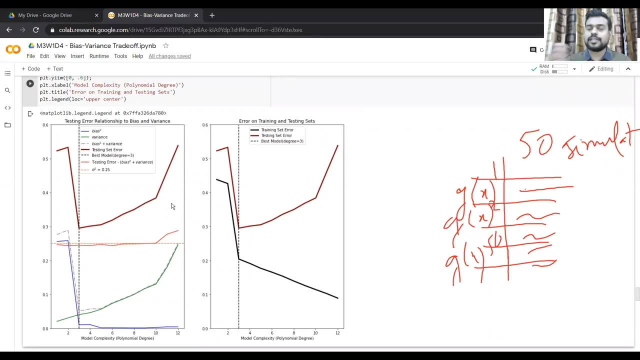 right, Because in machine learning task you want to be very good at your predictions and that will only happen when we have very estimate, good estimated. So this testing error is also called a generalization error, as in how your model is generalizing to an unseen data. 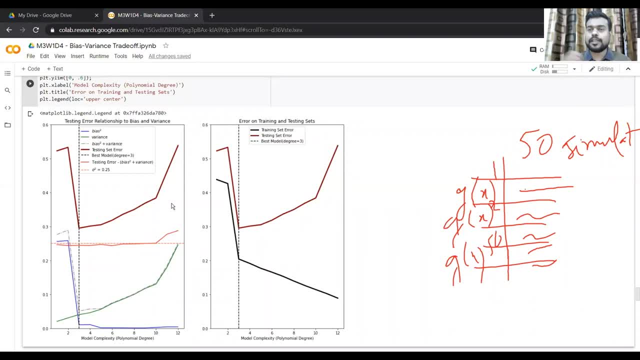 Right, So we have created our model and how our model is generalizing to any unseen data, right? So, as you can see, that if we have a very complex model, so it's not generalizing Well, right, because the error is quite high on this side of the spectrum.